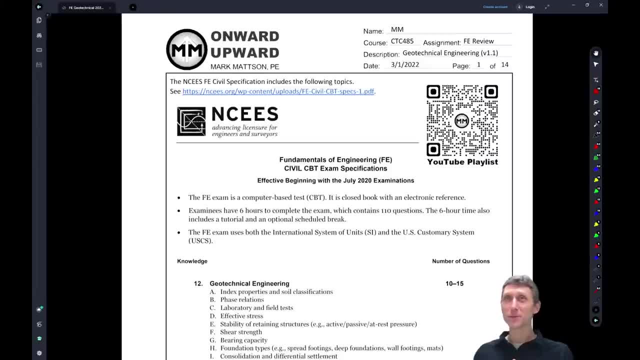 they won't be dirty, Okay, And the puns won't hit rock bottom, but we will try to have some fun here. So, as we get started, what we're going to be doing is we are just going to be working through problems, like we do each week. So this week we are going to focus on geotechnical. 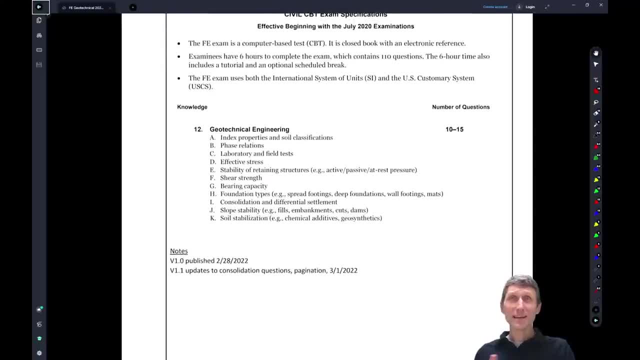 engineering and there are some problems up here. I did make a slight update here, So I reposted and added a problem here today. So if you have you know, previously downloaded this, you can definitely download the new questions. The link is down below, So updated problems are always going. 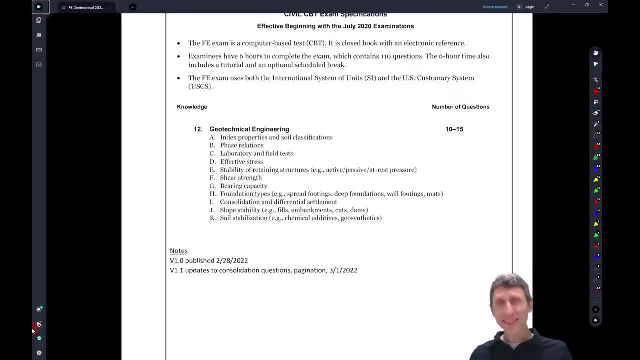 to be there So we can just jump in. There's a lot in geotechnical engineering in this problem set. There's actually a lot of questions that I put in- and a number of those are conceptual questions- just so that I can talk about a few different pieces here of geotechnical engineering that. 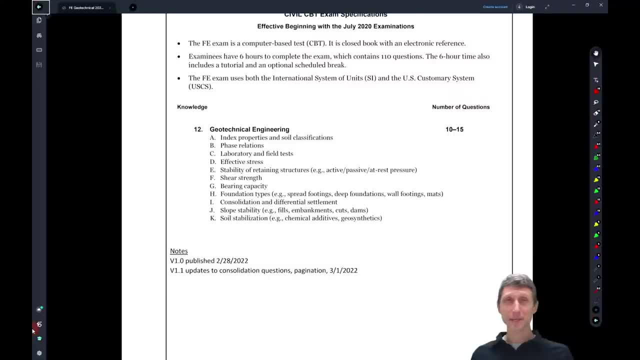 you know, maybe it might not have a huge problem, but they're concepts that you need to understand, And so we'll go through that. One of the things that you notice is, as we look at this, this list of what's on the FE, and actually, if you go back a couple of years I've been doing 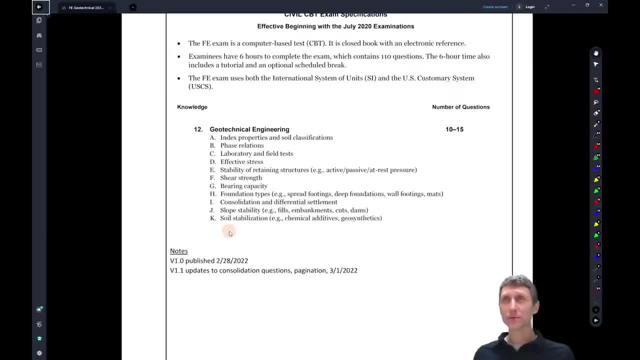 this a few years in version nine of the reference handbook. we're now into version nine of the reference handbook from NCES. In version nine there used to be flow nets. Now there aren't. So I don't put flow nets in this problem set And hopefully you like that I don't. 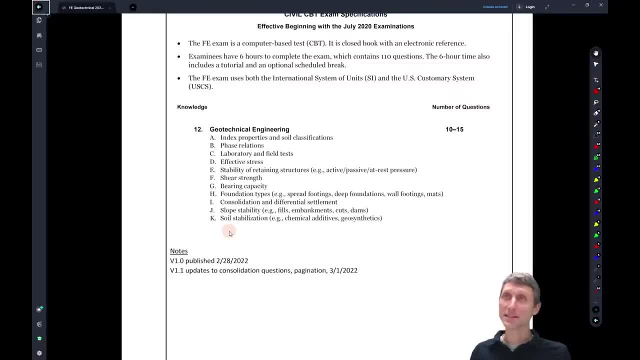 know, maybe you really loved flow nets And we're hoping that there'd be flow nets in this, but we're not going to have those, But index properties, something that you probably are going to see on the test. you know, uniformity coefficient, even that type of thing. 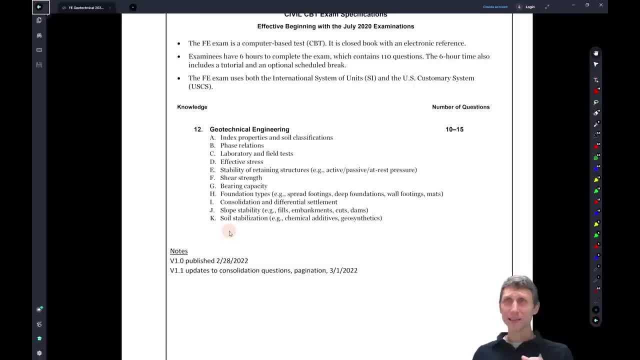 Phase relations, definitely lab and field tests- I think those are going to be there- Effective stress And then some of these other topics. they become a little bit more plug and chug, but we'll. we'll go through some of these problems and hopefully you'll get some good information as. 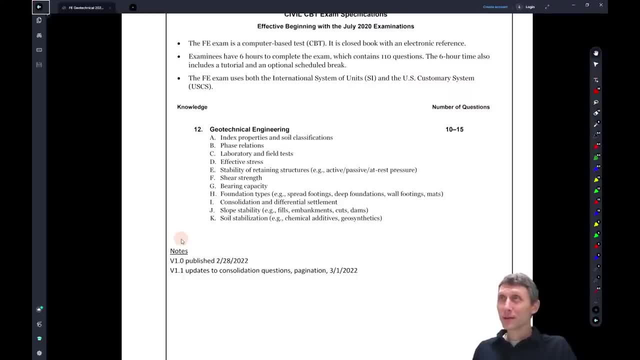 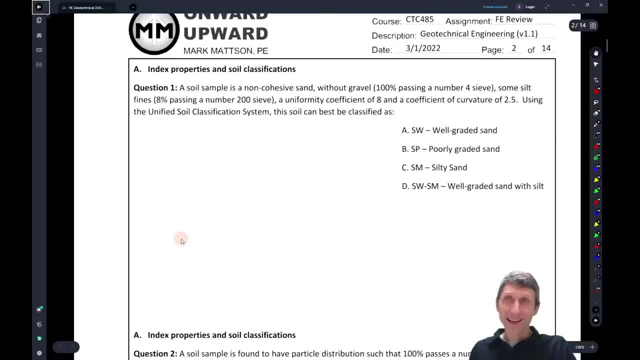 well, So as we go, you know, definitely feel free to put a comment in the box, but let's just jump in here. So, index property soil classifications number one, right? So what we have here is, anytime you see a question where you have to use a certain classification system, 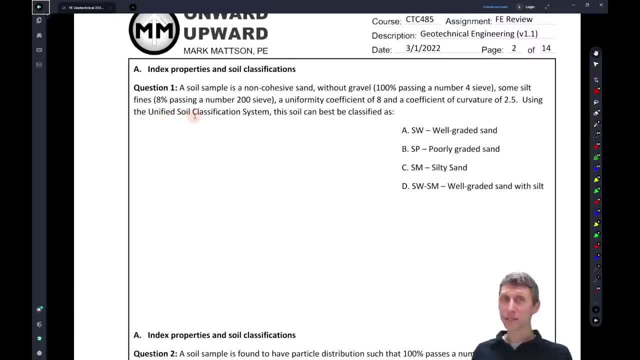 the first thing that you want to do is go find that classification system, right? I mean, you have to understand the soil properties here. So, yeah, we can understand the soil properties. Like we have a non-cohesive material, Typically sand- is not cohesive, It doesn't stick. 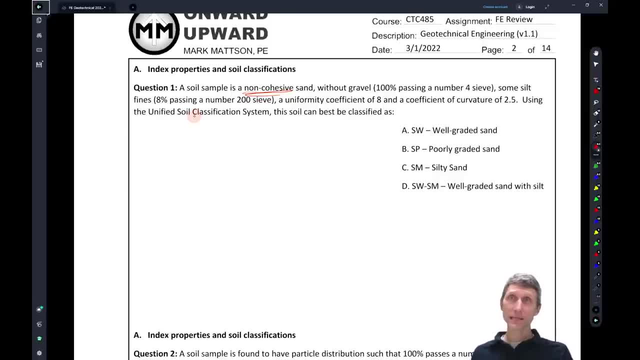 together right Without gravel. So we have a hundred percent passing number four sieve. So right away we know that we have a sand- it's primarily sand, but we have some silt. we have 8% passing a number 200 sieve And that number 200 sieve is the distinction between your. 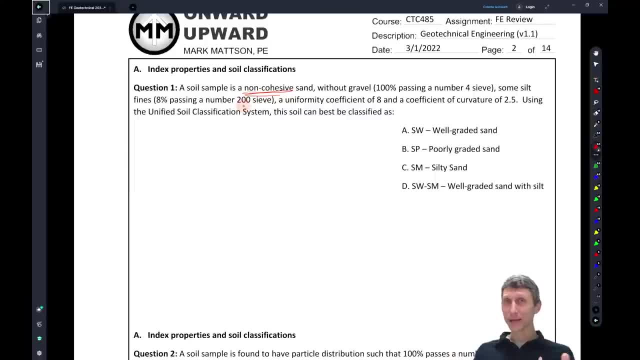 your sands and your silts and your, your clays, your sands and your fines, right And your granule, your cereal and your fines, and a uniform coefficient of eight, a coefficient of curvature of 2.5.. And we're told the unified soil classification system is to be used here. 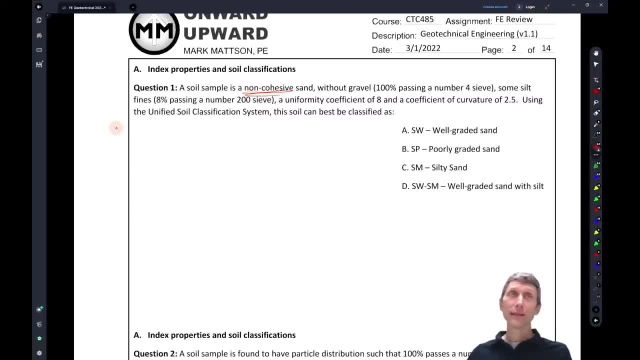 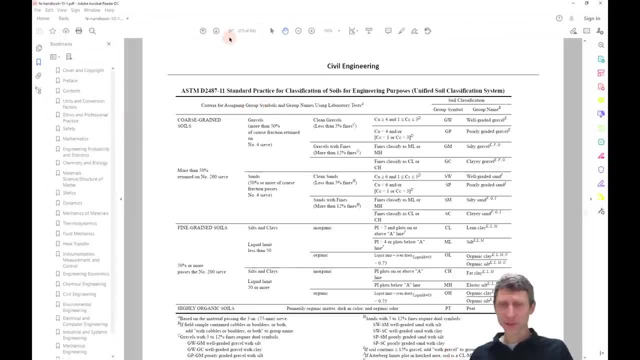 So this soil can be described as what? So in the epi reference handbook- and that's where we're going to go to start here- the epi reference handbook has this in. So if this is the latest version of the manual, I think, but it's, it's page 267 of the PDF. I'm trying to think here. 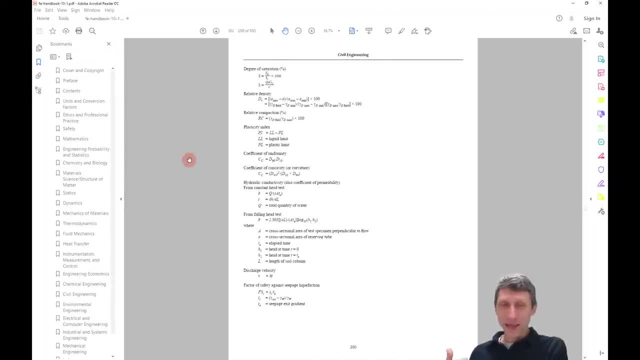 the. this is kind of far down in the geotech and actually it's kind of interesting- is civil engineering starts with geotech. I don't know, maybe it's because from the ground up, I don't know, but we get to start with geotech here And 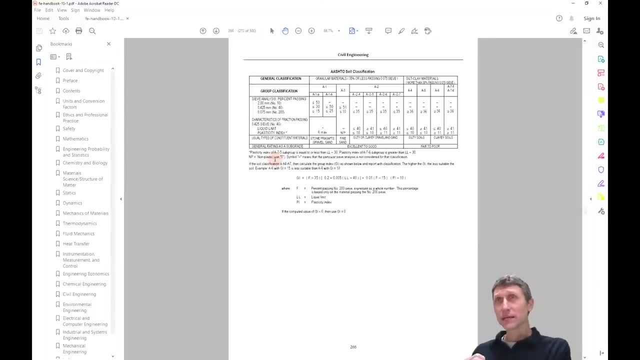 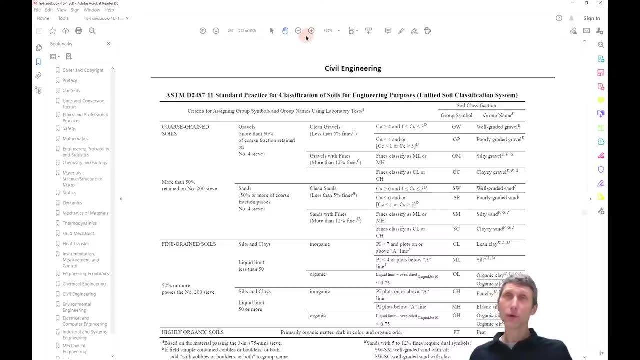 you know, a few pages in we get to the USCS soil classification system. So we'll go through some of these other pieces here. But this is where we're going to start And if you remember, what we were told is, we have 100% passing a number four sieve. So what you see here is number four sieve, is that? 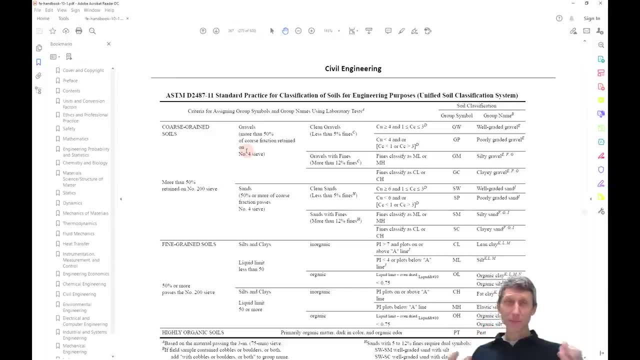 distinction, that dividing line between sand and gravel and number four, sieve, I mean it's. I think it's like 4.76 millimeters, So it's. it's, if you think of a number four, is kind of like a four millimeter. it's a little bigger than that, But it kind of gives you an. 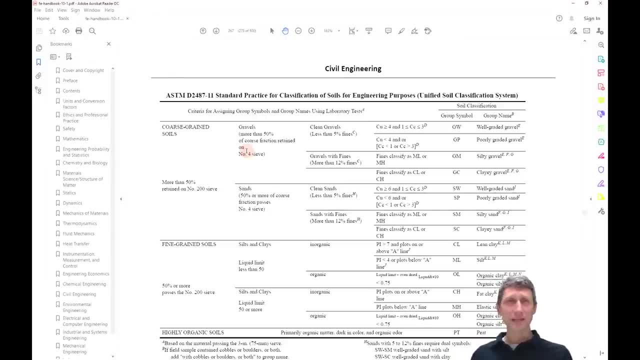 idea, maybe three, sixteenths of an inch type of type of thing. it kind of gives you an idea: bigger than that's going to be rock or gravel, smaller than that is going to be a sand. and then the number 200- sieve is where we get into the fine grain soil. So that's even pretty small. 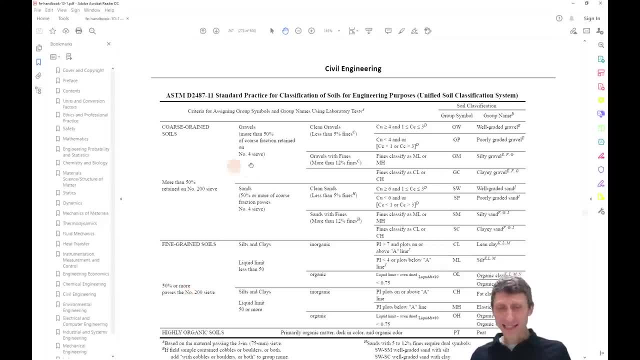 it's less than a tenth of a millimeter. So this tells us: we're in, we're in. you know, everything's passing. a number four sieve, So we're in a sand. And then where do we go from there? Well, we don't. 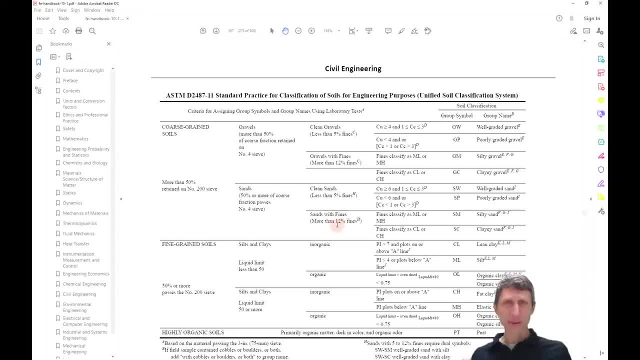 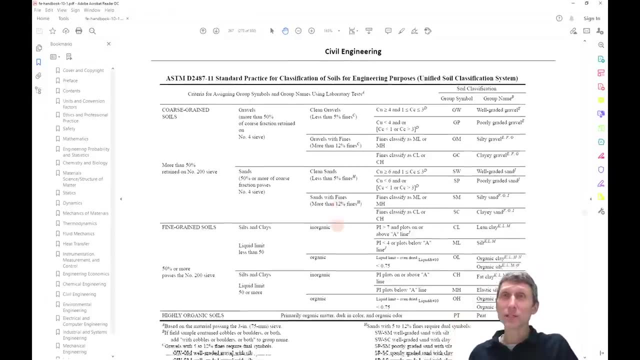 have less than 5% fines. we don't have more than 12% fines, we have 8% fine. So right away, this problem is sort of maybe a bad problem, Or what this means is actually: you have to go down and 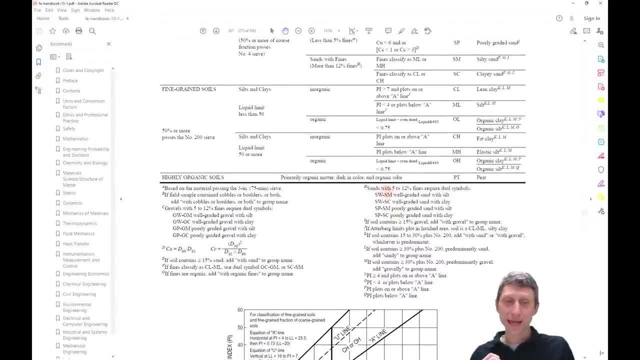 look in below. So below, what we see here is we actually have some sands with five to percent, five to 12% fines required, dual symbols. So the thing is, we can still use this even though we don't have our five to. you know, we're not less than five. 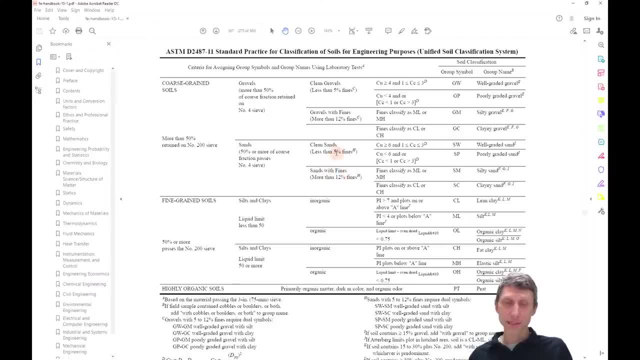 we're not greater than 12. We're still kind of in this range, though. So let's keep going with sands. And what we see here is we have a uniformity coefficient here of I think. well, let's go back and see what we had, I don't remember. So this, this uniformity coefficient was eight, the 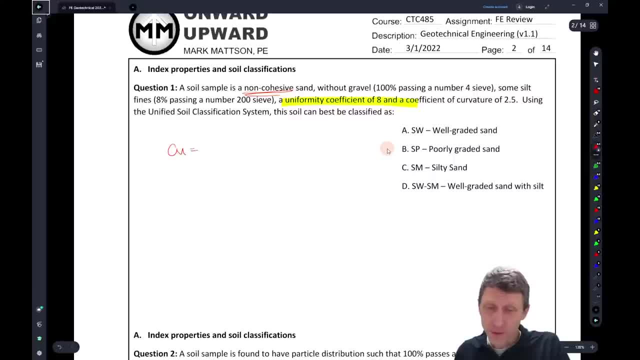 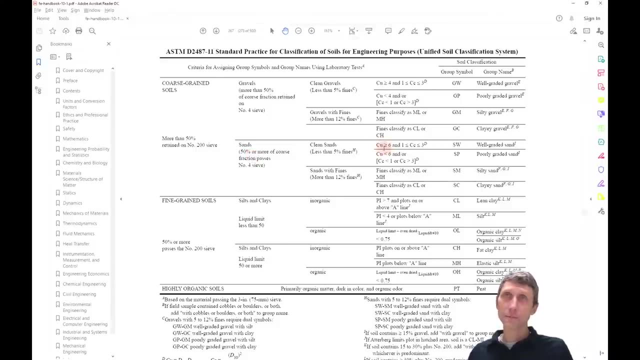 coefficient of curvature was 2.5.. So the uniformity coefficient is eight And the coefficient of curvature is 2.5. Okay, so that tells us something here. So if we come back, what we see is: we're greater than six, right, we're greater than six for uniformity. We're, what was, what were we? 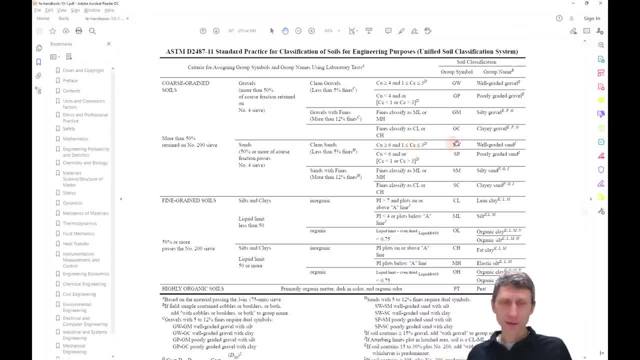 we were 2.5.. So we're in between this one and three. we're kind of a well graded sand right. But you have to remember we didn't have less than 5% fines, So what that means is instead. 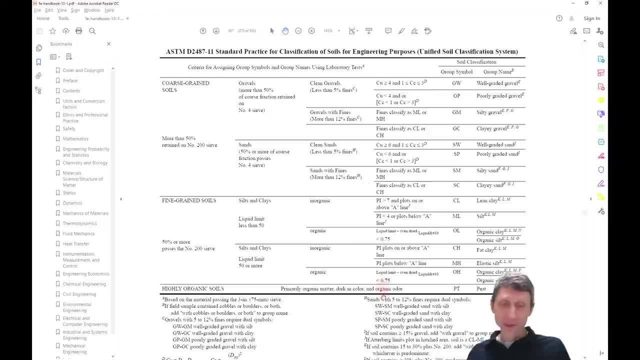 of having less than 5% fines, we have 8% fines and we're going to come down here and we're gonna have a dual symbol, Okay. so we're kind of in this well graded condition: the uniformity coefficient, the coefficient, the higher value. 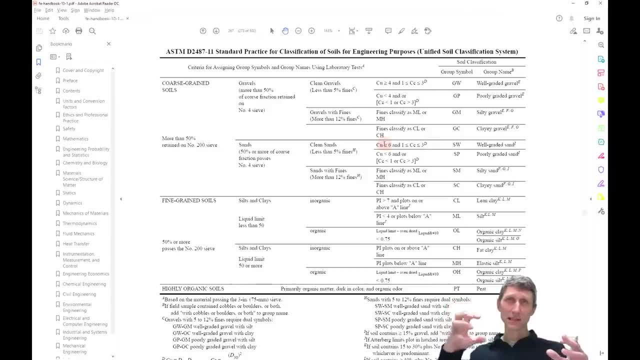 means it's kind of well graded. there's a good distribution size on there. It's not just like beach sand, where everything's the same. So what that means is we're going to come in here, we're gonna say this is going to be a well graded sand, But it's a well graded sand with themselves. 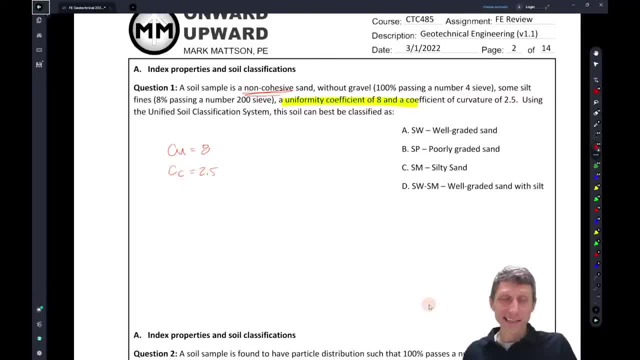 So if we come back, we hope that's in the in the list above And good news is it is. so we have well graded sand with self And that's our answer. So you have to understand some of these pieces, But you also have to understand some of the footnotes to the tables as well. So hopefully, if you get, 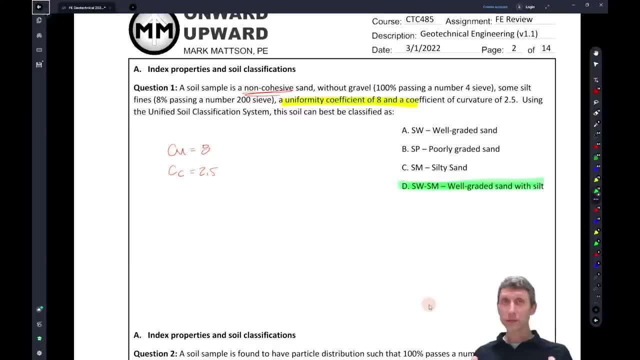 one of these questions. they're pretty straightforward, Honestly. hopefully it's pretty straightforward. You can just push it right through and go through the kind of the algorithm of that classification system and get your answer. So hopefully that's what happens with this next. 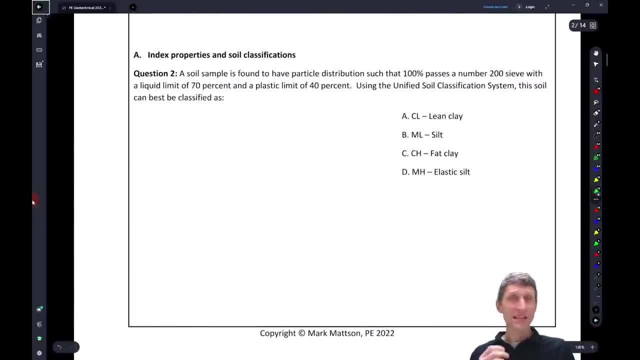 one right. This next one is similar. It's same type of thing, It's just using uscs. But now we're going to go back to the first one, So we have 100% passes, a number 200.. So, again, that's the. 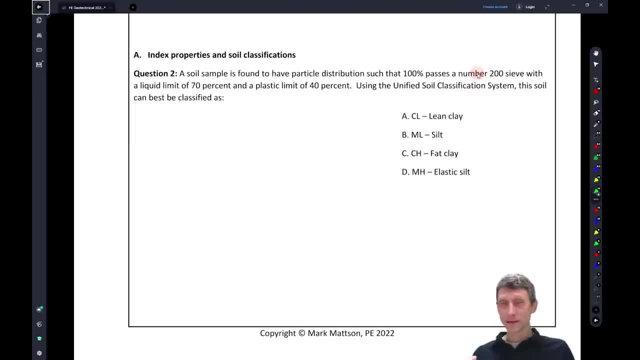 dividing line between the sandy soils and the fine grain soil. So even 100% of the passes, a number 200.. So this is your silts and clays, a liquid limit of 70%, of 70% and a plastic limit of. 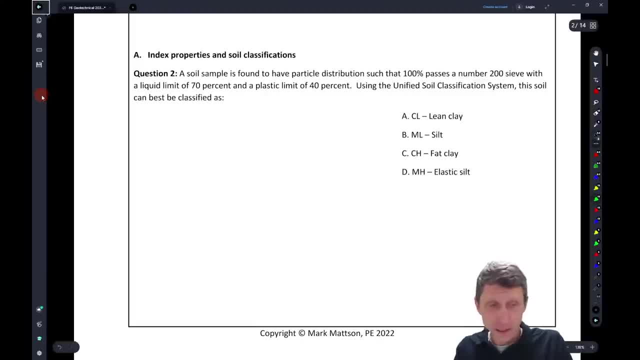 40%. So the liquid limit. oops, let's change this here. So we have a liquid limit of 70 and a plastic limit of 40. Using uscs, the soil can best be classified as well. let's go back to uscs and see. 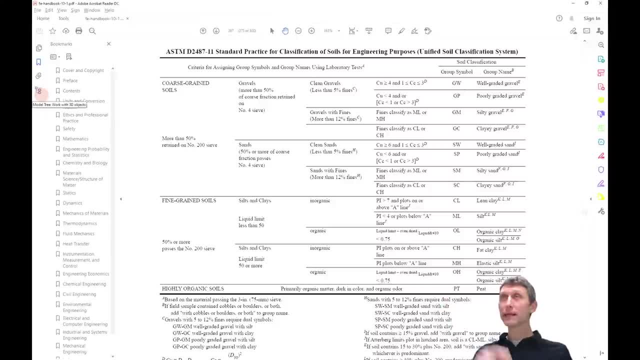 what we have to say. So, Sammy, it is up there now, So I just cut it up, So I apologize for that a little bit late, but it is there this week, So, um, so, so you should be able to find it, Hopefully, you. 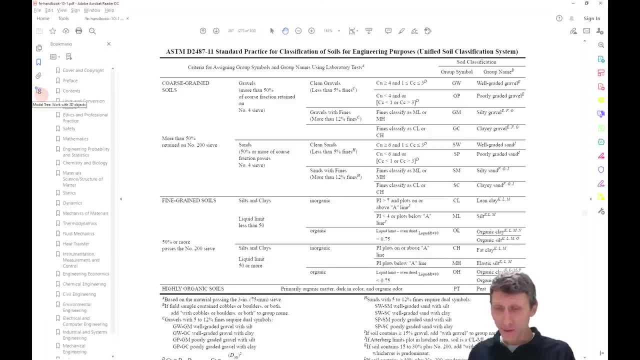 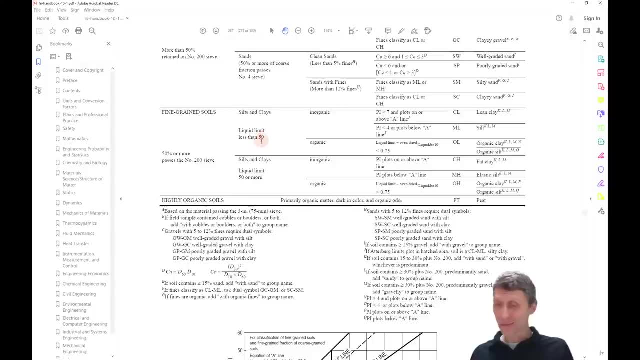 can get on that now as well. Okay, so we're back here. We're looking at fine grain soils. We have a liquid limit. I think we said that was 70. So we are. we're not less than 70.. We're more than we're more than 50.. 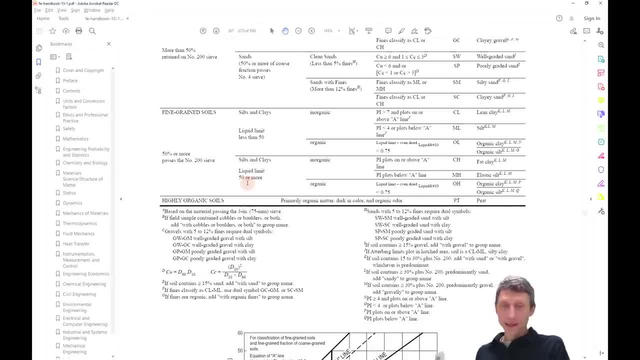 Okay, And what you'll see here is we, if our liquid limits more than 50, we are looking at a plastic limit of 40. But the problem is this: doesn't this? looks like a PL almost, but it's actually pi. If you look closely, that's a pi. So what's pi is pi. 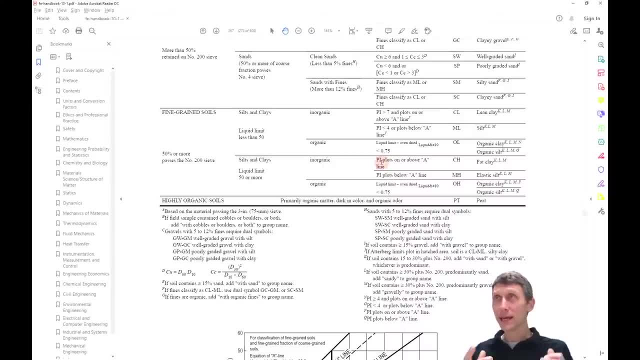 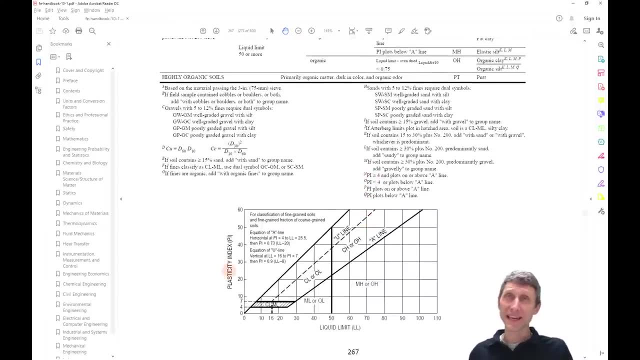 plastic limit. Hopefully you see that it's not And what we see here is the pi is actually going to be. if we come down here a little bit, this is the plasticity index And this is just a index of how kind of stretchy the soil is, if you will, right. But what this takes into, 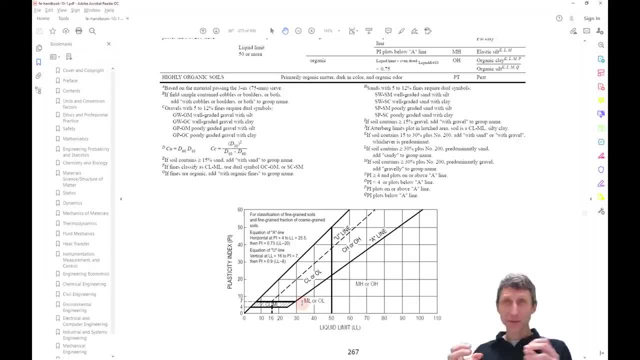 consideration is kind of the difference between the liquid limit and the plastic limit. That's our plasticity index, right. So the liquid limit, if you remember it's that machine you kind of crank, crank, crank, crank, crank and you get, you know, until the soil comes together. Maybe you 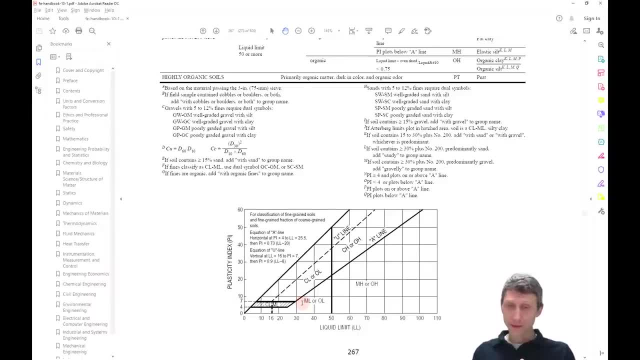 remember that lab where you did it. The plastic limit is where you roll it down and get that that eighth inch diameter. You get a 360, I think three sixteenths inch diameter. roll kind of eighth inch, three, sixteenths until it crumbles and you find out what those limits are. 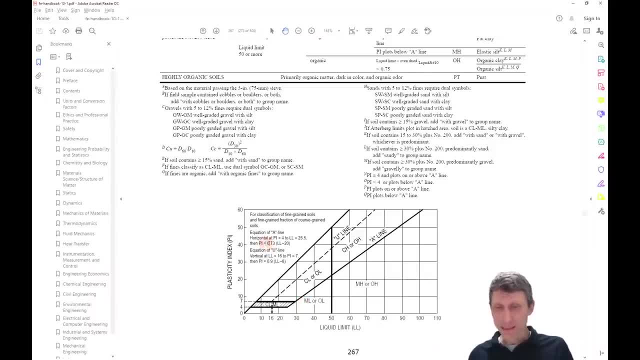 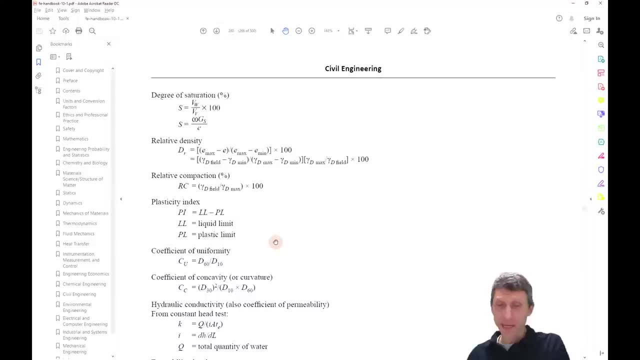 right. But the plasticity index right. the plasticity index is the difference between those. we could look at that here as well. So if we come back a few pages in the reference handbook you see the plasticity index, pi is the liquid limit minus the plastic limit. So let's just 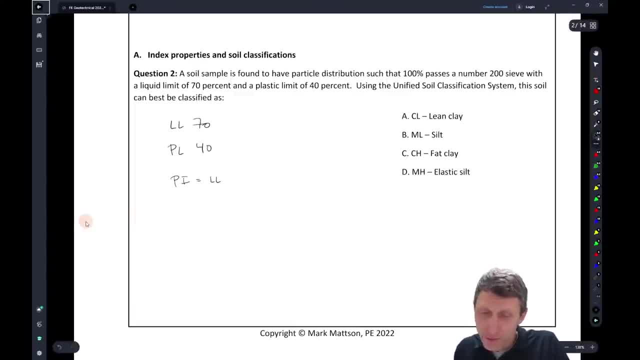 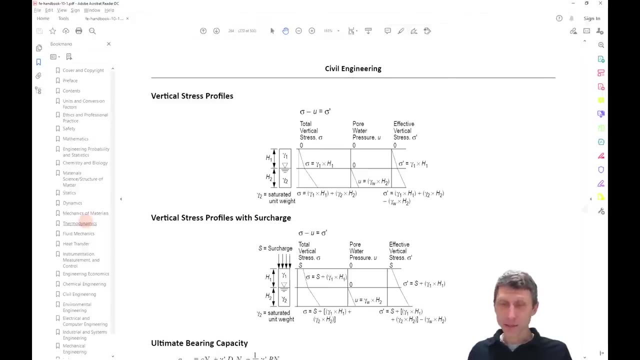 figure that out here: The plasticity index is the liquid limit minus the plastic limit. So what's that? 70 minus 40. And that's going to equal, you know, equal 30 here. So we'll plasticity index. And that brings us back to our USCS. So let's come to our classification. 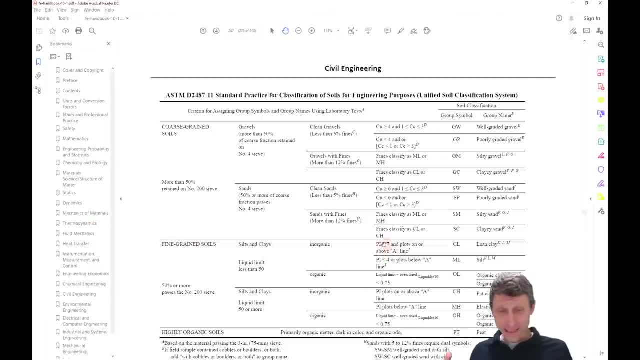 System. And what do we get? We get a plasticity index of greater than seven for sure. But let's look at this. Let's look at: we're not in organic materials. We don't have any, any organ, I'm sorry. 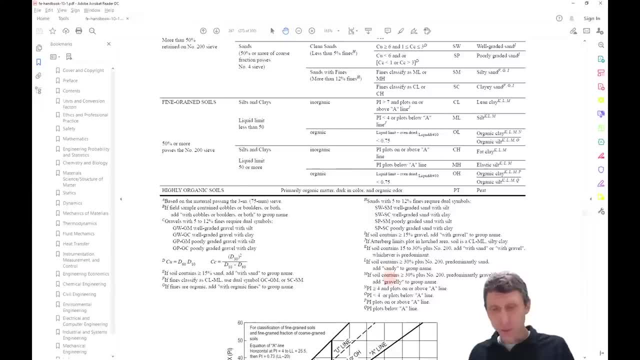 we don't have any organic materials. But let's come. let's come back over here. We were at a liquid limit of 50 or more, So now we're looking at the a line. What's the a line, right? We're. 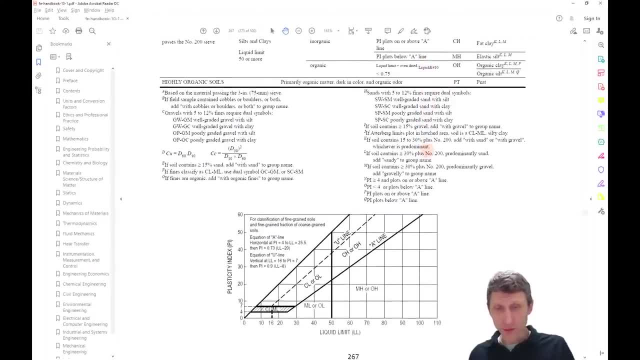 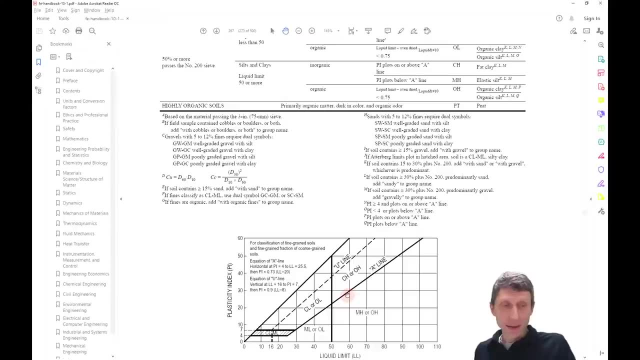 looking at an a line here. So let's look at this. Well, it's, if we keep coming down here, What you see down here is we have what's called an a line. So I can take a look at this a line. But let's look, we have a plasticity index which we got as 30,. 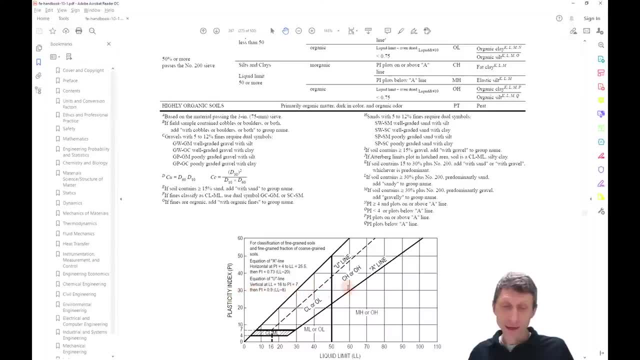 right. So 30 is this, this line across here, and our liquid limit was 70. So we're firm, kind of, on this point And if this is the a line up here, we are going to be below the a line right. And if we were used, if we did our plasticity index wrong, right kind of use that. 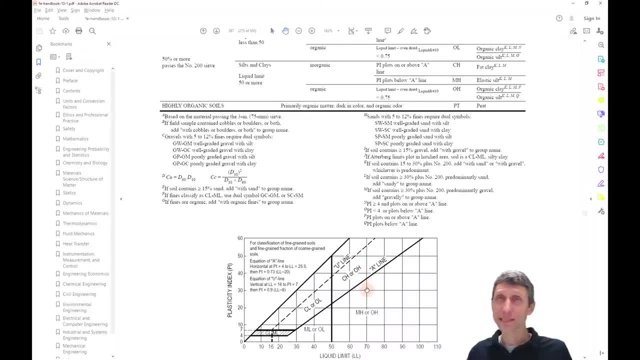 plastic limit, we would be above the a line. So you got to be careful with plasticity index versus plasticity plasticity limit. So we're below the line. Right here we have more than 50% or more than 50 of a. 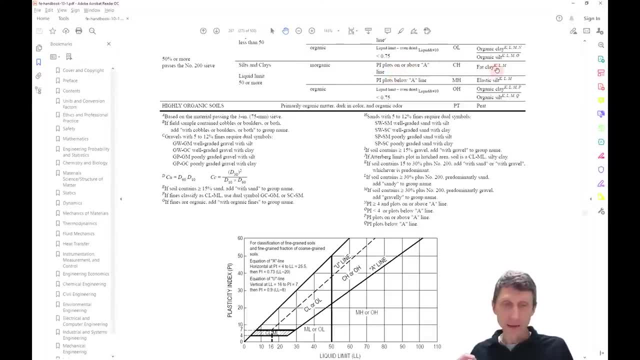 liquid limit. We are above the a line, So we got that clay going on. How's that sound? Is that right? Or did I do something wrong, Or Oh no, I'm sorry. We're below the a line, right, Sorry? 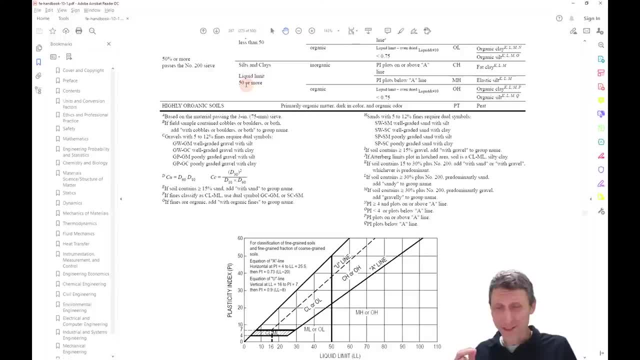 I think I read that wrong. We're: we're a liquid limits 70.. sink to go through all the work and then get it wrong. right, but yeah, so we're liquid limit more than 50. we're below the a-line rate. our plasticity index was 30 and our liquid limit was 70, so we're. 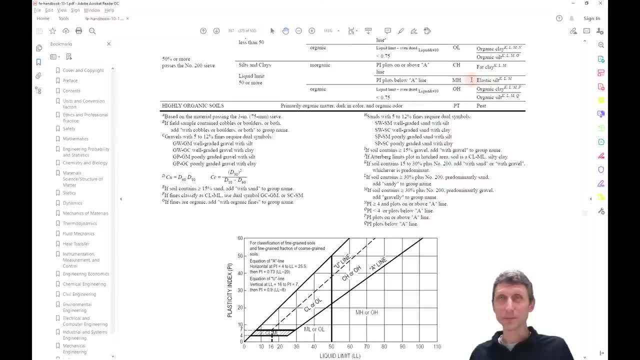 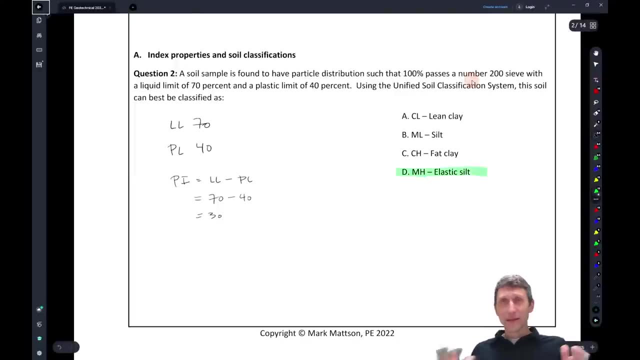 below the a-line, if that means we're at this, this elastic silt, okay, so we can come back here and, um, we can select an elastic silt. so, again, it's just knowing some of those terms, knowing what they mean, knowing where to find them and hopefully, uh, that's gonna gonna help you with. 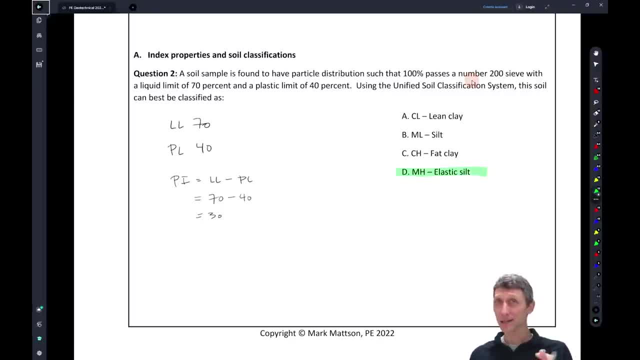 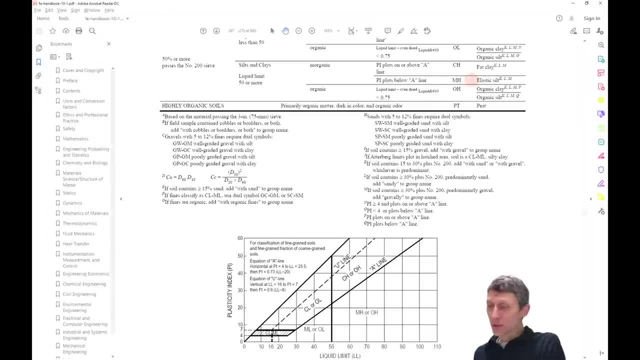 those. but i honestly, if you get a soil classification, i hope it's just kind of plug and chug. you look it up and it's not. it's not too crazy, okay, but there's, there's the uscs, there's also, i mean, if we come back and look at this, there's also an ash toe classification. so you 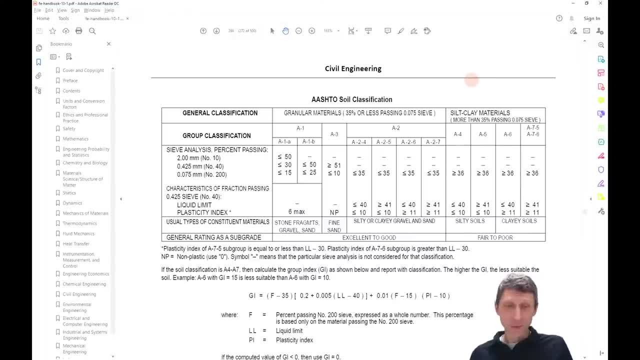 could be given something similar here, uh, but again, what we have here is is another classification. so if you have more than you know, more than 35, passing at 0.075 sip, that 0.075, that's our number. 200 sip. right, that's the the. 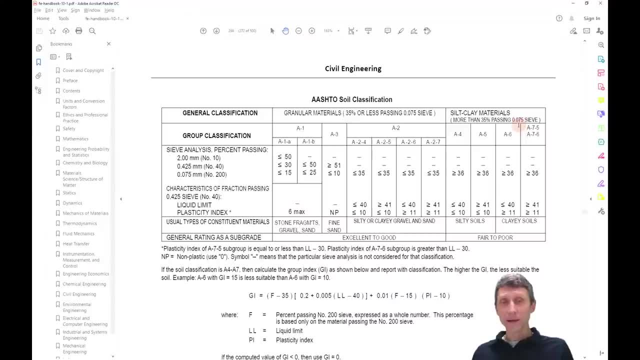 the small sieve, um, that distinguishes between uh, between fine uh, fine silts and clays and granular materials. and again what we have here is we have, you know, more than 35 percent uh passing a 0.7 five sieve and then the liquid limit, plasticity index, same types of things. right, we're greater. 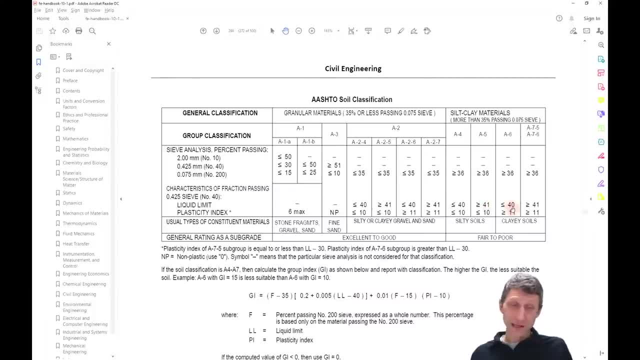 than 40 and our plasticity index is greater than 11. right, we're greater than 40, greater than 11.. we're going to be kind of in in in this range. a clay, um soil is what it's sounds like here, right, so um it's. you know, the the different. if i'm, if i'm doing that, right am. 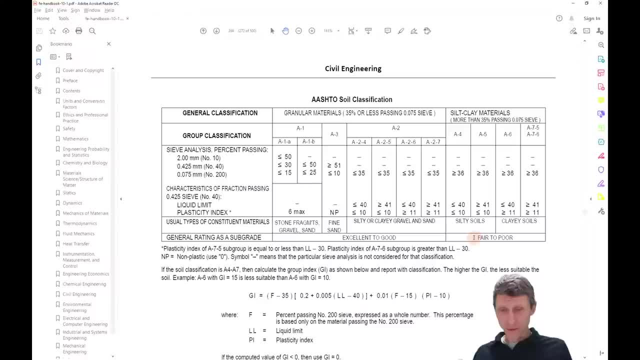 i looking at that right, uh, i'm i'm getting confused. so our liquid limit is greater than 40. plasticity index: uh, was, was around 30, i think. so yeah, we're in this, this side of things. so they, they distinguish the, they're the classify the soils a little bit differently, uh, but it depends. 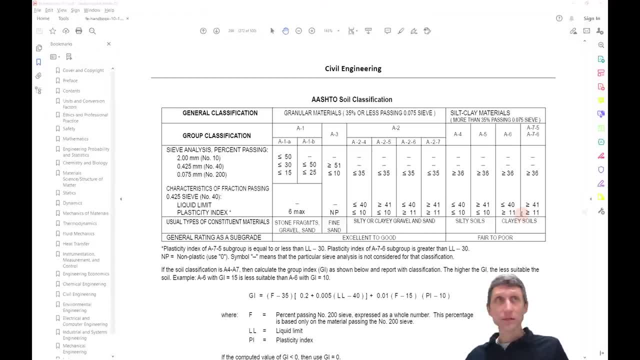 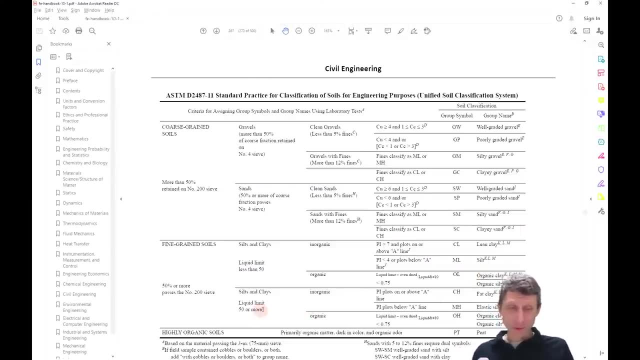 on kind of the two systems, uh, that you're working with here. so, um, in this one we- we specifically said the uscs, so you know, liquid limit more than 50, we're below the a line, and that's what we're going to go with, okay. so, as we keep going here, though, what we're 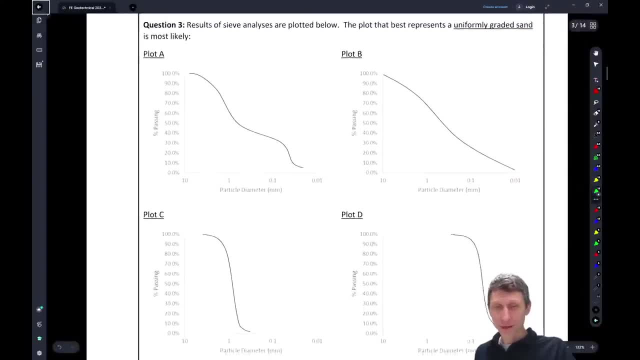 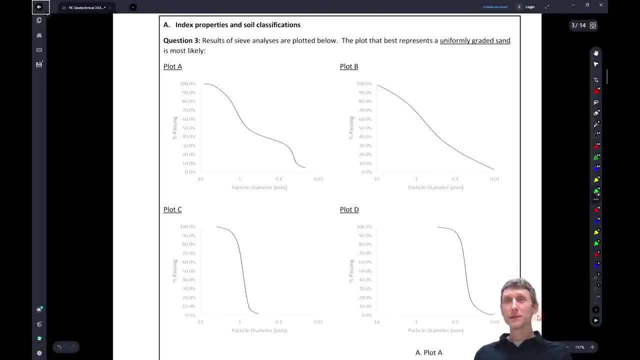 going to do is some of these questions are going to be kind of quick, some of them are going to take a little bit longer here, but, um, this one we could take a take a quick look at, or we could take a little bit longer. this one i kind of threw in there just because, um, sometimes when you go on, 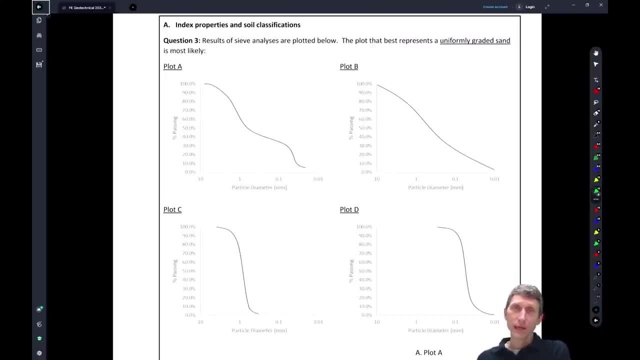 a job site, or when you are looking at a job site and you're looking at a job site and you're looking for materials and, uh, when you specify any materials as an engineer, what you'll get from the contractor- or maybe you'll be the project engineer for a contractor- what you're going to. 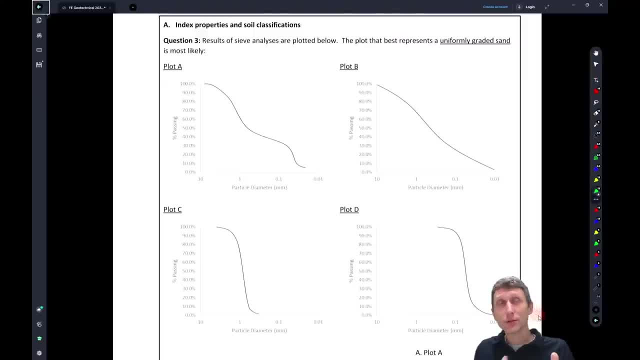 do is you're going to get a sieve analysis of that soil and you're going to give us. so you're going to go to a borrow pit or a test pit and take a sample material, get a sieve analysis done and send it off to the engineer and say: is this good? and then the as the engineer you're going. 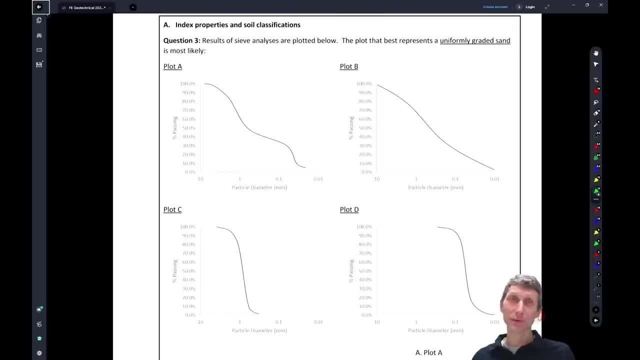 to have to say like: yes, it is or no, it's not. you're going to have to approve or not approve the material based on what's in your specification. so a lot of times the first that's done, especially for granular, granular materials like a uniformly graded sand, is going. 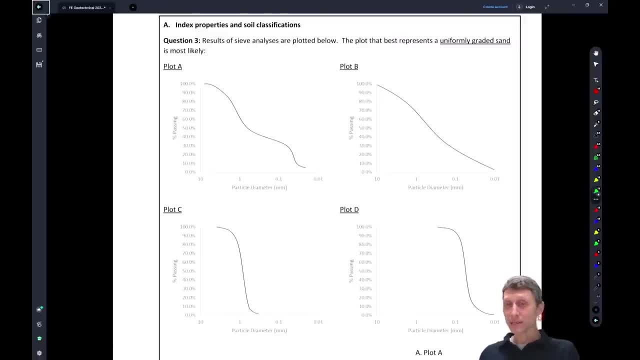 to be a sieve analysis. so the question that is asked here is: we are given a whole bunch of of sieve analysis results, right, and the question says which one's uniformly graded sand. so can you look at these sieve analyses and know what's uniformly graded? i mean uniform. 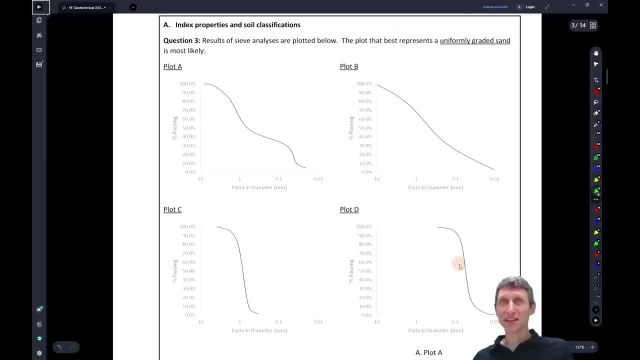 you might think: well, you know these two sort of look alike. i don't know this one sort of, this one does, just doesn't look uniform. this one sort of looks uniform, i don't know, does it? this is where you have to understand what a sieve analysis shows. 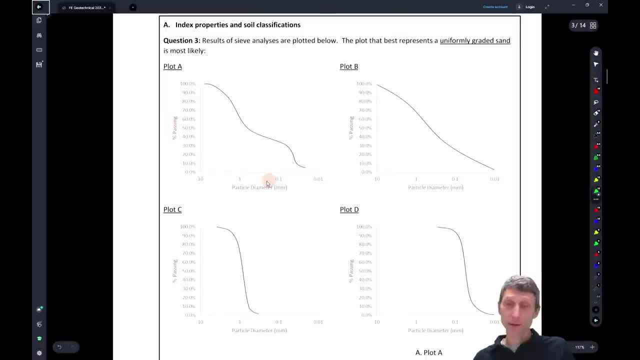 so sieve analysis says the percent passing in a particle diameter. this is a log base scale. and i mean, if we look at this, what you see is, uh, with this one you have a chunk of material that passes right here, a chunk of material that passes right here, and, and this kind of gives you 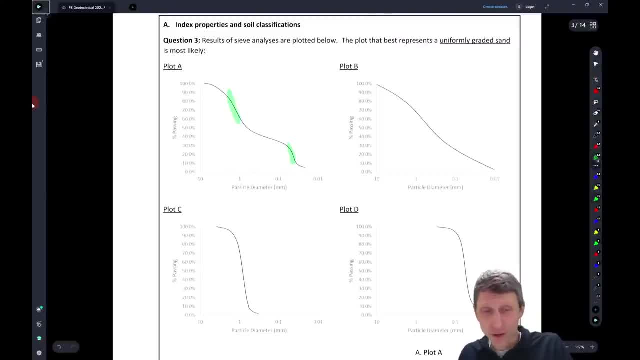 an idea that this is what we would call- or geotechnical engineers would call- like a gap graded soil. right there's, there's kind of a couple different pieces that are better put in there, a couple different particle sizes. um, that get that, get in there, and this is a gap graded soil. okay, so this one, it's not a uniformly graded sand, okay. 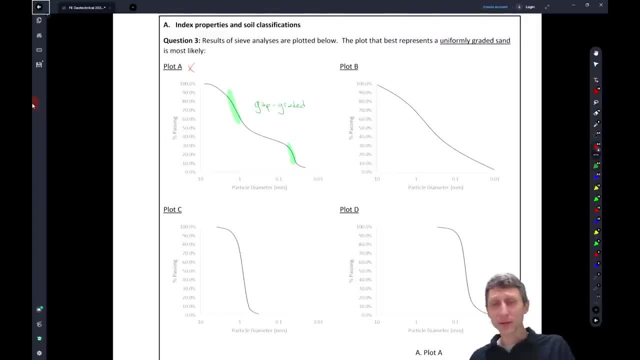 so we can get rid of that one. and then we get to bc and d. right, and the question is: what is? what do these mean? right? what this, this curve, means here is that as you go down and get progressively smaller with those sieves, you remember how the sips are. you get a bunch of pans, put some soil on the top, then you shake them right. 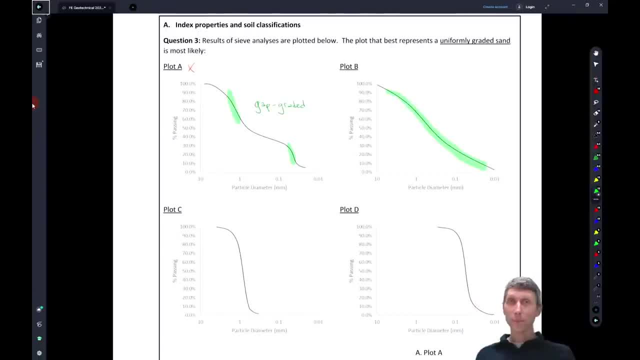 and the, the particles kind of sieve out and you kind of figure out, um, what sizes each of, or you know what sizes of particles you have in the soil, right. so with what we're doing here is is: is this shows, you know, this curve shows that you have a pretty good distribution. this is actually not. 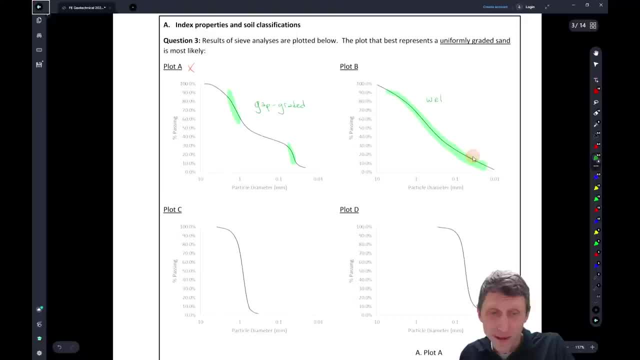 uniform. this is actually what we the consider like a well graded soil, right. but then we get down to these two. we see uniform soils. these are both uniform soils, so these are both uniform soils. these, this is a uniform soil and this is a uniform soil. sometimes we'll see that called a poorly graded soil. actually, if you come back to 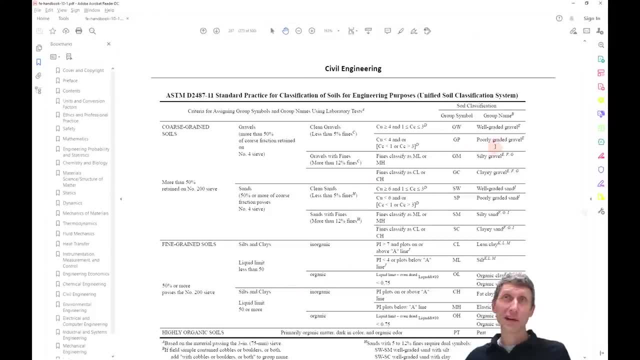 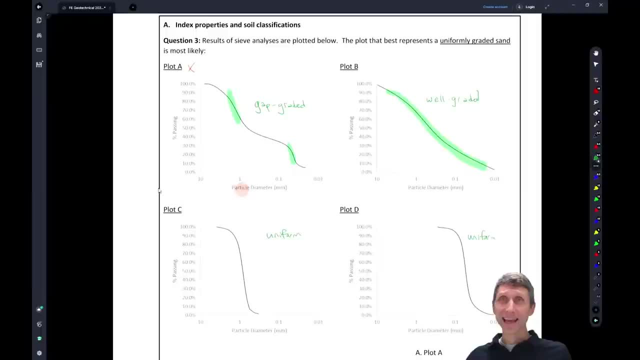 uh, the reference handbook, for a second. what you see it here is you have poorly graded sand. it's not called uniformly graded sand, it's called poorly graded um. it might also be called uniformly graded in the sense that this is your beach sand, this is the, the sand that's all kind of. 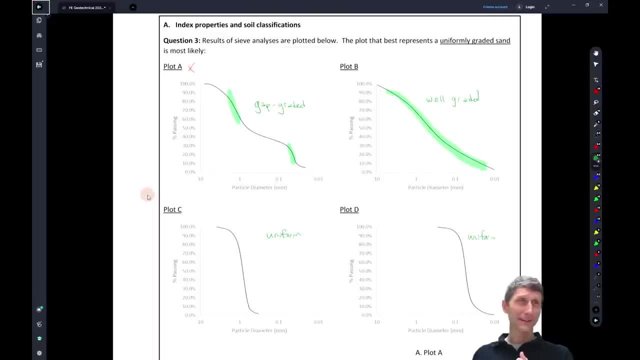 uniform and it's, you know, you can use it for, uh, you know, for leveling. at times you can use that under, uh, certain, uh, certain pads or equipment, uh, but this is, this is a uniform, a uniform soil. okay, so what it means is you, you kind of get to a certain sieve and all of a sudden, all it all. 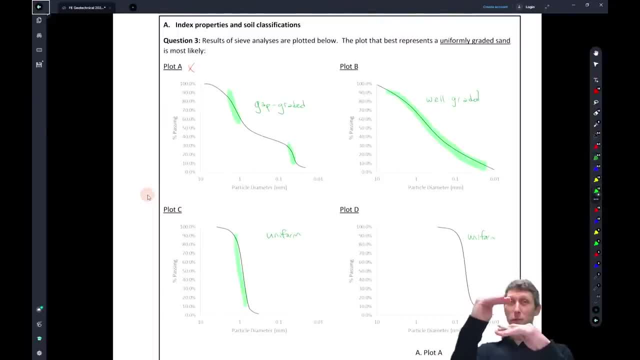 goes through, but then it stops on the next sip, if that makes sense. it's like it all passes through, kind of the idea here. and this is: this is going to be a uniform soil, now, which one is going to be sand? and this is again where, if you, if you know a couple of, a couple of sieve sizes, um, one sieve, 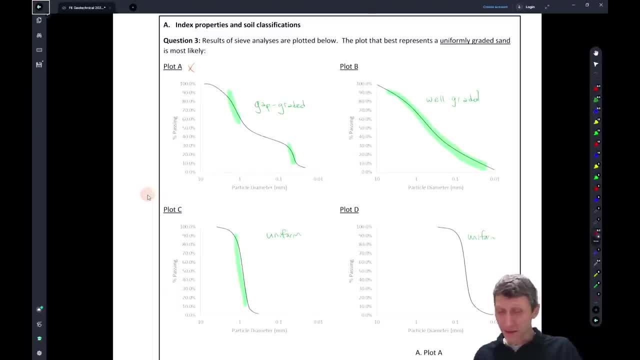 size is going to be that number four sieve. it's remember said it's about five millimeters, about four millimeters, five millimeters. um, if we look down here, we got one, two, three, four, if i'm counting right, five. so our number four sieve is somewhere around here and that number 200, if you remember. 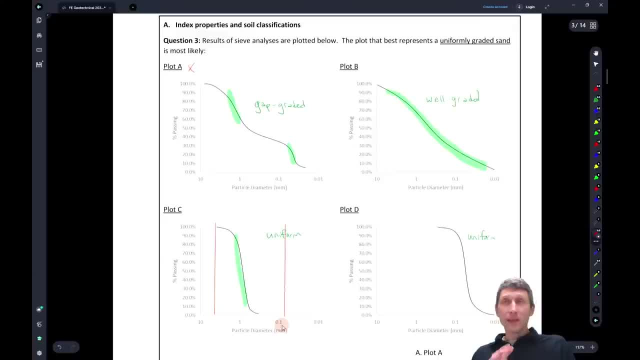 that's going to be somewhere down around here. So this is firmly in the middle of the sand. It's firmly, looks pretty good And this is going to be our uniformly graded sand. So this is like a number four sieve. This is like a number 200 sieve, Right, And how is this different than? 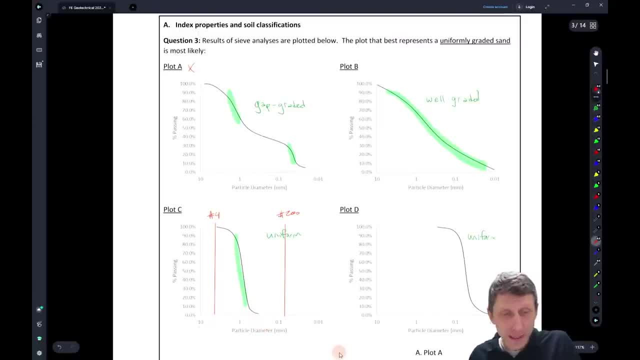 this one right. here It's different because, again, if we look at that number 200 sieve or number 200 sieve is going to be somewhere around here, Probably not getting it perfect, But what you see here is this is our number 200 sieve, Most of most of the material on this one right. 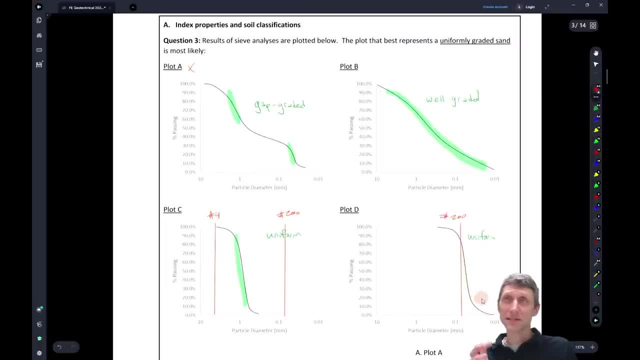 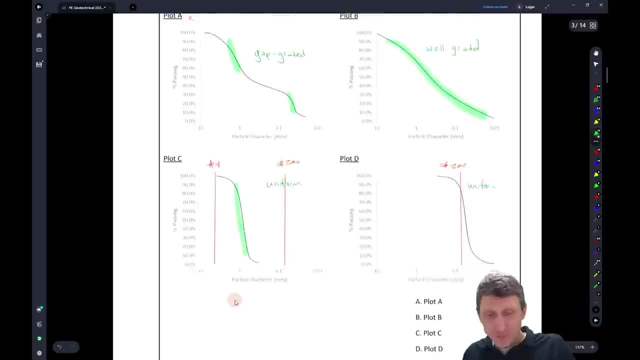 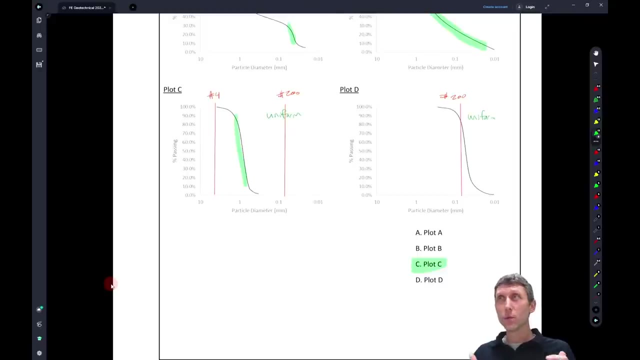 here is going to be is going to be in that fines area. This is going to be more of a uniform silt or clay. OK. so plot C in this one is going to be our uniform, our uniform sand. OK, we could also take a look at this, because what we see here is we could go and we could actually 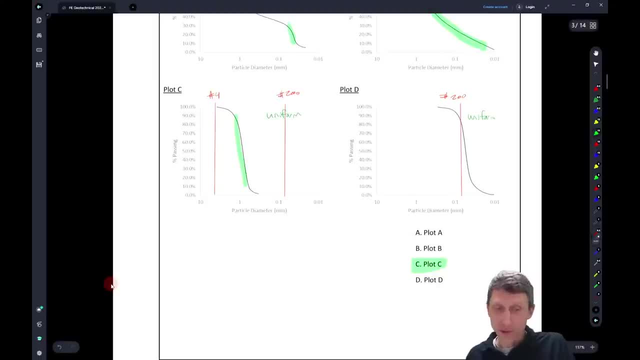 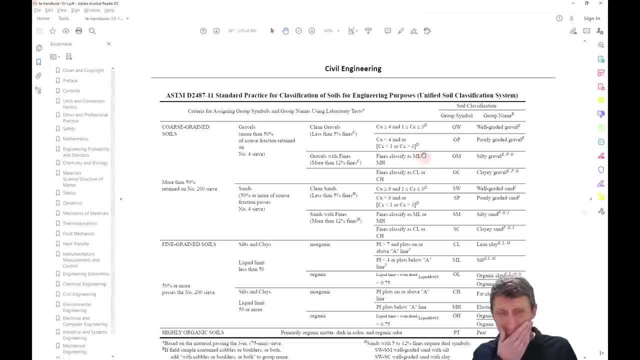 start to Calculate a few things. Right, If we wanted a more numerical approach, what we could do here is we could say: well, let's take a more numerical approach to this, because if we come back to our classification system Right, What we see here is CU is less than four for poorly graded sand. 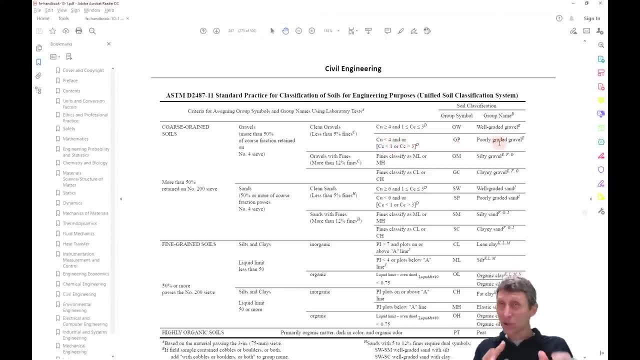 CC could be less than one or greater than three for poorly graded sand. Again, that's a uniformly graded sand. It's very uniform in size. The particle size don't have a lot of variation. They're not well graded in terms of they're all. it's kind of like those glass beads, that are all. 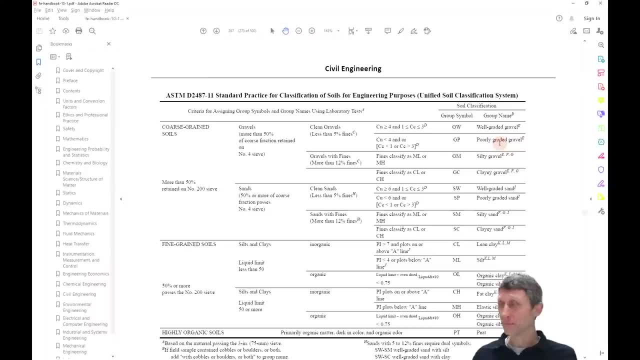 the same size, or marbles, They're all fitting together. They're all kind of perfectly the same size, Right That's? that's a uniformity coefficient Of like one right, if they're all exactly the same size. So what we're? 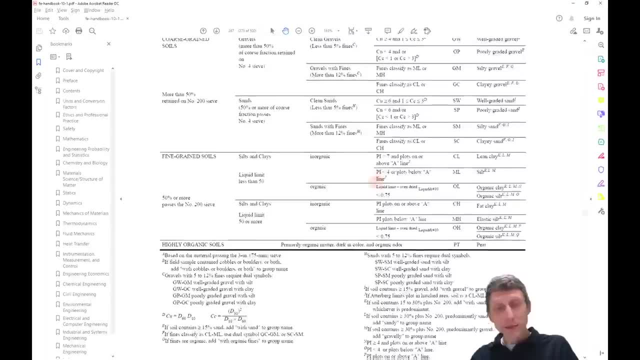 going to do here is we're going to say: well, what do we look? how do we find that? And this is cool too, because I think this is going to show up on the test, I think somewhere- CU, CC they're. 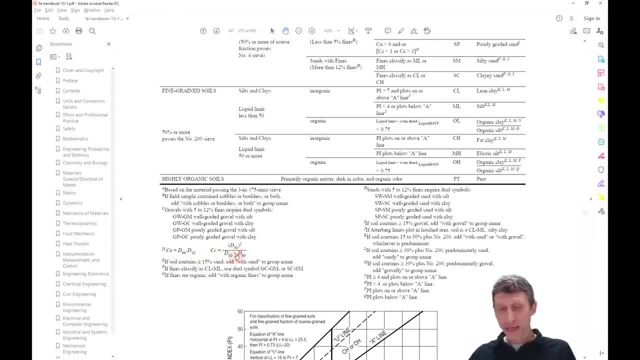 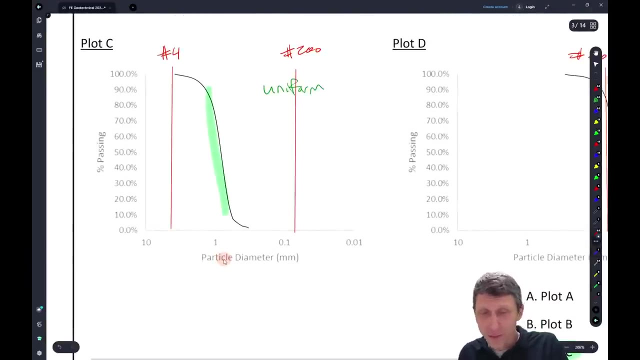 going to show up on the test and they're just basic formulas. This is D60 over D10.. And that's uniformity coefficient and the coefficient curvatures are D30 squared over D10.. Over D60.. So if we look at this plot here, what we can do is we can actually come back and we can. 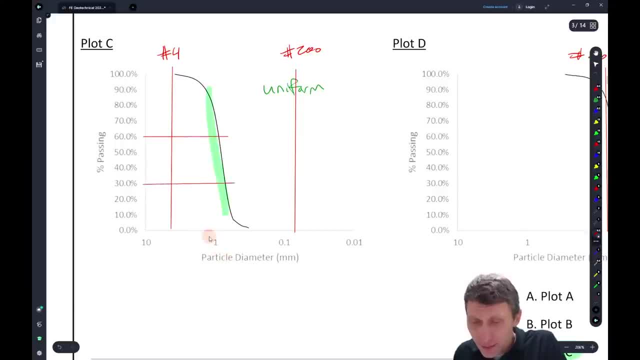 say, well, D60, what's that? D30, what's that Right? And lastly, D10, what's that Right? So we can actually go and calculate these values Right. So if we look at these values right, our D60 is. 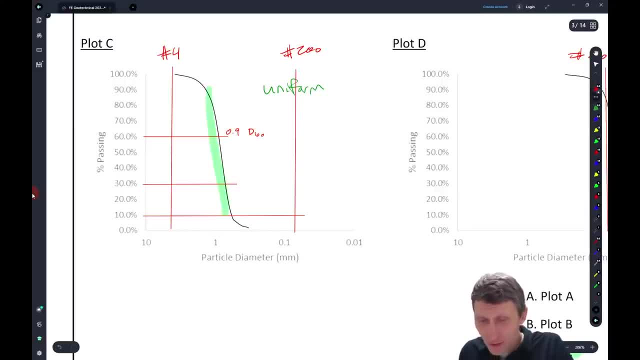 right about maybe zero point nine. That's our D60.. Our D30. This is like the kind of particle size at 30 percent Right, Our D30 is going to be: oh man, where is this? This is one, two, three, four, five, six, seven. maybe zero point seven, if I'm. 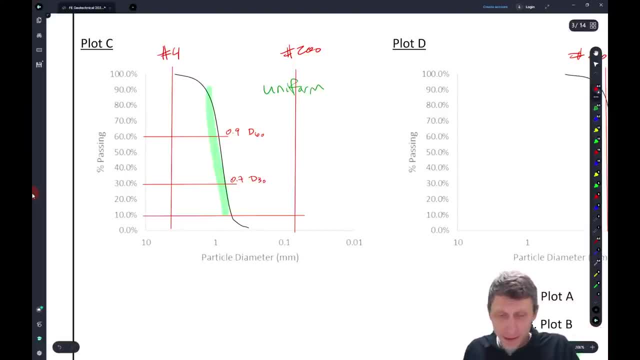 getting that right. That's our D30.. And then where's this? This is: maybe am I looking at this right? Let me just double check my numbers here, Make sure I'm not way off. But our D10,. this is going to be like: 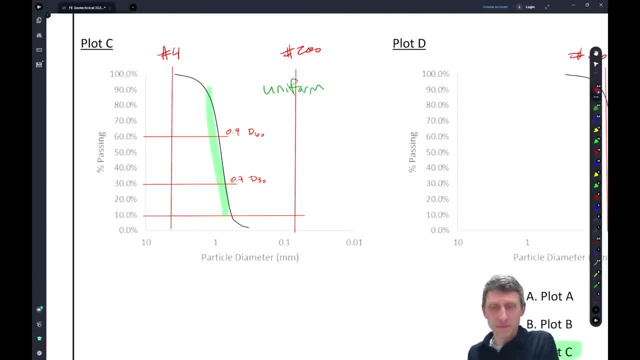 Up point O's. I'm messing something up here. Oh sorry, I'm counting wrong. So our D10 is going to be down at this point here. And what do we get? We get like one, two, three, four, So I'm sorry. 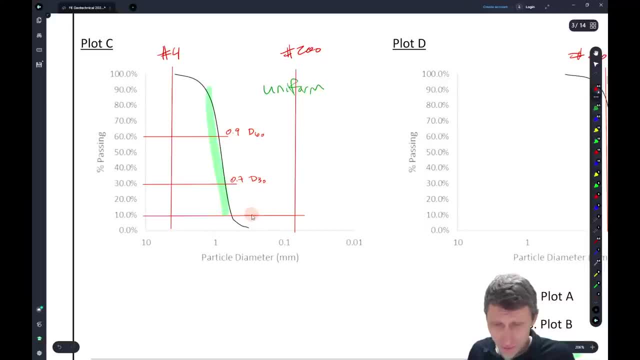 So this is point one, This is point two, This is point three, This is point four, This is point four, This is point five, This is point six, This is point seven, This is point eight. This is point three, point four, point five, point six. Maybe that's point six. OK, so sorry, So zero. point six. 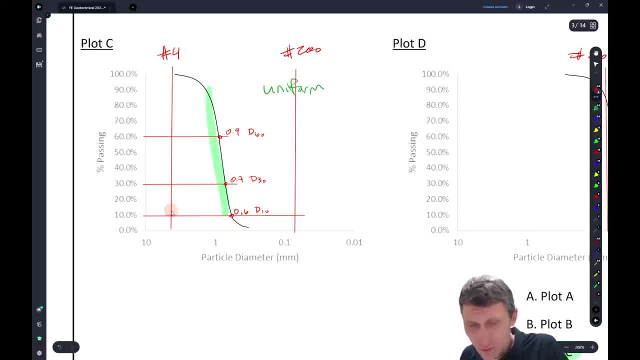 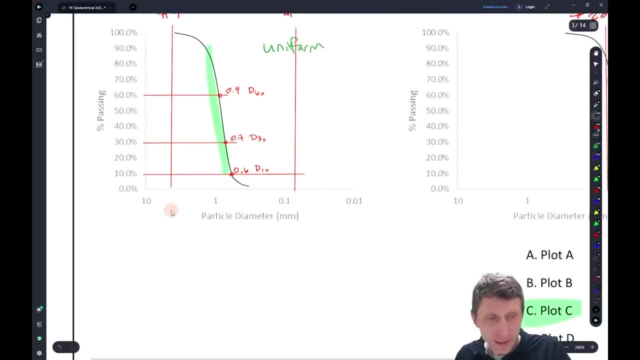 That's going to be like our D10.. Right, So these are the those, those points where we can go and now we can calculate. we can say we can go and we can actually calculate some of these values, so we can calculate the CC. which was what CC? If we come back to our our table here for a second, what we 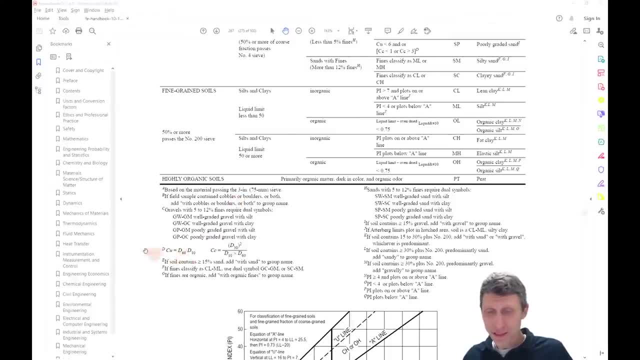 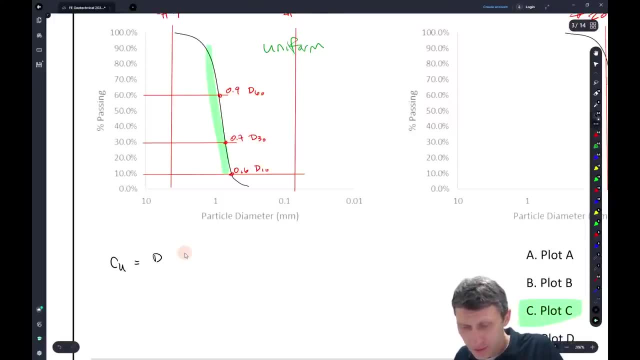 see is that CC is D60 over DC 10 or, I'm sorry, CU is D60 over 10.. Right, So see, let me start with. CU is D60 over D10.. So what's that? It's like zero point nine over zero point six. So that's about one point five. OK, that makes. 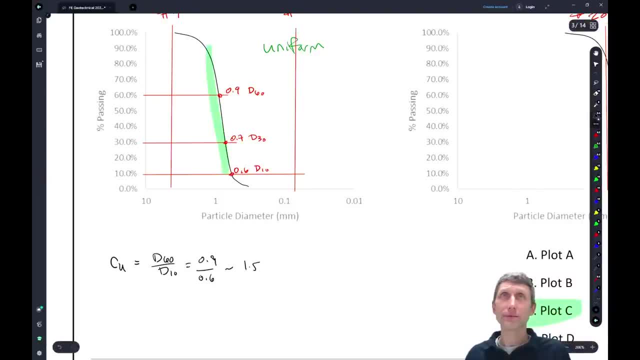 sense I think it does. So that's about one point five, And if we keep going here, we can say like CC, which was this: This is equal to D D30 squared over D10 times D60.. So these are, these are things that I think are probably going to show. 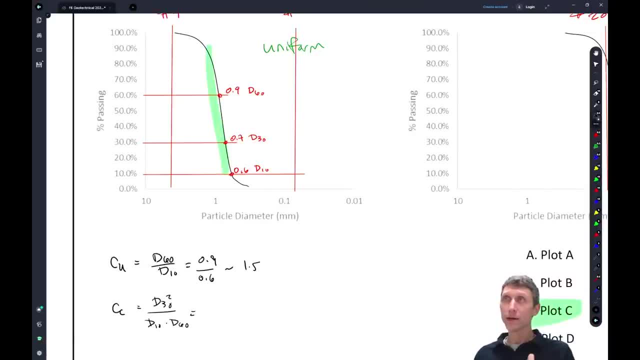 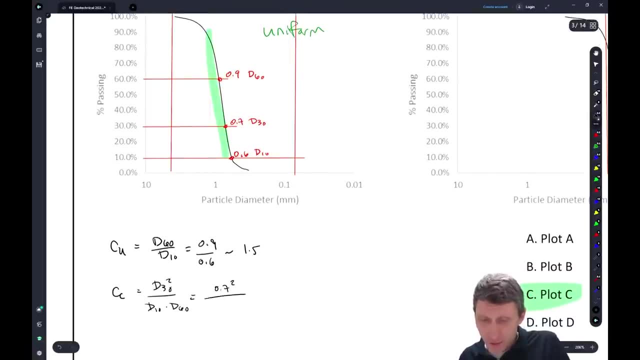 up somewhere, OK, And can you? can you solve for them? OK, so let's take a look. I mean, let's look at this. D30 is going to be about zero point seven squared over zero point six times zero point nine. 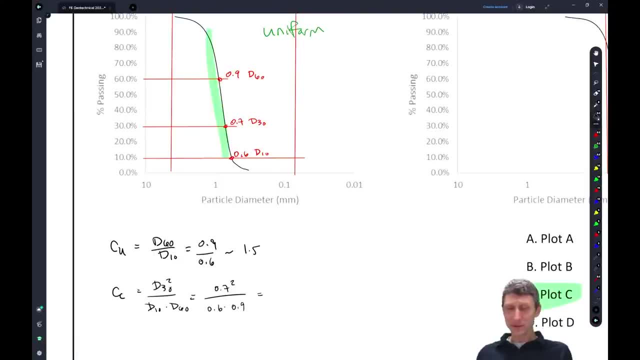 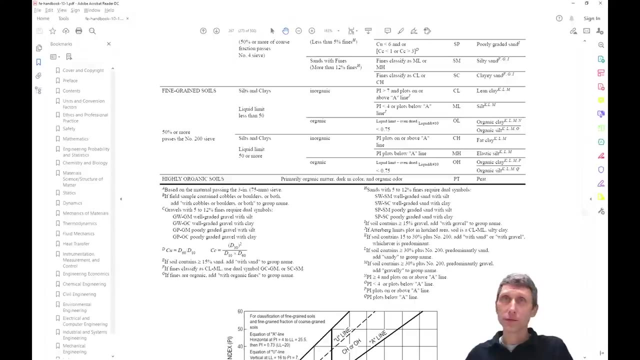 And if we do that out, let's see point seven squared over point six over point nine. I get about zero point nine, OK. so again that puts us firmly in that USCS poorly graded sand uniform sand range Right. So that puts us firmly kind of in this CU less than four. 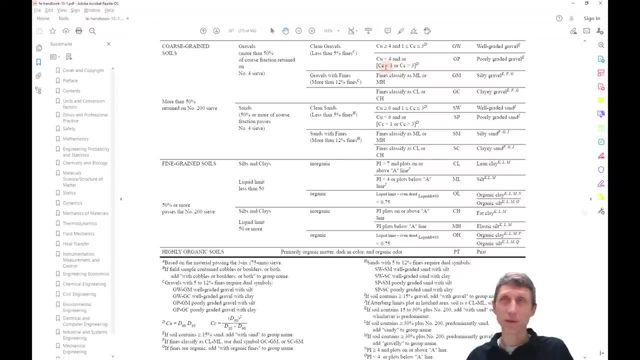 It's one point five. That's a pretty uniform soil. CC less than one is also again an indicator of pretty uniform soil. poorly graded sand- Or I'm up here with gravel, I'm sorry, I should probably be down here with sand. Less than six, less than one. 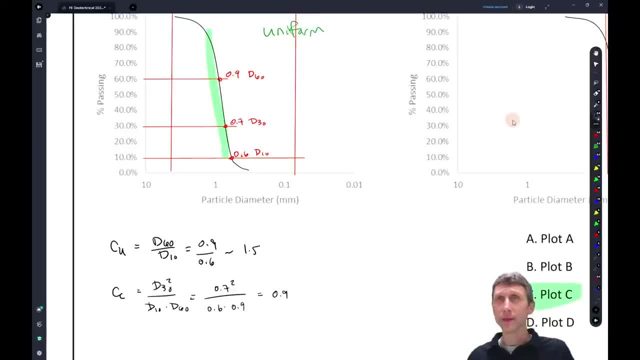 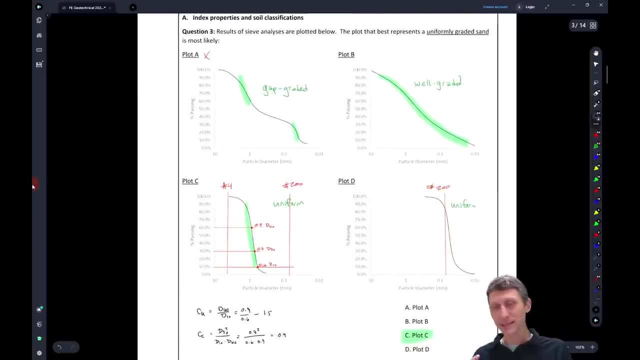 Same same type of thing, though Poorly graded, And and that kind of gets us in those ranges. So again, these uniformity coefficients, coefficient curvature, I think they will be there and potentially show up on the test. So good things to know. But I like this problem because it kind of gets in there a few of the different pieces. 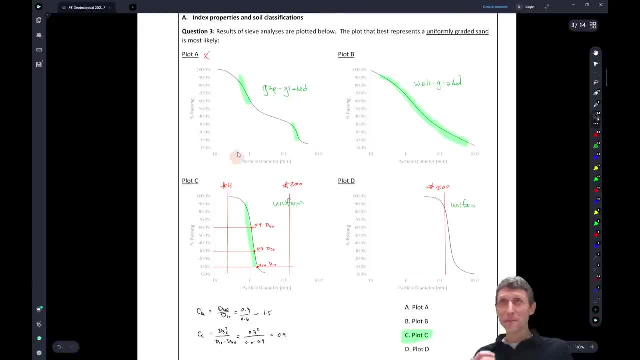 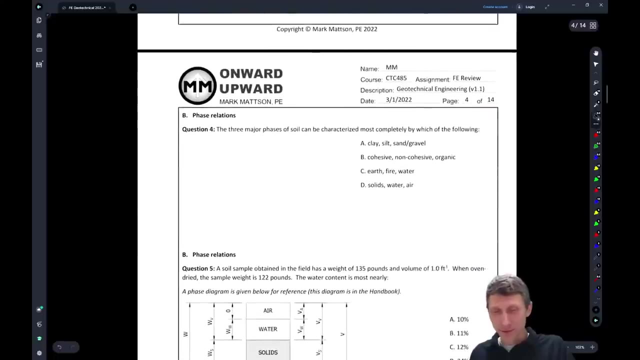 Right, It talks about those, those, the sieves, It talks about the how to interpret these, these lots, a little bit, And I put this one together to try to get those different sizes in. All right, I mean, man, we're fine today We have three questions and we're going OK. 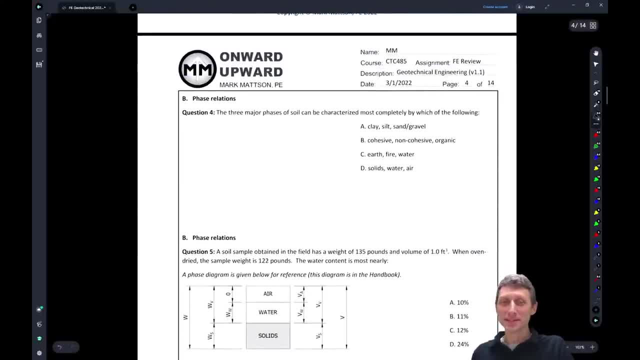 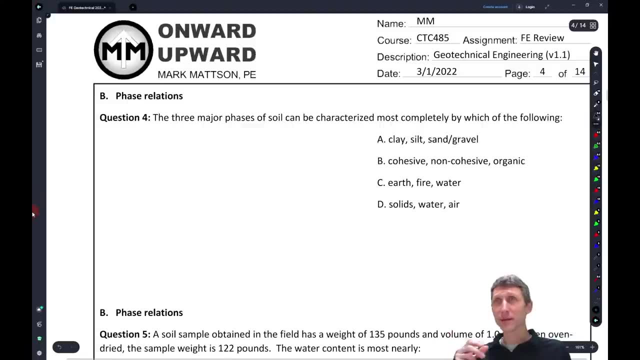 So let's keep going. Three major phases of soil: OK, so three major phases of soil. This is supposed to hopefully not be that difficult, but this is just a concept question, Right? I mean, you're going to get some concept questions. Hopefully these are the questions you can answer in 30 seconds. 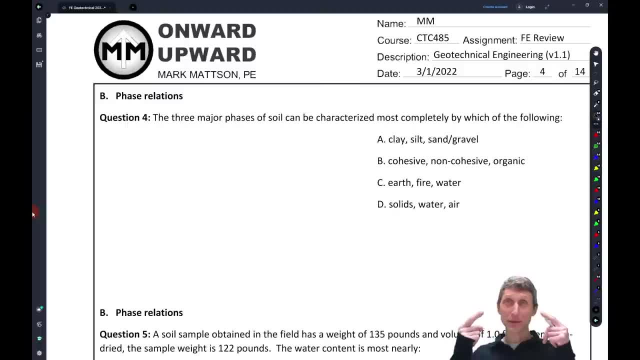 I put this one together just because I wanted to get you thinking about some different things. right, clay, silt, sand, gravel, these are different. you know, fine versus granular materials. right, fines versus granular materials. that's not a phase of a material. what's a phase of of water? well, you, 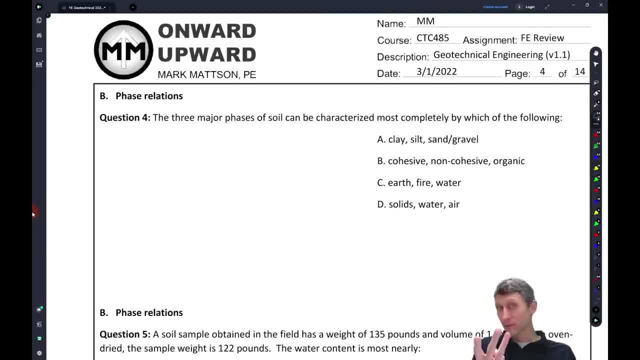 have ice liquid and steam, right, or in other words, a solid, uh liquid and gas, and that's the same thing that we have with soil, right with soil. we have solids, water and air, right, so earth, fire, water. i mean, that was just for fun, you know. but uh, what else? cohesive, non-cohesive, organic, these? 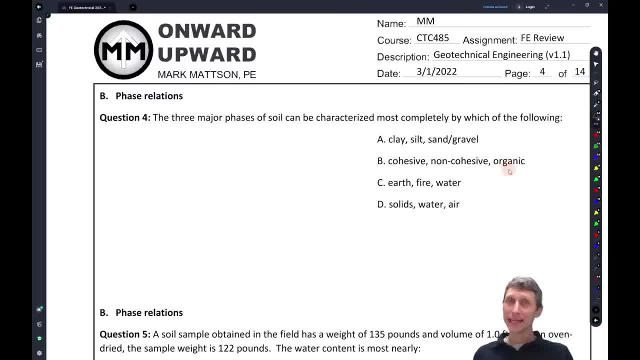 are just categories of soils, but they're not phases. phases kind of get into, uh, the kind of the components, uh, but this is solids, water and air, and this is where we get into phase diagrams. so now we're into phase relations, part b, and when we start taking a look at this, this actually 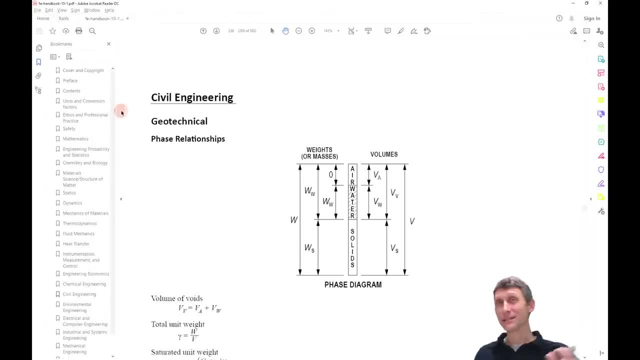 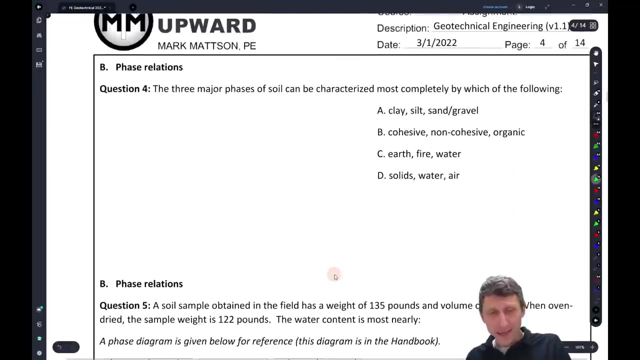 starts us off where, honestly, the geotech reference starts. so there's a phase diagram here. I made another one that I stuck in, uh, the problem sets, but I just took this, this thing. you know, this diagram. I made one kind of similar for the next few problems. so, yeah, the answer here. 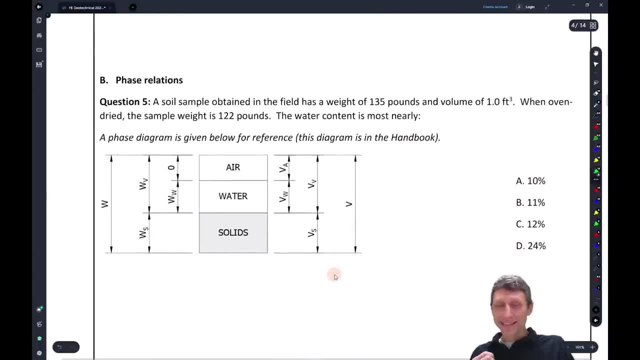 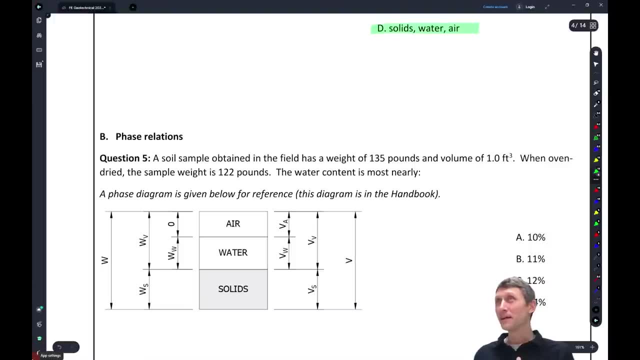 is solids, water and air. but this also comes to light when you see kind of this question, this next question, I mean this next question. hopefully it's just a warm-up question. it's not really, uh, that super, super challenging yet, but the idea here is we have different phases, right, we have. 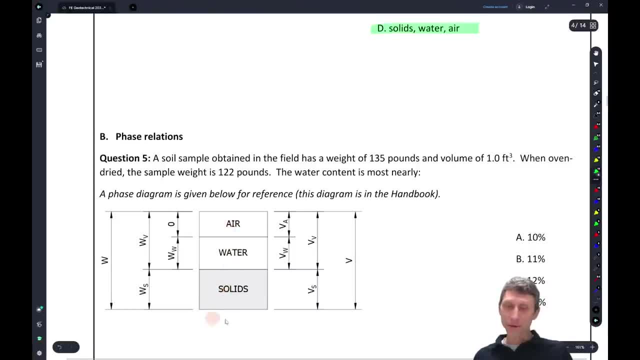 these, these solids, the water, the air, they all make up a composite solid right, a composite soil. I should say, uh, that you have to understand the different components with, and probably one of the most basic tests that you did in your soils lab is: you took a piece a can of soil, you stuck, you know, you weighed it, you know. 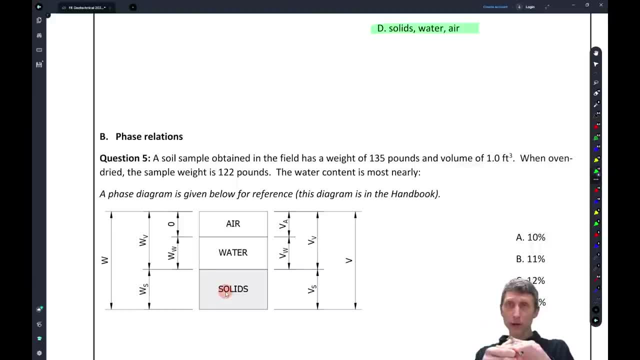 you found either the mass or the weight of it before with water in it, and then you stuck it in an oven and then you waited again and a day later. why'd you do that? because you wanted to evaporate all the water. so if you evaporate all the water, you're going to have a lot of water. 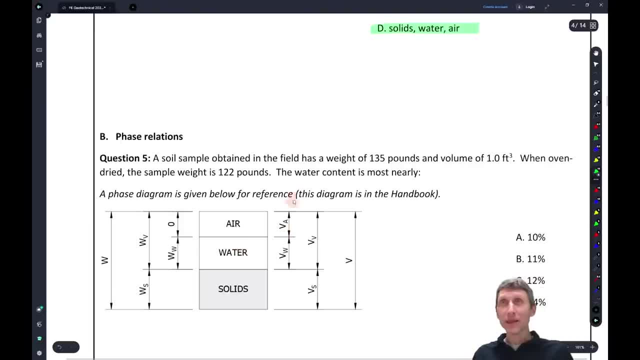 so if you evaporate all the water, you can figure out how much water was in it and you can figure out the water content, right. so this is kind of one of those basic things, just kind of get you warming up. it's to talk a little bit about the different phases of soil, right, but this is where we get. 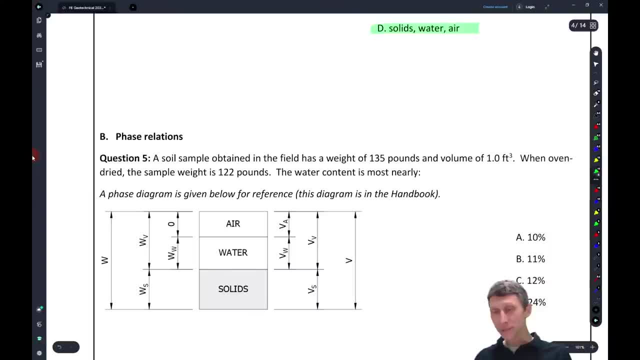 into phase relations. so this question starts off with the soil sample obtained in the fields: the weight of 135 pounds, right? so what is that? that's 135 pounds and, honestly, if you're doing one of these problems, I would suggest sketching a little diagram like this: so you sketch a little diagram. 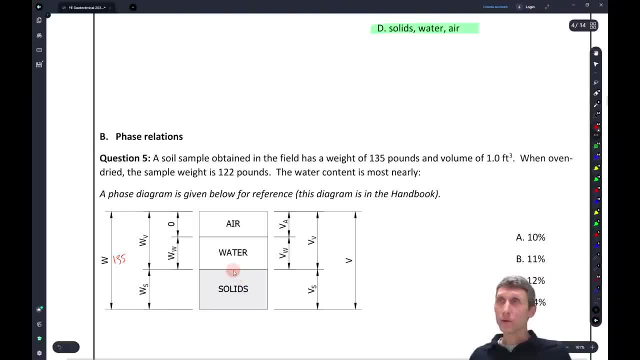 on your soil and then you're going to have a little diagram like this. so you sketch a little diagram on your little notepad that they give you and you you start to just fill in the pieces that you have right and this is, this is one of those things. so we know we have 135 pounds of field weight. that. 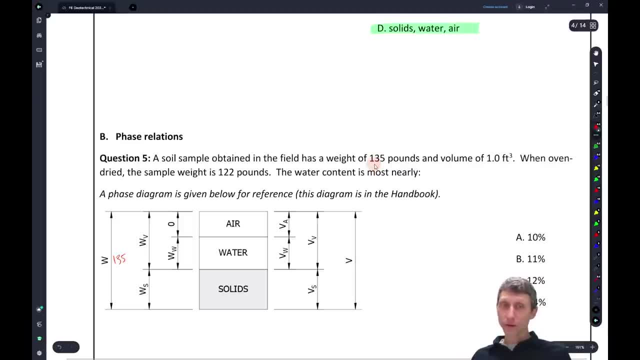 includes both water and soil, right, so it's the volume of one cubic foot, right, so 135 pounds one cubic foot. and what's next? so what's next is we oven dry the sample and we get a weight of 122 pounds. what's left if we? when we oven dry the sample, it pushes all the moisture out it. 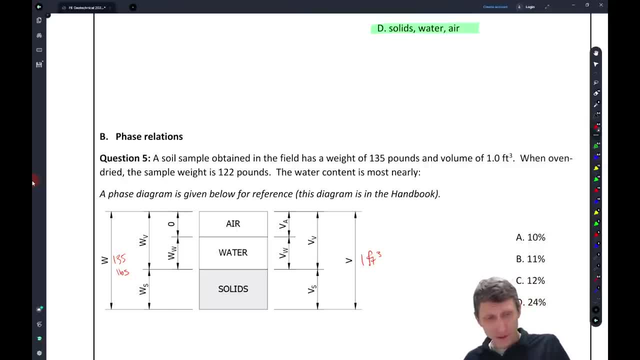 evaporates it all and what word dries it all out. what we get is 122 pounds of solid. so what does that mean? that means if you're doing this, you can start to figure out the volume or the weight of the voids here, which is the water and the air, the way the voids. it's going to be 135 minus. 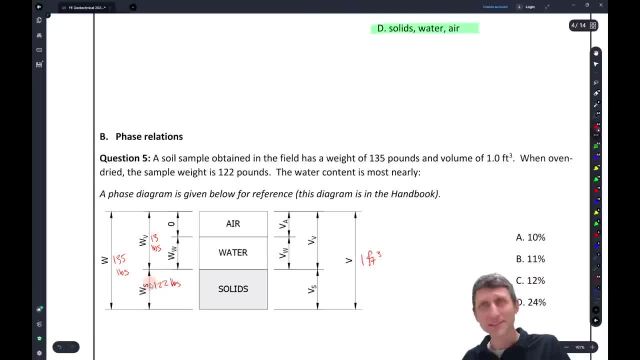 122. if i can do that in my head- and still i know it's late, but if i can do that in my head- 113 plus 122, i think, is gives me 135, right, what does that mean? that means that we have the water volume, or 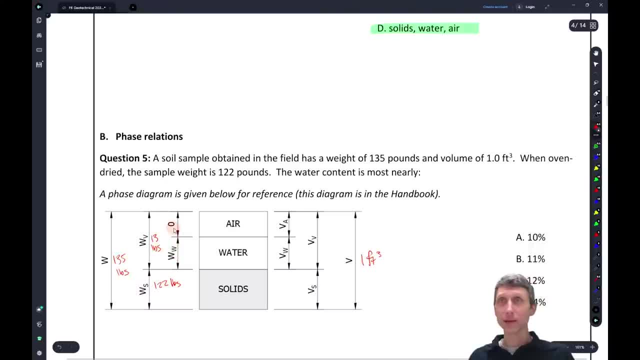 the water weight here because air weighs nothing. okay, in in the grand scheme of what we're doing here, um, we're saying air, uh, doesn't weigh anything and that's okay, so air does, air is not going to weigh anything. um, that means this whole, uh, this whole void weight is going to be our water weight. 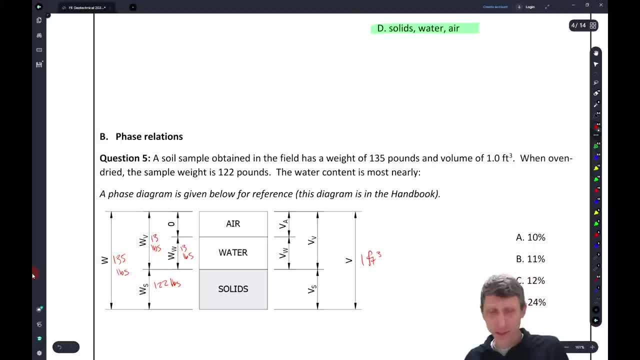 right, 13 pounds over here, and then the. the question really is just asking for what's the water content? so again, this question isn't meant to hopefully stump you, hopefully this is an easy one. but the question is: do we divide 13 into 135 or 13 into 122? and if you don't remember, 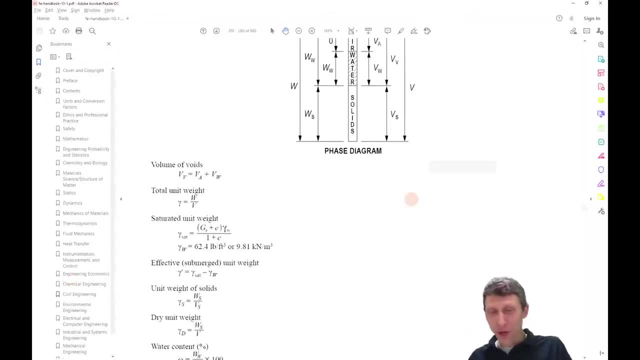 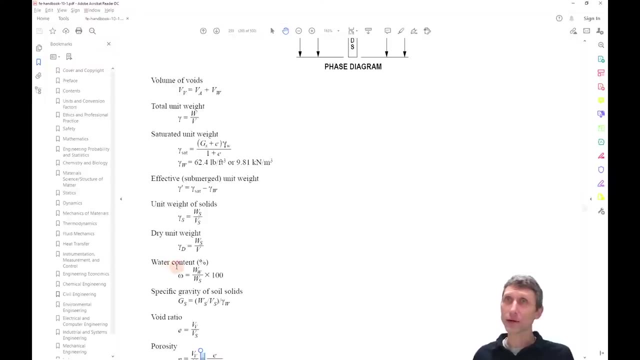 uh, that's okay. these, these relationships show up right in: uh in the in the reference handbook. so the water content: right. so if we look at the water content over here, the water content is going to be the weight of the water divided by the weight of the solid times: 100. right, the weight of water. 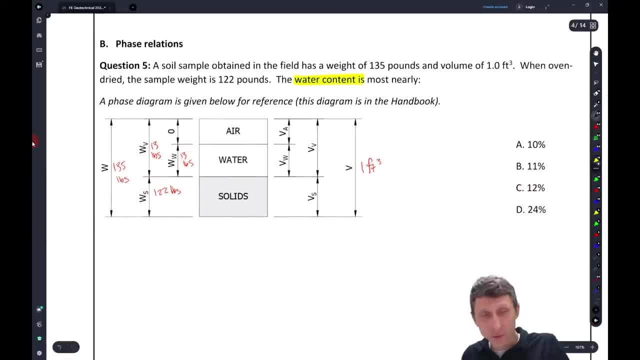 by the way, is solid times 100. so what does that mean? that means this: um, water content is the weight of the water divided by the weight of the solid times 100. so we get the weight of the water right. what's the weight of the water? the weight of the water is 13 pounds. 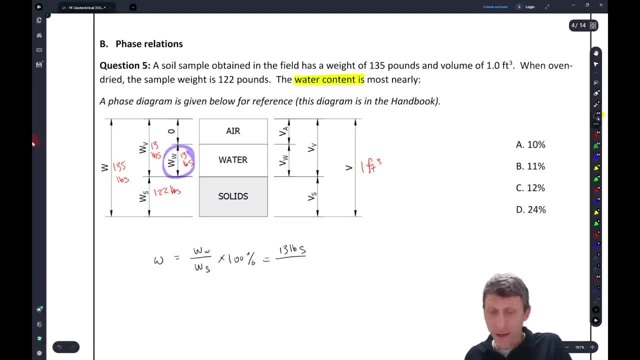 uh, divided by the weight of the solids, which is 122 pounds. uh, in a perfect world, all our units are going to work out wonderfully and never have any problems. okay, so the good news is we, we worked our units out here. 13 divided by 122, oh, is about um well times 100. 13 divided by 122 times 100. i. 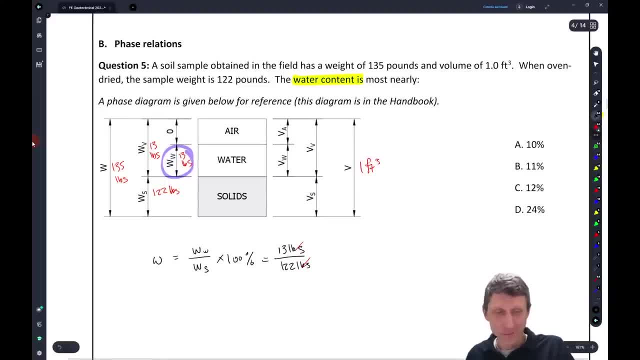 got about 10.6. okay, so 10.65. so, uh, maybe i could have written this a little bit better. this is close enough to 11 that i'm going to use 11 here, so i probably could have made my number a little bit better. giving you decimals: 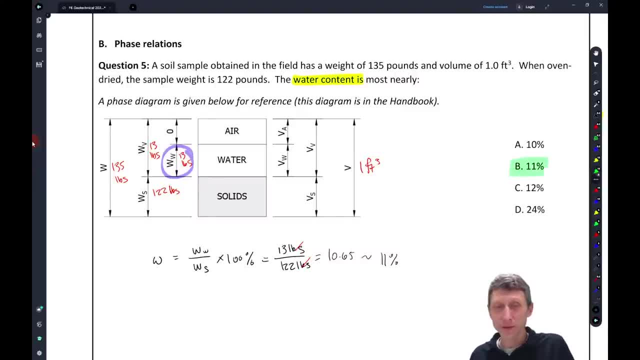 and the answers, but it still rounds to 11. i mean, if you, if you did it, if you did the wrong way, right, if you did the wrong way- 13 over 135, you'd get closer to 10, right? but that way, uh, we said is: 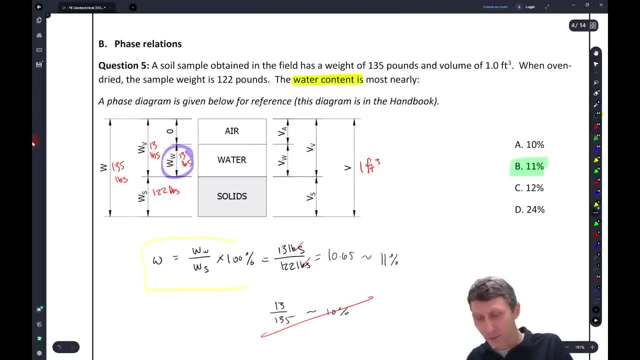 wrong, because what you really want to do is you want to go get these formulas right. you want to get the the correct formulas and you don't want to get the wrong formulas and you don't want to use them. okay, so, water content, one of those real basic ones. um, hopefully, uh, if you get something as 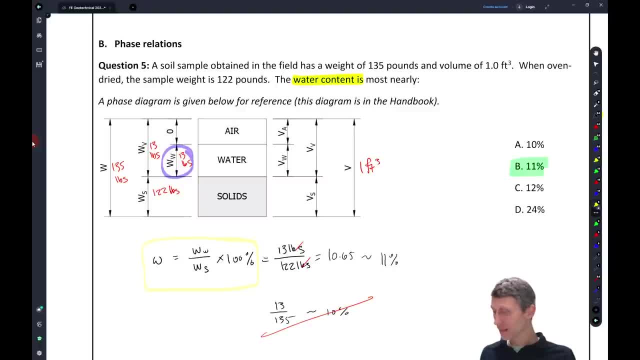 easy as this. it's going to work, but it will get a little bit more complicated as we go through some of these phase relation problems, because some of the questions and some of the equations actually get a little bit more, uh, complicated, right, and sometimes you need to know some conversions. 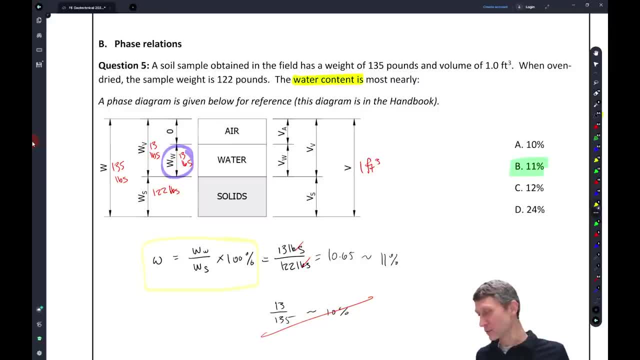 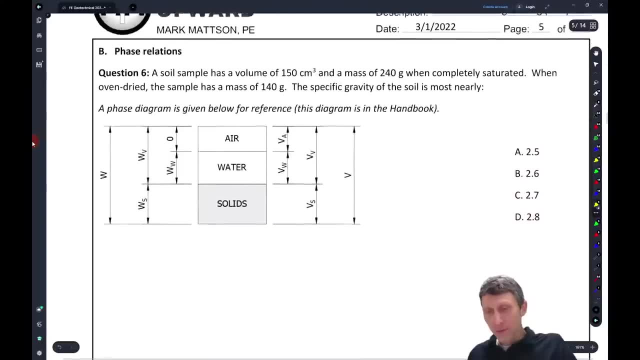 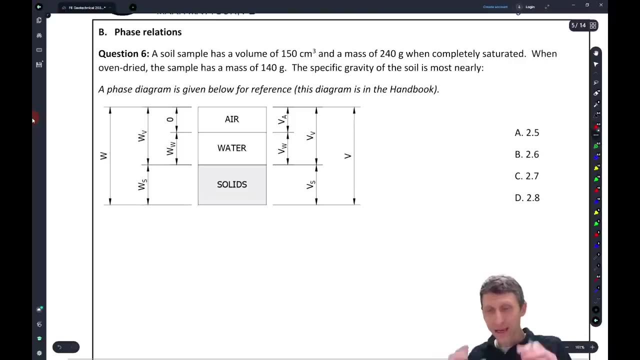 and they're not quite as straightforward as this one. uh was so let's go to. let's go to the next one. so where do we? what do we have here? we have a soil sample with a volume of 150 cubic centimeters. so, again, what i like to do is is i have my phase diagram here. i just again, i copied this in: 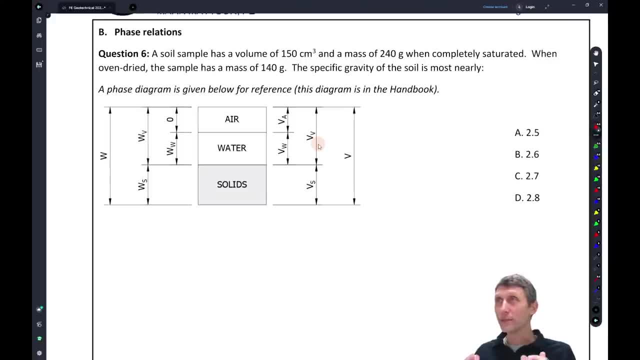 i made my own. but this is one of those things where i i made my own here and i'm gonna go in and sort of plug these in, so it's just like you have free body diagrams and statics and structures. you know, what we're gonna do here is we're gonna make this phase diagram anytime we get a problem. 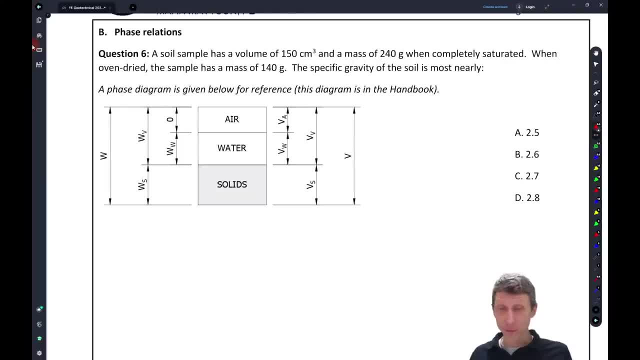 like this because it's going to help you organize what you have, what you don't have, what you need to have and what do we have. we have a sample. it's 150 cubic centimeters- okay, 150 cubic centimeters and a mass of 240 grams. 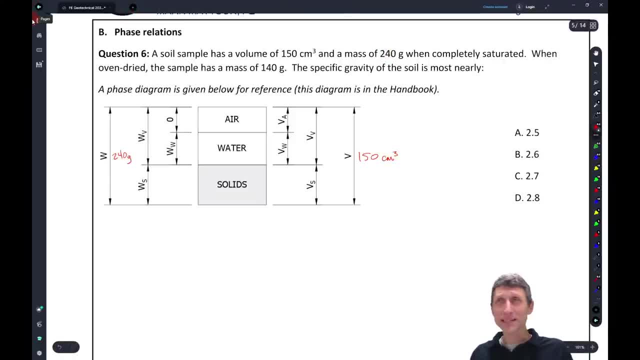 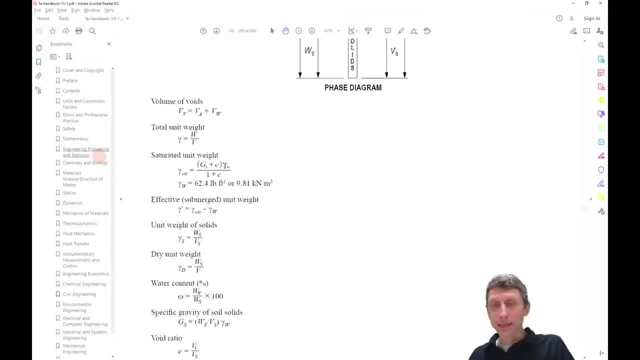 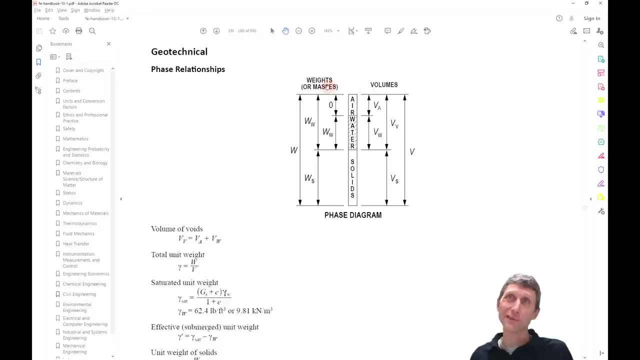 240 grams. and you might be saying: but wait, this says w it does. and that's okay. you're only given one one. you know um phase diagram. this says weights or masses. so if it's a mass, you just substitute w for m. okay, not a big deal, uh, just. 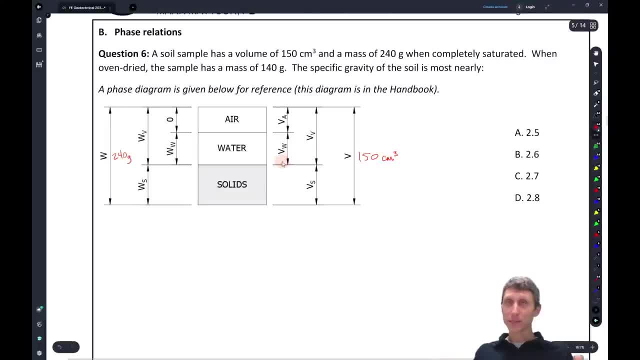 something you have to deal with. and what a weight or a force equals a mass times acceleration. so what's the difference? um, weight or mass, uh times gravity is going to give us our weight. so here, uh, you know, we, especially when we get to metric, um, sometimes we'll, we'll use masses, okay, so what? 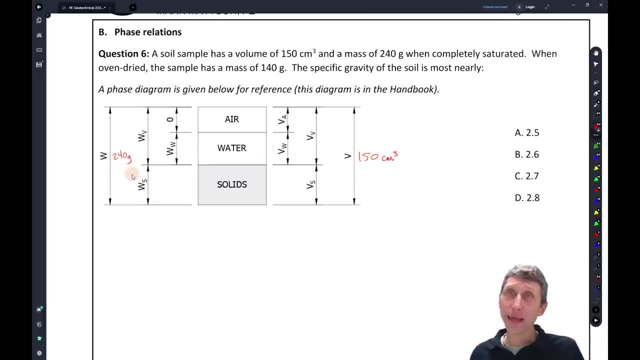 does that mean that means what we're going to do here is we're going to come in and we are going to go, uh, next, we're going to keep reading the problem. so when other people are going to be thinking, well, how is this plant is completely saturated? what does that mean about the volume of the air? 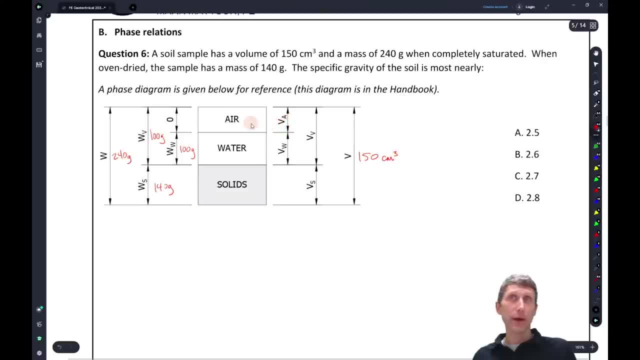 completely saturated means there was no air, right? Okay, so it was full of water and no air, So that means that that's going to tell us something here, too, right? What we're trying to find, though, is the specific gravity, And so what we're going to do is we're going. 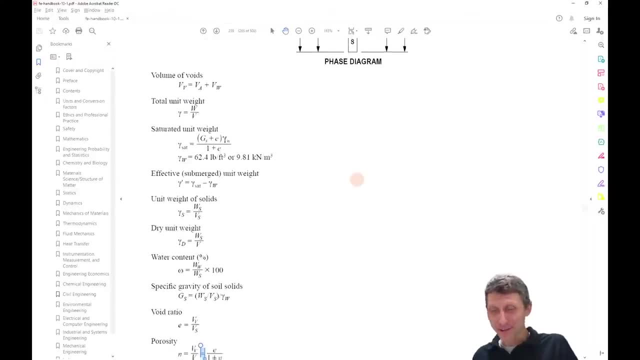 to come back and we're going to scroll down and look for specific gravity, right. So hopefully there's just something here that we can plug in, plug and chug and solve right. But so the GS is specific. gravity here is going to be the weight of the solids divided by the 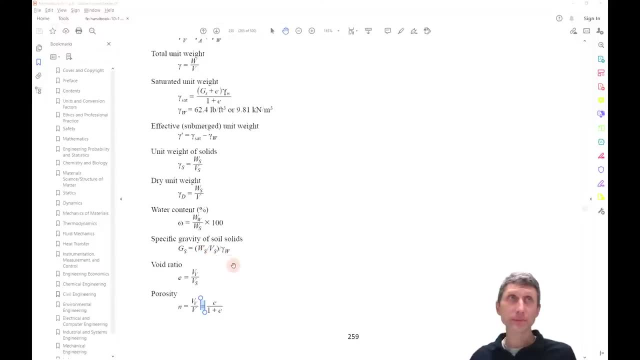 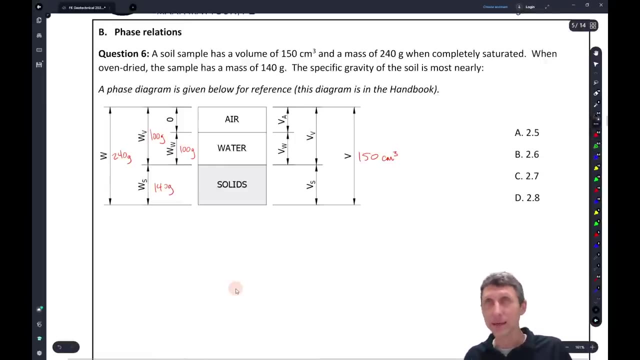 volume of the solids divided by gamma water. And I specifically chose this one because I don't know about you, but for me, sometimes I have to think about my units and my conversions because I don't always use and think in terms of 9.81 meters per second squared. I don't 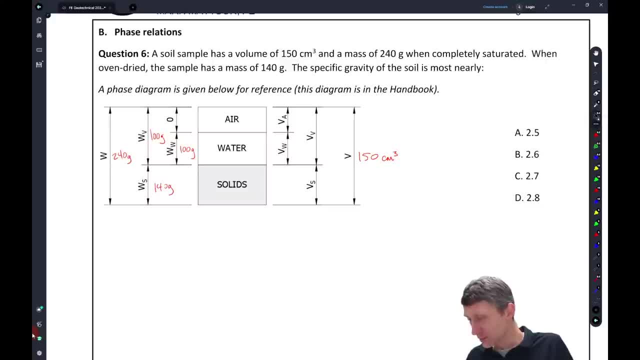 always think in terms of milliliters and centimeters cubed and all those things, And I think it's probably good to review that a little bit. So the specific gravity equation gives us the weight of the solids divided by gamma water, And I specifically chose this one because 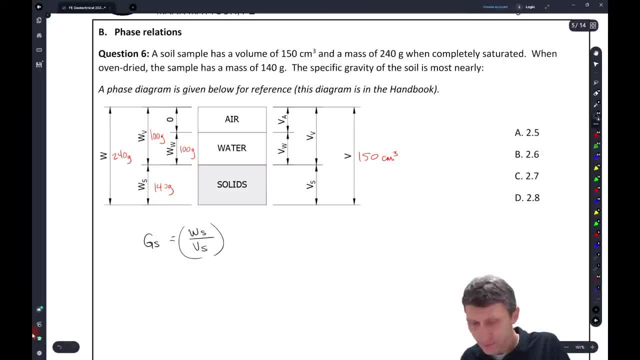 I don't always need to repeat this, Any sounds good. So this is where we go. OK, I think. for every unit, I think the weight of the solids divided by the volume of the solids, All of that's divided by gamma w. So the question is now: 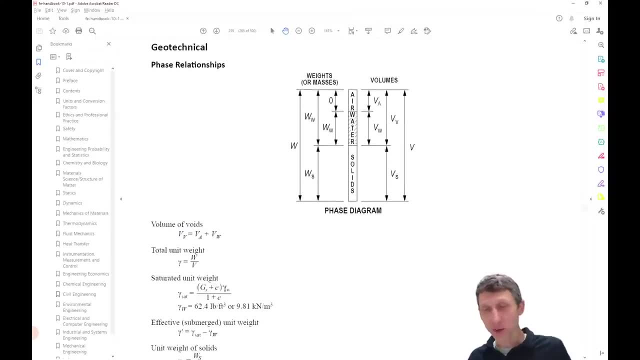 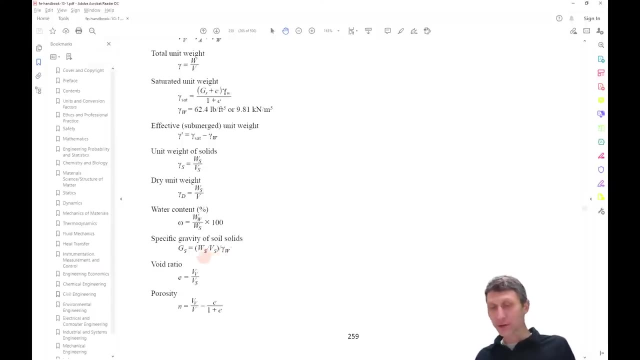 this is. you know, we're given this phase diagram over here and it says, OK, weights are masses, but what we have is a mass. So do we convert everything that wait and then go there, or do we convert all of this to masses? and we have to be consistent, OK, So, 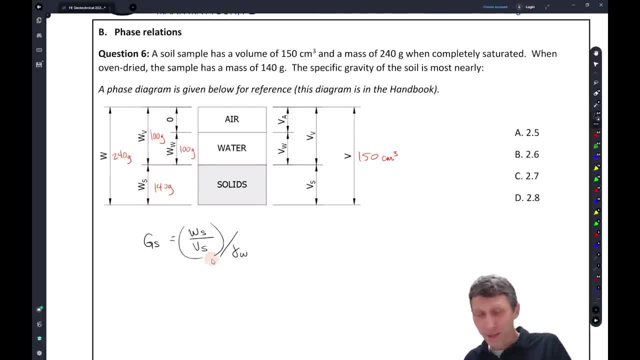 the way that I think of this is: I think of ein había, no like this. So I think of this: is this equivalent here? it's gonna be what? well, what we said: a force equals a mass times an acceleration. so a weight equals a mass times gravity, right does? 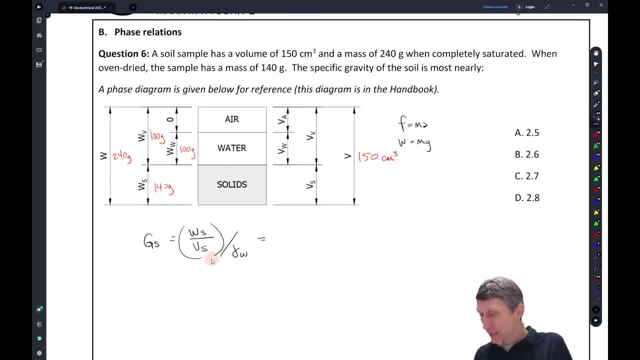 that make sense in. similarly, if we're thinking about the unit weight here, right, the unit weight we're gonna have kind of like the density is equal to Rho G, okay, or the- I'm sorry, the unit weight is gonna equal the density times Rho G. so what you see here all of a sudden is it is we get the mass of the. 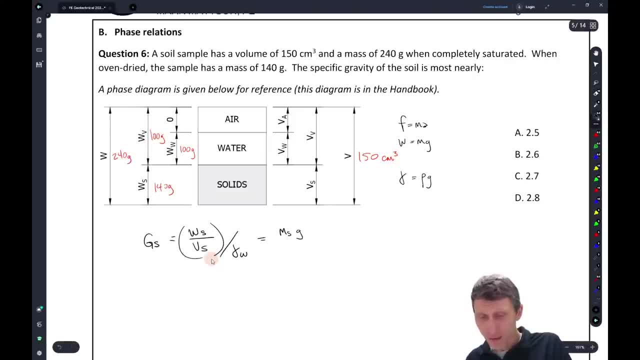 solids up. sorry, I wrote the wrong thing: mass of the solids times gravity over the volume of the solids. right. divide all that by a row of water times, G. okay, and the cool thing is here the G's go away and we just get an equation where we get the mass over this density rather than unit weight. what's the density of? 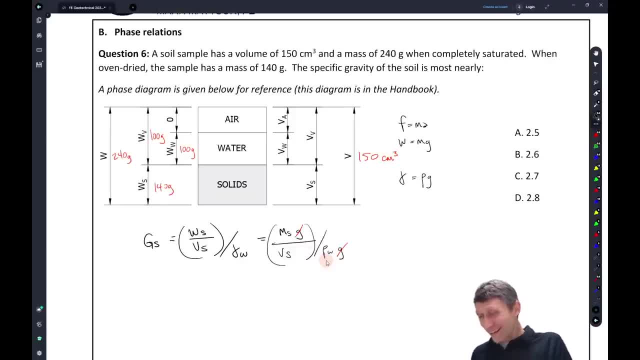 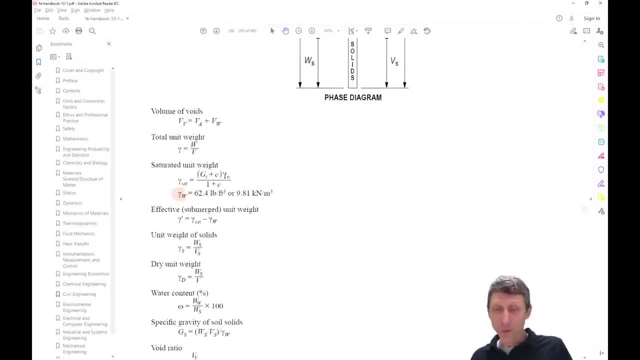 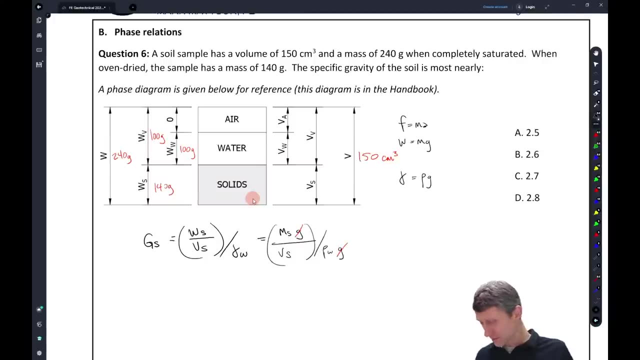 water. okay, that's one of those things we're. hopefully you don't have to look it up, okay, so hopefully you don't have to look it up. if you do need to look it up, um, the good news is we're told that the unit weight here of water is 9.81. but also, hopefully, one of those, one of those, one of those. 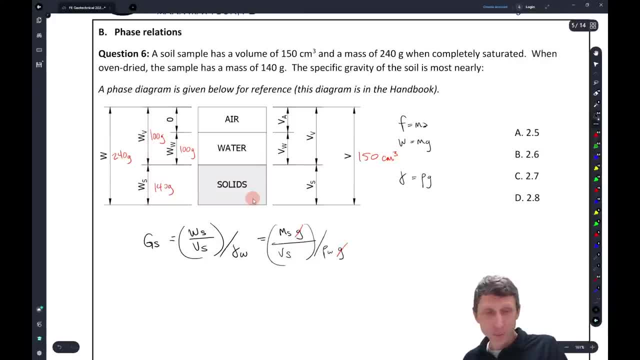 numbers that you know is is what the Rho of water, hopefully you know is one gram per, or what? per milliliter or one gram per cubic centimeter. okay, so if you know that that's gonna help you out a little bit, you as well. right, and what this is gonna tell us now is is a couple things we 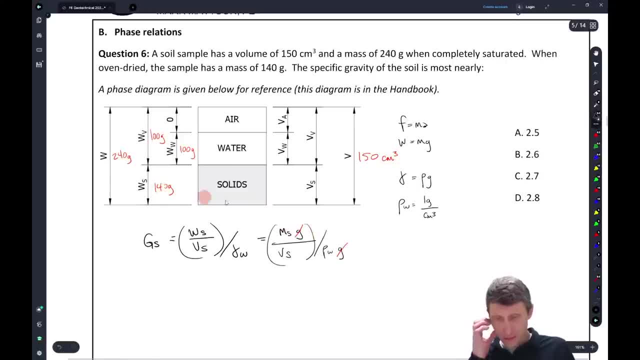 still have the mass of solids. so we know, we know the mass of the solids, but we don't know the volume of the solids. yeah, so how do we get that? this is, this is where we do know the volume or the weight of the water. we can find the 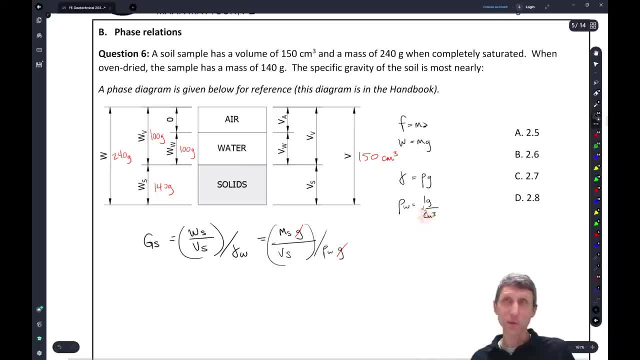 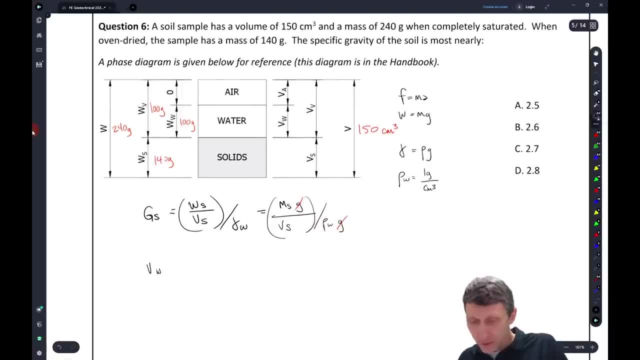 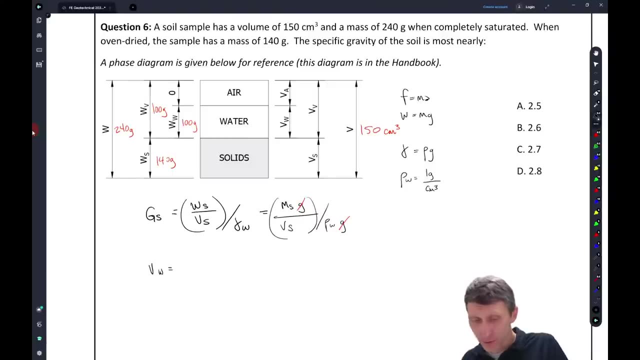 volume of the water. right, because we know that one gram of water is equal to what one cubic centimeter, right? so if we have one, so we can find the volume of the water equal to what is is equal to essentially mean we have 100 grams of water divided by one gram per cubic centimeter, which. 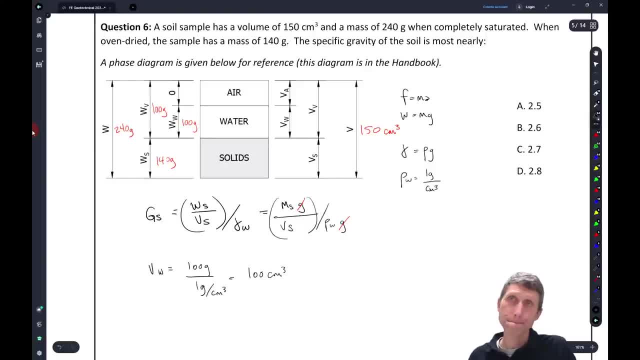 is going to equal a hundred cubic centimeters of water, right? I mean is, does that make any sense? I mean, the numbers here are fairly, fairly simple in terms of: we don't need a calculator to do that, but it hopefully. the units make sense. so what that means is we have a hundred. 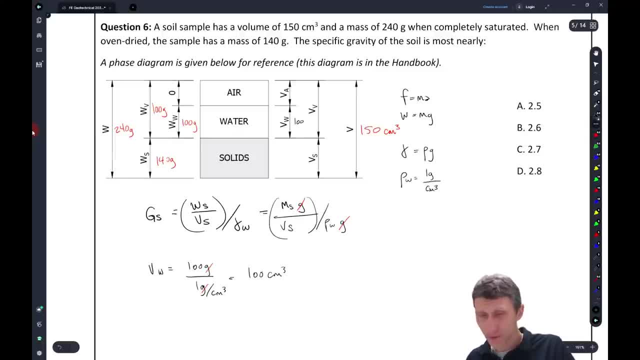 cubic centimeters of water. okay, in that also means that if we, if we plug in and use our phase relationship here, we know that. remember what I said earlier: this is completely saturated, right? so if it's completely saturated, that means the volume of the air is zero, that means the volume the voids is a hundred cubic. 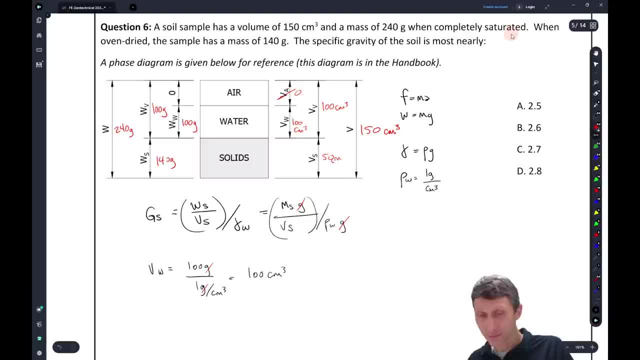 centimeters, which means the volume of our solids is a hundred or fifty cubic centimeters. follow that right. once we found this, this volume of the water, we're now able to kind of work backwards to get the volume of the solids and once we have that, the rest. 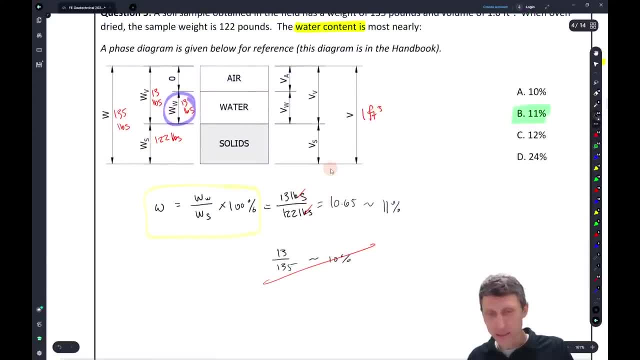 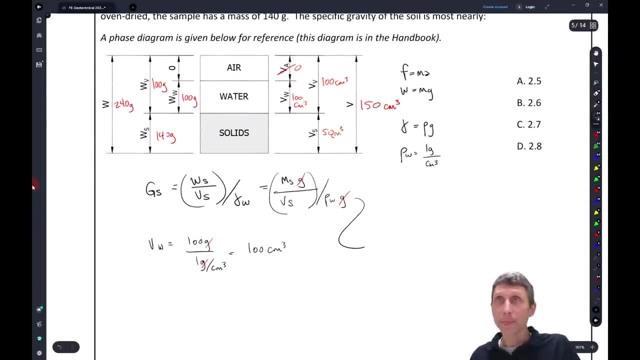 becomes kind of plug-and-chug here. so I skipped down a little bit here. but let's, let's go through and finish our sorry, wrong question. um, let's finish our plug-and-chug here. and what do we get? so if we finish this plug-and-chug, we get. 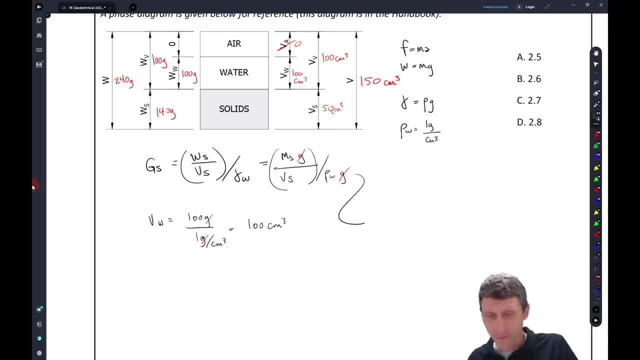 the mass of the solids, or 140 grams, divided by the volume of the solids. and then the mass of the solids, or 140 grams, divided by the volume of the solids, which is 50 cubic centimeters right. and if we divide that by a one, what divided? 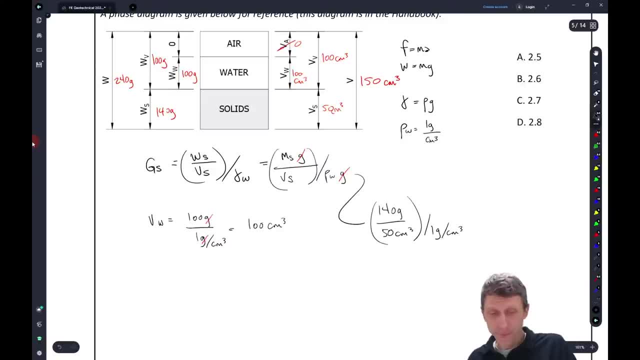 by row of water, grow waters. one gram per cubic centimeter, right. so the cool thing is, what we see here is units are falling out. the radar grams go away, our cubic centimeters go away and when we solve this, we get a value of 140 divided. 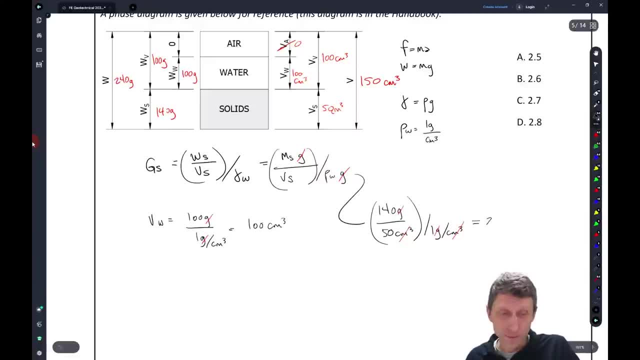 by 50 essentially, And when I plug that in I get like 2.8.. OK, so 2.8 is kind of on the upper end of a specific gravity of a soil, but it should. it should work. OK, to make a little bit of sense. 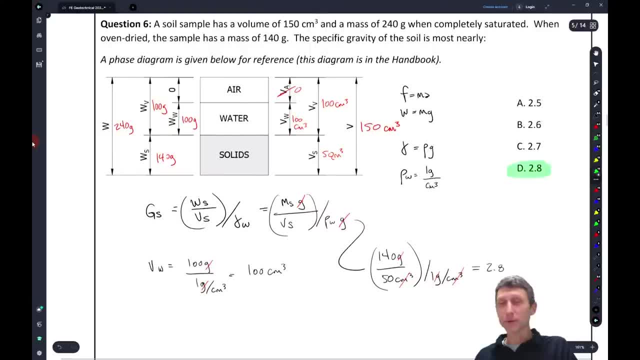 But again, these phase, these phase diagrams are going to be helpful in terms of trying to figure out what you know, what you don't know and what you need to figure out. OK, so hopefully that one makes a little bit of sense And let's go to the next one. 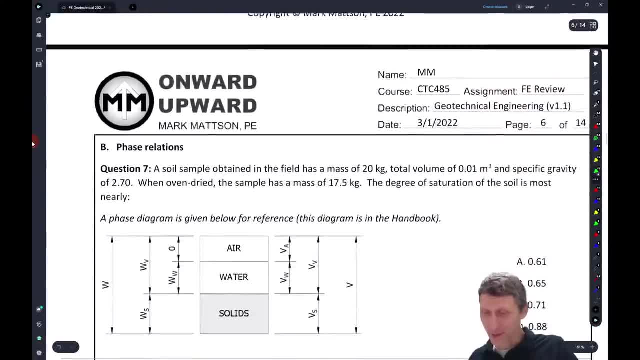 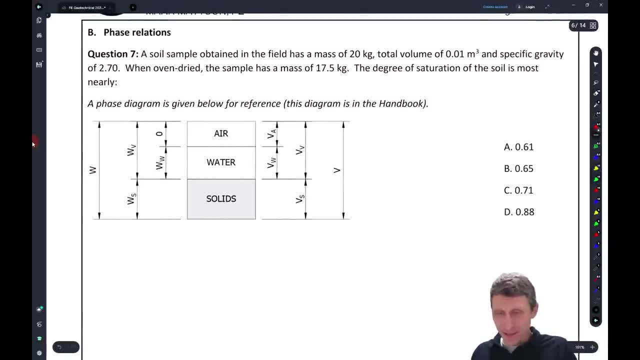 All right, we'll keep going here. Phase, phase relations, Right? So phase relations. Oh man, One day you'll have in-law relations And I love my in-laws. So where are we going to go? So we're going to go and we're going to say: a soil sample obtained in the field has a mass of 20 kilograms. 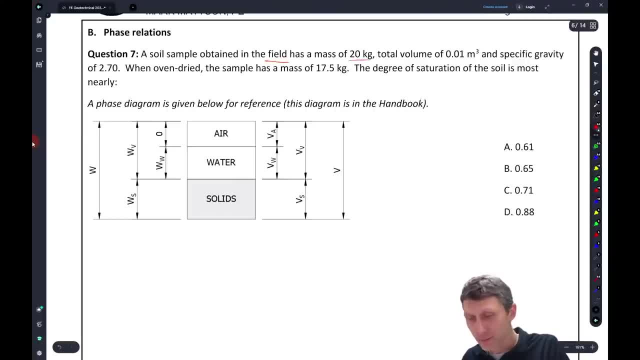 So again, a field, think it has water in it. 20 kilograms. This is going to be our total 20 kilograms. OK, a total volume of. we just shape This, put in a point zero one cubic meter box and we got zero point zero one cubic meters. 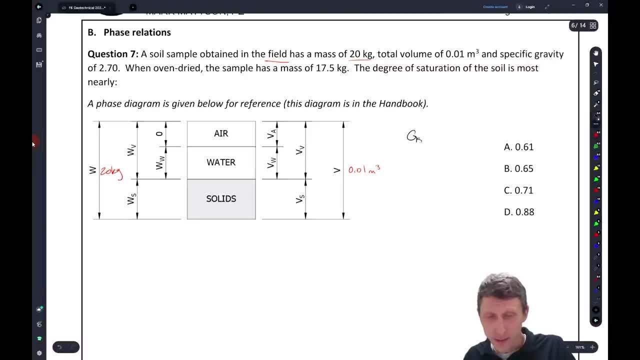 OK, we know that the specific gravity of this soil is equal to two point seven, So we already have that. So when oven dried, the sample has a mass of 17.5 kilograms. So we're given the 17.5.. 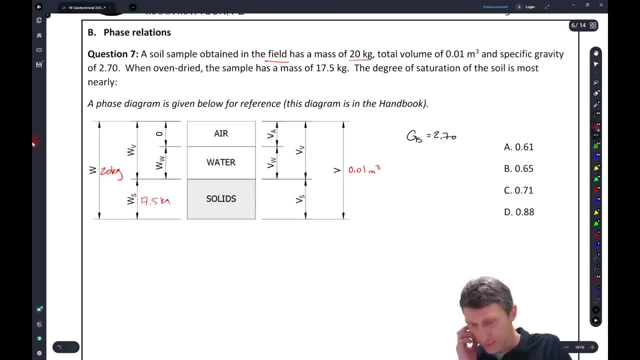 Kilograms over here, So 17.5 kilograms. OK, so if you've been tracking with me Right away, what am I doing? I'm saying, OK, I know 20 minus 17.5 before I even read the rest of the question. 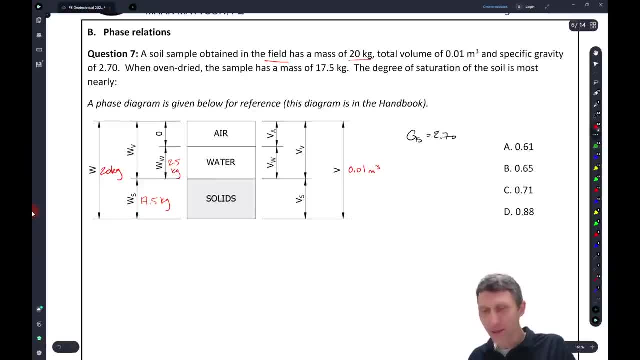 I'm thinking like: what's that way to water? Two point five kilograms, right? So so again just trying to figure out what I know, what I don't know, what I need to know, But the degree of saturations this, this question asked for- degree of saturation of the soil- is most nearly. 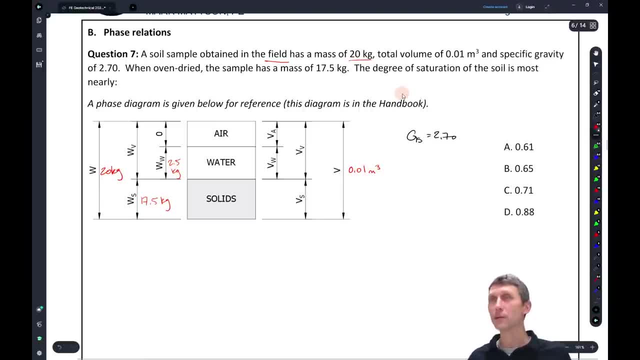 So how do we get the degree of saturation of the soil? So what we get there is is: let's go back and take a look, Look for that equation. So degree of saturation is what we're looking for. We come back here and you know we have some dry unit weights. you know weight of solids. 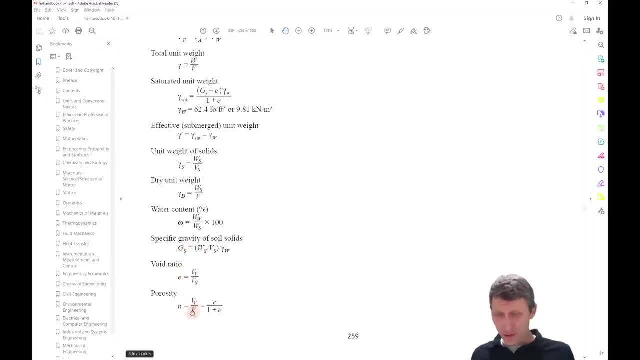 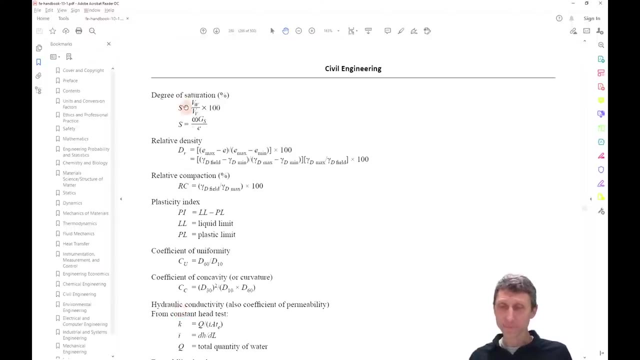 What else do we get? We have. we have a void ratios, porosity and what else. So what else do we have? If we go to the next page, this is where we get. the degree of saturation is either the volume of the water or the volume of the voids. 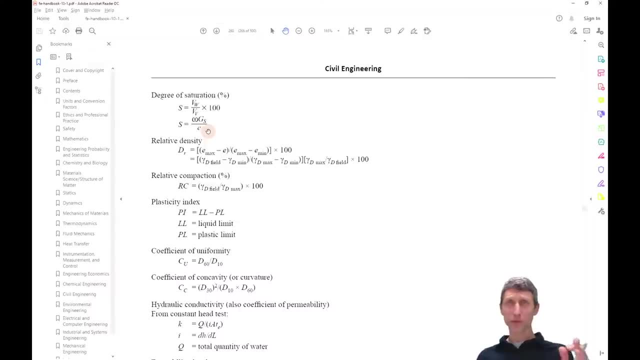 Or the water content times, specific gravity over the void ratio, And there's a lot of things we don't know there. So what I'm going to do is I'm just going to come back and kind of write those equations in and try to see what we have, what we don't have and what we can get here. 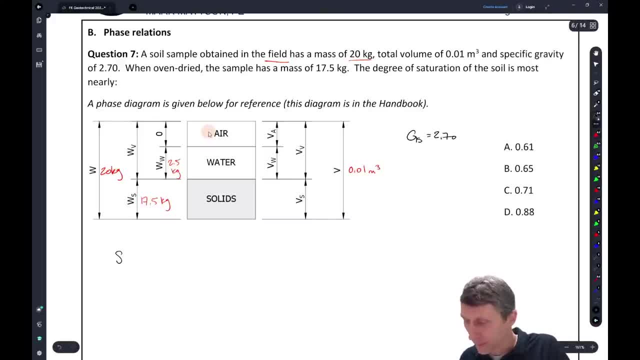 So so the two equations that we had: degree of saturation is equal to either the volume of the water divided by the volume of the voids, or the water content times the specific gravity over E. OK, so this questions Definitely more complicated. in right away. 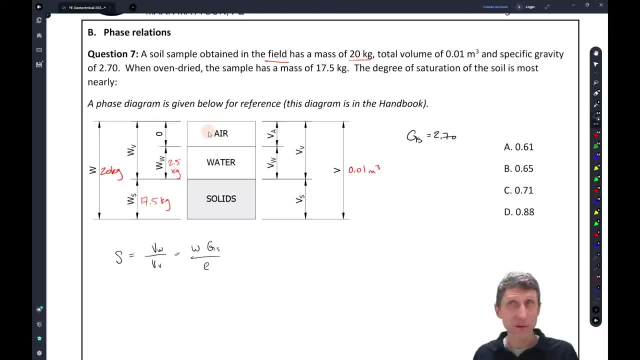 You can see that there's. there's some bigger pieces here that I have to figure out, because I don't know the void ratio. I don't necessarily know the water content yet. is what's the water content, or do I know the water content? Can I find the water content? 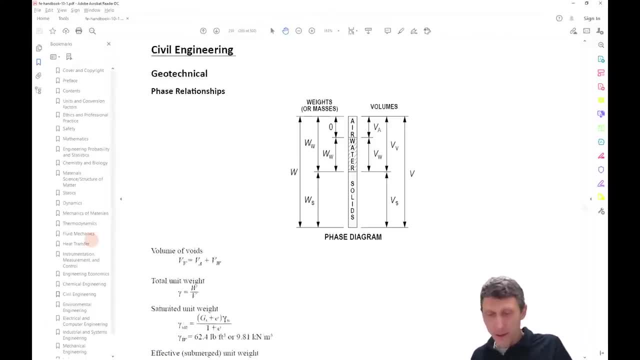 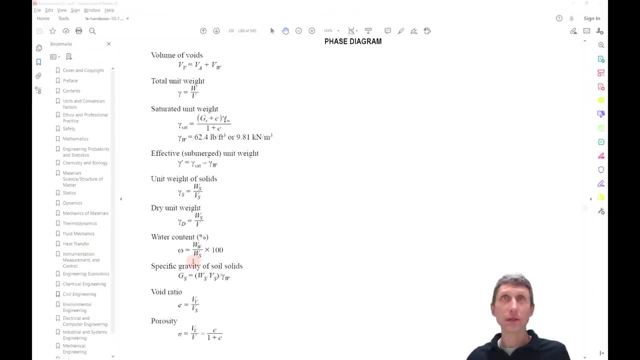 Maybe I can. Let's go look. What's the water content? right, The water content is is what the weight of the water divided by the weight of the solid, so I can get the water content. That's pretty cool, So let's go look. 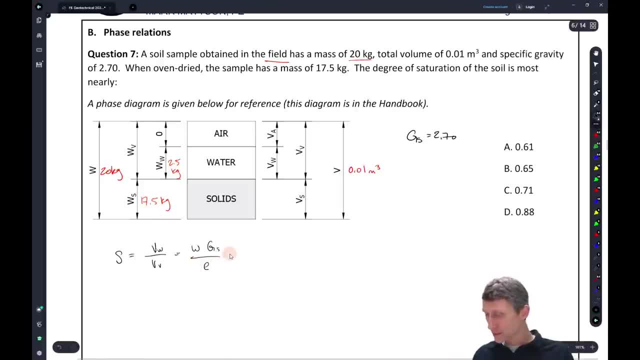 So I don't know. This is where you kind of have to piece This out and see: what do I know, What can I figure out, and how can I make this, this work here? So, OK, let's, let's, maybe we can go down this route. 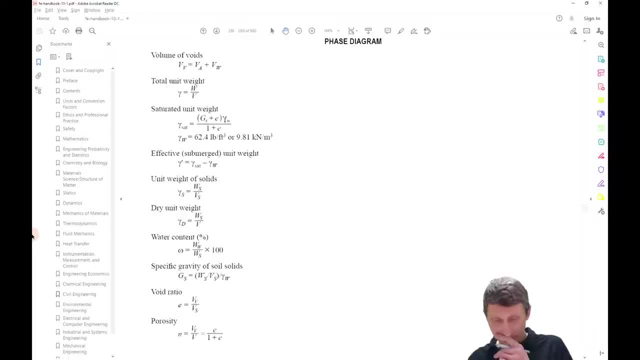 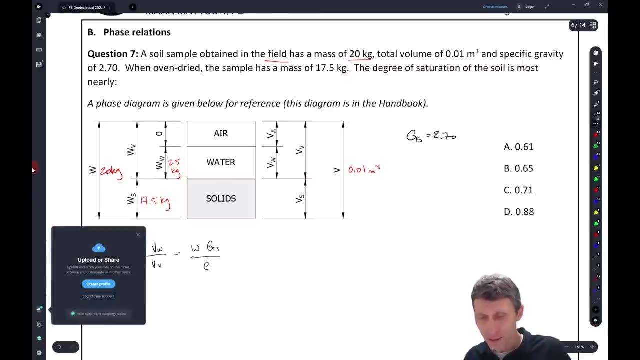 If we go down this route, though, let's look for a second. What's E? E is the volume of the voids divided by the volume of the solids. OK, so let's, let's just keep going here. So the water content we said is going to be the sorry, the water content. 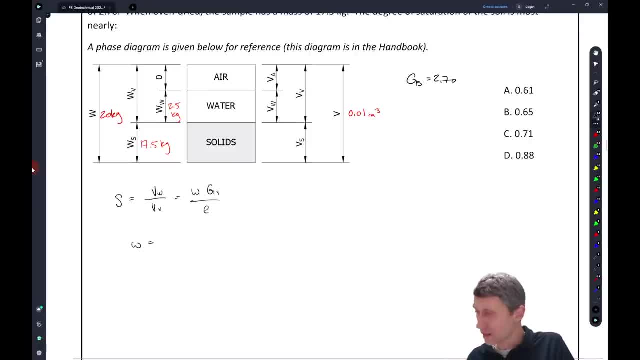 It's going to be the weight or the mass of the water, the mass of the water. So we just did this one earlier. Mass of the water divided by mass of the solids. the mass of the water divided by mass of the solids. 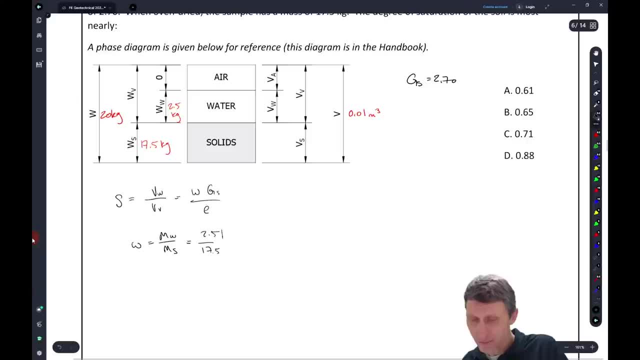 So with that, two point five over seventeen point five times one hundred percent, And honestly I think a lot of times I'll just leave the one hundred percent off, But we get what we get about. we get, Oh, two point five Over seventeen point five. 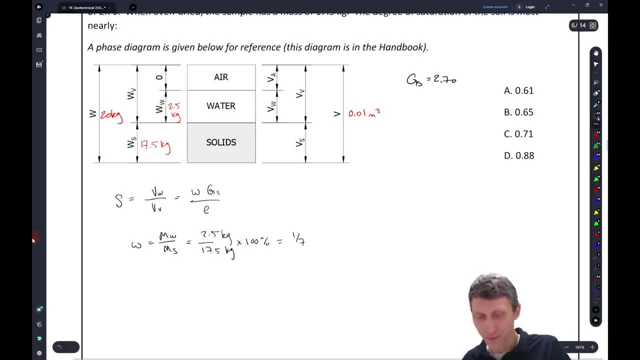 And that's actually one seventh, Right? So if I- if I don't multiply it times one hundred percent, I get one seventh. That's OK. It's like what? Fourteen point three percent, OK, That's good. So what else do we need? 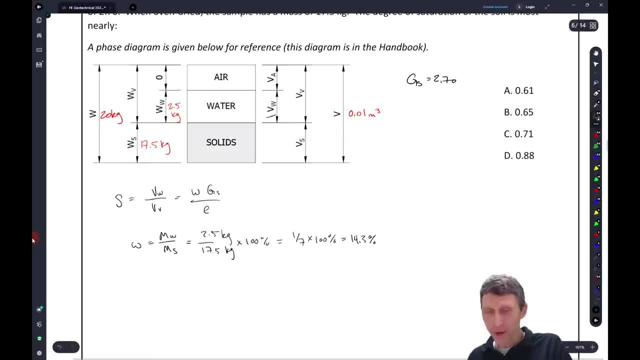 Well, we could go and we could find the volume of the water here, Right, Or we could find, But ultimately what we need is we need to find the volume of this, This, The voids, and the volume of the solids. 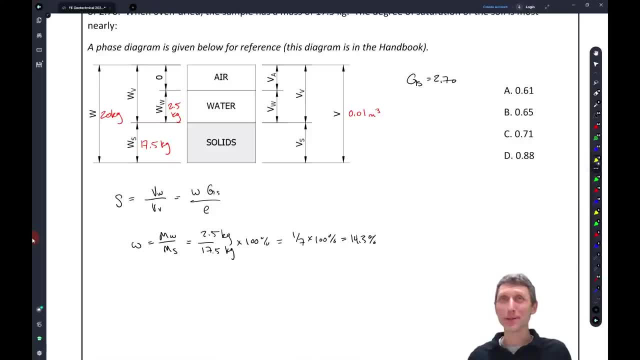 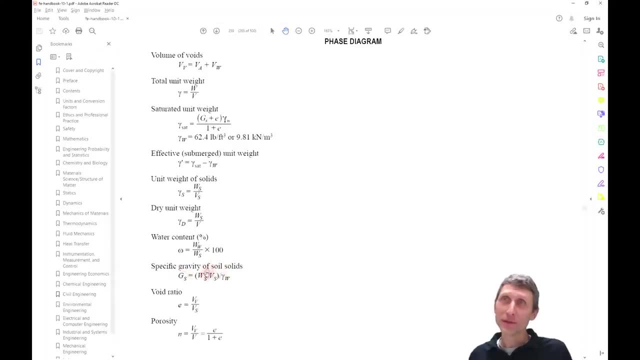 So one of the things that we just learned, or maybe remembered from long ago, is that specific gravity formula also comes into play here, Right? So if we know the specific gravity, sometimes you just look in and see: OK, what do I have? 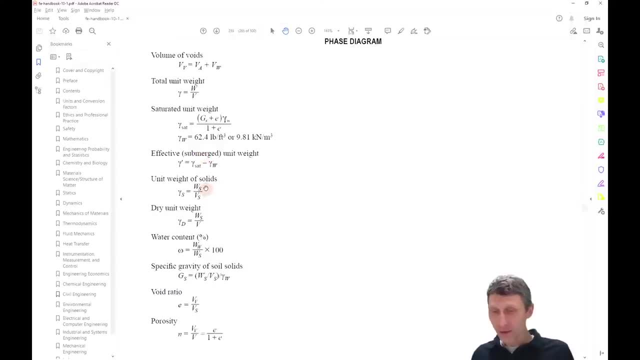 What pieces can plug in where I mean I know, you know, I could go from a gamma, I could go here and I can find my gamma, my solids, to find my volume of my solids, or I could just plug into this: 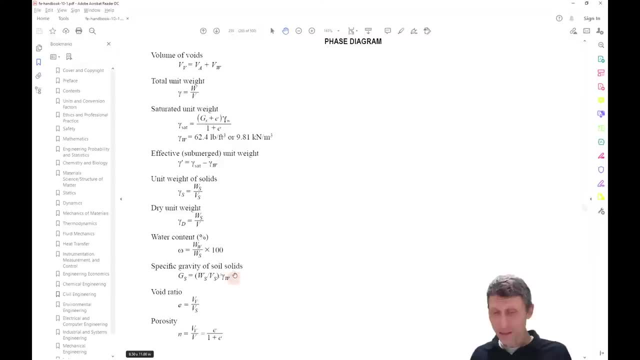 Equation, because I know my specific gravity. What pieces can I use here to make this work? And, honestly, I think this equation is probably going to work out for us. But let's take a look, Right. So? so if we take a look at that, 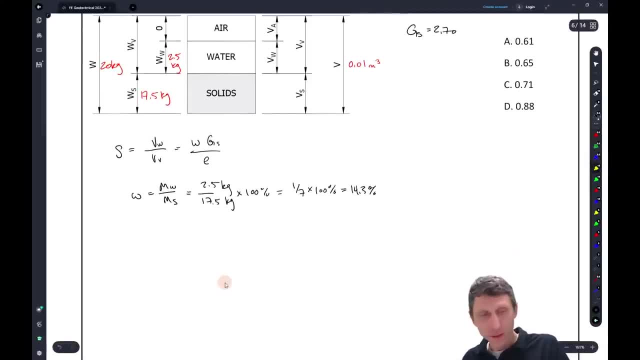 Let's, let's, let's try it. OK, So what do we get? We have the specific gravity equals the weight of the solids divided by the volume of solids Divided by Gamma W, and what we said the last time, this is going to be mass of the solids divided, divided by the volume of the solids divided by a row of water. 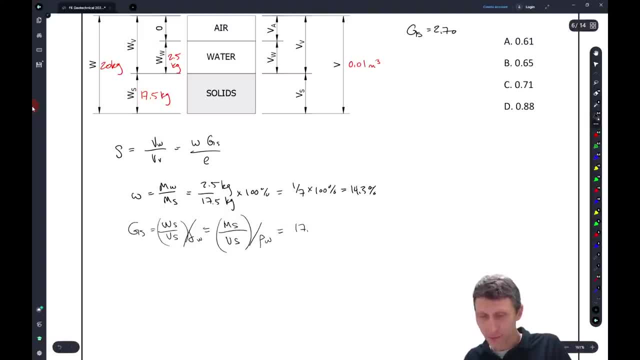 So the mass of the solids was 17.5 kilograms divided by the volume of the solids, which is something we don't know yet. OK, we don't know that value yet Divided by row of water. OK, so row of water. 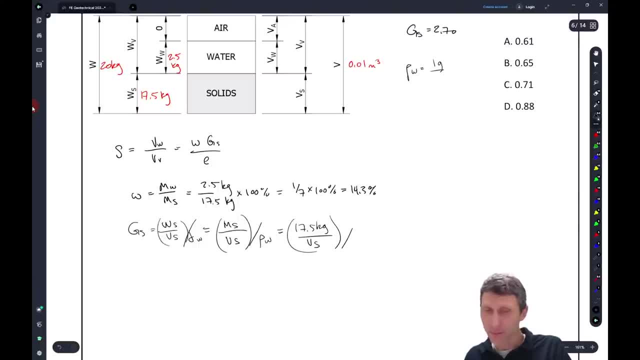 What we just Had. we just said row of water was equal to one gram per cubic centimeter. But the problem, or maybe a problem, is we have kilograms and grams. So what do we have to do? We have to convert it and maybe know this conversion already. 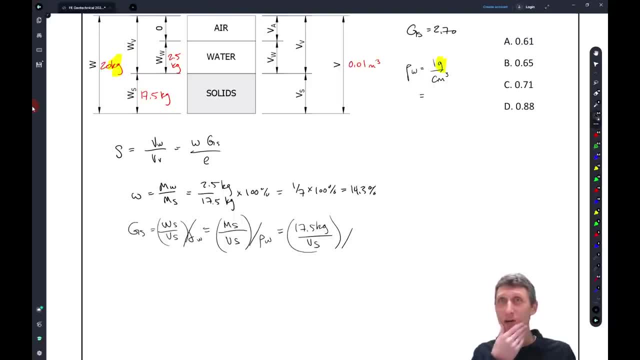 Maybe you don't, Maybe this is one of those ones that you want to write down somewhere in your recesses of your memories that you remember it. But what would we give? I mean, if we multiply it? we could use conversion here. 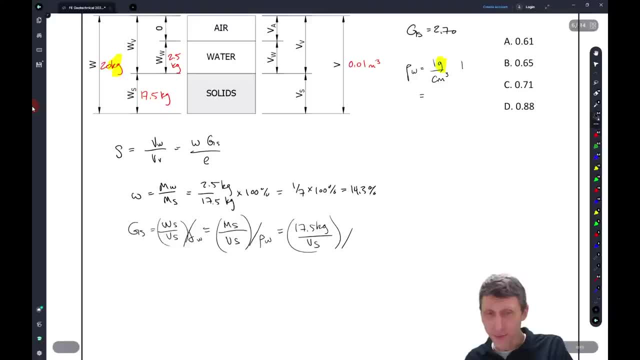 But essentially what we're going to get is we're going to multiply by 10 cubed and divide by 1,000.. Why is that? Because we have 1,000 grams per kilogram and 10 cubed centimeters cubed per per watt per meter cubed. 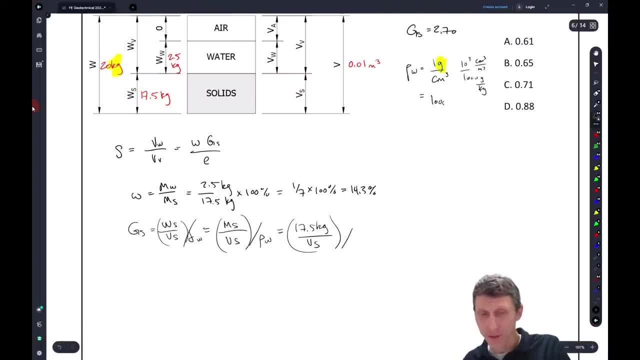 So that's going to get us our conversion, which is going to mean we're going to 1,000 kilograms per cubic meter. OK, so we have that- 1,000 kilograms per cubic meter- and that's going to equal 2.7.. 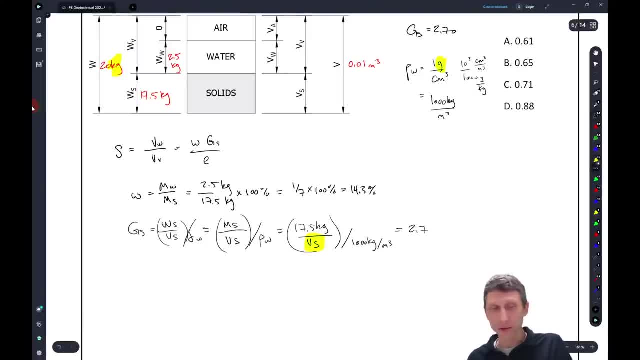 So we have to Come back and solve for this value right- The volume of the solids. And if we can solve for the volume of the solids, we've got this problem close. We're in its grasp, OK. so with the volume of the solids is going to equal. we got to rearrange a few things. 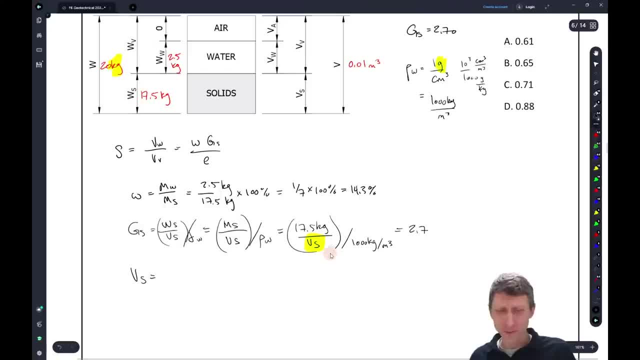 We're going to multiply both sides by more. What are we going to do? We're going to multiply both sides by divide by 2.7.. So we're essentially getting 17.5 divided by 2.7. divided by 1,000 is going to give me 0.006.. 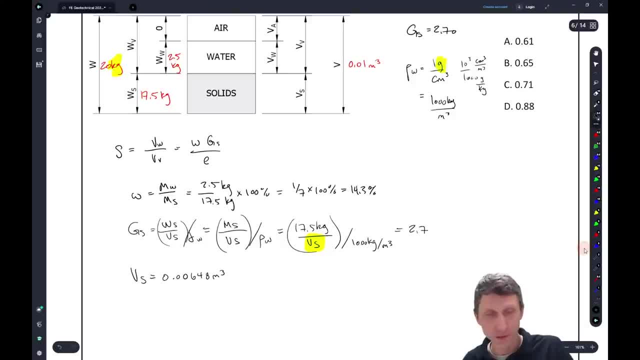 40.. 8 cubic meters. So I like to, once I get something I can use, I like to put that up here: 0.0065.. OK around that, But that means now I can find my volume of my voice right. 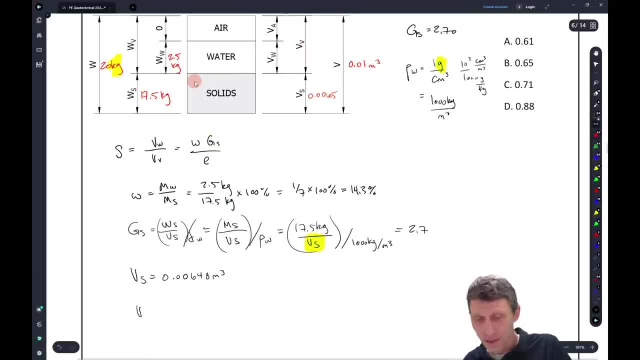 Because what's my volume of my voice? My volume of my voice is just going to be: the volume of the voice plus the volume of the solids equals the volume total. Or we could say: the volume of the voice equals the volume minus the volume of the solids. 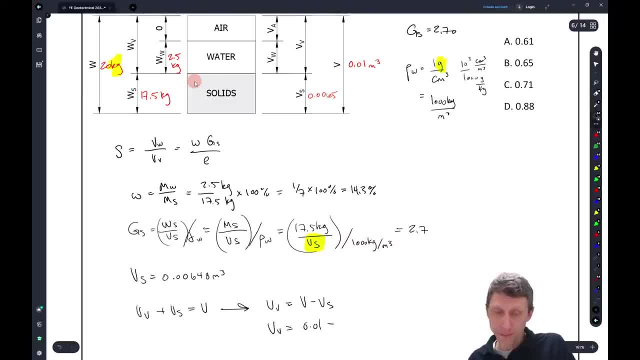 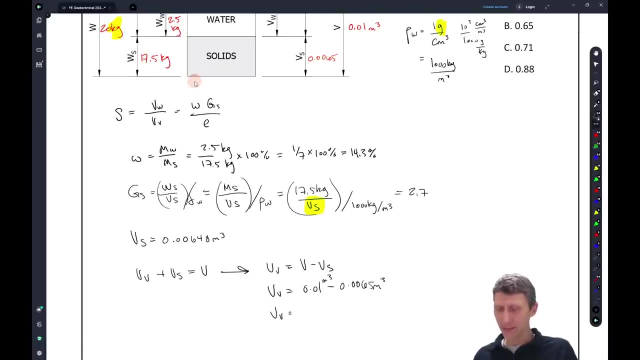 Right. so that volume of the voids is going to equal 0.01 minus 0.0065 cubic meters- And I'll keep my units in there because they're so important- And we get the volume of the voids equal to what's that? point zero one minus point zero zero six five. 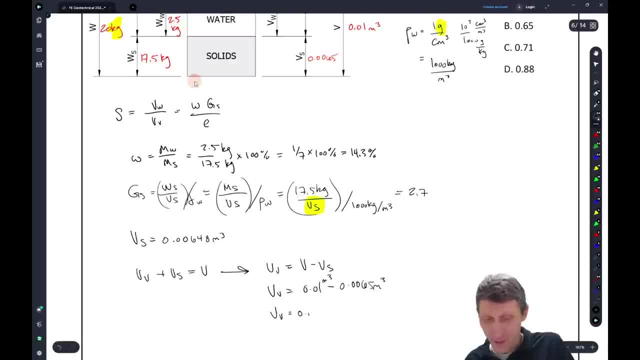 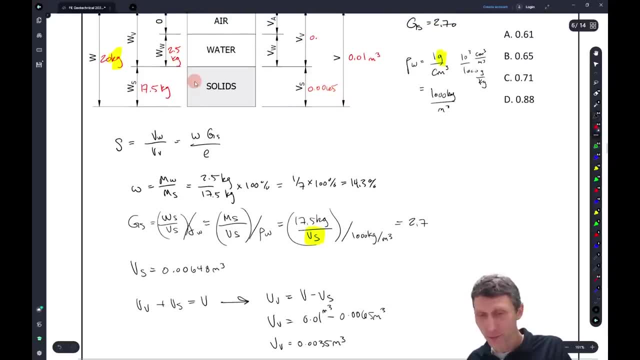 I like to put these into my calculator, just because otherwise I tend to screw them up with zero, zero, three, five cubic meters. OK, so now we have that value and we can come here 0.0035 and keeping this, this in focus here, what equation are we going to use? 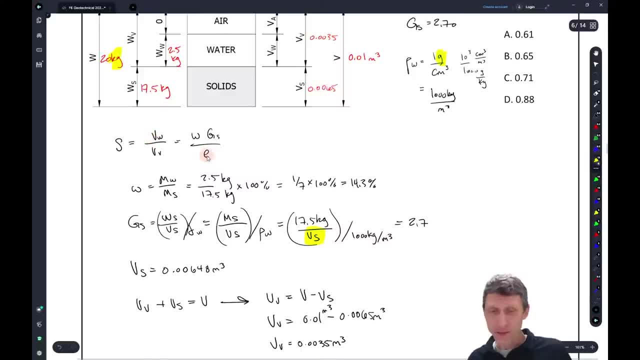 Well, we could either come back and solve for our volume of water, We could solve for our void ratio. Honestly, I think the volume of the water is going to be the easiest one to solve for here. And the volume of the water is going to equal what? the volume of the water is just going to equal our 2.5 kilograms divided by the density of the water. 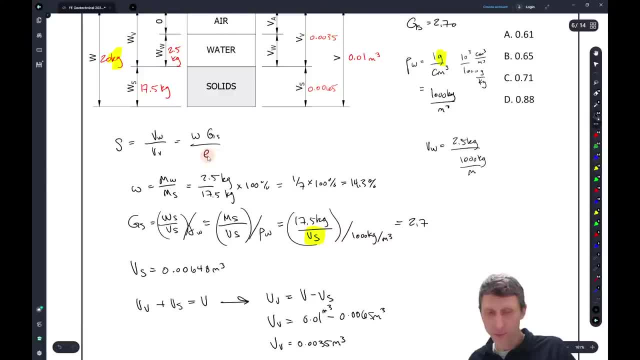 which is our thousand kilograms per cubic meter, has a 2.5 divided by a thousand. I shouldn't need to put that in my calculator, but it's late and I'm you know. I mean you're going to be going a mile a minute on the test here. 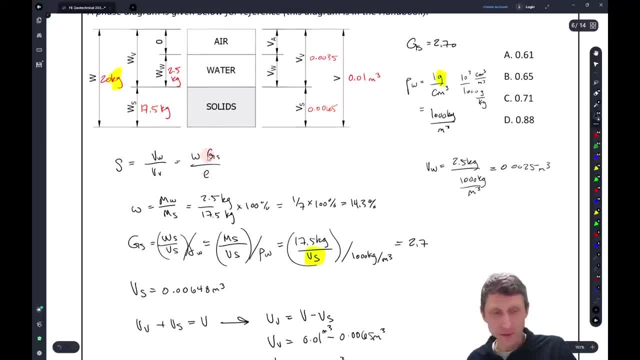 But point zero, zero, two, five, point zero, zero, two, five, zero. point zero, zero two, five. So what does that mean? It means the volume of the air is your point zero, zero one. OK, because the volume of the air plus the volume of the water 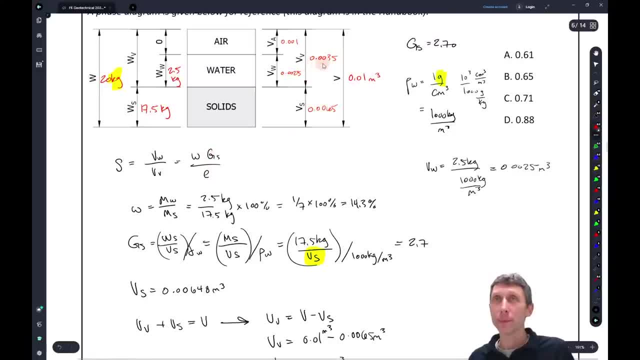 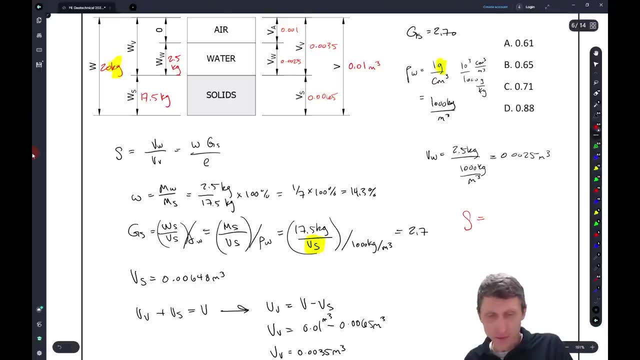 Has to equal that point. zero, zero, three, five. OK, And now again we could go and solve for our, our void ratio. but this equation is going to be the easier one to use And we can say: the degree of saturation equals the degree of saturation as equals the volume of the water. 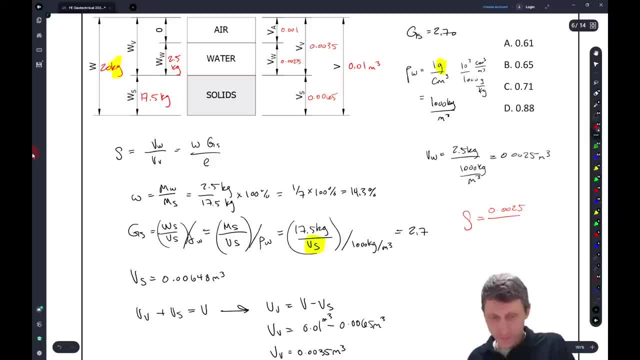 which is zero point zero zero two five Divided by the volume of the voids. volume of voids is point zero zero three, five. And let's see what we get. Well, I got about point seven one, So I got zero point seven one, which I'm going to go with. 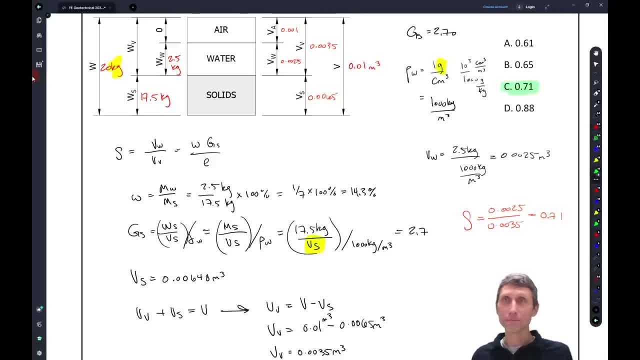 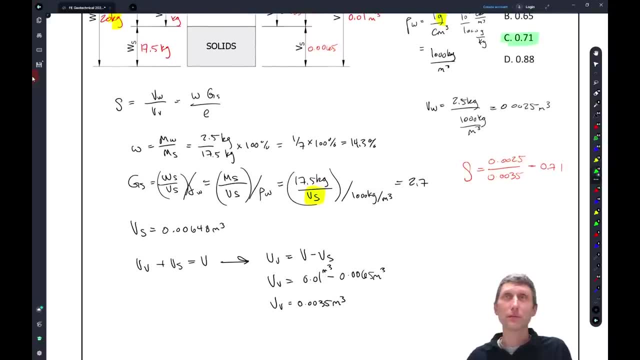 So I'm going to, I'm going to take that as our answer And we should be good. We could solve it the other way. And just for completeness, let's, let's do that, But let's, let's go and look, just for completeness. I mean, not that you're gonna have time to double check things on the exam. 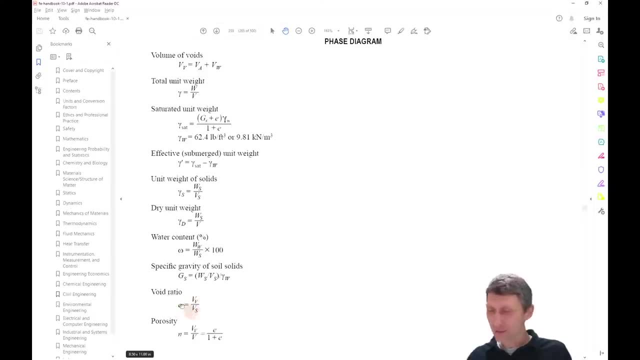 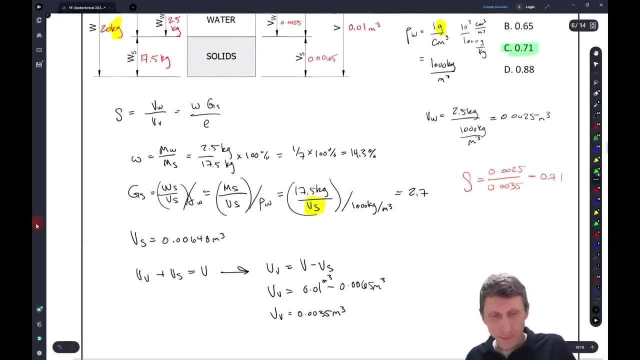 But what's this? This is the void ratio. E Is the volume of the voids divided by the volume of the solids. right, So E we could have. just we could have stopped here, We could have found E right, What's E? We could say: I'm just curious. 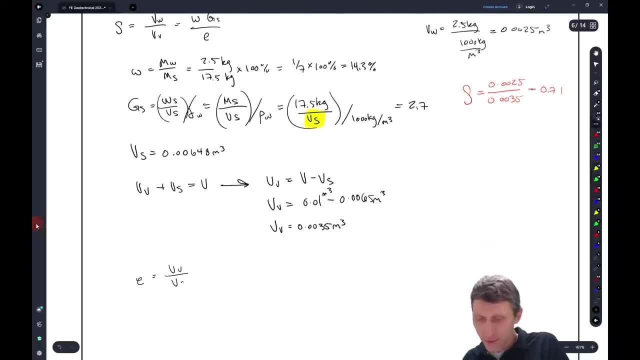 Let's. let's do this. E equals the volume of the voids divided by the volume of the solids. So the volume of the voids is zero point zero, zero, three, five. The volume of the solids is zero point zero, zero six, five. 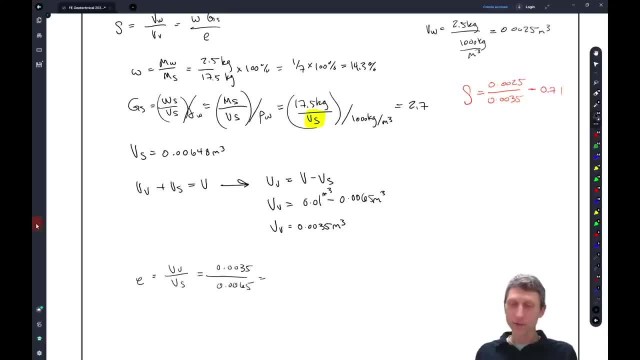 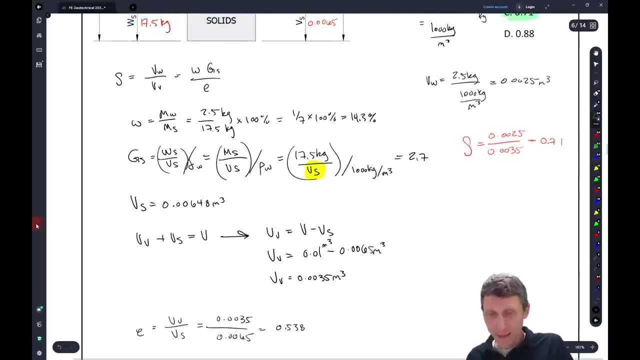 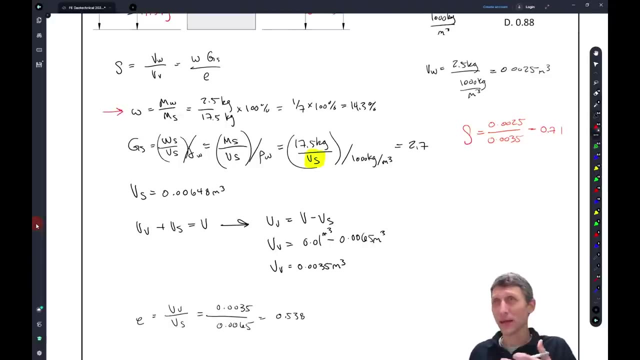 So point oh three, five divided by point oh six, five is like point five or roughly zero. point five, three, eight. OK, And what else? I mean, did we really need to solve for this water content? Not really, unless we're doing it this, this way. Right, But what do we get? 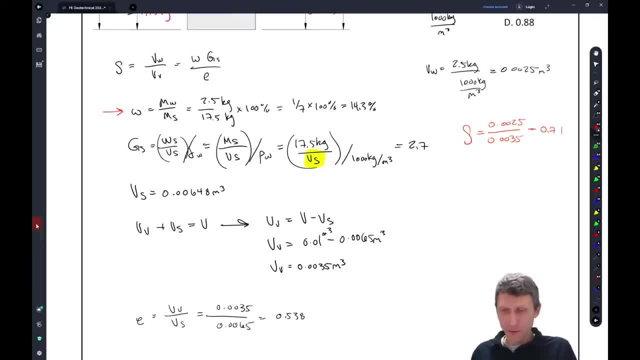 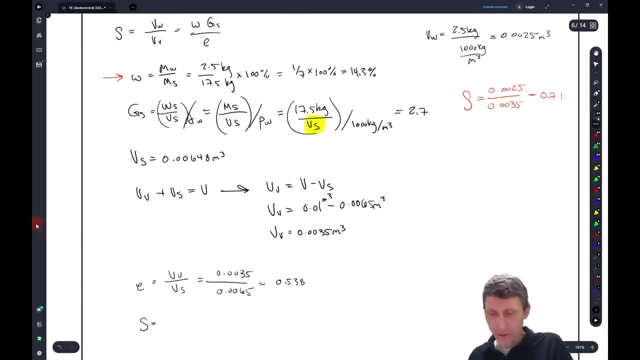 We get the So, so we could solve, We could solve all this Right. So we could say the one seventh- Let me read it out- to the degree of saturation Also. alternatively, could equal the one Seventh for our water content times, or two point seven divided by zero point five, three, eight. 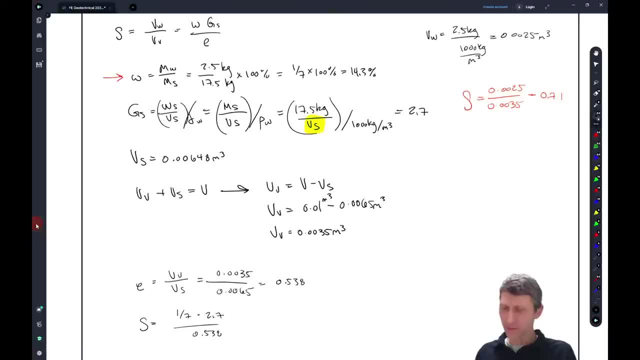 And let's see if we get the same answer And we get like again, we get about zero point seven. This is like seven one seven. It's close, OK. so if I, if I kept more significant digits, I think I'd be at that point seven one. 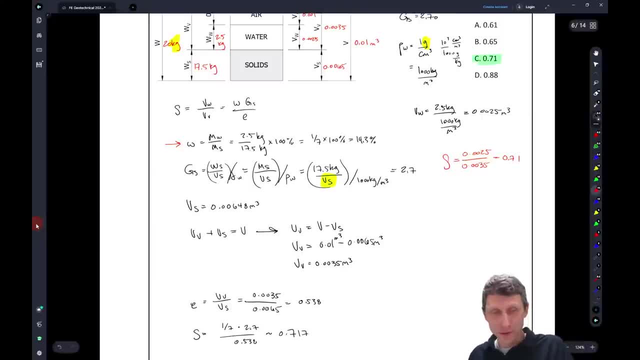 So, either way, you know whether you use, whether it would you know, whichever formula you use, whether it's the first one or the second, when you get the same place you might be saying: but that second one looks so much easier. 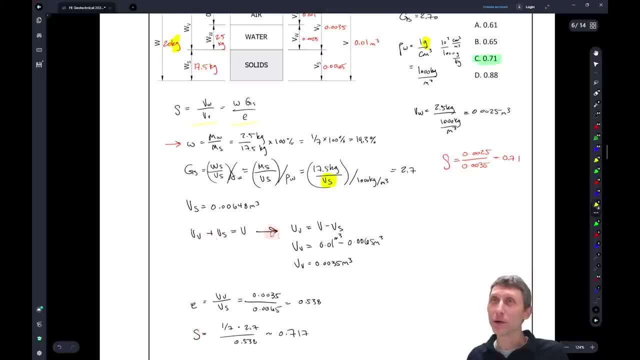 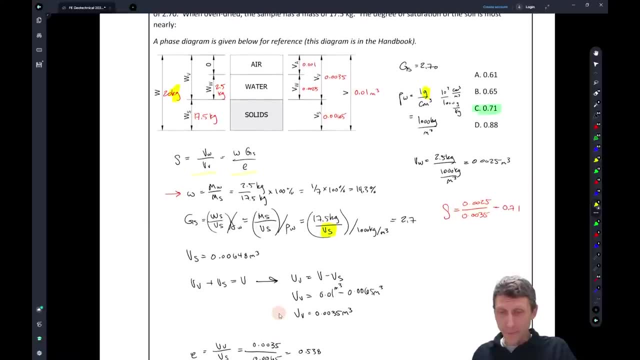 And the reason it was easier is because we had already solved for the volume of the voids, We had already solved for that volume of the solids And we've gone through this Right. So that's that's. that's where it's at, OK. 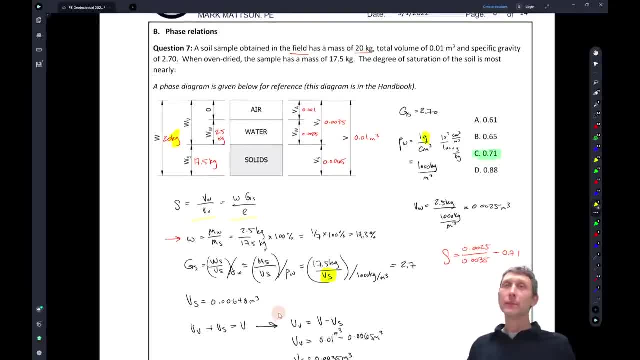 So these can get complicated, They can get messy, But the. what I would suggest is, if you get a phase relations problem, take the, take the. you know the little bit of time right down here You're for, you're not your formula, phase diagram here and in. go from there, write down what you know, what you don't know. 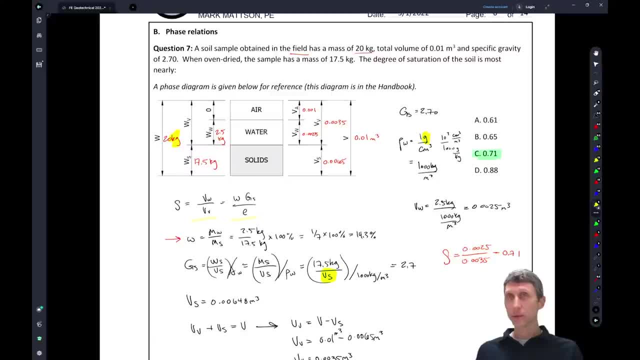 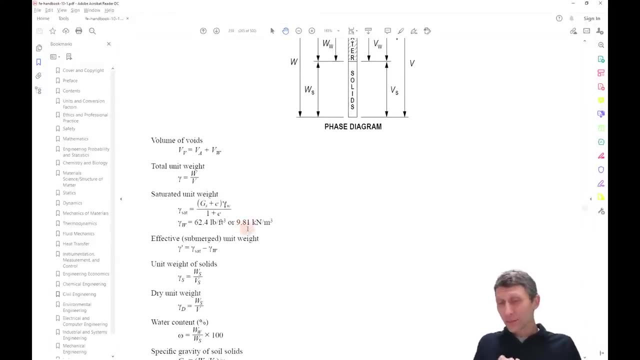 and then start looking at the equations and seeing which ones will work to get you what you want. But again, using these, if you're given mass, you kind of want to know some of these mass units in SI because, again, as we come back to, as we come back to, to what we have here, we're only told this nine point eight, one kilonewtons per cubic meter. 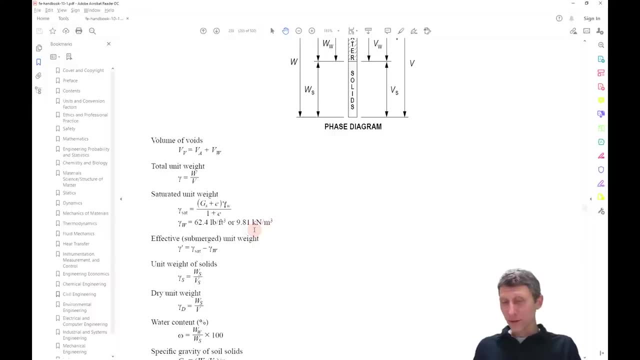 We're not told kind of the density, We're told the unit weight of water, But a lot of times in metric you're using grams, and grams per cubic centimeter or kilograms per cubic meter. So just something to think about, something to keep in the back here your mind. 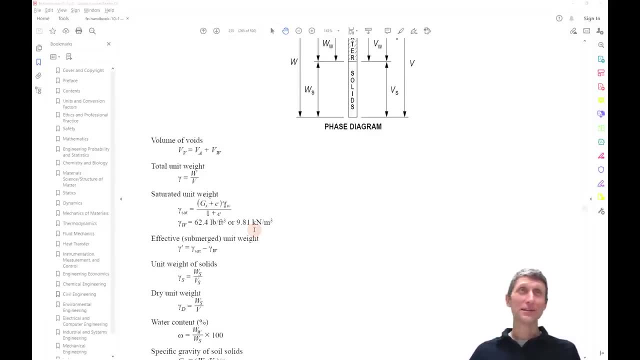 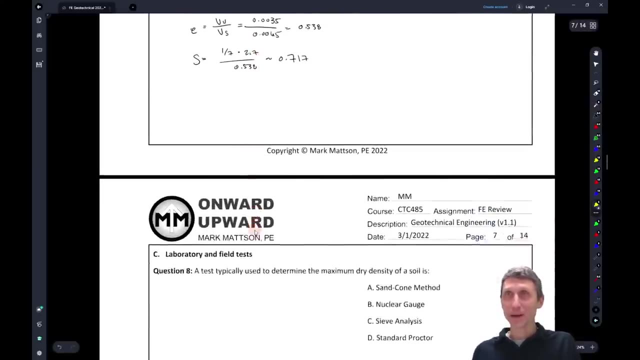 And one of those conversions that, hopefully, will get you a right answer on the past, because that's that's where you want to go. I mean, you want to be at the point where you're getting these, these things and get them right. OK, that was a long one, We'll follow with a short one. OK, 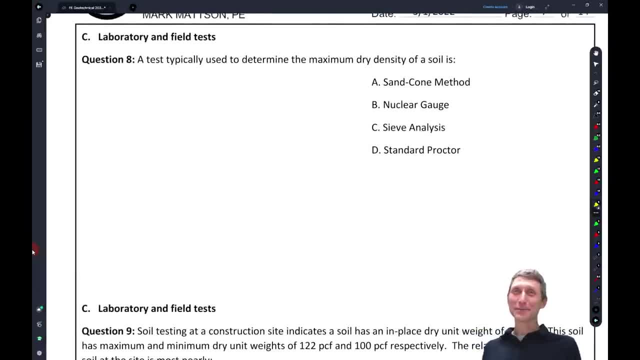 And you'll notice a theme in my my answers to these concepts Questions here. But a test typically used to determine the maximum dry density of soil is what? So I just threw out a whole bunch of of of tests that you might see in your, in your lab. 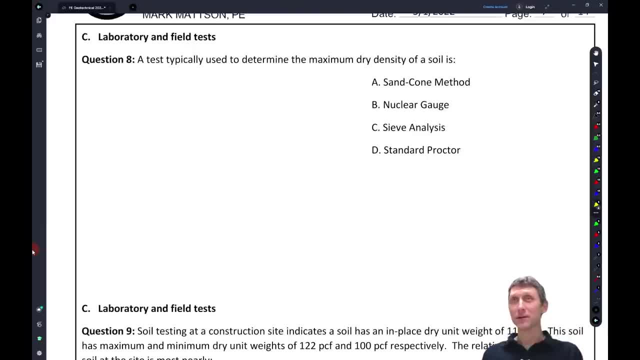 I taught a soils lab at one point and it's like we did all these tests. you know the sand cone, the nuclear. Well, actually we didn't do nuclear density gauge, but that's, and that's typically what's used in the field. 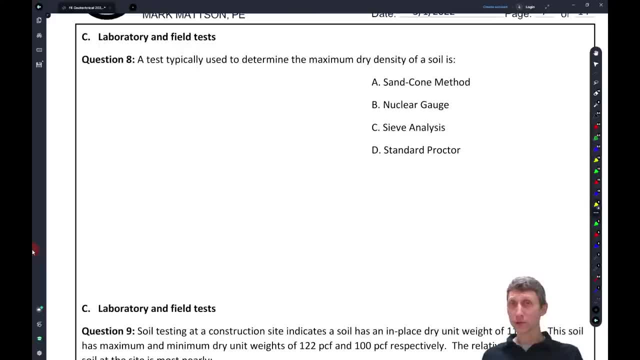 I saw that in the field quite a bit. where we'd get. we get reports from the field of nuclear density gauge readings, you know of people doing compaction And inevitably I remember one project where we had a four foot lift that was going underneath a building. 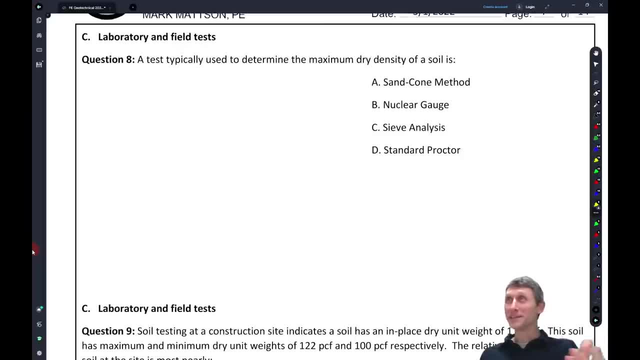 Four feet of soil was going underneath the building And what we said was we had to be, you know, we had to have one foot maximum lift to make sure that each lift is compacted. So four foot total, you know, total fill. But we could only do it in one foot lifts to make sure that each, each one was was compacted. 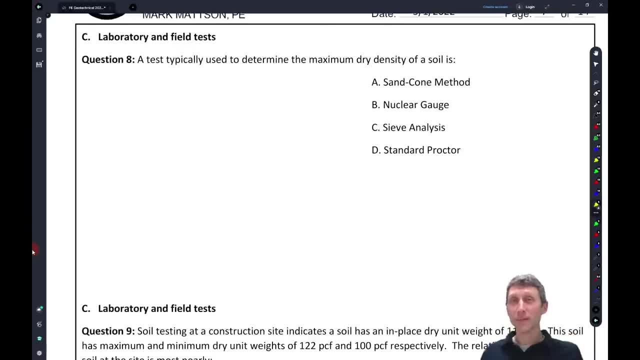 And, of course, the contractor- or a weekend- decided to put all four feet in And didn't get it tested. So this was- I think this is one of the first jobs I had when I was a young engineer. right out of college, My boss said, OK, go to the site and sit there while they dig it all up and put it all back in one foot lifts. 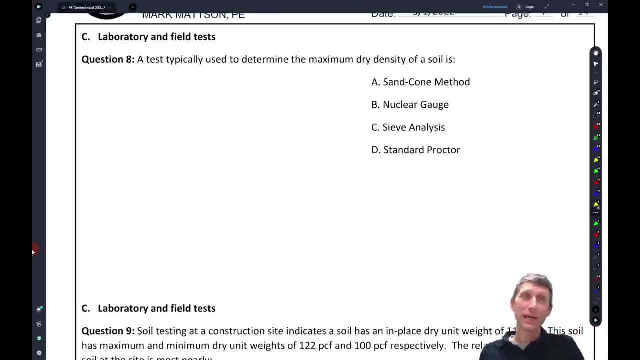 I said you're serious. I'm like, yes, I'm absolutely serious, Is what my boss you know he's like and we're going to charge him extra for this because they did it wrong And we're not messing around with the building. that was put in a big four foot chunk and didn't get compacted properly. 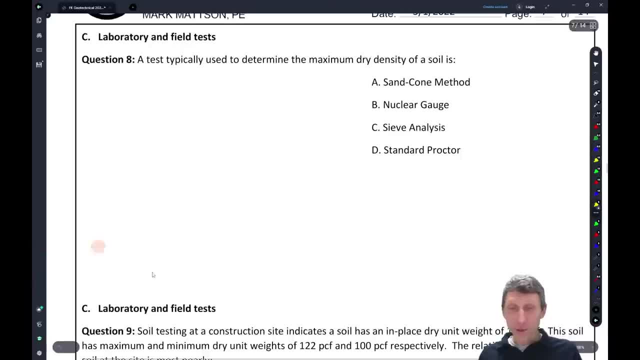 So nuclear density gauge? OK, so sorry, That's the story, But what nuclear density gauge? what is that? It's a way to check the relative density of a soil, Not the maximum dry density, So that checks the relative compaction density, just like a sand cone can kind of do the same thing. 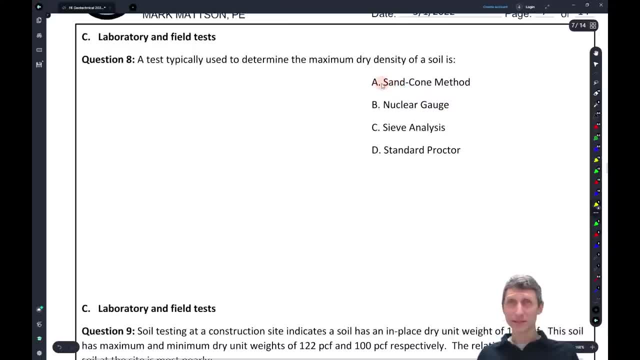 But this one you might have done in your, in your lab, where you know you take some out, you fill it with a known, a known volume of sand. The sieve analysis: we kind of talked about the sieve analysis and the sieve analysis does what it shakes the soil to get you a particle size distribution. 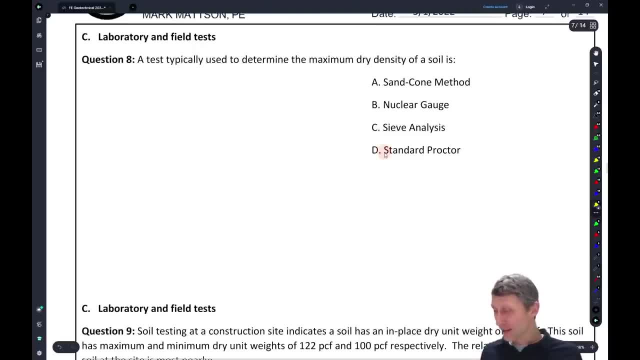 OK, so what's left here is a standard proctor. Do you remember what a proctor is? And maybe you didn't do a proctor in your lab? but what's a proctor? A proctor is where you have a. you know a can. you got a rod, you put soil in it and you poke it until it fills up, and then you measure some. 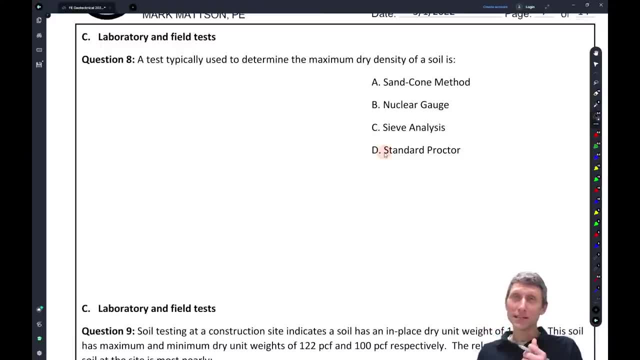 This is a really crude drawing, but you measure essentially compaction effort and eventually you get a curve right. You get this curve- and maybe you remember this- this curve- the dry density Versus the water content- right And eventually you get some curve that looks like this: you know, and it's in. what you're looking for is that maximum dry density based on water content. 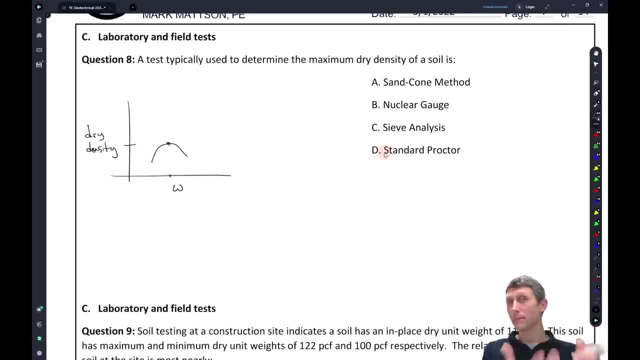 Because if you get too much water it just becomes soup, right, It just becomes a mud and a mucky mess and you can't, you can't get it dense, no matter how how much you try. If it's too dry you don't have enough kind of lubrication there. 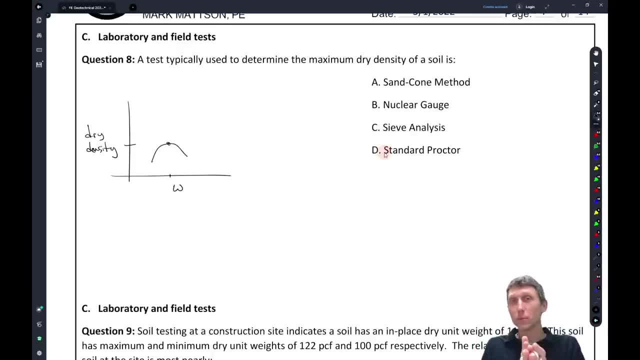 You can't get the particles closer together. But if you get the optimum moisture content, the optimum water content, you can get the right amount of compaction. So that's what we're looking for here. Dry density Sometimes you can use like this might be, a standard proctor curve. 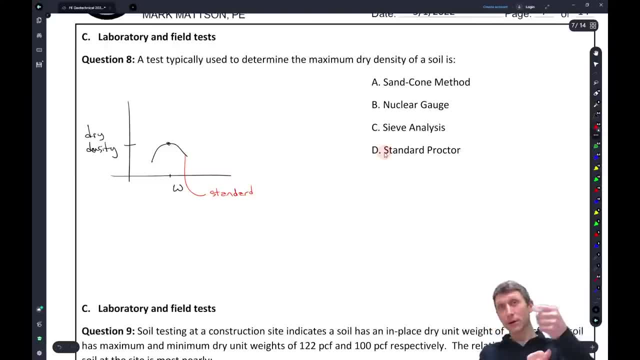 You can use more compaction effort with a bigger hammer for a modified proctor curve And you might have a modified proctor curve that looks like this, And what this does actually is: it approaches this idea here of a zero air voids curve. 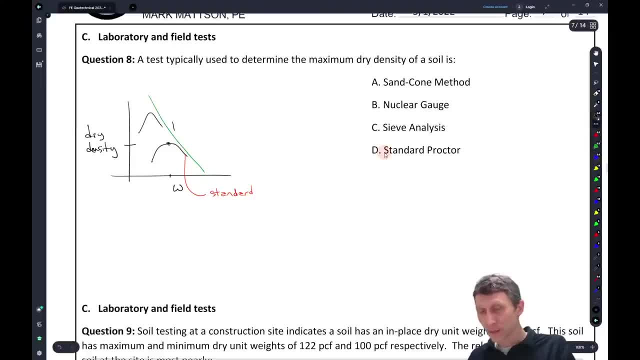 And this is kind of a zero air voids. It's 100 percent. It's kind of like 100 percent saturation, Zero air voids, right. But what you're trying to figure out is what is that maximum dry density? Because when you put in those lifts- right, whether it's under a roadway or it's under a building or wherever it is- 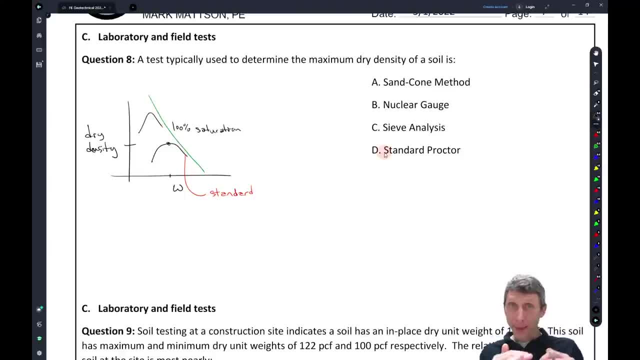 when you're putting in that soil, you want to make sure it gets put in compacted. You want it. You want it solid. You don't want to have settlement that you can take care of just by some compaction effort. So that's what we're going to. 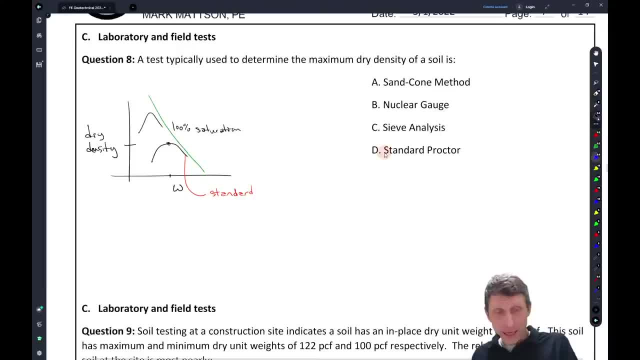 That's what we're going to look for here, But but basically this answer goes to that standard proctor. Hopefully that's one of the tests you did in your soils lab When you took a soils class. Hopefully you did some of these other ones, like a sieve analysis or a sand cone. 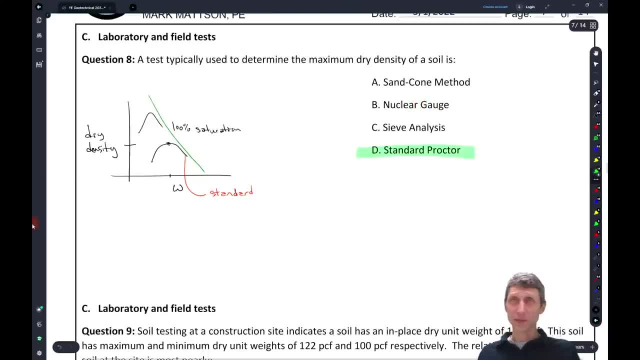 Probably didn't do a nuclear density gauge. But if you get into the field and do any soils testing in the field, that's one of the ones you'll probably see out there as well. Sometimes this will be calibrated in the field with a sand cone, but it just depends. 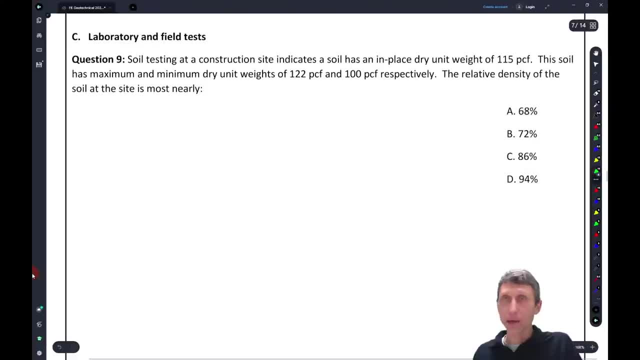 It depends on the job, depends on who's doing the testing and what's what's required. So again, laboratory and field tests. What's the point? The point is we want to make sure the soil gets put in. I appropriately. 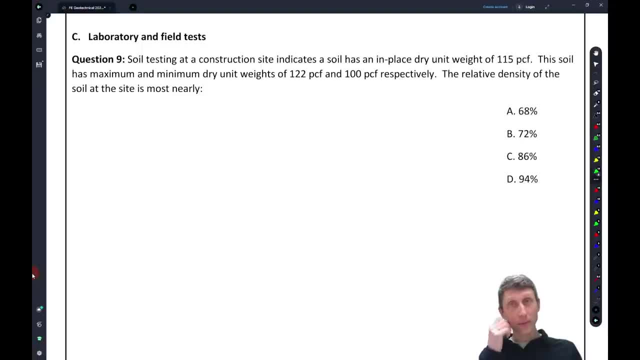 Right. We want to put in appropriately, whether it's in lifts, or we want to put in the right soil, So that does what we want it to like in a dam, Typically. you want impervious layers and then you want pervious layers. 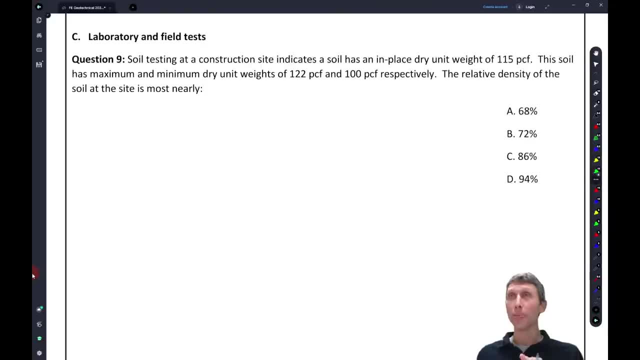 You want certain layers that drain and certain layers that don't drain. OK, In a, in a, in a roadway, A lot of times you'll want strong materials, like a whole bunch of rocks or whatever, to create a nice base. OK, But what we have here is your soil, soil testing and construction. So it indicates that soil is an integral In place dry unit weight of one hundred and fifteen. So this is our field weight. Our field weight that was measured whether it was a sand cone or nuclear density gauge. One hundred and fifteen pounds per year per cubic foot. 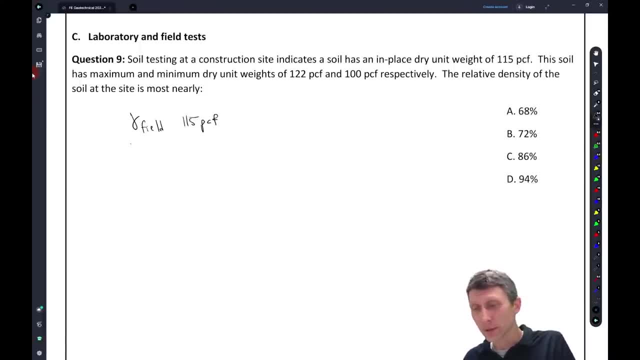 OK, We have a maximum, minimum dry weight. So gamma max is going to be one hundred and twenty two pounds per cubic foot And gamma min is going to be one hundred pounds per cubic foot. So these are. you know, These values here are from the lab. 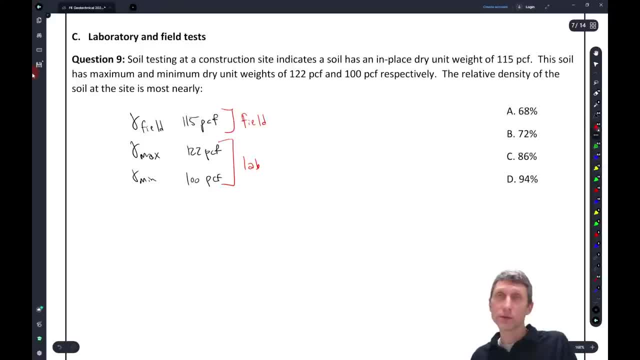 This value here is from the field And basically what you need to do is when a soil is going in and you want to make sure that it might be specified like in the spec is like ninety five percent standard proctor compaction. What? what that means is it needs to get installed to a certain density in order to be acceptable. 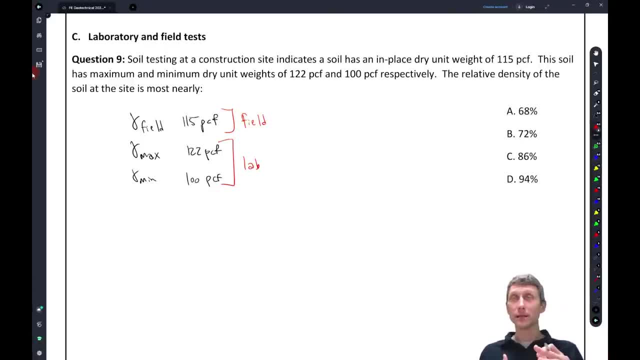 OK, And that limits it kind of limits the consolidation of that material, because you're putting it in at a pretty consolidated state. It basically creates a known condition, if that makes sense. So what we're trying to say is: what's the relative density to the soil? 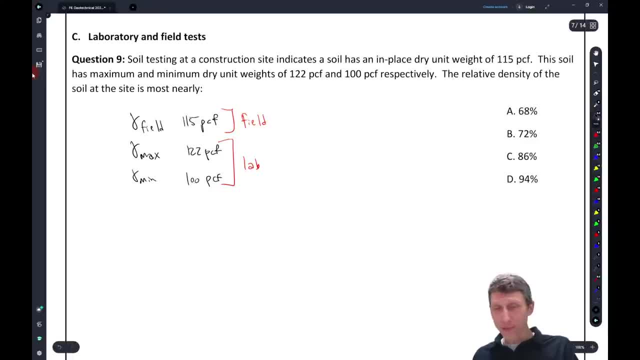 So some of you are probably going to be tempted, because it's the FE you just want to get this over with. You're just going to take the one fifteen divided by one twenty two. I mean, that's, that's an answer here, But that's actually. this is the relative. 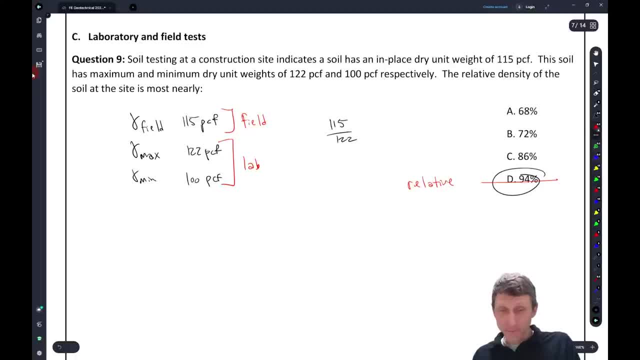 That's the relative. The relative, not density. But let's go to the manual here and look for a second and see what that is. So if we, if we, come back to the manual here for a second- Actually, let me get to the manual here- 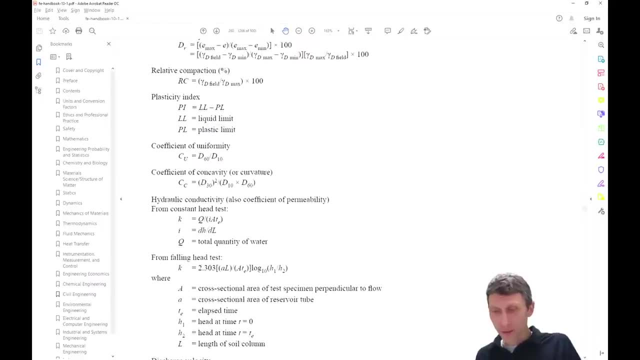 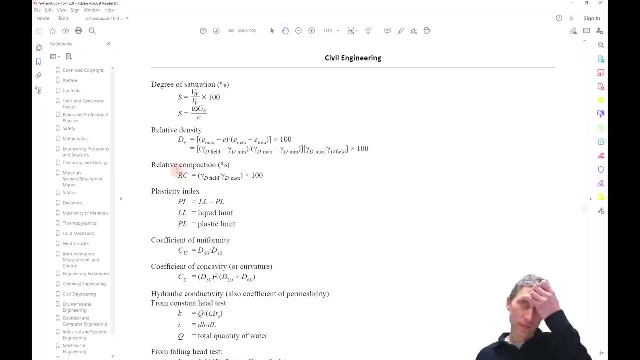 So if we come back to the manual here for a second, What do we have? Well, let's, let's come back here. We have relative density versus relative compaction. OK, So be careful between those two terms. the relative compaction is the one where you have your field density divided by your maximum. 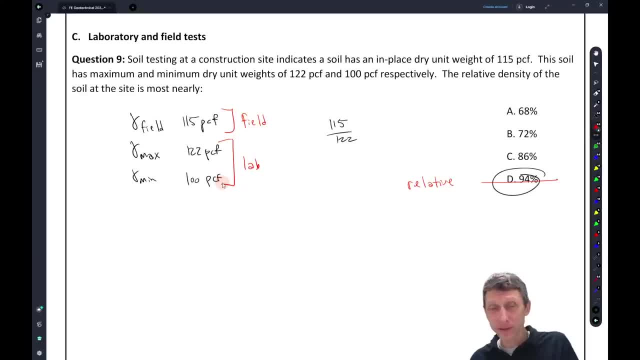 That's what you're looking. That's typically what's specified. It's typically like: it's like a 90.. You know this might be the 95 percent. you know standard compaction or relative relative compaction, So that might be. that might be specified in the spec right. 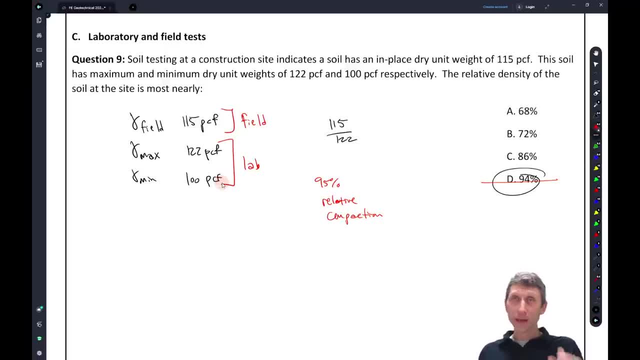 And normally that has to be within a certain water content. If it's too dry, you'll have to actually add water in order to get up to that much, And if it's too- you know- too wet, you'll have to dry it out Or wait for it to be dried out. 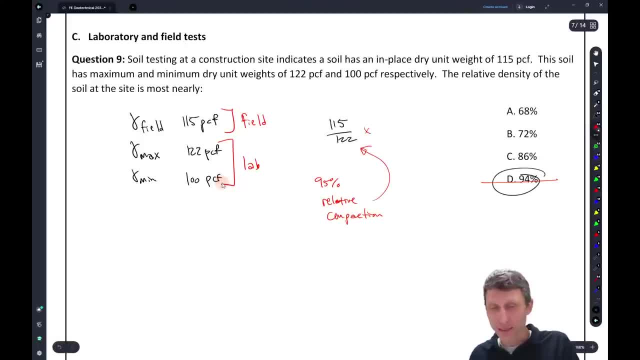 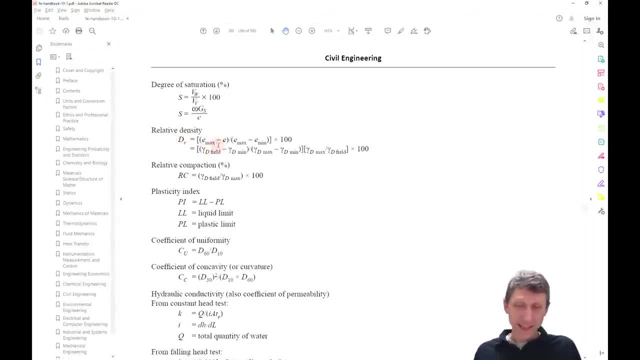 OK, So this is. that's the relative compaction, That's. that's not what we're doing here, But the relative density: Right, We have another formula here. The relative density is going to be: we could either go with with void ratios or we go with what's measured in the field. 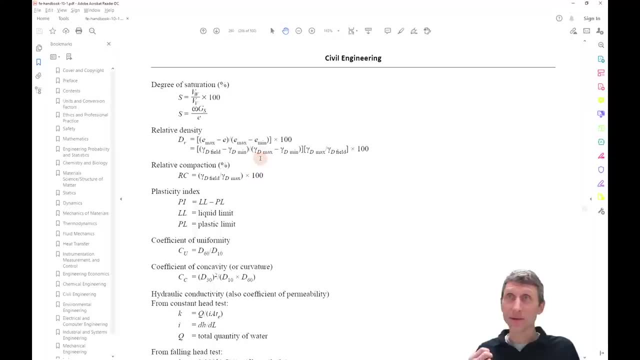 And what's measured in the field here is going to be this: gamma minus gamma, gamma minus gamma, gamma over gamma. Right, There's a lot of gammas going on here And you just want to make sure that you get them right, So I'll try to write this down. 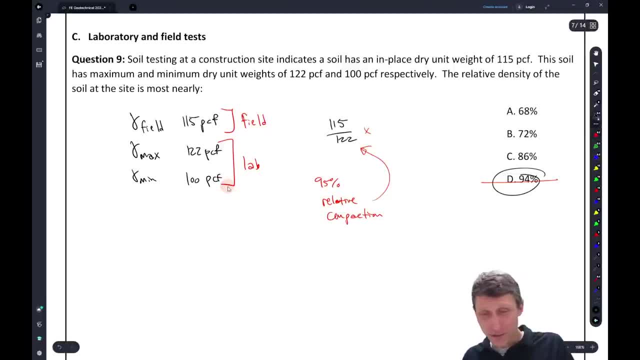 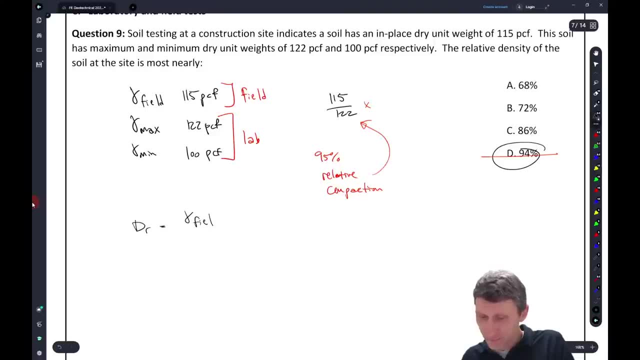 Hopefully I get it right here, But if I don't just shout at me, shout me down and we'll fix this. But DR is what it's: the gamma, the field, Minus the gamma min, And I'm dropping the D's here. but gamma max minus gamma min. 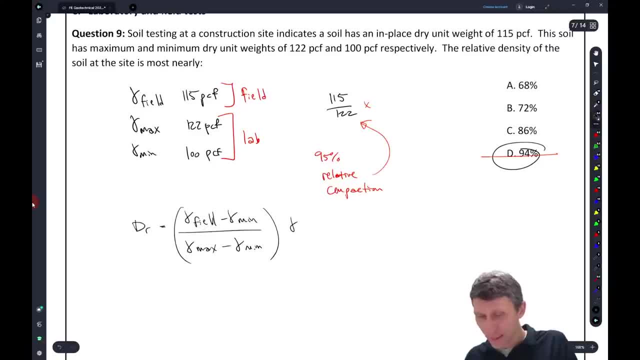 OK, And all of that times what gamma max divided by gamma field. So that's kind of just a little bit. That's kind of just a long plugging chug equation. But the reason I threw this one in there is because I wanted to just just to step back and think, especially with relative compaction versus relative density. 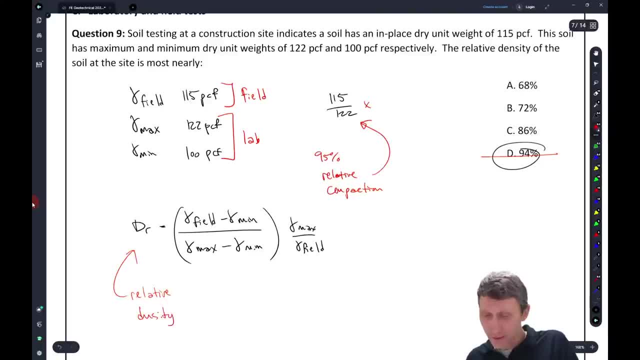 OK, So these are two different numbers and they're you know, they're both useful numbers, are just different numbers, OK, So what we're going to get here is, if we plug this in, gamma field is 115, and I'm going to leave the PCF off here, because everything's in PCF. Counts per cubic foot. So I'm not going to like get super crazy about this right now, But what we're going to do here is we're going to 115 minus what the minimum is going to be: 100 divided by our gamma max is 122 over 100 or minus 100.. 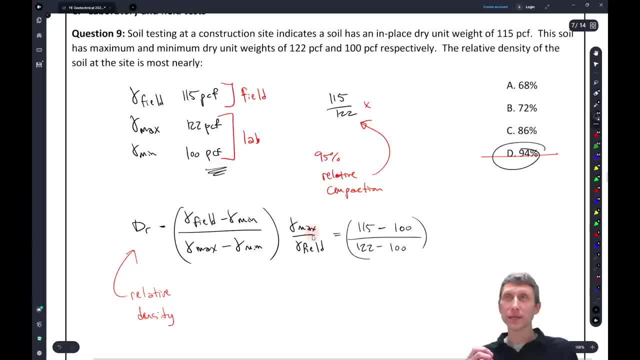 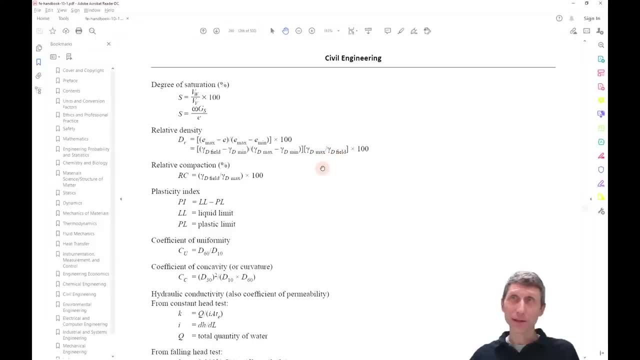 And then times. I think the first time I put this in I screwed up and I put gamma field over gamma max, And it's easy to make those mistakes because it's like you're trying to copy from one to the next. But gamma max over gamma max. 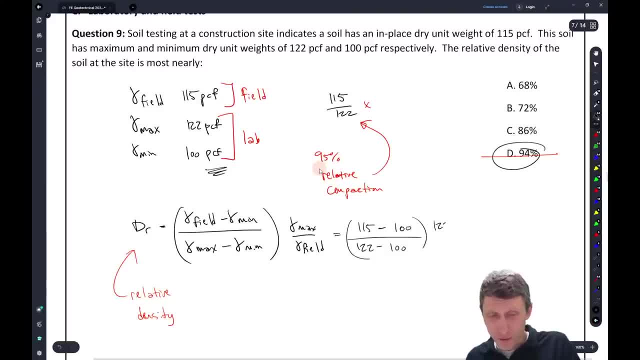 Gamma max over gamma field is going to be what? gamma max is? 122 over 100.. If you can put that into your calculator right, I think you get about 72 percent. So I did it earlier if I didn't do it right. 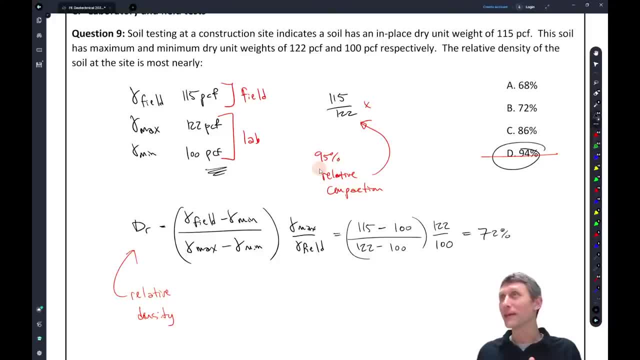 Somebody shot me down, But, Michelle, thanks. I mean I'm glad to do this. I hope it helps somebody you know And hopefully it'll go beyond just today as well. So if you do like it, you know, give me like whatever, But not seriously if it's, if it's helpful for you. 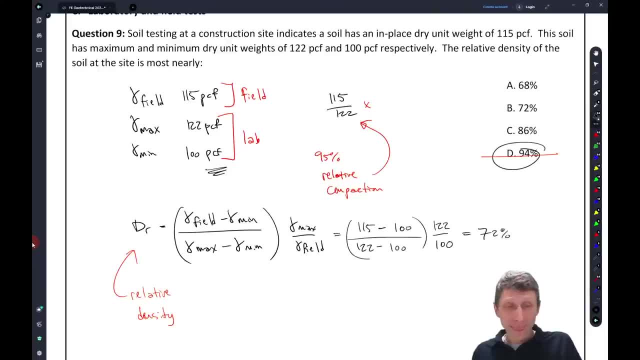 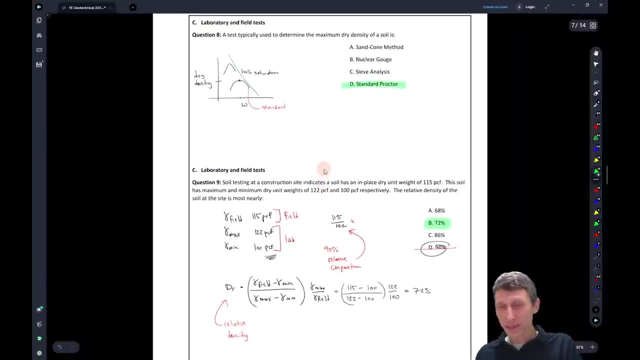 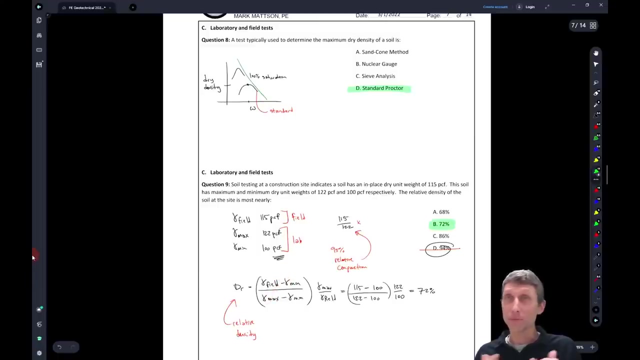 OK, I'm grateful for that. So I think this is where it goes and we get to that 72 percent, OK. So relative compaction versus relative density: Typically this is what's specified, Which, again, when we're looking at this- I put this with that proctor test because the proctor test is going to give us some of these, you know this, this maximum value down here from the lab. And that's going to kind of be our starting point, And sometimes I've had this happen in the field. I've had this happen in the field where, like no matter what the contractor does, they cannot hit their 95 percent relative compaction and typically either they don't have enough water or they're using a different soil, or the soil change. like they took one side of the sample, the borrow pit, and over on here the soil is a little bit different. 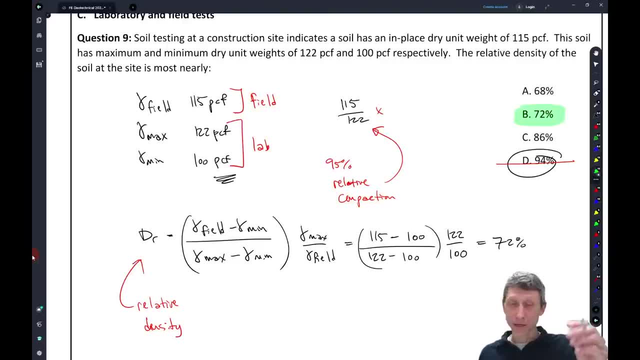 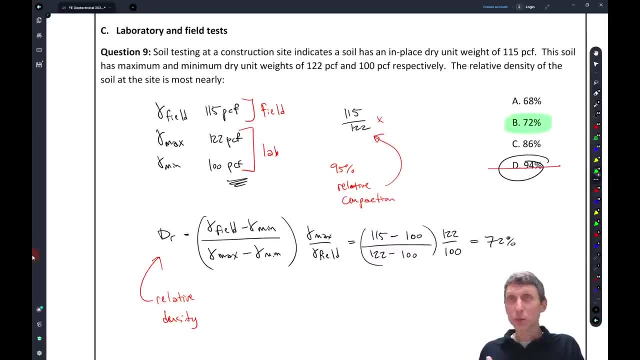 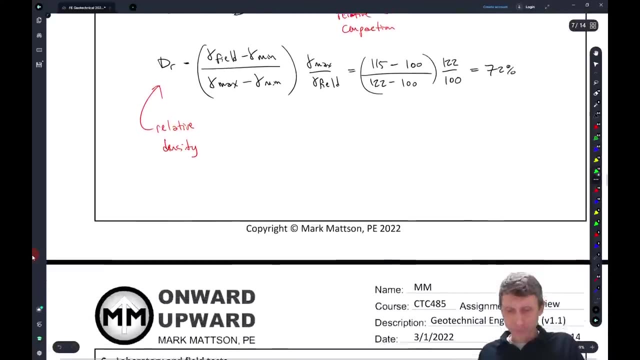 They need to go get a new proctor to recalibrate to make sure that they're actually getting the correct compaction. OK, So again, my field test. This is one of the ones that I ran into all the time when I was, you know, not just teaching, but doing a lot more real engineering. 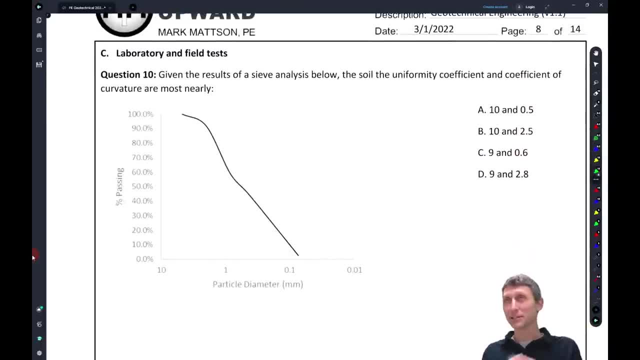 So not that this isn't real, this is teaching. this isn't real engineering, so to speak, but it is. it is just getting you ready to on the fundamentals. All right, Question 10.. Here we go. We kind of did this one earlier, but I think it's. this is specifically just looking at that uniformity coefficient and coefficient of curvature. 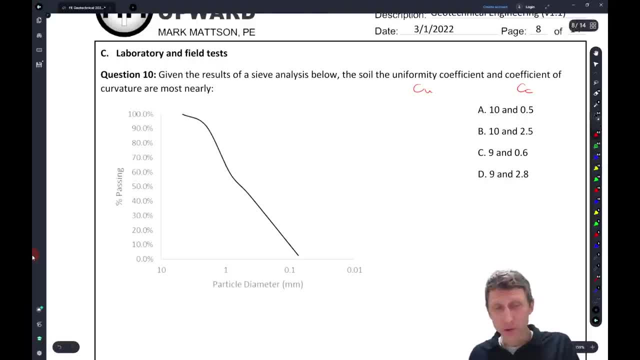 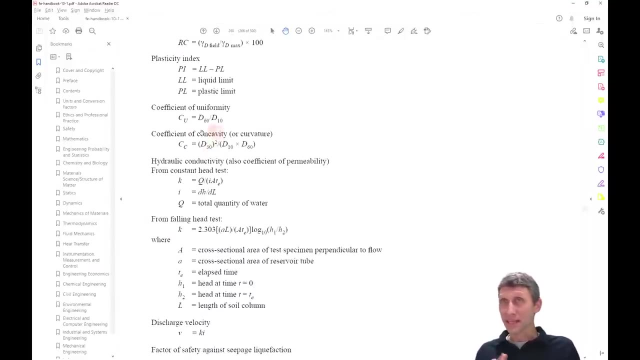 Right. So I think this is going to be on there And, if you can remember, the uniformity coefficient is D60 over D10.. If you don't remember that, these actually show up as well in it in their own spot, So not just in the USCS classification system, they show up here as well. 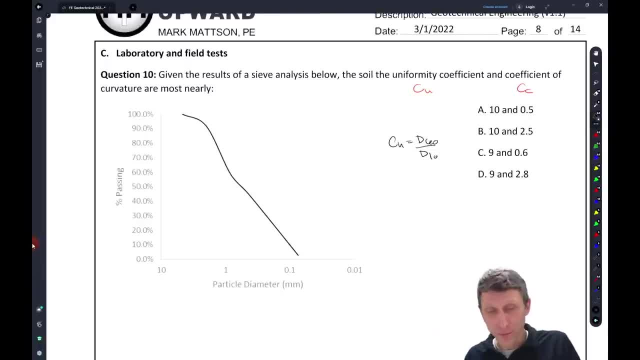 I think they're probably going to be on the test at some point, And I don't know. But this is where I made this problem a little bit more tricky. I don't know, Maybe a little bit, But if we, if we look here actually, let me try to draw that a little bit better here. 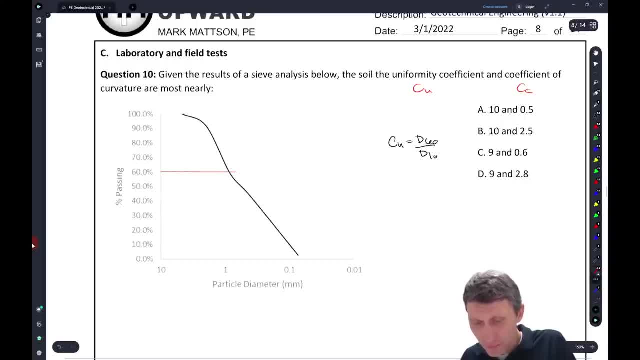 If we look here, we're trying to figure out where these points of intersection are for 30 percent passing, 60 percent passing and 10 percent passing. So some of these are easier. OK, So some of these are easier, Like, for example, if again, if we have these lines here, 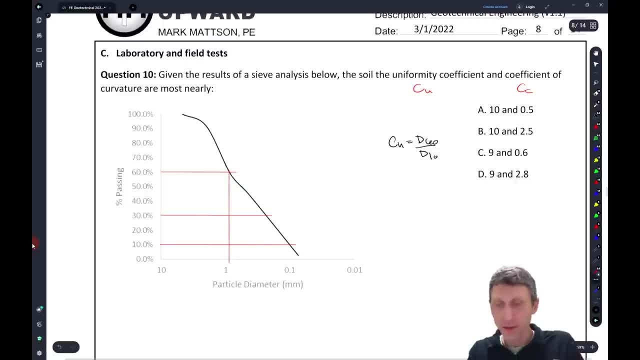 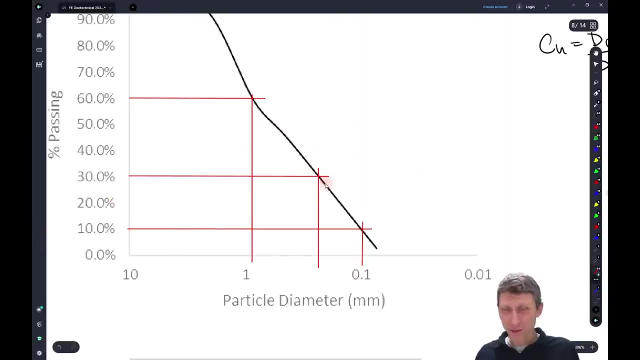 So how did I get that one? I did, OK. This one's a little bit harder, though, And I just want to call this one out a little bit, Because if we zoom in on this quite a bit, I don't know how the lines are coming, if you can see the gray here. 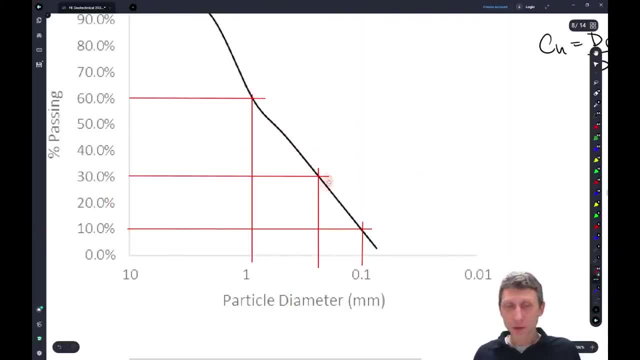 This is a log scale, right. So as we go kind of from one line here to the next, as we go from one line to the next, it looks like we're kind of in the middle, maybe you know, But we're actually. if you think about this, we're closer to this 0.2.. 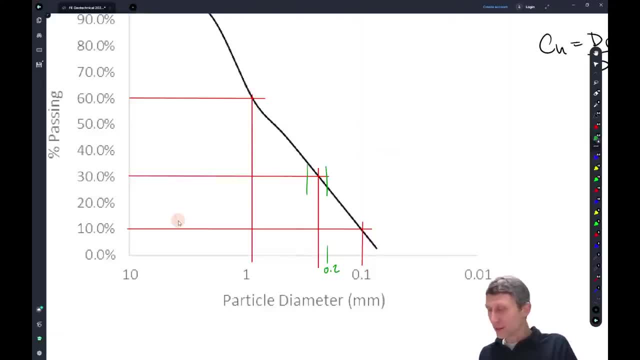 So we have to kind of think about this a little bit, Right? So as we zoom in here, Right, I mean, you have to know how to read this log scale. So point one up to one and we're back to, you know, point nine here. 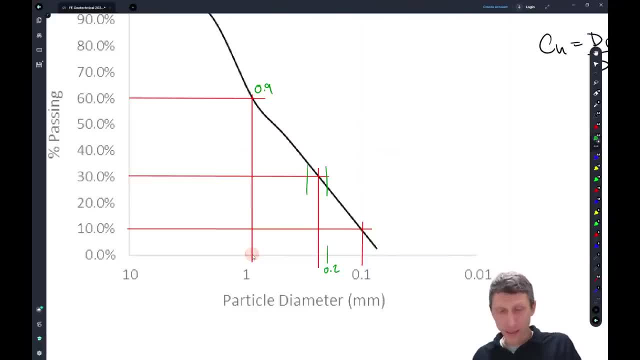 So this might be 0.9.. Not too crazy. This one has a pretty good point of intersection: 0.1.. This one in the middle, Right, I mean you might be tempted to say I don't know, let's, can I move this over? just a hair. 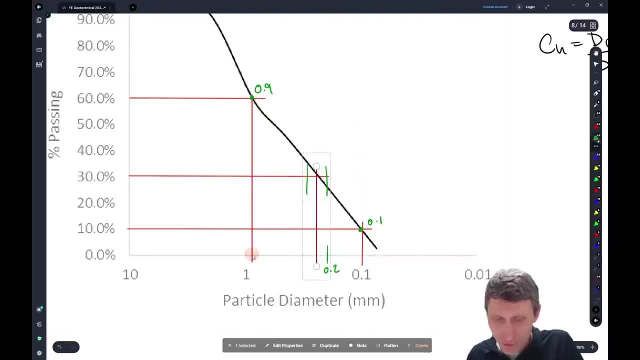 Maybe I can move it over a hair, I don't know, Like, maybe I moved it too much, It's it. I can't get it Perfect. Maybe I had it OK. Where is this right? This is going to be kind of this point. 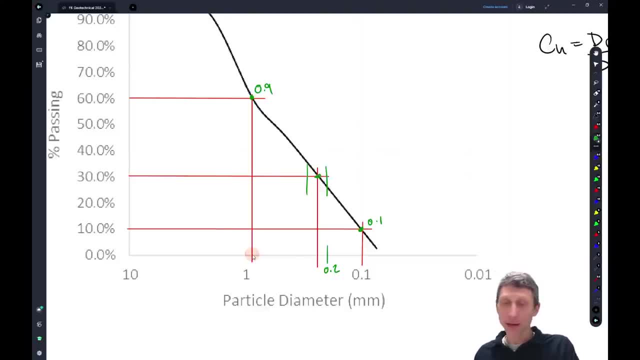 I mean you might be tempted to look, but this is going to be a little bit closer to point to. actually, because of the way the log scale goes, This is going to be about zero point. Let's see 0.23. And it doesn't look like it's you know three tenths of the way. 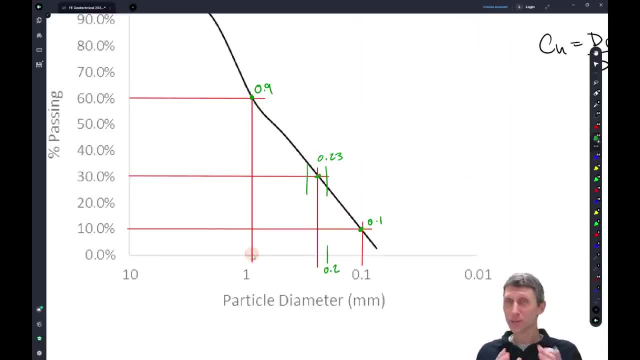 And that's because it's not, But it's actually closer to 0.23.. So when you're interpolating on log scales, just be a little bit careful with linear interpolation, because linear interpolation sometimes doesn't quite cut it. But just just be careful. 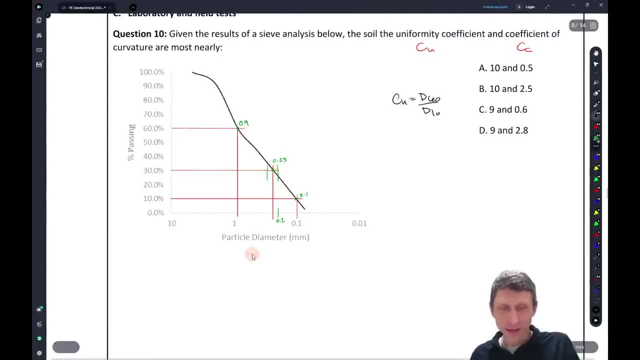 So, so you know, even if you're close, a lot of times there's going to be a range here, but we can find a uniformity coefficient. What's this, You know? 0.9 divided by what's this is D60 and D10: 0.1.. 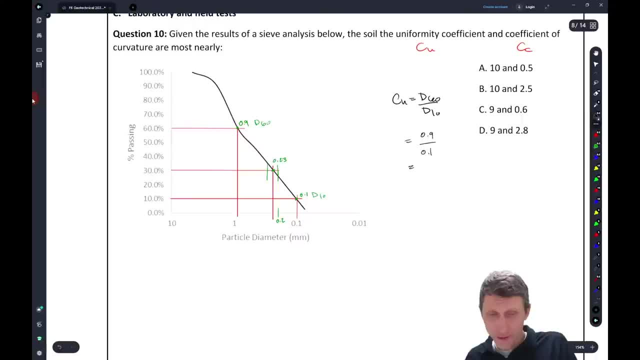 OK, So This is. This is going to be about nine Right, And then CC, that you know. the coefficient curvature is going to be one, D30 squared, divided by D10 times D60.. So, again, this is I. maybe I hit this, this topic, too hard, but I think it's going to be on there. 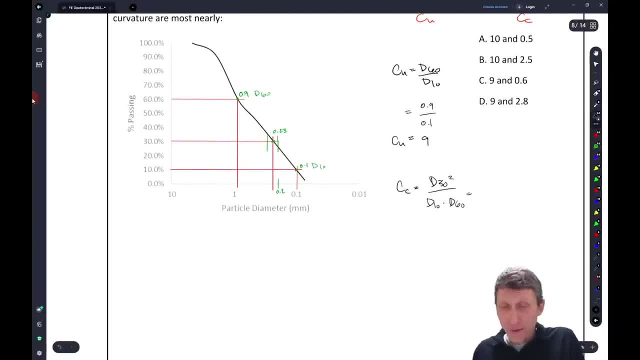 So I think it's probably worth hitting a little bit and talking about. So what do we get? We get like maybe 0.23 squared divided by 0.1 times 0.9.. Right, And I think that gets us pretty close to 0.6.. 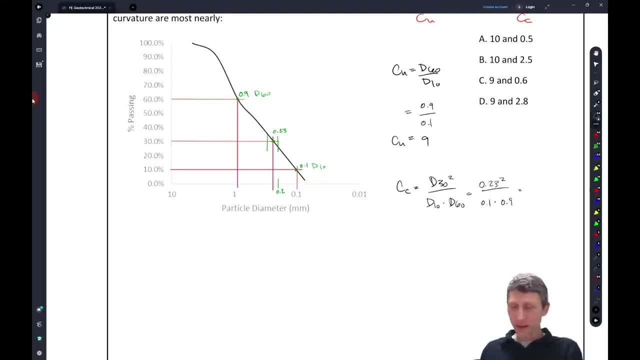 So let me just double check that: 0.23 squared divided by 0.1, divided by 0.9.. Yeah, I get about 0.59, 0.59.. OK, So that means we do have some values here, 9.6.. 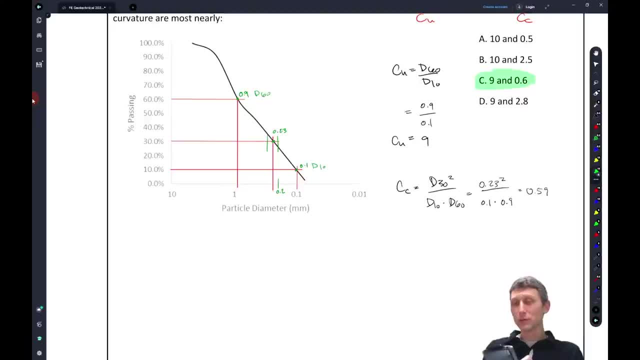 I mean if, if, if in thing is, if I use like 0.25, let's say like I interpolated and use 0.25.. Right, I'm at like 0.7.. So it's not crazy. So like right. So if I, if I used, you know, 0.25 instead, I would get like a CC of maybe like 0.7.. 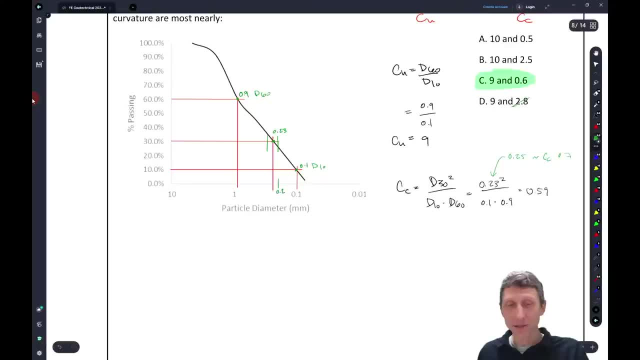 They're not crazy far off, But if there was an answer like 0.9 or 0.7, then then it's it's. it's asking: can you interpolate on a on a on a log scale? And that gets a little bit trickier. 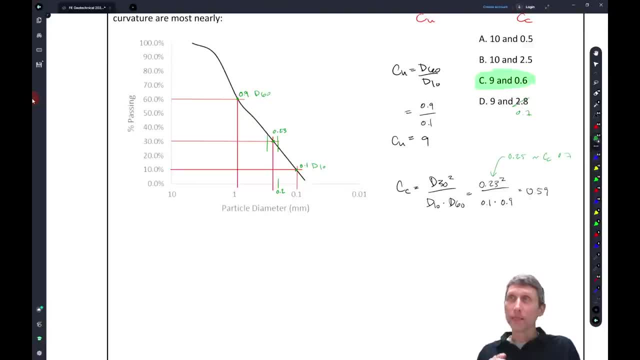 OK, But the thing that we see here, too, is: look what. This is kind of cool. This is like. look at this. Remember we talked about that uniformly graded versus and poorly graded versus well graded. We have this uniformity coefficient here of 9.. 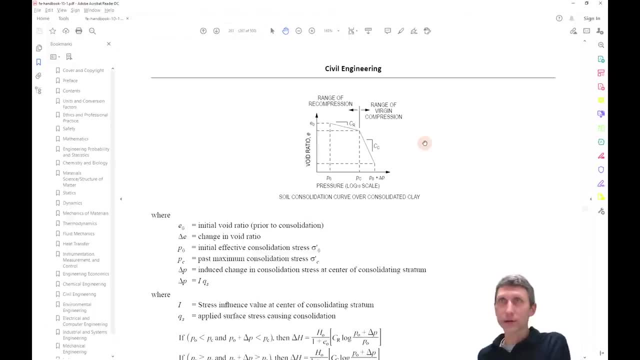 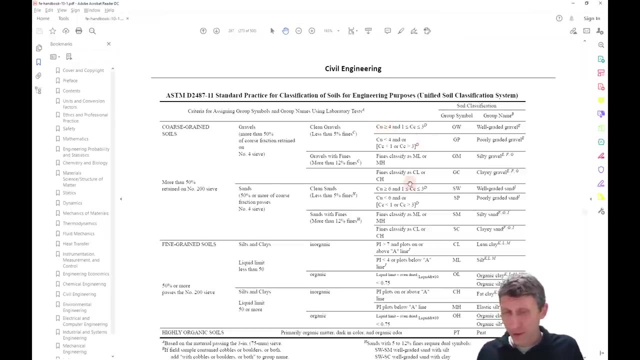 Right, Uniformity coefficient of 9.. Let's just go back to what we learned earlier, or thinking about earlier. Right, If we look at that uniformity coefficient of 9 and come down here, see you greater than 4, greater than 6.. 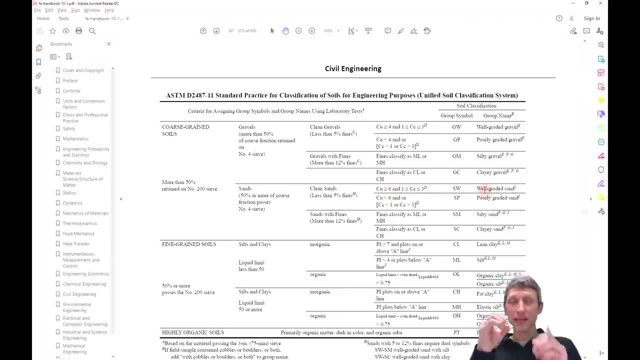 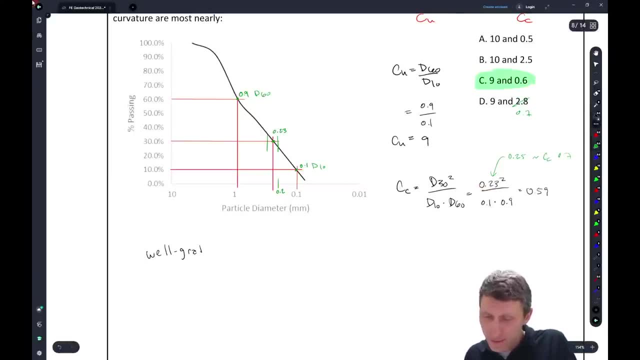 That's going to put us into that well graded Right It has. It's like, when I think of well graded, I think of like what? What do I think of? well graded is like this, where you have, you know, various size particles that all kind of like fill in the voids. 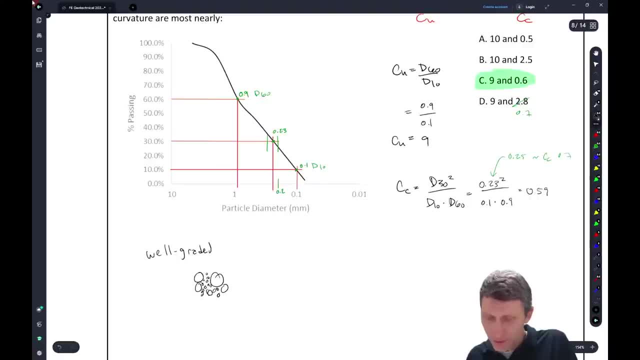 Right. So like you get these little particles, the big particles, it's well graded and they all kind of fill in, versus the poorly graded Right Or the uniformly graded, where basically you get a whole bunch of particles that are all what? all the same size. 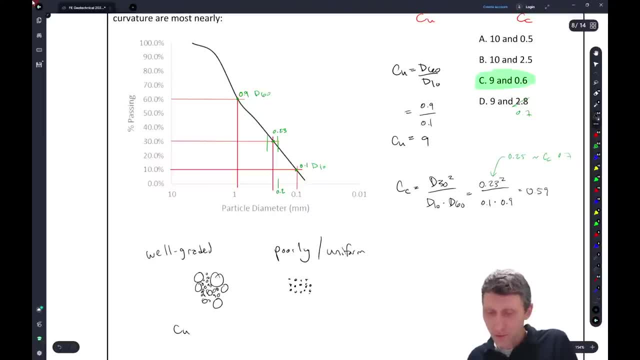 Right, So this is, you know, the CU of greater than, let's say, 4 to 6.. And here is the CU like less than 4.. Right, So this is that kind of gives you an idea as well where it's like. this is like you're. 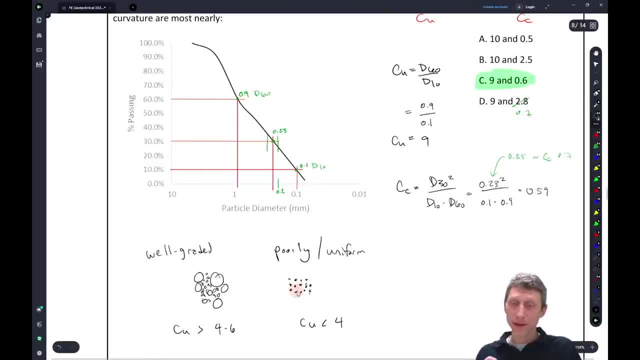 you know, you might get your beach sand versus your your crusher run, Right? They're just a couple of things like that, So let's keep going, All right. So we got question 10 and let's keep going. OK, So question 11.. 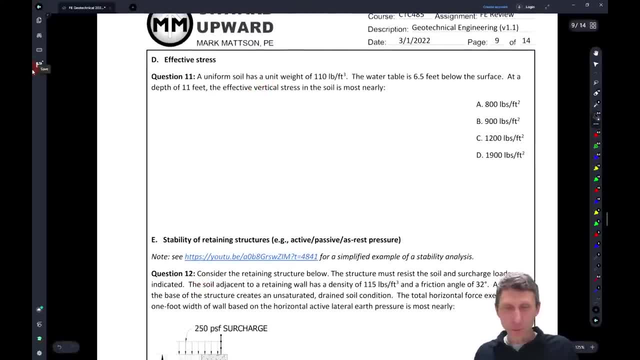 Uniform soil is a unit weight of 110 pounds per cubic foot. The water table six feet below, or six and a half feet below the surface. So we know that there's a surface here, There's a water table, That's, that's what. that's six and a half feet down. 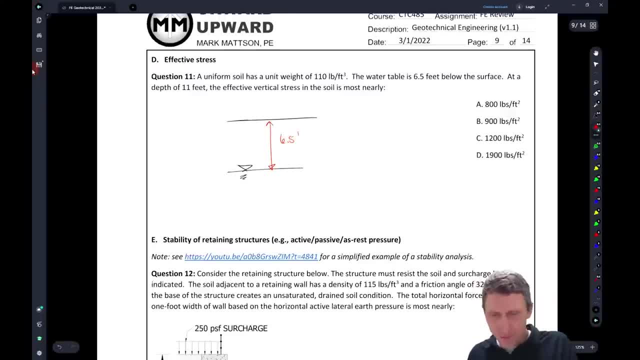 Six point five feet, OK, At a depth of 11 feet. So down here, maybe at 11 feet Right. So we're down at 11 feet. What's the effective vertical stress? OK, The effective vertical stress In the soil. 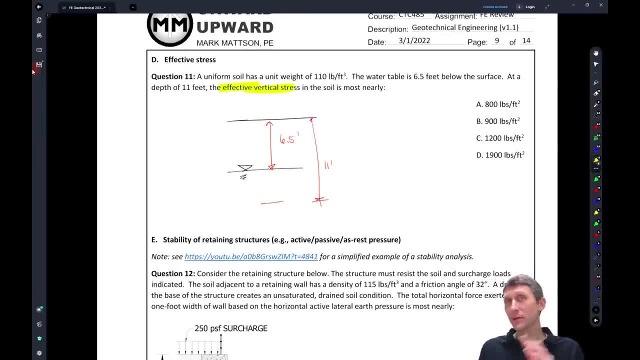 Well, this is where I think this, this type of question, could be on there too. So so there's a topic: effective stress. But what's the idea that's going on here? Let's come back here for a second to our reference handbook, And what we see is we have vertical stress profiles. 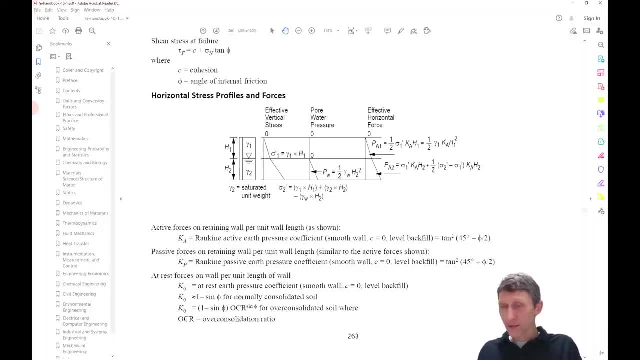 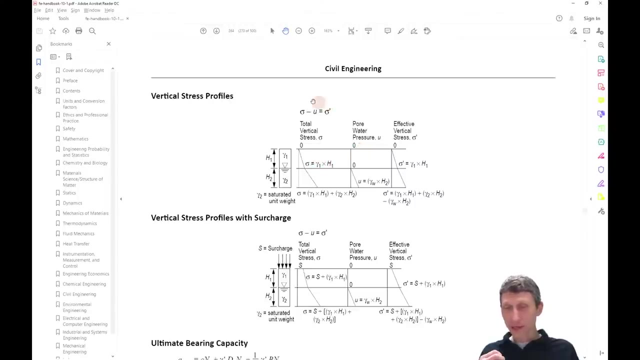 We also have horizontal stress profiles where we deal with, you know, different layers of soil and water And we have different effective stresses versus, you know, vertical, poor pressure And horizontal forces. here we're looking at vertical stress profiles And if we look at this, if we think of the total vertical stress right, 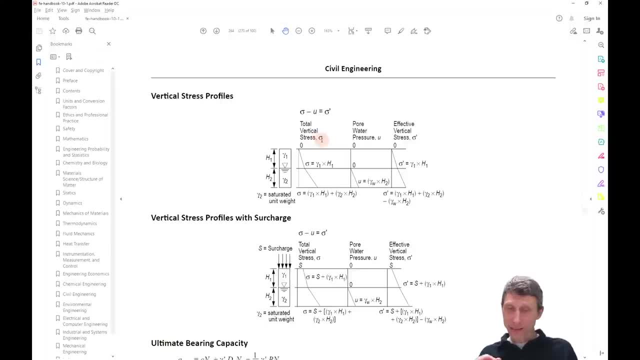 The total vertical stress it has to basically accounts for everything of the soil Plus the water weight. OK, So plus the water weight. So so in basically, what's kind of happening is the soil takes part of the load, The water takes part of the load. 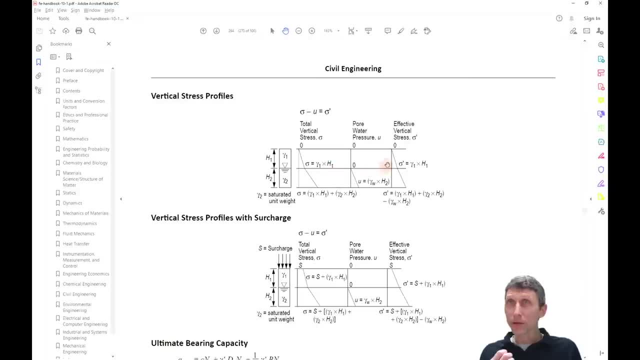 And that's the total vertical stress, because you have both going on. But what we're looking for here is the effective vertical stress, Right? What we're looking for, kind of, is going to subtract out the component of the water. So the effective vertical stress is sigma prime is going to take out that component of the water. 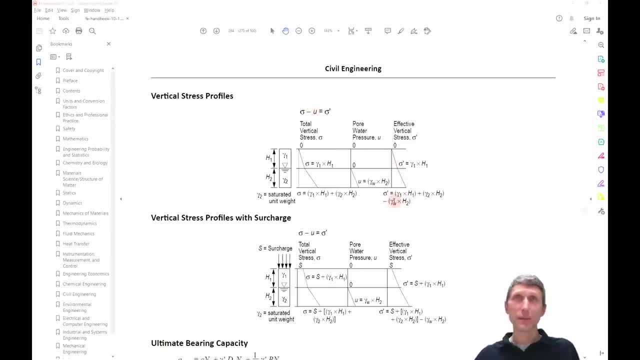 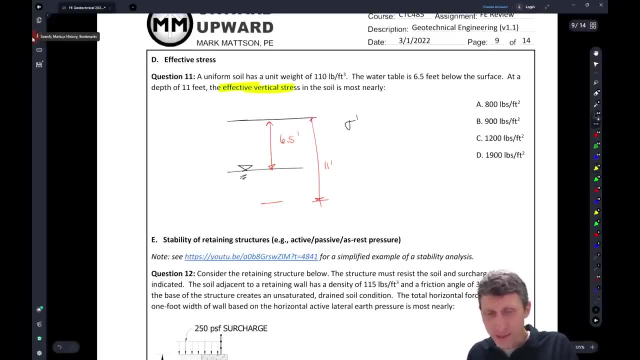 So this is one equation. I kind of think of it similarly. But basically the equation that we're looking for here is going to say: sigma prime, This is our effective vertical stress is going to equal. Let's just let's go look at it, make sure we're doing it right. 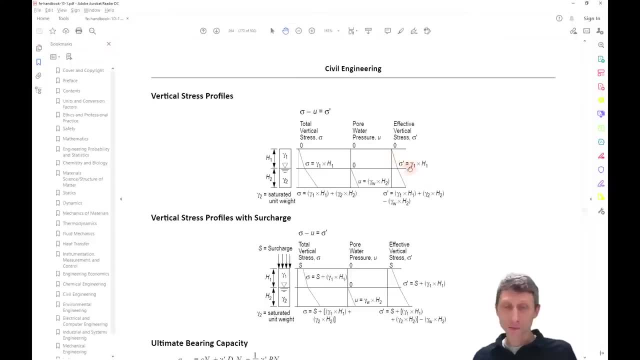 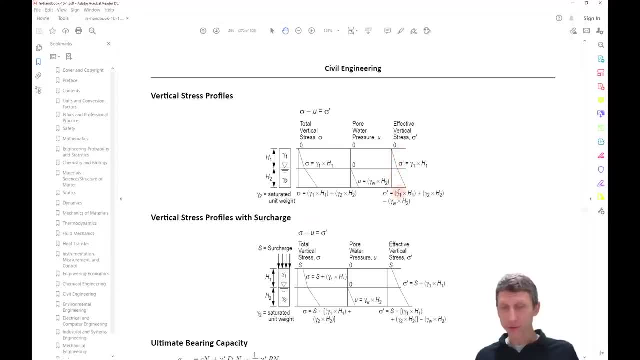 So it's not like gamma 1 and gamma 2.. We have one gamma for the whole thing It's. you know, here we could have gamma 1 and gamma 2.. For us, we only have gamma 1.. OK, But what we're going to have to do is we're going to subtract out the water times that 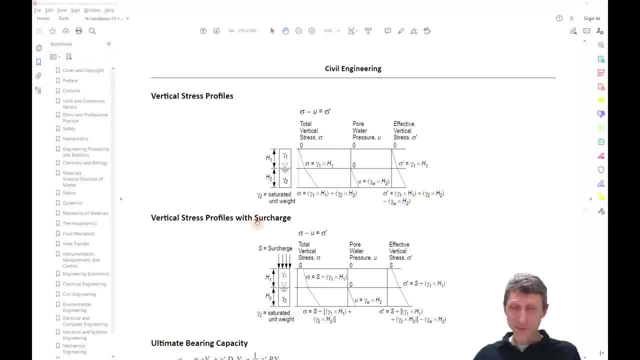 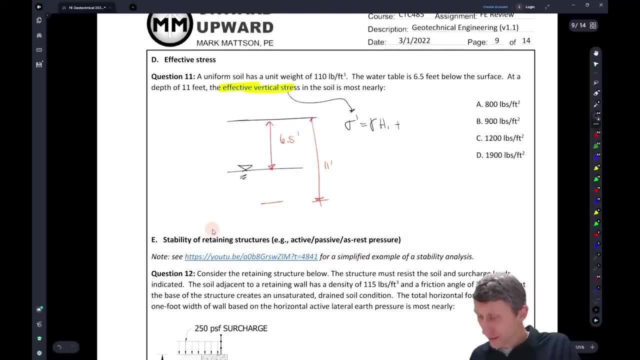 height. So you can see, here there's an H2 and an H2.. Typically, what I'll do here is I'll say this is kind of like gamma times H1, you know, plus gamma, minus gamma, water times H2.. OK, So that's going to be our effective stress. 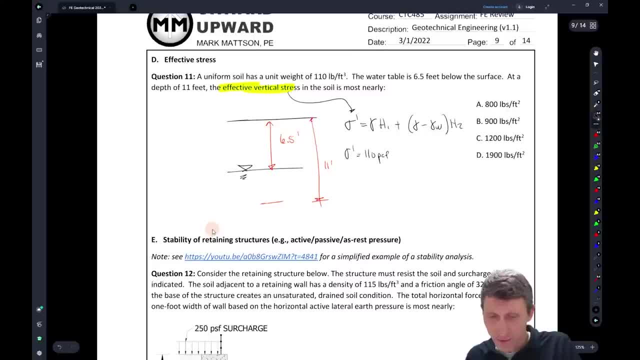 Sigma prime is going to be our 110 PCF, times what our six and a half feet. And if again this is sort of sort of like those phase relations, Right 11, six and a half plus what gives us 11. Well, I don't trust myself tonight. 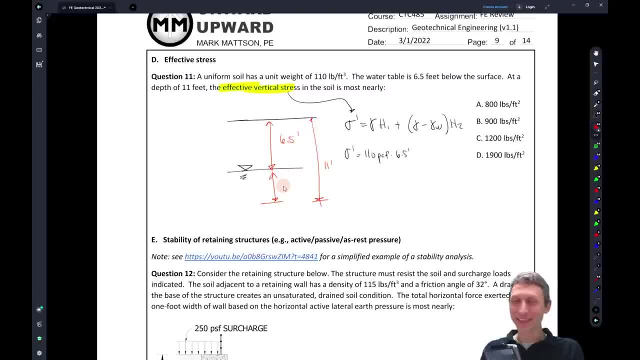 11 minus four point six point five. I'm thinking it's four point five. Yeah, So it's four point five. OK, So we got four point five here, So that's our H2.. All right, So what are we going to do? 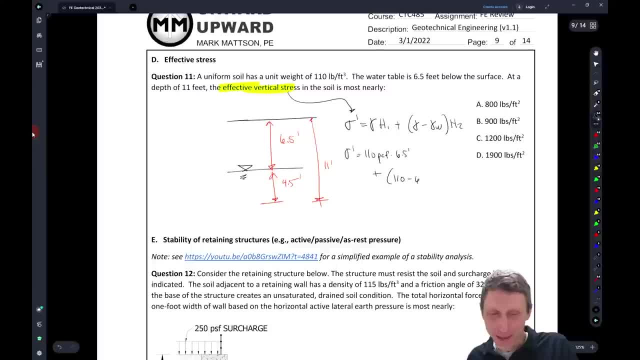 Then we're going to add in this this hundred and ten, But we're going to subtract off the weight of water, and the weight of water is sixty two point four pounds per cubic foot And everything's in feet times H2, which is going to be four point five feet. 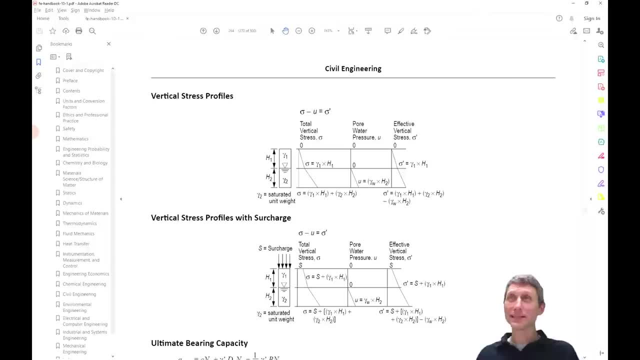 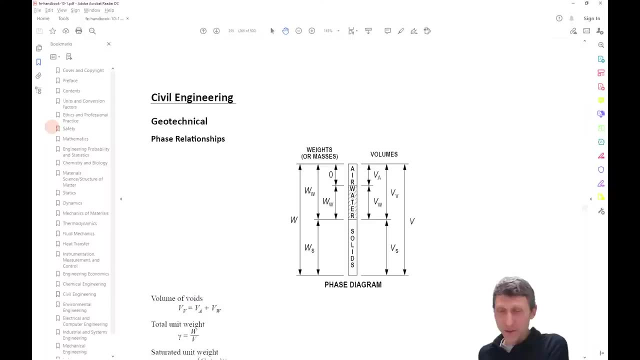 And if you don't know, If you don't know, sixty two, point four, The good news is that one does show up. It doesn't show up right here, but if you remember and you come back a little bit Right, Remember when we were looking at our phase diagrams that unit weight of water was was. 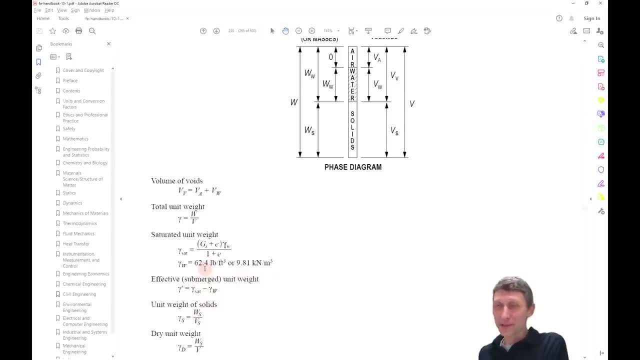 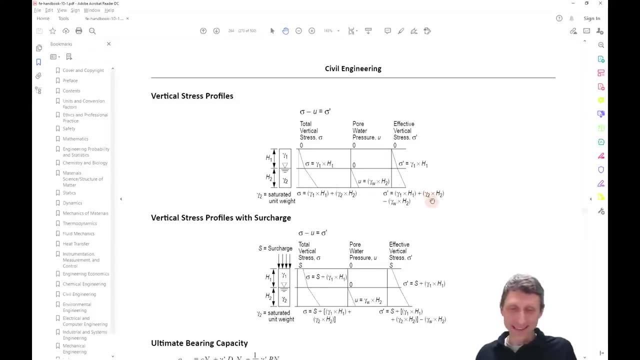 right here. So again, getting familiar with the reference handbook is going to help you remember in some of those, those components is going to help you as well. But yeah, this is where I just kind of factored this, this H2, out to make the computation a. 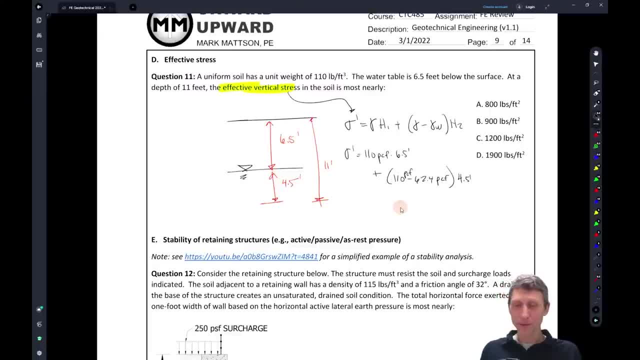 little bit easier. But what do we get? one hundred ten times six point five, plus, in parentheses, one ten minus the sixty two point four times four point five, and I got like nine thirty. So Sigma Prime equals nine thirty pounds per cubic foot. OK, 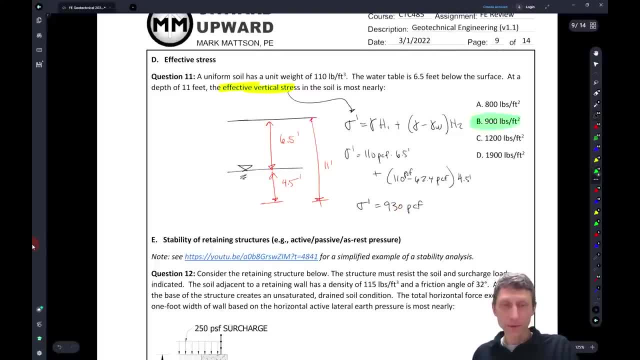 Close enough to call it nine hundred. in a perfect world I probably would have made that nine thirty, but I didn't actually think I had different numbers I think I might have had. when I first did this I had ten in my spreadsheet. I can't remember what I had. 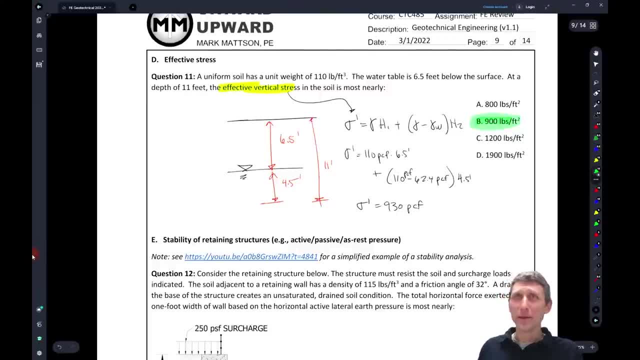 I was doing this on a spreadsheet and I had another number, so it was closer to nine hundred, but nine thirty works. OK, I'm good with it. You know that I hope so, OK, So let's keep going. We got a few more of it. 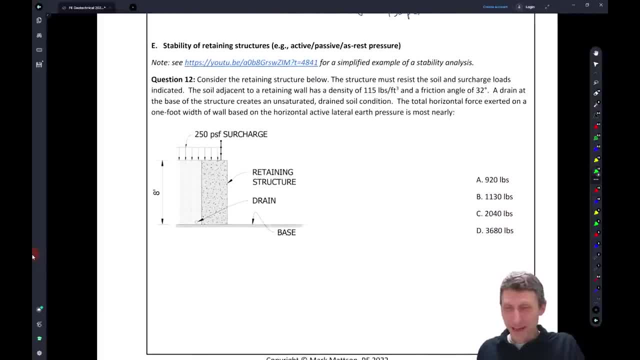 A few more questions to answer here, but hopefully they all make sense. Stability of retaining structures. So in the structural design piece of this I kind of did a stability analysis so I put a link to that up here and that actually takes you right to that problem. 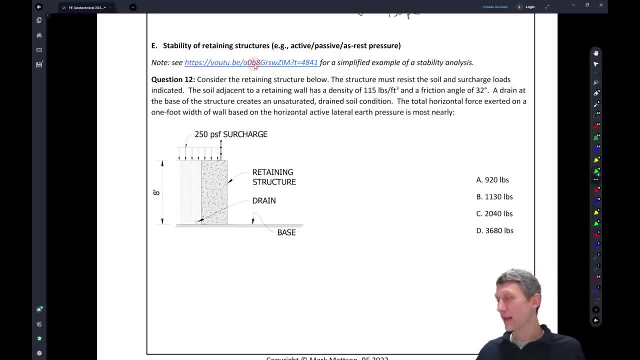 So if you want to see that problem, You can go to a little bit more of a stability analysis In this one. what I did is I just said kind of the difference with soil. What's the difference with soil? In the last one I did a dam section, just use water. 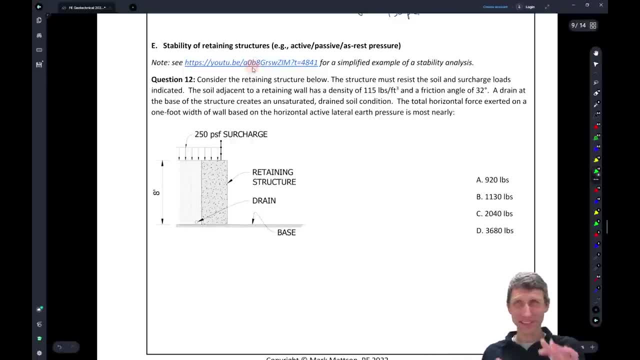 Here we have a soil and I took the water out of it, So it's, you know, maybe we can have something in between. and another problem where you have a- you know, partially drained, partially drained, you know- wall or something, But here we have a retaining structure. 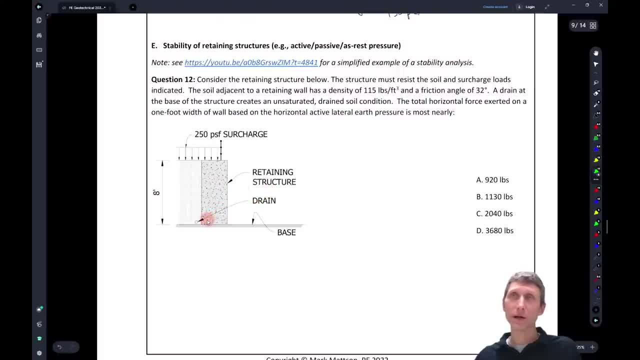 It's a big, you know big- hunky concrete, right eight feet tall, and behind the concrete we put a drain in. Why do we put a drain in? We put a drain in because we don't like that water behind the wall. We want to drain it to get the water away so that the wall doesn't have to hold up all. 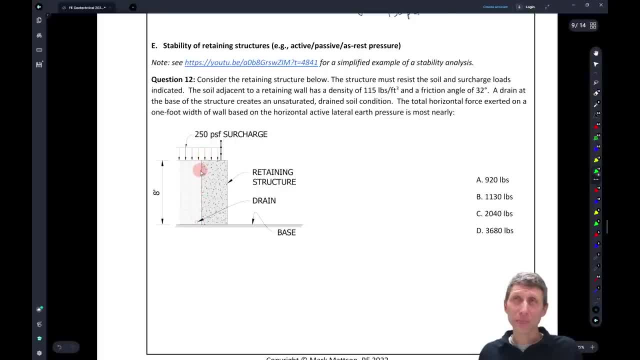 that water Right. So a lot of times you'll put in a forest layer a fill like a stone with a drain at the bottom to try to get the water away quickly. OK, So what we have is a retaining structure, and the structure must resist soil and surcharge. 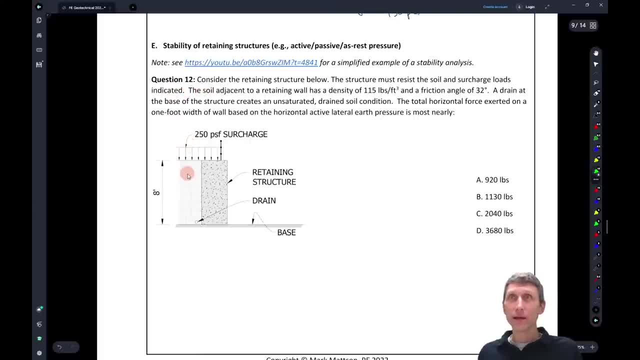 loads indicated. So we have a surcharge and a soil here And, oh, I think I made a mistake And I'll probably need to put an update here. I don't know if any of you guys did this ahead of time, but maybe you can call me out and 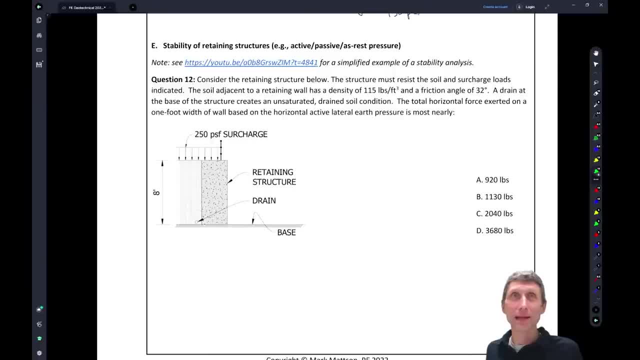 tell me if I did something wrong here, But I think I think I forgot the surcharge when I did my hand calcs. We'll find out here. I think I did, though, So so we'll add that in. But what we have here is a soil and a surcharge, and we have to come up with the total horizontal. 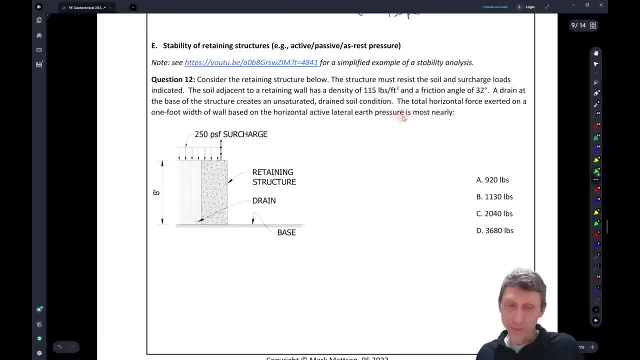 force exerted on water. So that's the one foot wall, based on the horizontal active lateral earth pressure only. So not the greatest question, because I'm telling you to just do the just the lateral active earth pressure. but then I gave you a surcharge. 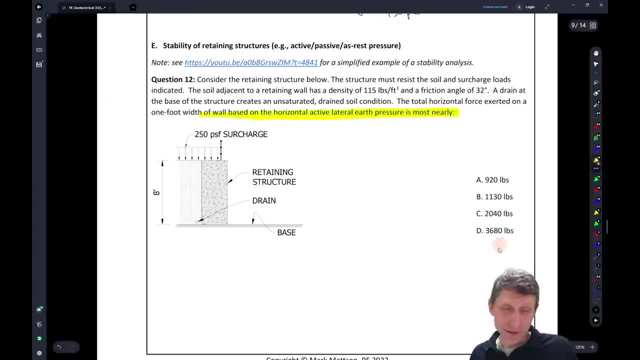 So, honestly, I made a mistake here. The answer does not include this surcharge. So maybe what I'll do is I'll just cross the surcharge out, because the answer does not include that surcharge And when I ask you this question I'm just asking for the active lateral earth pressure. 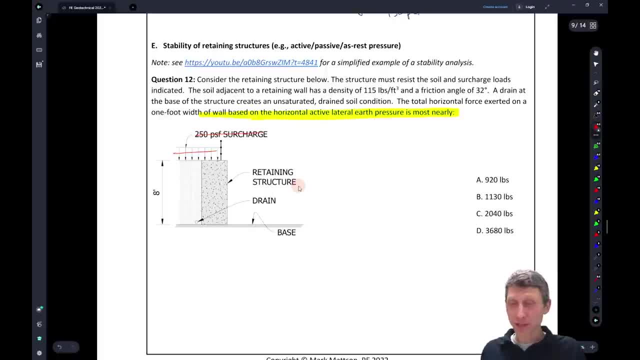 on the wall. OK, I'll show you what to do if you have a surcharge in there, But let's just start with this for now, OK. So let's modify the question and keep going. OK, So what we have here is 115 pounds per cubic foot. 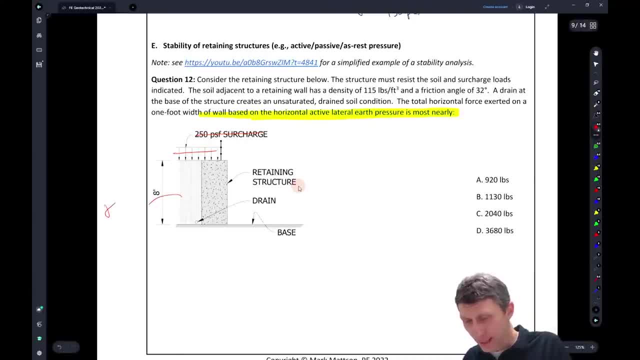 So this soil has a gamma of 115 PCF. OK, And what else do we know? We know it has a friction angle. This here is going to be friction angle of 32 degrees. So typically in soil friction angle is known as phi. 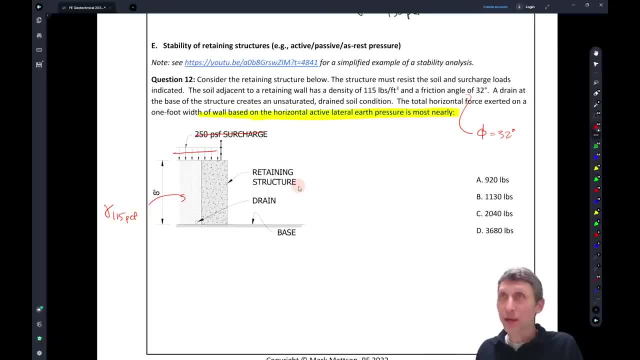 So 32 degrees? OK, What else? A drain of one foot, You know. So we have a drain at the bottom of the structure. What's the horizontal force? Well, if we think of this again, what we're going to think of is we have this structure. 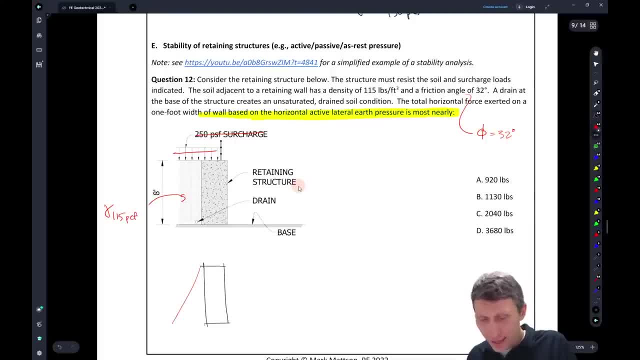 here And this soil is going to act just like a liquid sort of- Not exactly, But what we're going to do is we're going to use a coefficient to make it act like a liquid, So we're going to get a pressure. 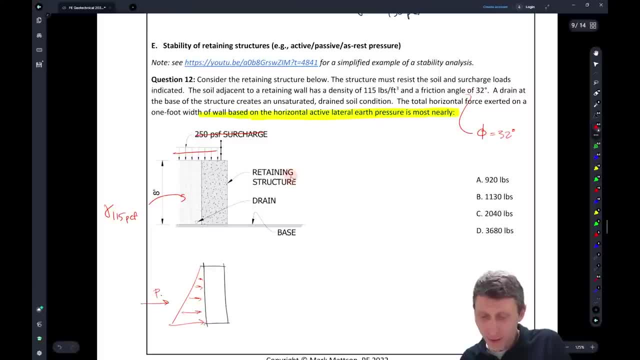 We're going to get a pressure, this P, you know, active one or whatever. This is going to be a pressure. It's going to be a horizontal earth pressure And if this was just water, we do what we take one half gamma H squared. 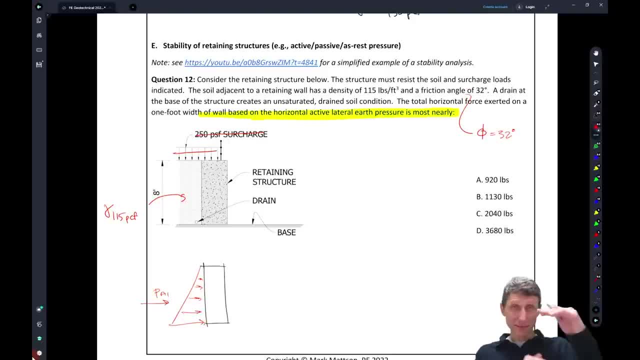 Right, You remember that formula: one half times the unit weight of water, times the height squared, to get us, essentially, the area of this triangle. But it's not. It's not water. What is it? It's a soil. So what do we do? 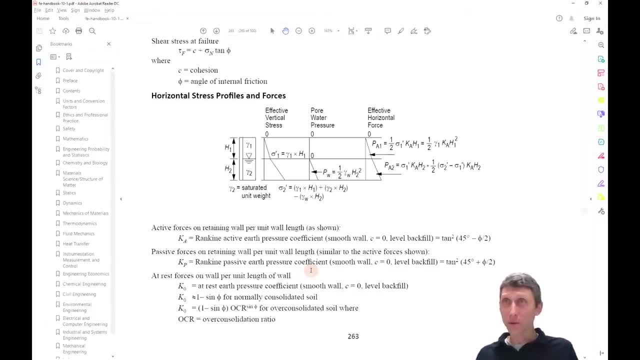 Well, because it's a soil, we have to come back here and we say, OK, well, what do we do with this soil? What do we do with this horizontal stress? So if we had a water table, it would get more complicated, But all that we have here is we don't have a water table. 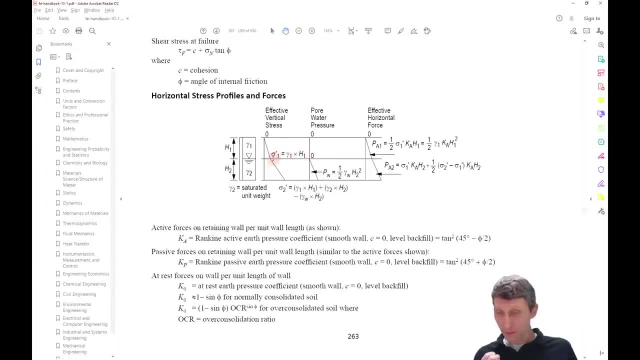 We have a gamma and an H. Right, We have this. We have a pressure which turns into a horizontal force. OK, That horizontal force is going to take a look like this: So P a one active pressure is going to be one half sigma. 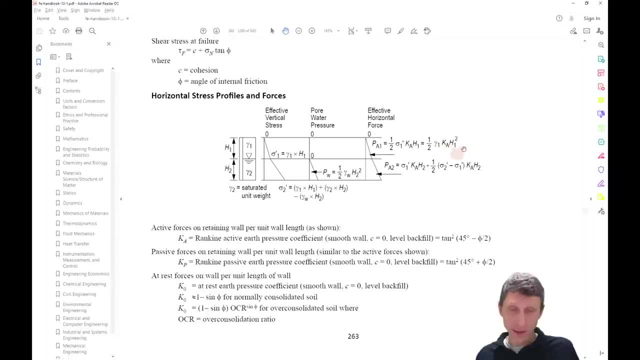 Sigma prime K H one, one half. In other words, what we're going to get here is one half gamma, one K a, H, one squared. So let's go there. And what's the difference between this one and just the water version? We get this extra K a. 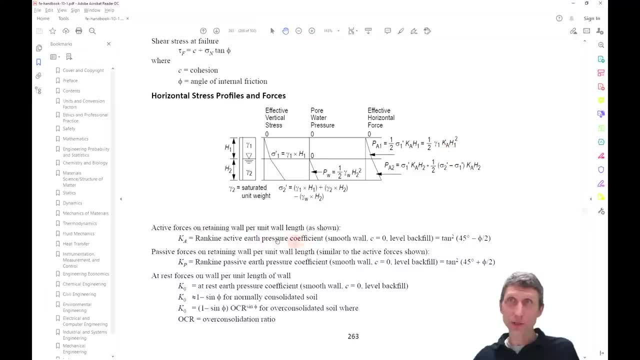 Right, What's K? a? It's a, it's an active earth pressure coefficient. So this basically says: OK, well, if it was water, K would be one, Everything would be. everything would be pushing up against the wall. but it's not water, it's. 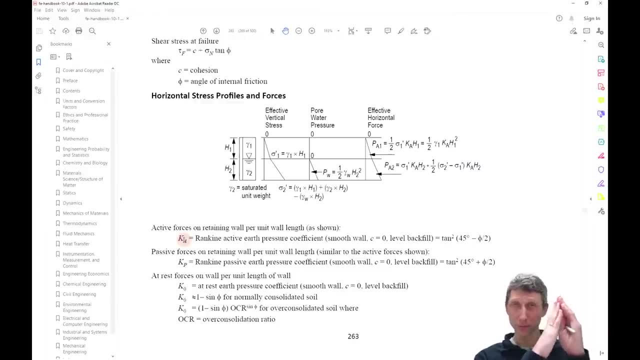 a soil. So we're going to reduce that pressure and we're going to say, well, a certain portion of it's going to act. That's going to be what the active earth pressure coefficient does. It says, OK, well, how much of that acts horizontally? 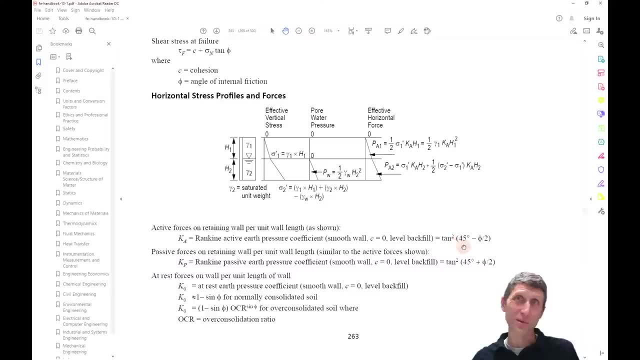 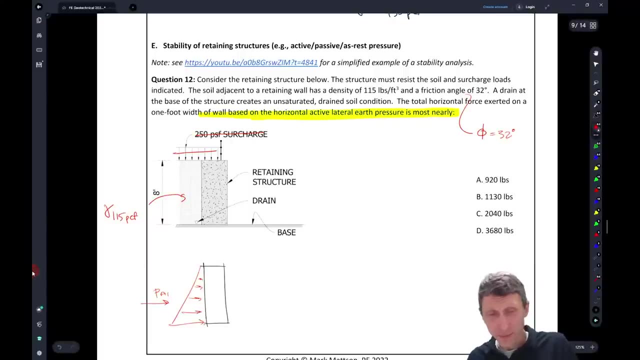 And that's what we're going to get here. So K a is going to equal tan squared, you know, forty five minus you know tan squared of forty five minus V over two. So that's going to give us our K a. But let me just write this down first. 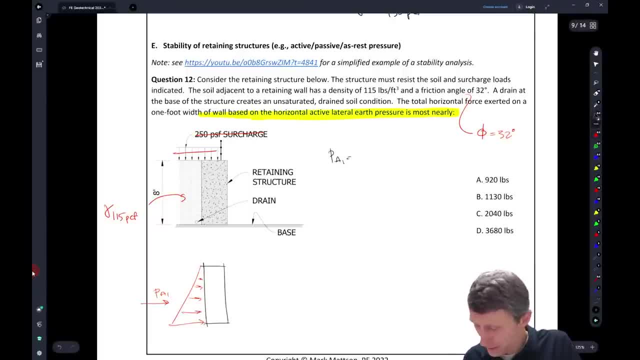 So the P a one is equal to one half K a times gamma H one squared. But before we can solve that We have to solve for K a and K a I. it's funny, I don't like this formula. tan squared forty five minus V over two. 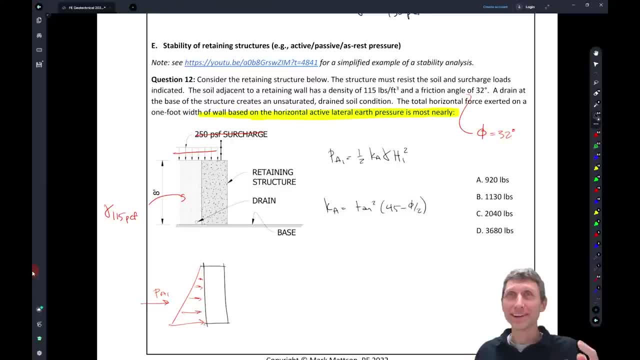 When I was doing real engineering before teaching engineering, we would always use K a equals one minus sine phi over one plus sine phi. Maybe the next math review session I do I'll we'll have to say see if those are equivalent. They should be OK. 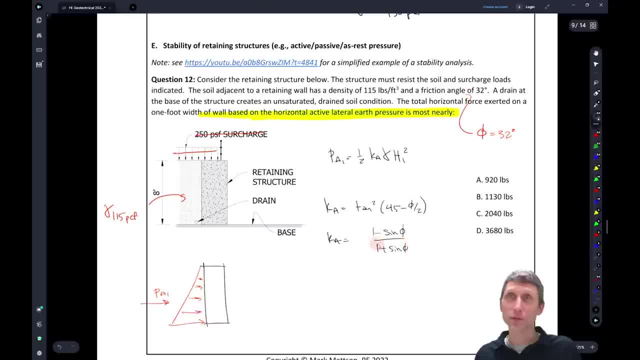 But I don't know, maybe in your soils class this is what you learned, as opposed to this. Either way, you plug in and you should get a value down here of K. a equals Y. I'll do this- the first one, because that's the one in the reference manual, but forty. 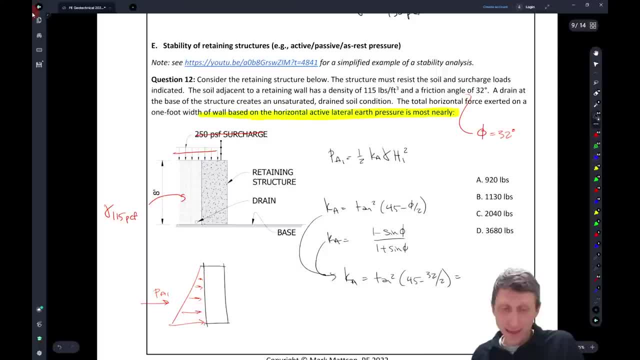 five minus thirty two over two And I think that works out to about point three. oh, seven. But yeah, Do you know how to enter the tan squared? you just do the tangent and then square it. OK, Forty five minus thirty two over two. 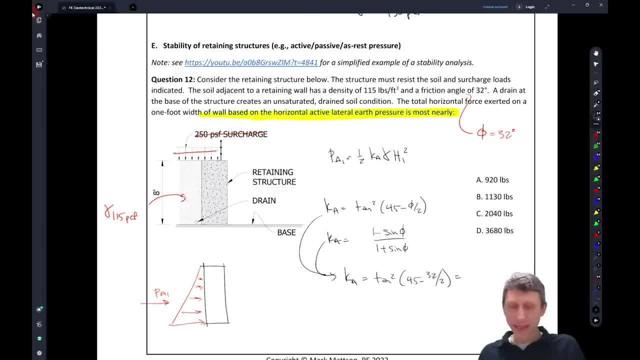 OK, And then I hit the square button And I get zero point three, zero seven, And if I do, if I do the one minus sine phi, one minus sine of thirty two Over one plus the sine Of thirty two, You get the same exact value, so that both of them work. 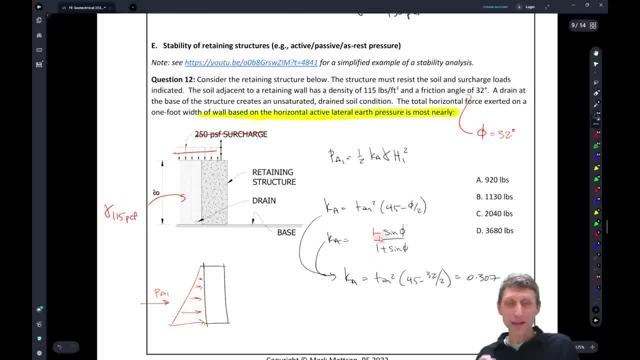 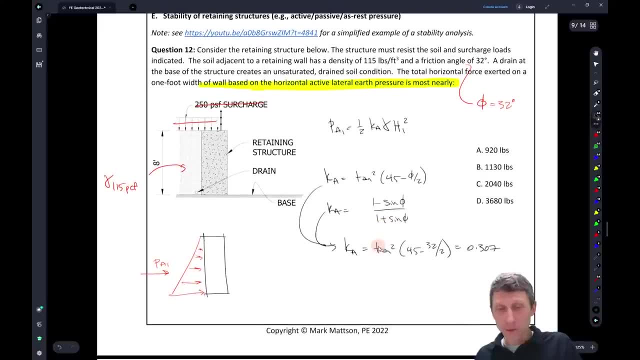 It's just I put. I put them up there because This is the one I used to always use in practice. I don't know, Maybe, maybe this is the one you were taught in your geotech class. OK, But once we have that value. 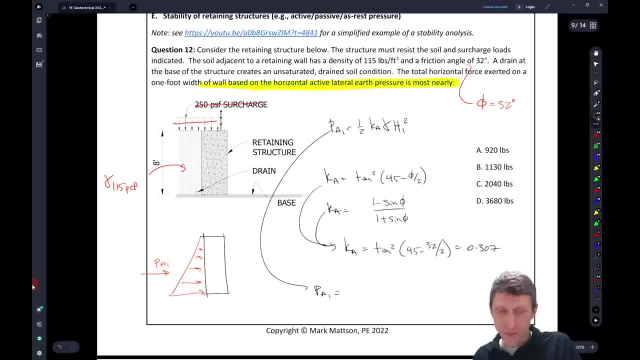 Right now we can come down and we can say this active earth pressure is going to be one half- I'm zero point three- zero seven Times our gamma, which is one hundred fifteen pounds per cubic foot. Times our height, which is eight feet Squared. 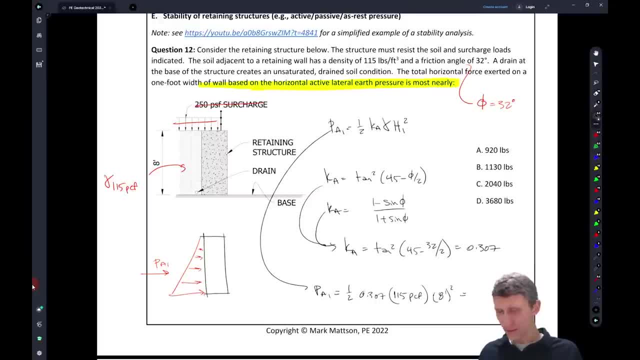 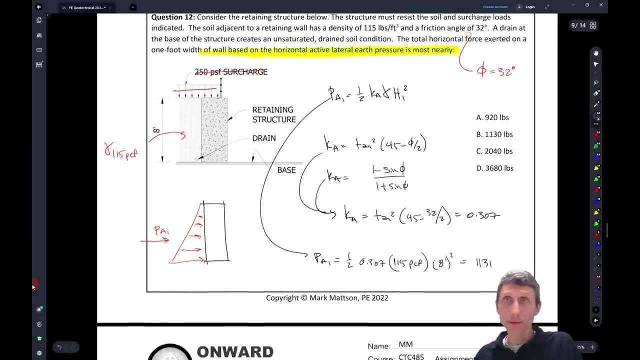 And I think We're going to get that eleven thirty value. Does that sound right? The point five times point three, oh, seven Times one, fifteen times eight squared. Yeah, I got about eleven thirty one. OK Pounds, OK, Eleven thirty one pounds. 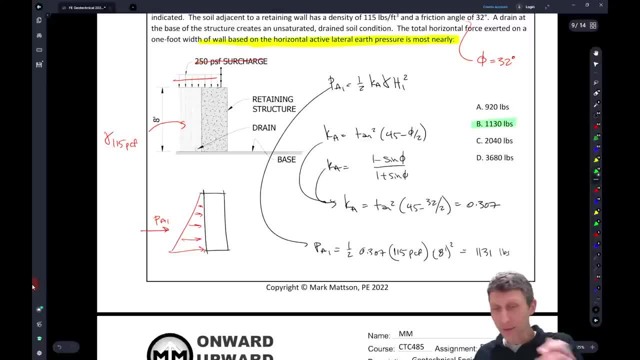 OK, So let's, let's go with that for now. Eleven thirty. And somebody's saying: but what about that two hundred fifty pounds per square foot surcharge? because I know When I get to my test I'm going to get something going on here where I've got a surcharge. 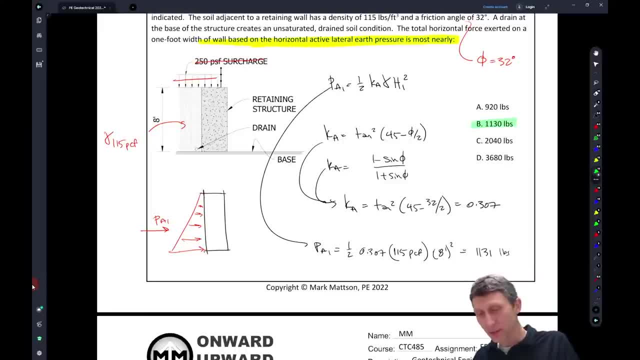 What happens with that surcharge? If we have a surcharge, Let me just take this for a second and move it up, And what I'm going to do is I'm going to actually do. That's not what I meant to do. 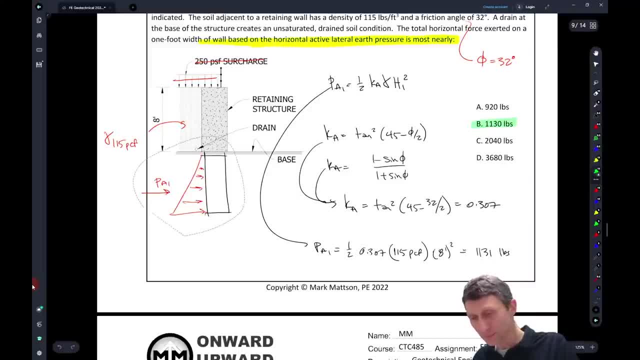 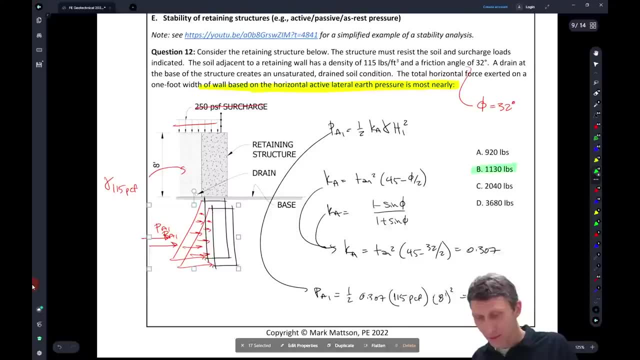 Let me try it one more time here. So if I take all this, If we had a surcharge, I'm going to duplicate it. I'm going to move this Down. if I can, Can I grab it? Let me try to grab it here. 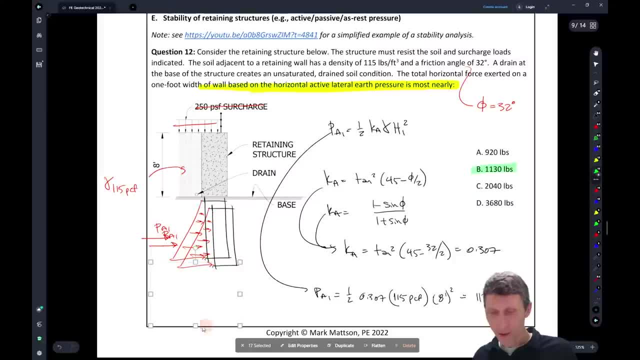 It's not grabbing. There it goes. I got it OK. So if I move that down the surcharge, basically what that's going to do here is it's going to take this force here And can I get it over? And no, it's not going to work. 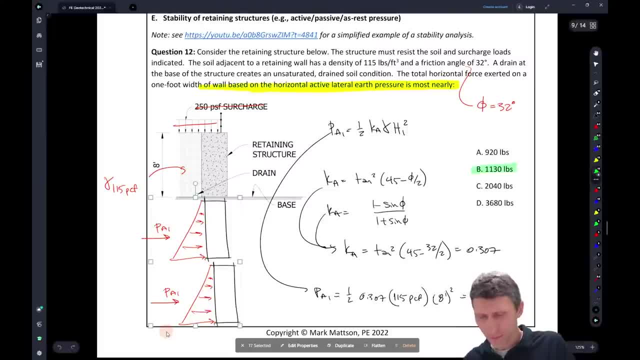 It's going to take. Let me see if I can. Let me try one more time here. It's going to take all of this Force. I'm not doing it. Let me just Delete it and start over here. It's going to take that force and move it over. 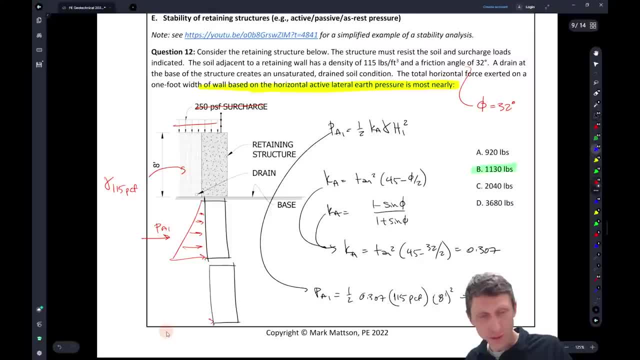 OK. So essentially, what we're going to do is we're going to take that surcharge and let me write the surcharge in here, So we're going to have a kind of a surcharge in here, OK, And then we're going to have the same active earth pressure here. 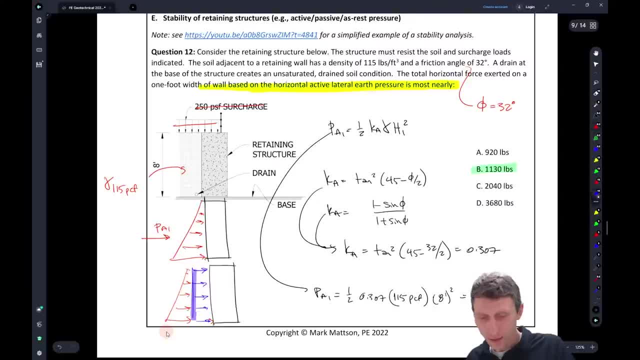 So if we had the surcharge Right, This would be kind of this: the surcharge load. OK, So I can, I'll update. OK, You know the question. So if you're looking at this later and thinking like, but my question doesn't have a surcharge, 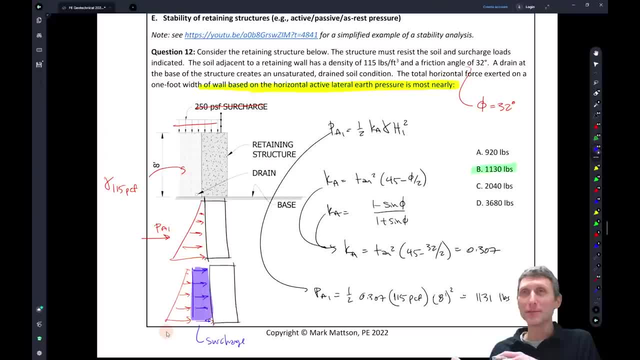 that's because I deleted it between the time you're watching the video and what I just what I just went through, because I, when I saw this beforehand, I you know the answers- didn't have a surcharge in there, So let's just go with that. 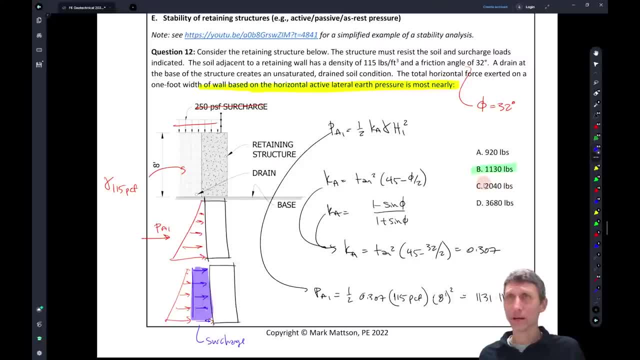 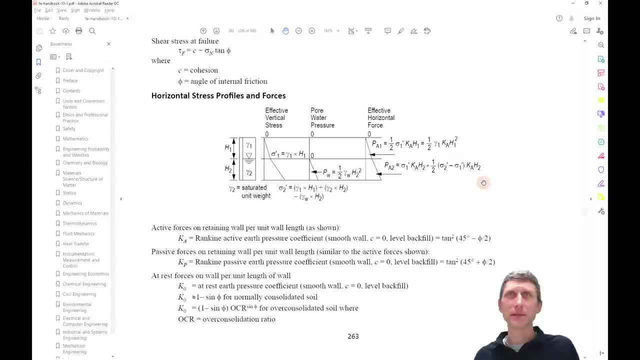 OK, Is that OK? OK, But yeah, I mean the surcharge would increase that load obviously. And I'm trying to think, if that's in the reference handbook, Let's come back here and look. I don't remember seeing it in here. but oh yeah, here's the surcharge. 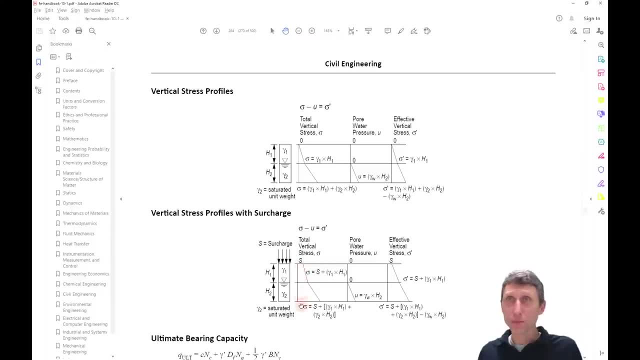 Right. See, look at that, The surcharge. What does that do? It just moves this diagram Right. It moves this diagram to the right, Right. So it adds that extra, that extra surcharge pressure, Right, That extra surcharge pressure that we have to deal with, which is going to impact the 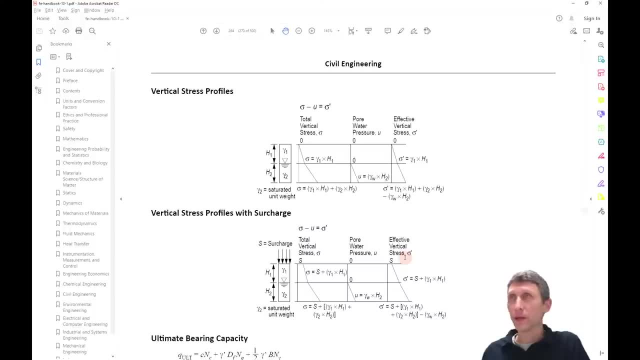 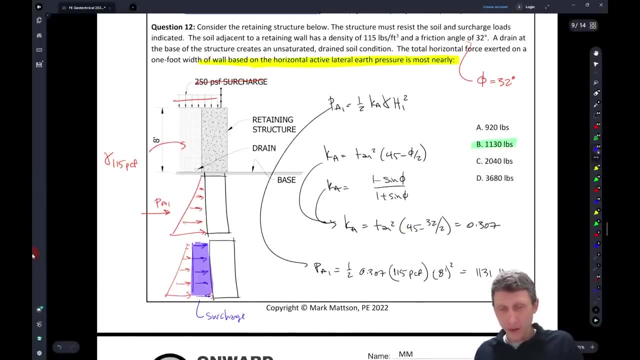 horizontal horizontal pressure. OK, So, So, let's keep going. OK, Let's keep going, And let's keep going. So where do we go next? Oh, shear strength. So this is shear strength, and this kind of gets into that point. 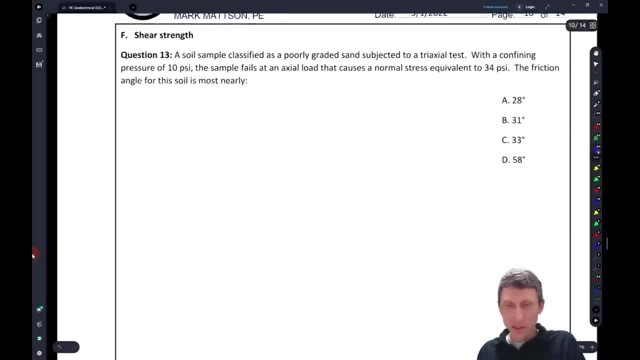 There's a couple different ways of looking at shear strength. When I took my geotech class a while ago- actually, I was looking through notes for my geotech class Just looking to see you know, do I think what's what's fundamental? What I think is fundamental? 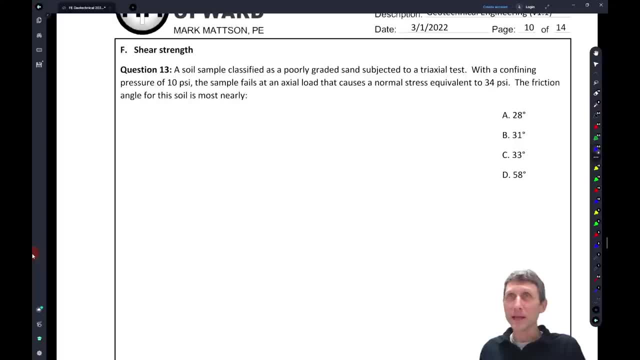 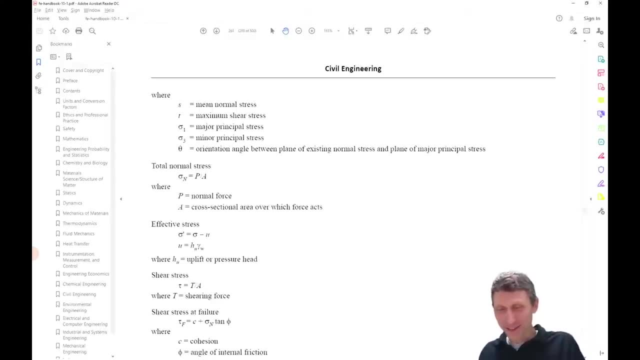 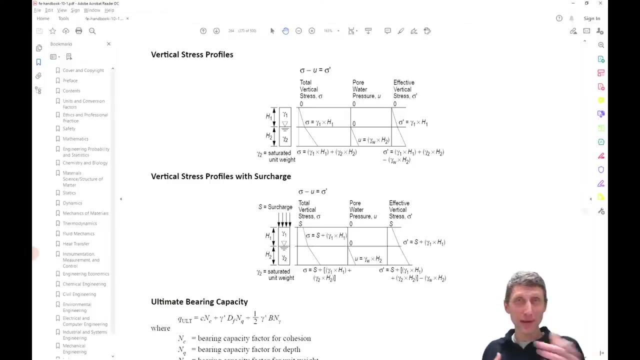 Is that the same thing that was fundamental when I took a geotech class? What I think is fundamental is that the same thing that was fundamental when I took a geotech class, And actually a lot of it is. But let's come back here for a second. 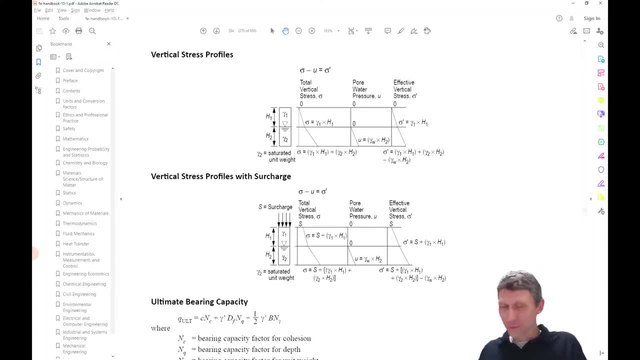 And we have a few other things actually retaining walls- We'll come back to those in a second- They kind of, They kind of, They kind of look here. So, Oh, good question. So, visual representation of passive earth pressure underground, laterally to resist. 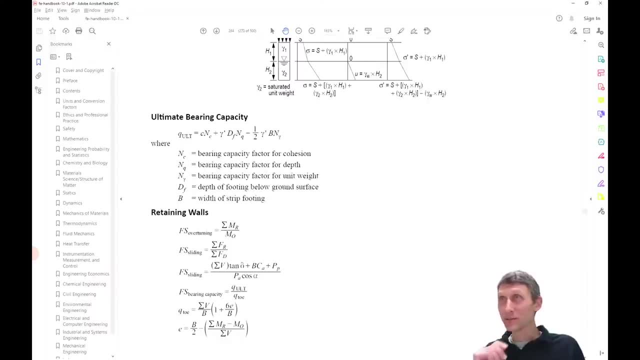 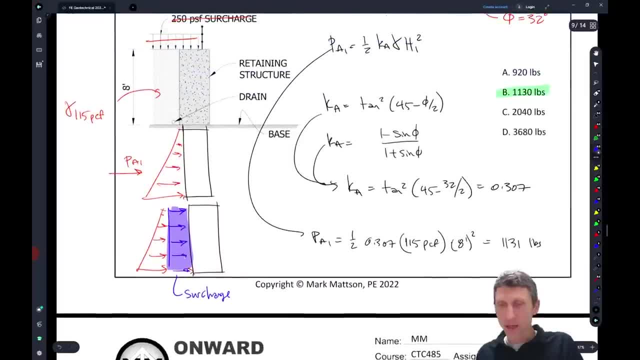 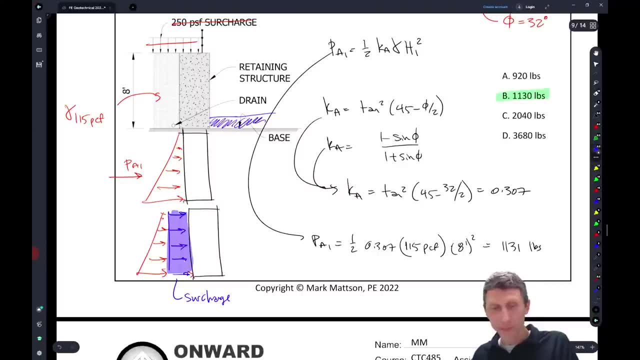 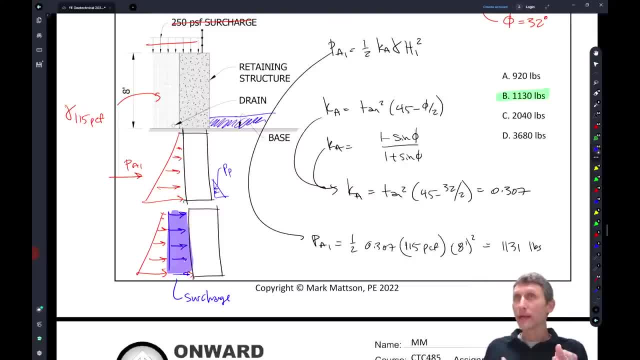 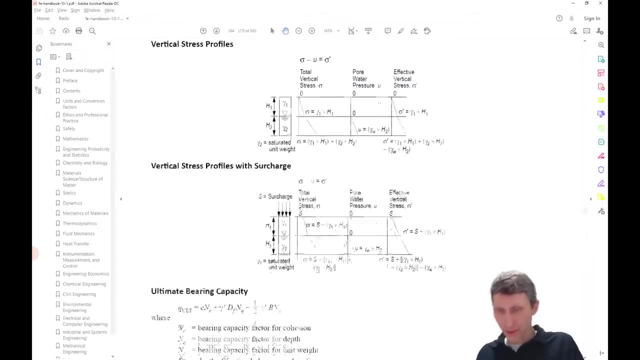 Right, A passive pressure that we'd have to overcome in order to push that wall over, And it's it's really hard to push soil. It's really hard to push soil out of the way compared to the what we have been on here as. let's come back to those pressure coefficients for a second. 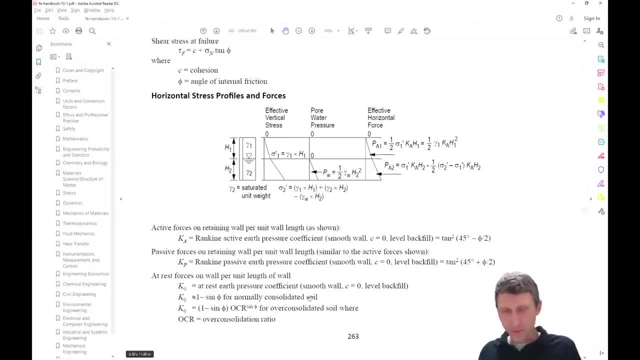 And if I can find my way there down my we're not scrolling that wonderfully If we look at this, plus v over two. well, I'm just gonna, I already have this in my calculator, So I'm just gonna do, instead of minus v over two. 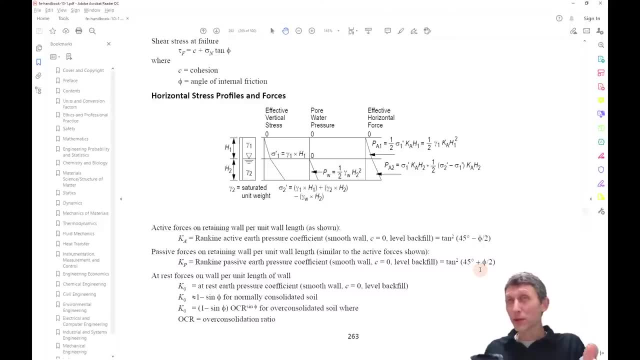 I'm gonna do plus v over two And instead of point 307, guess what I get? I get 1.8.. I mean it's huge. It's a huge difference, right That that passive earth pressure is going to resist. 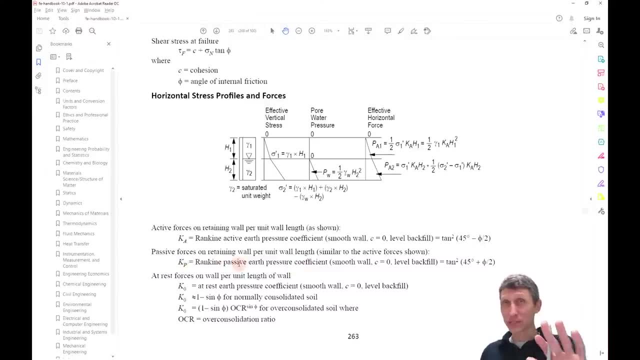 the wall being pushed. right it's going to resist the wall being pushed And that passive earth pressure coefficient is huge compared to the active earth pressure coefficient. So a little bit of you know embedding that toe is going to help you quite a bit when you're. 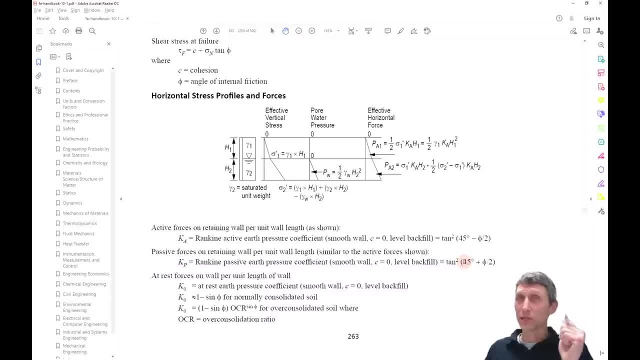 trying to resist overturning, you know, but you have to engage it, Okay, And that's where you know there's some debate on active versus passive, versus at rest, And it's, you know, this is where you smooth wall, and there's there's some other. 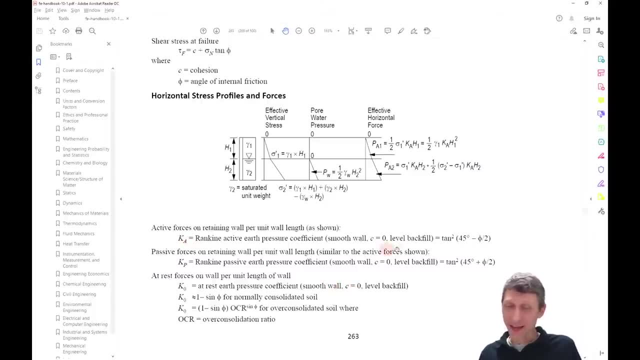 things going on here, But typically, what I would, what I would think they're going to ask you- is probably more like an active pressure coefficient situation. Okay, Retaining walls. we're actually going to come back to retaining walls in a minute, Well, maybe a few minutes. 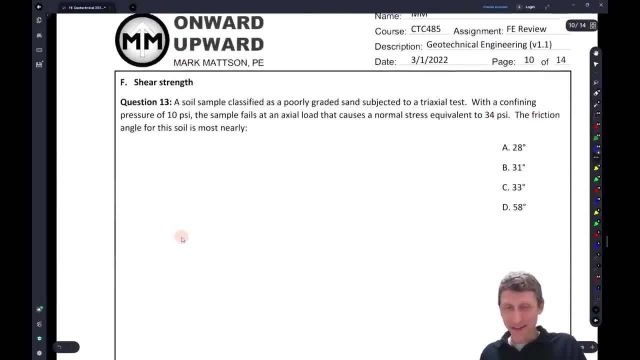 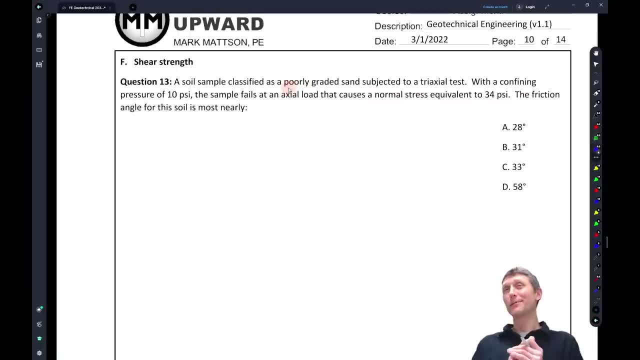 but let's keep going here And again we'll get to our poorly graded sand. So this kind of I probably could have put this in the lab test. I could have put this on other places, But this is there's a test for shear strength, Okay, And what we have is here. 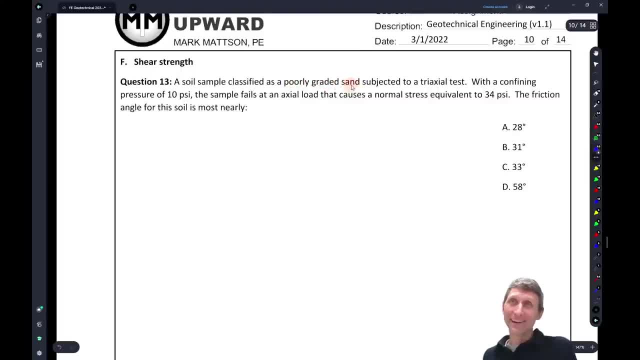 is a poorly graded sand. So what is poorly graded sand mean? You're all thinking it means a uniformity coefficient of less than four. Yeah, that's great. I'm glad you're thinking that. That's not what I'm thinking here, though Uniformly graded sand also means. it's what it means. Let's. 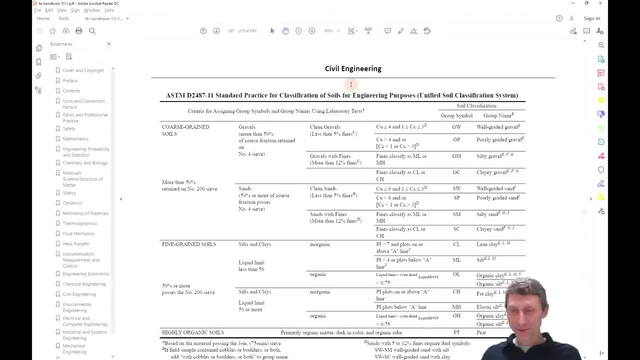 go back to our our, our, you know, coarse grain soils thing here for a second. It means it's not fine grain, which also? what do you know about sand? You pour it in a pile. I mean, there's a. 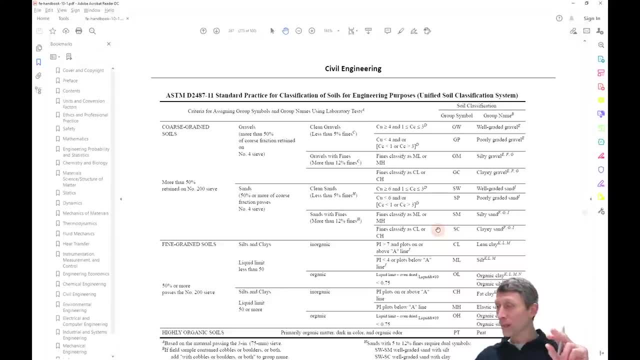 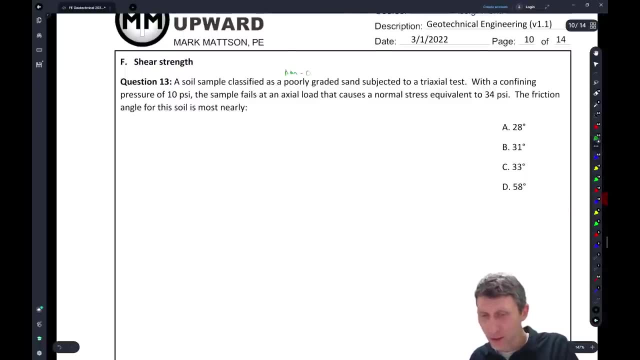 reason we have, we have timers that have you know, we have you know, we have you know, sand in them, right, Because the, the sand doesn't stick together. It's non-cohesive. Why is that? Why is that important? Non-cohesive Because when we're talking about shear strength, 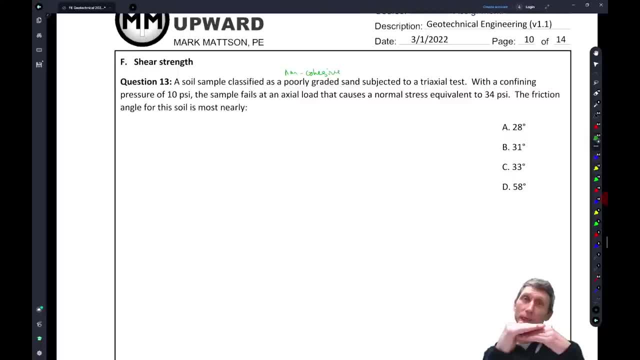 and trying to shear a plane of of of soil here. if it has cohesion- cohesion that's going to kind of stick it together, right. So a poorly graded sand typically is non-cohesive, doesn't have cohesion built in, Okay. So what we're looking for here is that that's. that gives us a clue. 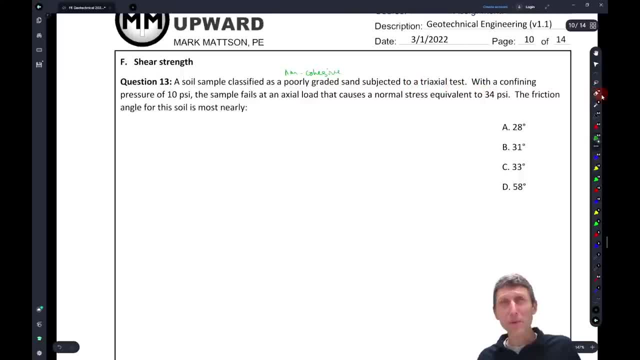 about what we're doing. It's subject to triaxial test, So there's a couple of ways of doing shear tests. One way is kind of to put you know shear and put a pressure, put a soil in, you know put. 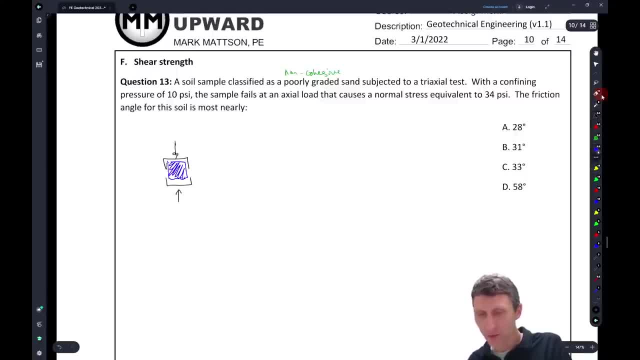 a soil kind of in in in here. So we've got a soil in here and then it's like a direct shear test, So we just push on one side, you know, push on the other side. This is kind of like a direct 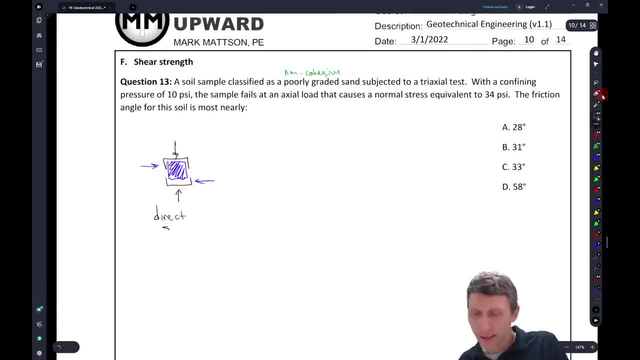 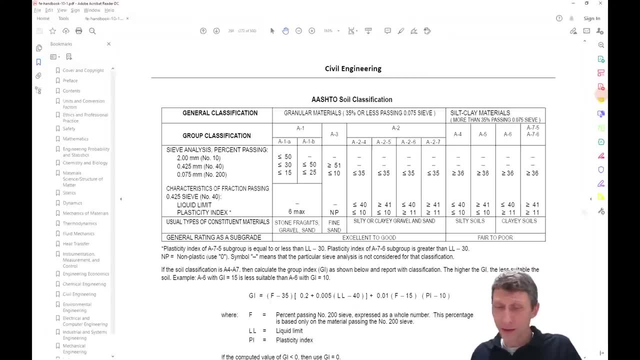 shear test. And if you were to have a direct shear test, um, it's great. What you could do is you come back here and if we come up, uh, we're going to have. we have bearing capacity. What else do we have? We have effective stress, We have shear stress. So 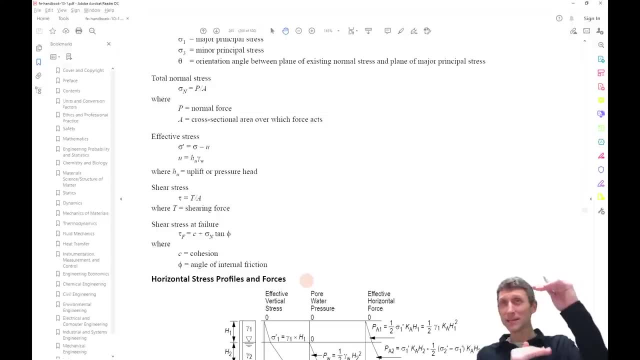 the thing is this: this is, you know, the ABCD version of what NCS puts out there. that's on the spec, skips all over the reference handbook. It's kind of all over the place. Um, but what we see here is we come back to shear stress, and if we have a direct shear stress, we could just you. 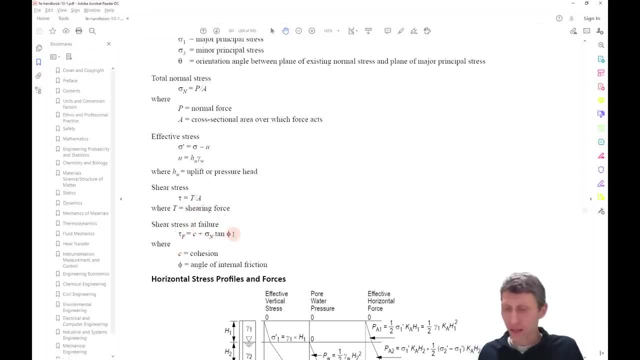 know, if we were given our direct shear stress, we could come up and calculate that friction angle- I don't know Internal friction angle. but also, going back to that cohesion thing, for a second, Cohesion gets added in when we're dealing with shear stress. right, That's there's. there's the part. 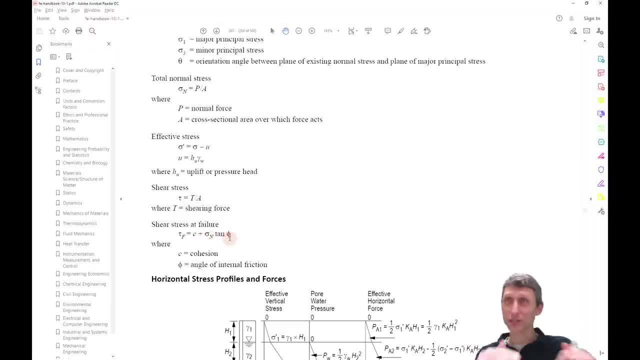 that's the, um, the, the soil, kind of like the shear strength. And then there there's the cohesion strength piece of it for the, the shear at failure. So if you're given a direct shear stress, you can kind of use this equation and plug in. That's not what we have. I just had to. 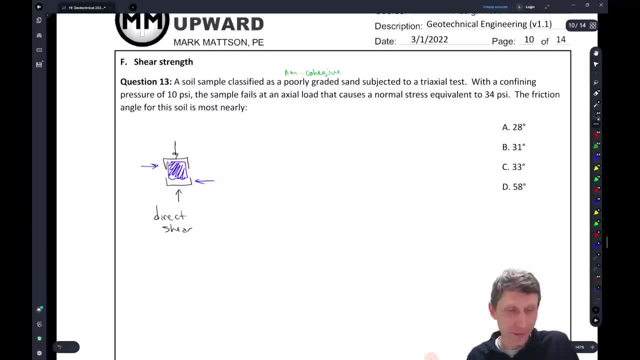 make it a little bit more complicated. I don't know, Maybe. maybe it's a little bit more complicated, Maybe it's not more complicated, Maybe it just hits another topic. You know, this is. this is kind of a problem. 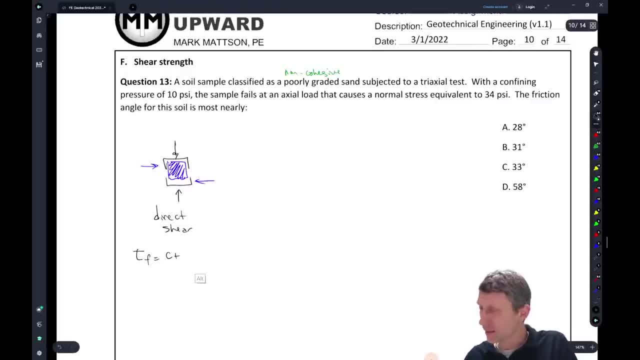 Plug and chug equation, or tau, F equals, you know, C plus uh. what was it? Tan uh um Sigma and tan fee. So Sigma, and that's the normal stress. tan um fee, right? So that's. 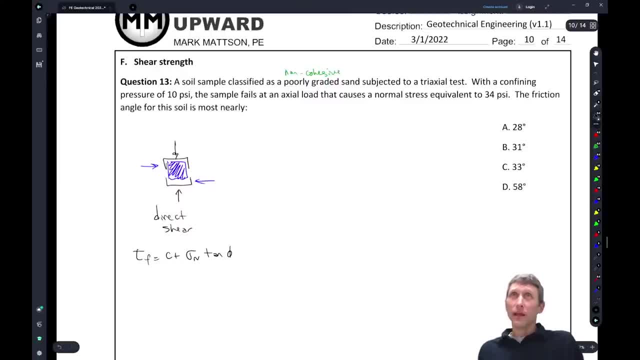 your direct shear? We don't have direct shear. We have a triaxial right, So we have a triaxial test. What's triaxial? Triaxial is kind of like you get this ring Okay And you push. 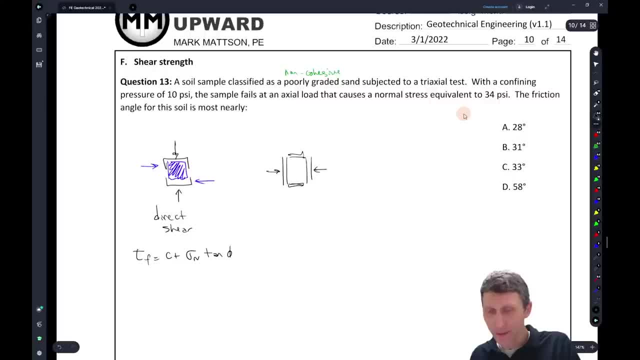 a constant pressure on the ring and then you have a disc on the top and the disc on the bottom, And then you have a disc on the top and then you have a disc on the bottom And you push here. So so we're kind of compressing this thing in multiple directions. So we have 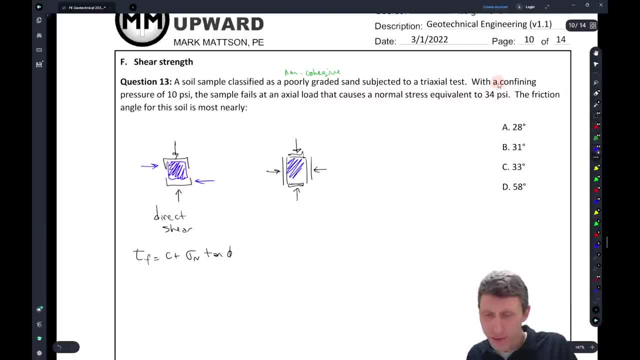 a confining pressure of for what we have here, right Here's the soil sample inside it, But what we have is a confining pressure of 10 PSI, And what happens is it fails with a normal stress equivalent to 34 PSI, And normally you do a few different tests like this and you get 10 PSI and 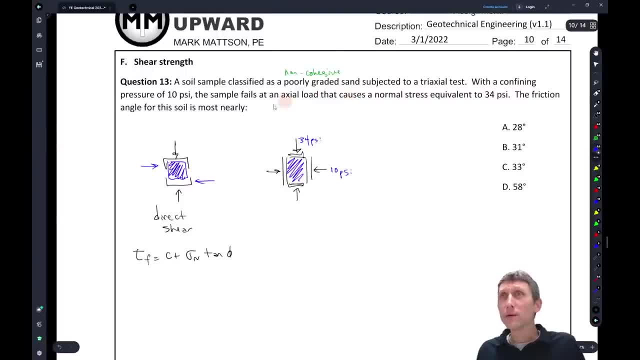 then you keep going. But um, for what we have is we just have one data point. the friction angle for this soil is most nearly. Well. you come down here and you say: but I can't use that equation. And you're absolutely right, You can't use that equation directly yet, but we can use that. 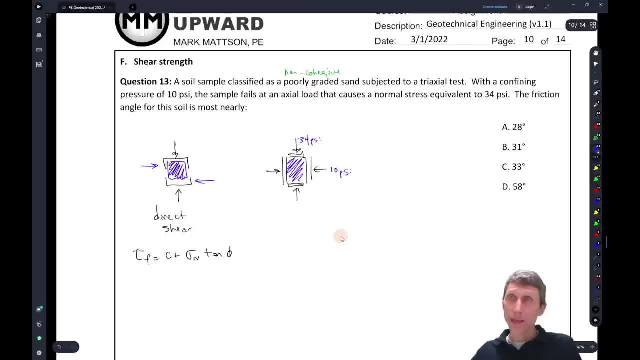 equation to solve eventually, for what we're looking for here, And this is going to um, this is going to give us something. So what we do know is we have a zero cohesion right, But what? what do we have? I mean, do you just take the normal stress? but 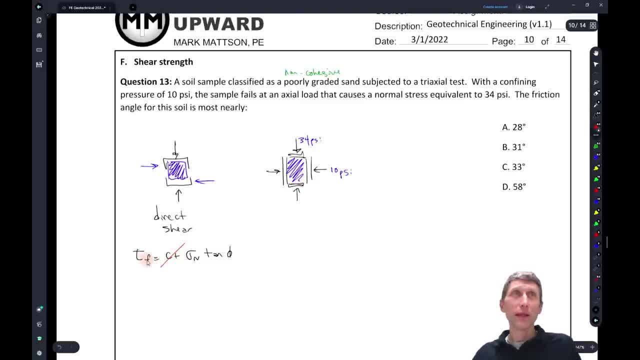 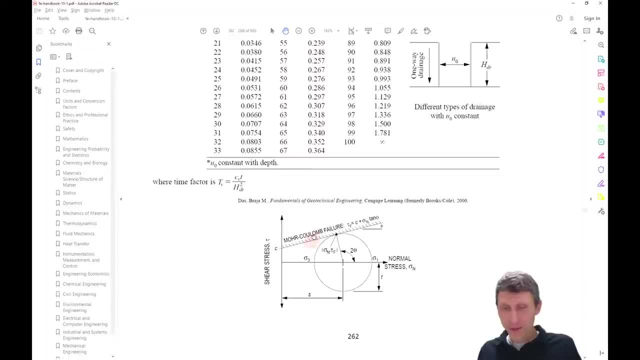 but we don't have a shear stress, right? So what do we do? Well, if you remember- maybe you don't remember, but maybe you do- um, maybe you learned something called more cool and plant failure plane, And I don't know kind of when we did, I think, mechanics. 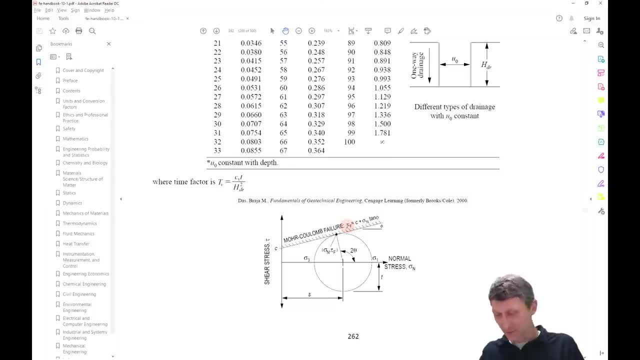 what did we do? Did we take a look at, uh, uh, did we take a look at more circle? that kind of the same thing going on here. What we're going to do is we're going to make more circle. We've 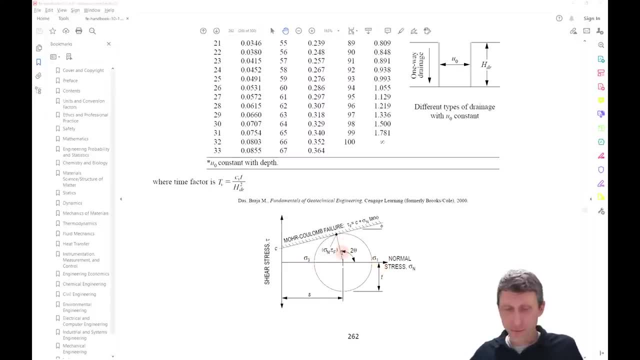 got the Sigma one, Sigma three, and then we're going to go, uh, from there. But what you see here is this fee is going to be the angle of this line That's tangent to that circle. So, uh, and then we're going to go from there, And then we're going to go from there, And then we're. 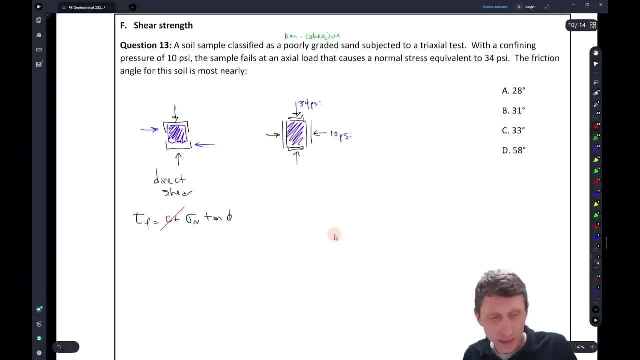 going to go from there. So if we come up here, um, what we could do is we could basically create this surface here, right, And what we're going to have is if we come out to you know, 10 PSI, 10 PSI and 34 PSI- uh, maybe I can drag this line out a little bit more. 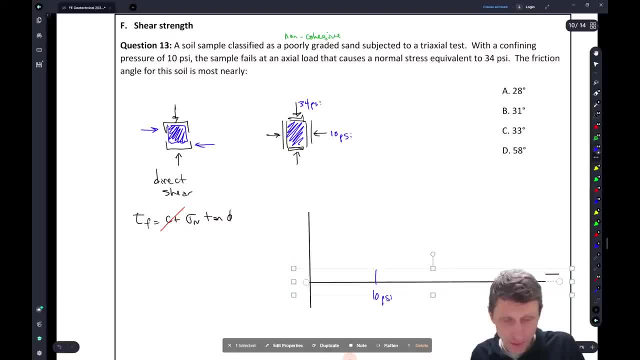 and I could make this like 34 PSI. maybe not what I wanted. Try it again. Um 34 PSI. um, what this is going to do is it's going to give us a circle and let's see if I can draw a. 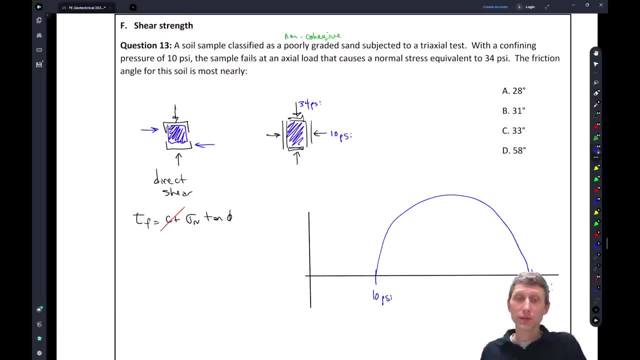 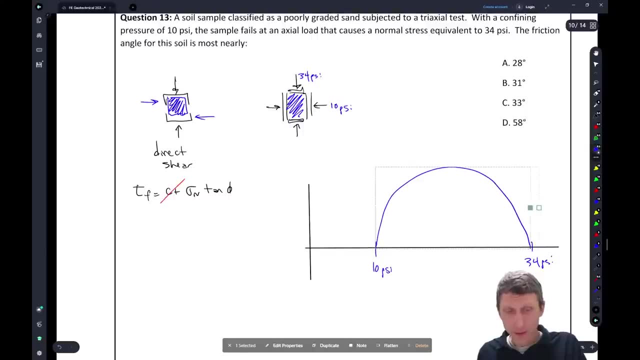 circle. Yeah, not bad. Um, it's going to be a circle That's going to be our more coolum failure circle, And maybe I can stretch it a little. a little, Okay, Um, and that's going to give us. 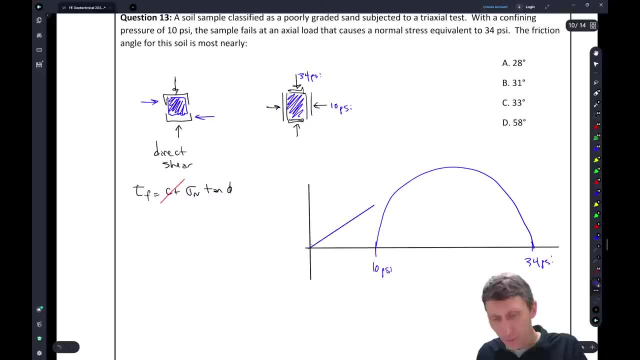 our circle, But what we ultimately want to do is we want to, we want to take a point here and we get this tangent to uh the curve. So so, if we know this point, you know this point and a line. 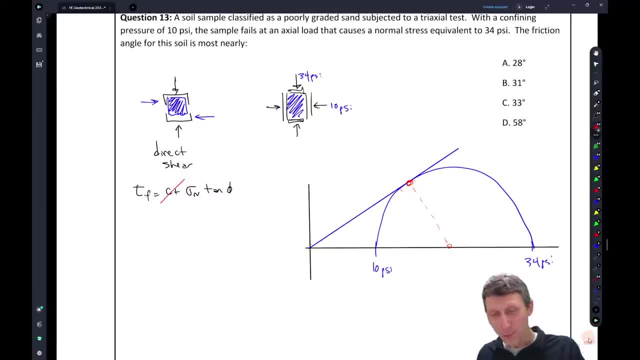 that connects them. guess what we have? we have a right triangle, which means we can come back here and find fee once we can, once we can do this right. So we can find fee just based on, uh, that right triangle. 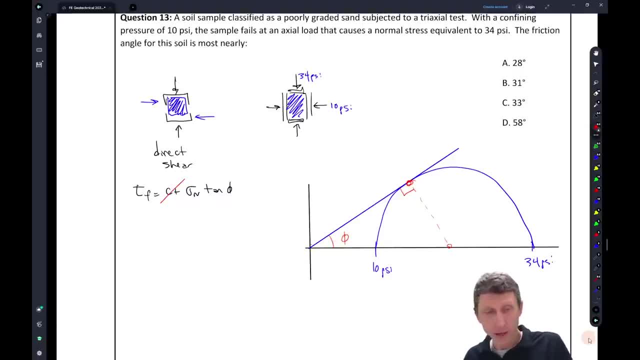 right. So with with this, what we can do is we can say, well, okay, wait, wait, wait, wait. I know that the sign of fee equals what. it equals the opposite over the adjacent right, I mean. 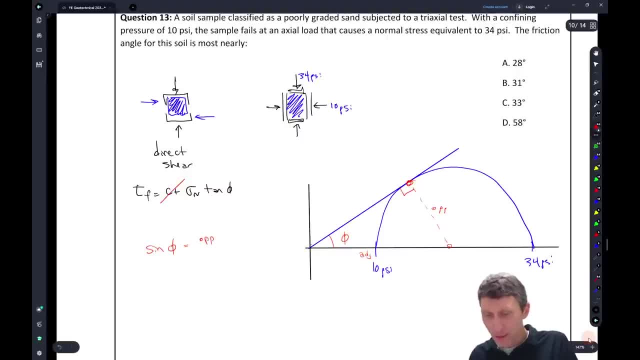 this is just trig, one-on-one um, but the opposite, the opposite over the adjacent. So what's that going to be? It's going to be the radius over the Sigma average right. This, this is going to be our Sigma average right. So how do we get? 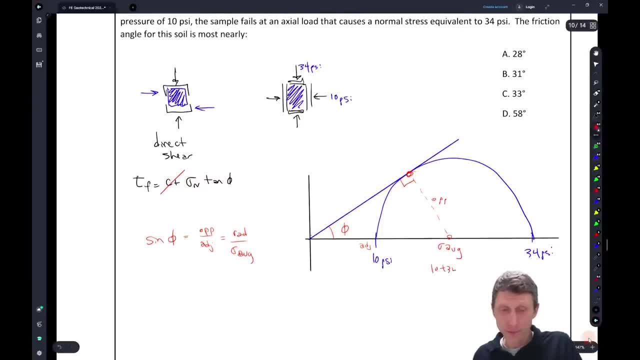 Sigma average. Well, Sigma average is just what? well, that's 10 plus 34 over two, which equals what? 22 PSI. Okay, So that's our Sigma average. So you know, sign fee equals, uh, the radius. 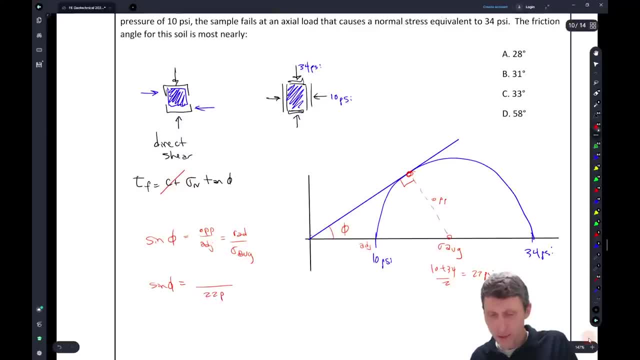 over Sigma average. What's this? Um well, we have 22 PSI, which is their Sigma average, The radius. hopefully you can see this, but we have 12 PSI here. 12 PSI here, right To go from. 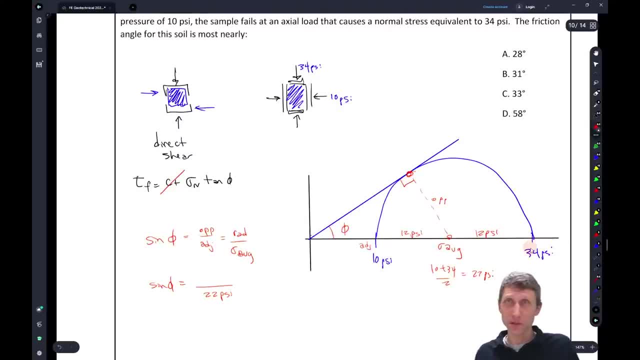 um, the 10 to the 12, to the, you know, or to the 22 to the 34.. Okay, So that's our radius. That's going to be our 12 PSI here as well. So, um, we can find fee right. Sign inverse of what 12 over. 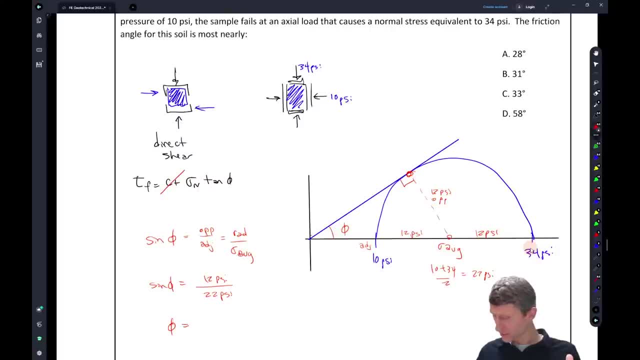 22 is going to be: um, did I what? did I screw up? Did I screw something up? Oh, I did. the sign That doesn't work. Sign inverse of 12 over 22 is a 33 degrees Okay. 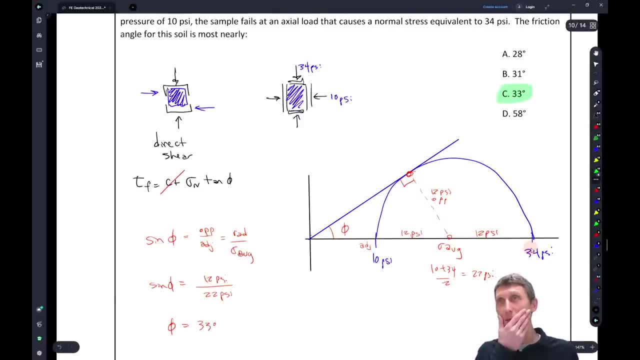 It's a lot of C and D answers today, but that's where it goes. So you know, we could, we could find I mean this point here is Sigma N tau, right? This is that point. Um, right, That's. 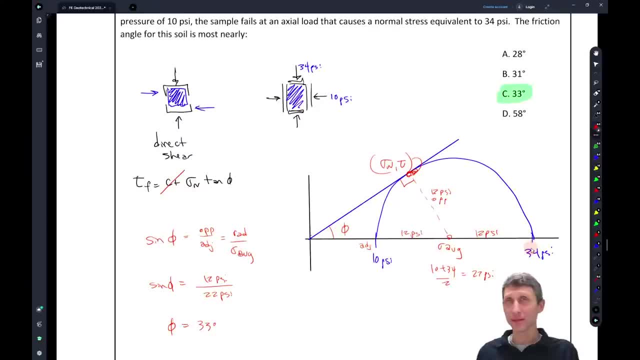 that point. We could go and find that point, but the, the, the sign is a lot easier to use if we have- uh, if we have, a circle and a right triangle. Okay, So that's a, that's a sheer strength. 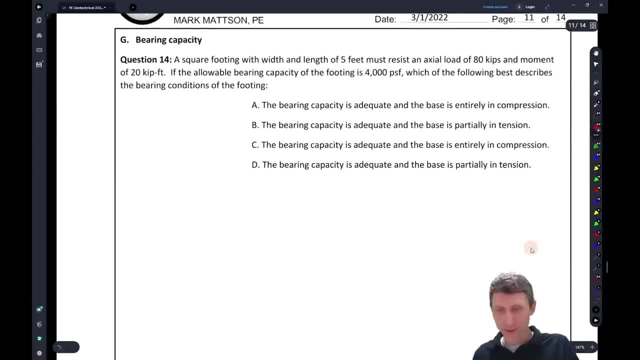 Well, let's keep going. And uh, this is, this is one of those ones that I think is kind of fun. Um, we've, we've got a couple more that are, I think, hopefully a little bit easier and after this, but we'll see, maybe they're not easier, I don't know, Maybe they're more. 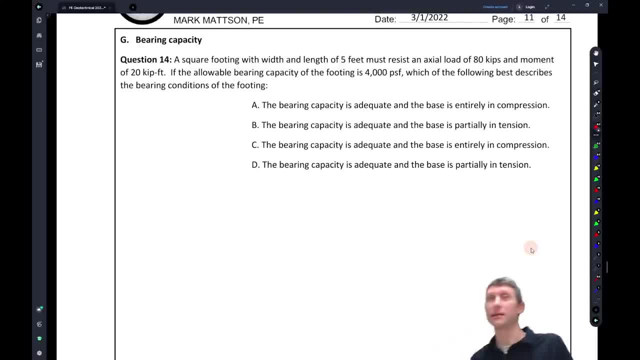 plug and chug This one. this one's interesting. This one's interesting because, uh, this one gets to retaining walls, It gets to bearing capacity, It gets to a whole bunch of things. And you know, if we come back to the manual, uh, there is a bearing capacity equation in here. 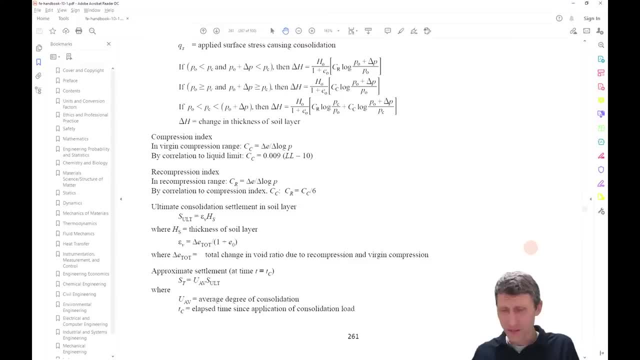 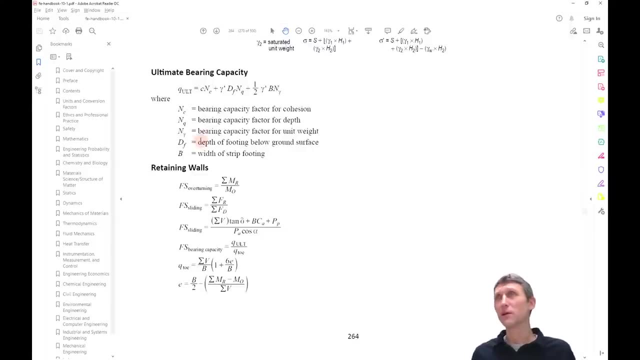 And am I missing it? Where's the bearing capacity equation? It's, it's down here somewhere, right, There's a bearing capacity equation. And if you get a bearing capacity equation and you get a whole bunch of parameters, great, Just go, plug and chug. Okay, Plug and chug, Make sure that your 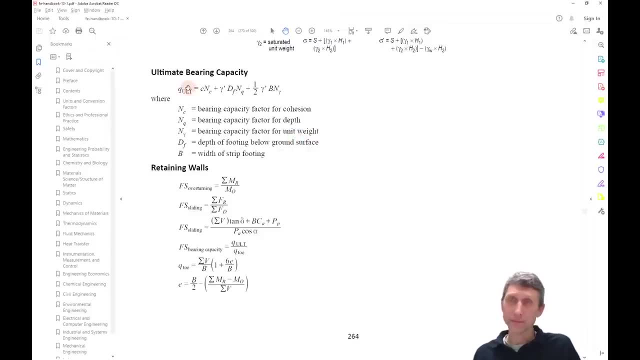 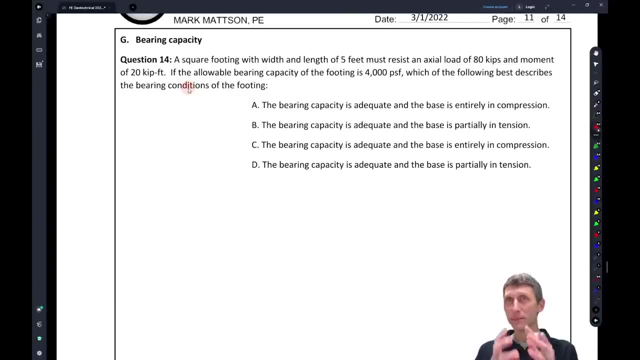 your units all work out, Plug and chug. You should be able to evaluate that right. So so I'm I'm skipping over that problem today. So then, idea of let's look at bearing capacity here on a bigger picture, kind of this is what 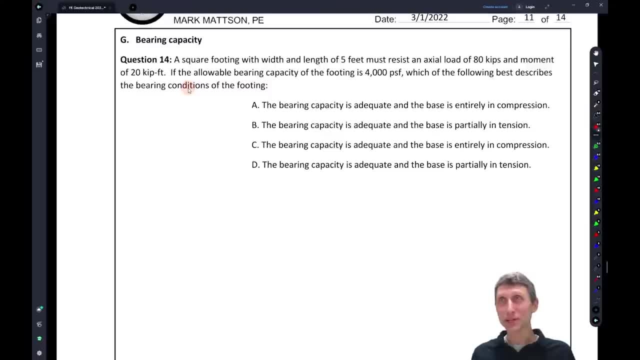 you're worried about when you're designing to a certain degree. I mean you're you want to make sure that when you do your footing or whether it's a wall footing or it's a retaining wall, right. So I mean coming back to our retaining wall for a second. I mean I could have made this. 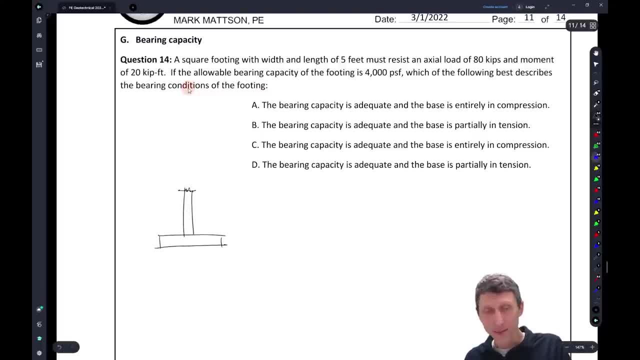 a retaining wall footing. Um, I, I made it kind of a column footing, but the idea here is: we have, you know, 80 kips acting down and we have, uh what, 20 kip feet trying to overturn the thing. 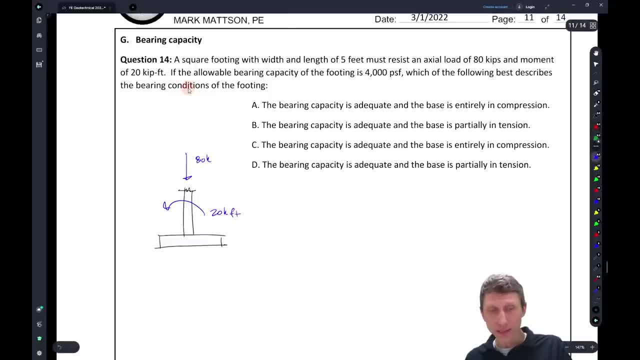 So the question is: we're going to get some base pressure underneath this thing. Okay, So we're going to get some base pressure underneath this thing, And is it adequate? And is it entirely in compression? In other words, if this moment here is big enough, it can start to lift up this. 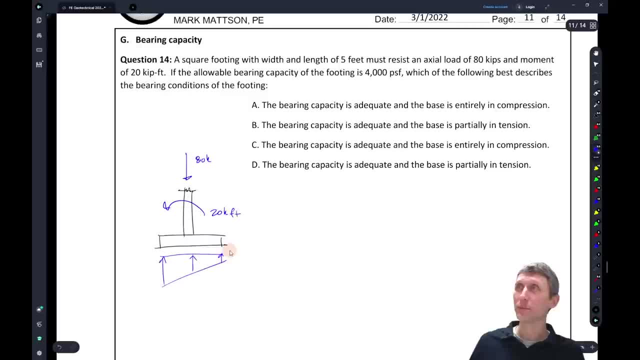 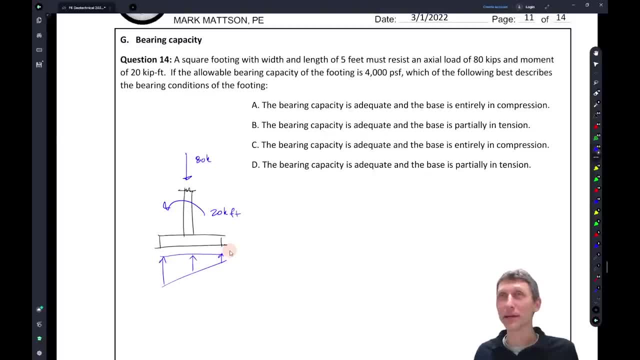 don't. normally soil doesn't pull back on your footing to hold it down, unless you put like a rock anchor in or something. So the question is: can we do this? And I thought this was a better question than just a plug and chug one. So I figured: let's, let's look at this And this is: 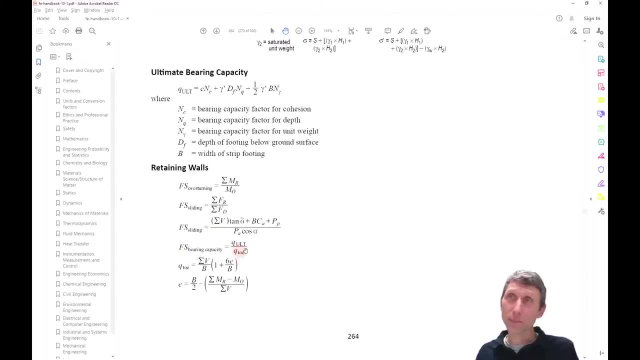 where we get back to this retaining wall piece of it as well. So we know that the bearing capacity is just like the essentially the allowable, um. well, this here's the factor of safety, of bearing, but. but basically, what we want to know is, um, what do we have So? so what, I'm told. 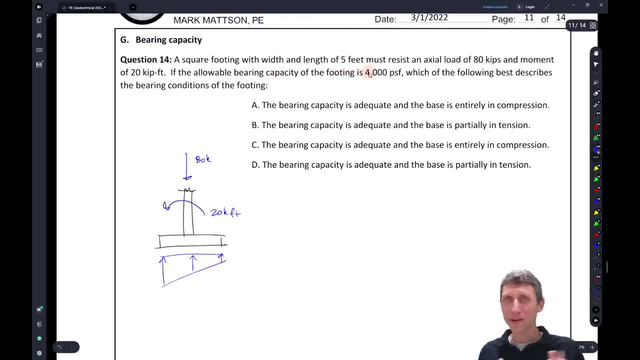 here is: this is an allowable bearing capacity, and we're not doing an ultimate here, but this is just allowable. So the first thing that I kind of want to check here out with this one is: it doesn't make sense. Okay, Um, in other words, the force divided by the area is that okay? Well, it's not that. 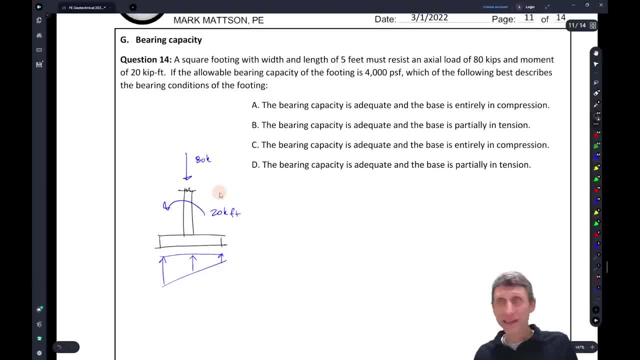 simple, because we have this bending going on in here. So again, I can take a look at like for a one foot strip here. you know, for one foot strip, what do we get for a one foot strip? Um, you know, I, I I'm looking at a five foot by five foot. you know, square column footing. 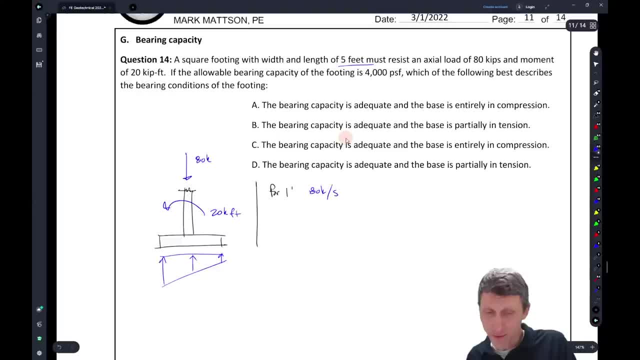 but for one foot we could say: well, 80 kips divided by five is going to be what? 16 kips. and you know, 20 kip feet divided by five is going to be what? that's uh, four, right, Four kip feet. 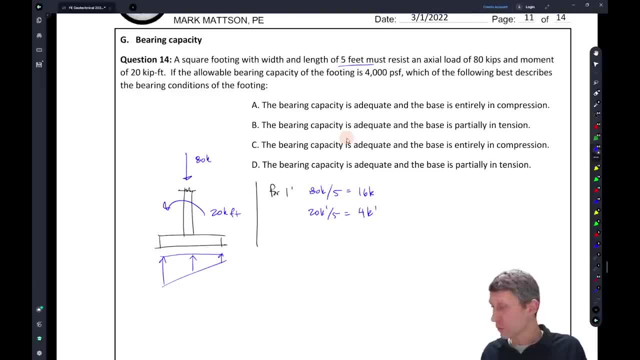 Okay, So that's great. This sort of brings it back into retaining wall world, right? And then we get into all these equations here which are all sorts of like: ah, now we got to find the bearing capacity. So we're going to get into all these equations here which are all 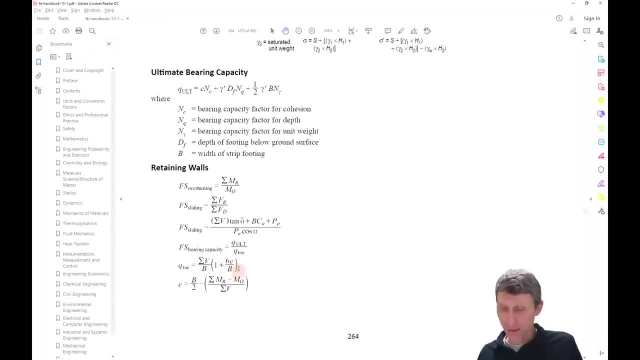 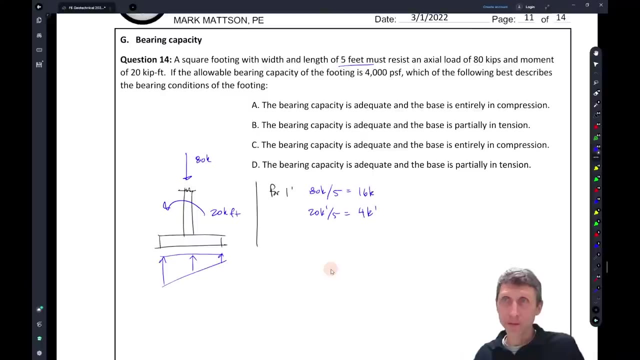 pressure at the toe and, you know, kind of at the heel. So can we do this? The Q, toe and E, what? what does all this mean? And let's come back and take a look at it. Okay, So what's this? Um, you know, let's look at that, Let's just write it down. 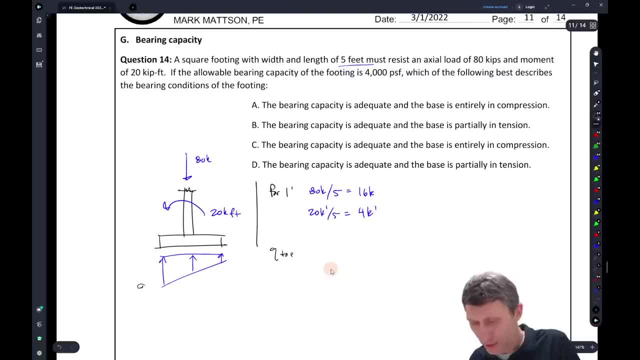 Sorry, It's not G, it's Q toe. They're right, This is the pressure at the toe, This is the pressure at the heel. A lot of times with, you know, retaining walls, they look like this right, They look like a little shoe there right, Um, where you have. 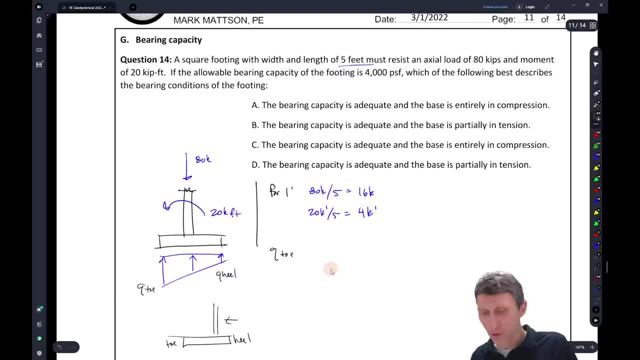 a toe on one side and a heel on the other, And you're trying to push it over this way. So we, we, we kind of don't have that for us, but that's okay, That's. that's where the toe and the heel comes from, Um, and that's. 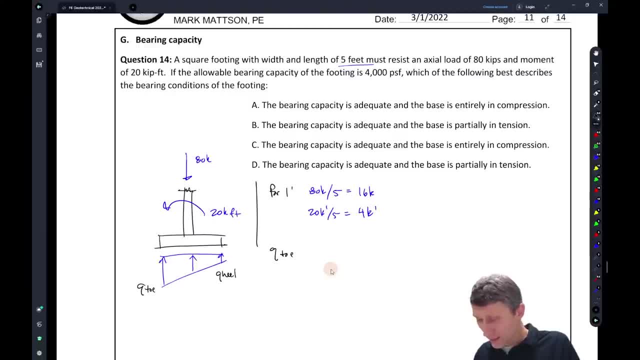 that works too. but basically we have a Q toe and the equation was equal to some of the vertical forces divided by B times one plus six E over B. And you're thinking, man. I just wish you did the plug and chug formula because it's getting late and that would have been easier and it would have. 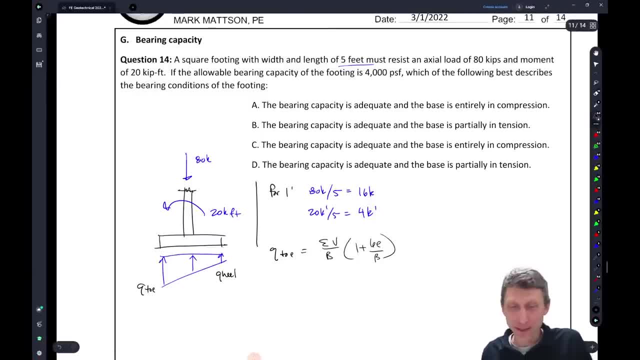 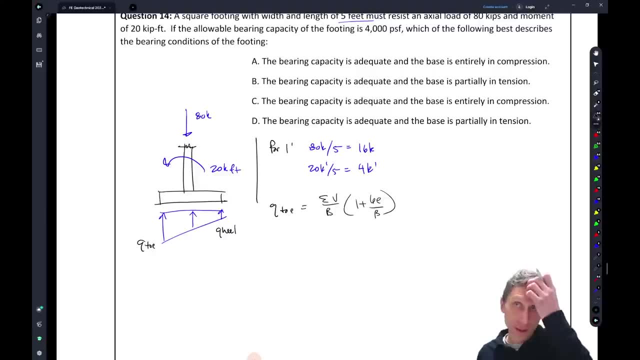 been, but I think this is a better question. Okay, This is actually something that I wrestled with a little bit when I was first starting out as an engineer, and all of a sudden it made sense, And I hope it can make sense for you as well. But basically, what we're trying to say is: what's the eccentricity on this? 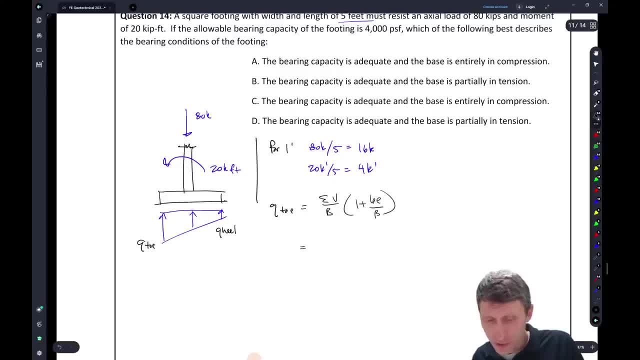 footing Okay. So so what we have so far is the sum of the vertical forces. We got 16 kips down divided by the width, by feet, right, So our width here, our width is just five feet, Okay. And if 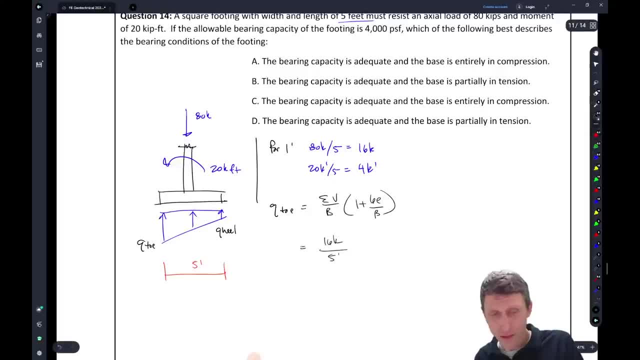 we're doing a- a one foot strip of wall, let's take a look- Or one foot strip of footing, whatever 16. And then we're going to do one plus six times E. We still don't have E yet, So I'm just going to leave E in here as a placeholder. I'll come back, I'm. 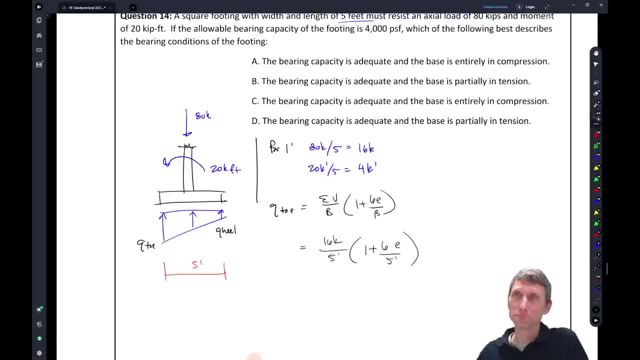 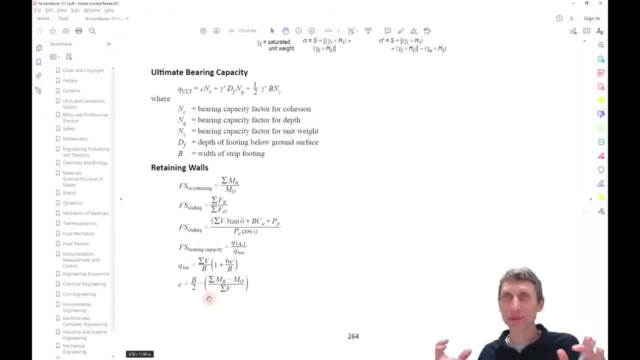 divided by five feet. So all we have to do is find E right. What could, what could be hard about that, It's I don't know. but then we get another equation and it's like: ah, we have to do a. 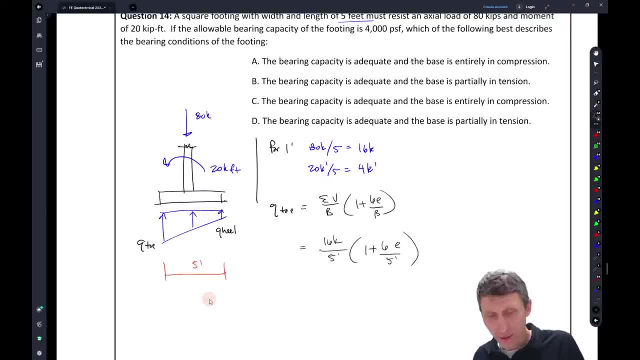 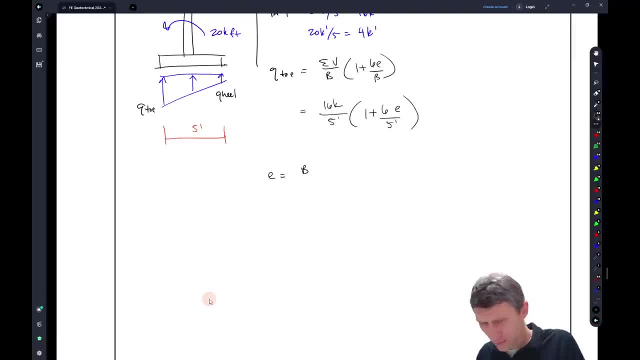 stability analysis again. So let's look, let's write that equation down and let's see what this says. So E equals B, B over two minus Sigma, M resisting minus Sigma, or no? let me just double check this: Sigma um. 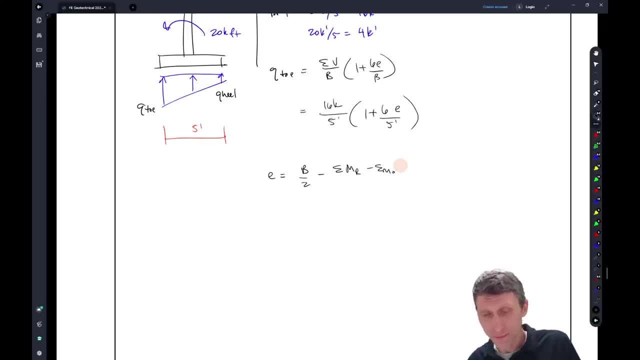 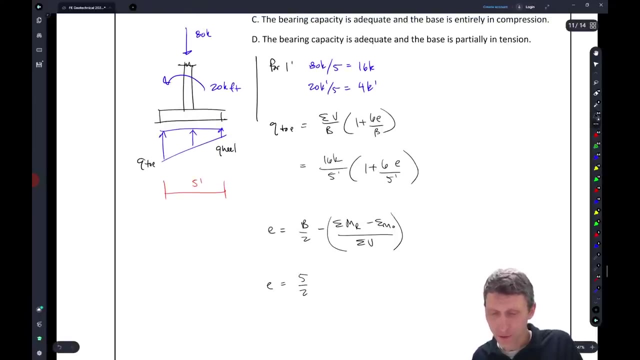 Sigma M overturned, moment overturning, and um divided by Sigma V. Okay, Can you do this? I think you can. Okay, So let's take a look at this for a second: E equals B over two, So five over two, five feet over two minus what. 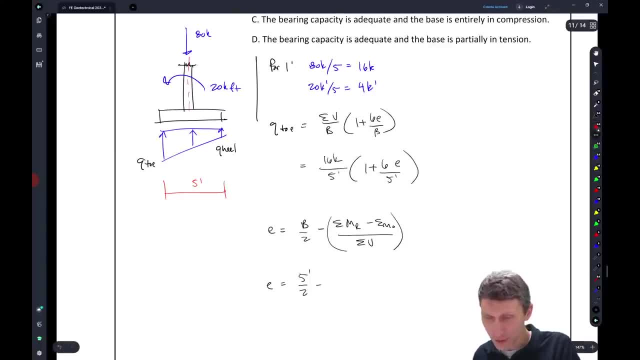 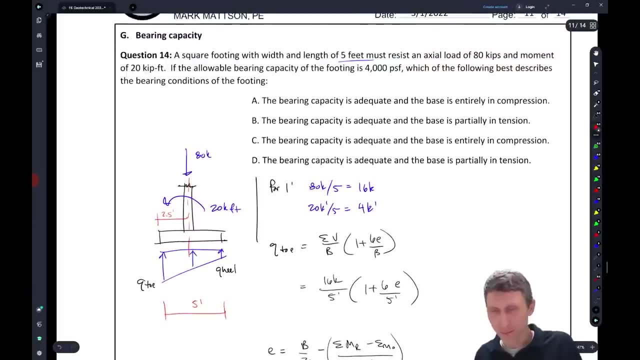 So. so essentially we're saying E. So if we have a column, you know, center line here, that's that's. I probably should have said that this is 2.5 feet somewhere in the problem statement. Maybe I'll update the problem statement for this one as well, You know. 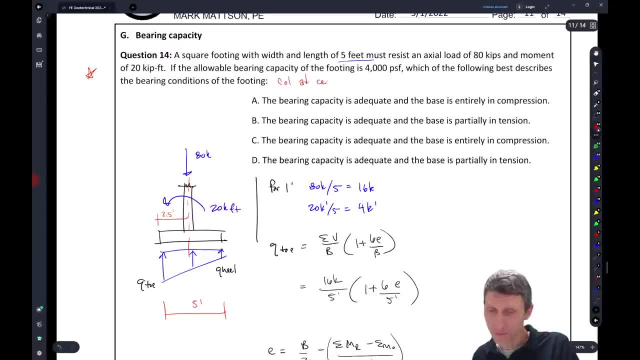 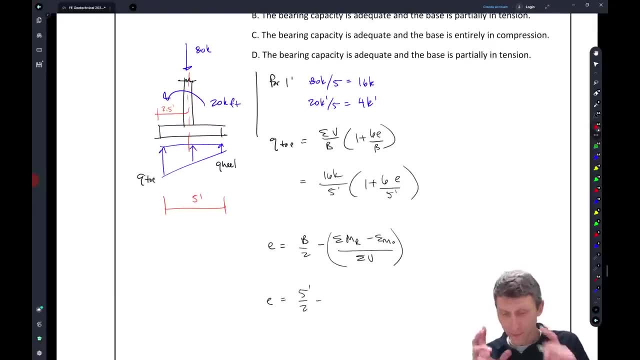 the column is at the center. Um, right, So the columns at the center. what does that mean for E? Well, it means that that's the five over two. Um, but why do we care about that? Because the resisting moment is what? The resisting moment. 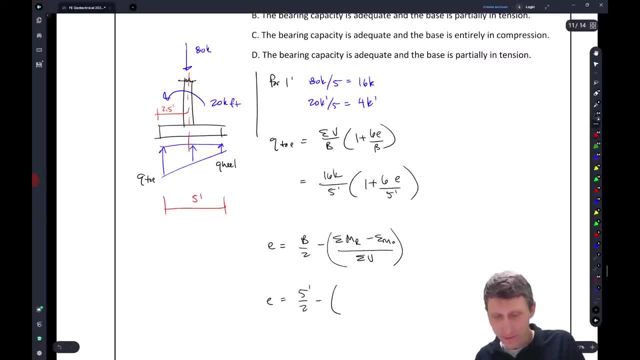 is 80,. well, actually it's 16 kips times 2.5 feet. That's the resisting moment. right, That's our resisting moment. Um resisting, Okay, That's our resisting moment. That's what's holding this. 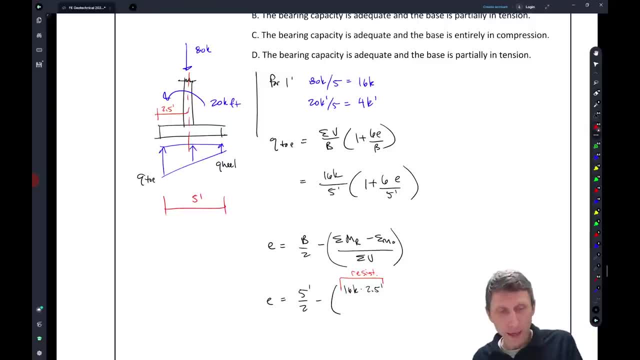 thing down. It's, it's holding this thing down, but the 20 kip feet is trying to push it over And that's our overturning moment is going to be. you know we're using instead of 20 kip feet. 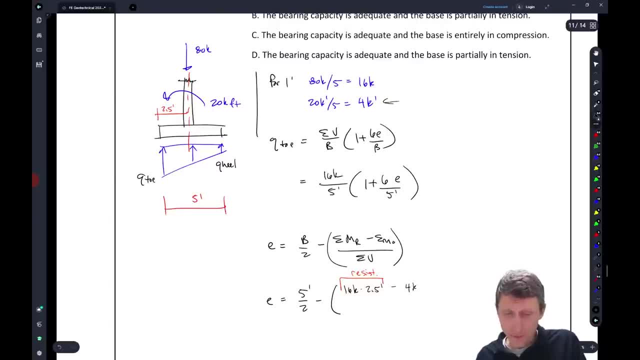 we're using four kip feet because we're just taking one foot section. So four kip feet, that's our overturning moment. Okay, All this by the vertical forces, which is 16 kips, And that's going to give us an eccentricity. 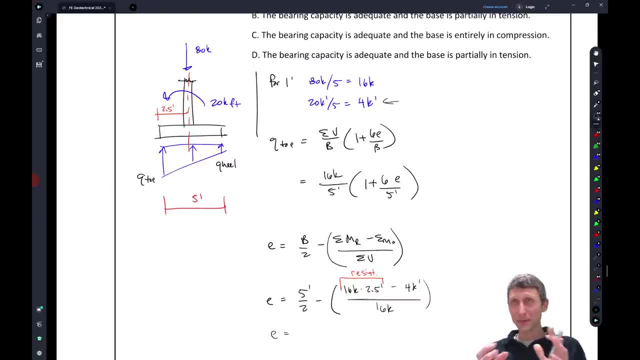 here. So, in other words, it's taken this 80 kip feet, it's taking that 20 kip feet And it's kind of balancing and saying: what is the eccentricity, What does that look like? And if I did this right, 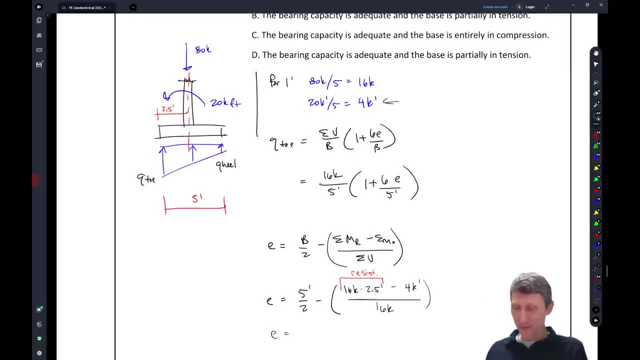 five over two, uh minus what in parentheses- 16 times 2.5,, uh minus four, and then divide that by 16. I got like 0.25 feet Okay. So the good news is we can come back. 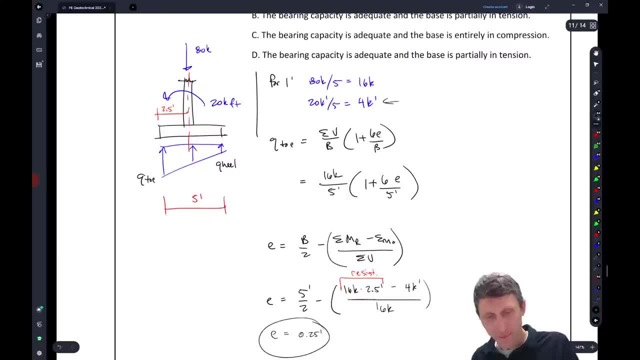 In here. Um, I can take that 0.25 and I can. I can plug it in, All right. So I can take this and plug it in right up here and I'm going to get my Q at my toe. Actually, I'm just going to erase this. 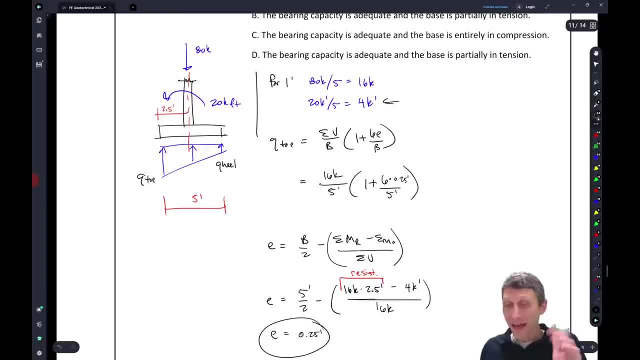 because that's going to make my life easier- 0.25 feet, And now we can solve this. So the Q at the toe equals what? 16 over five times in parentheses, one plus six times 0.25 over five. 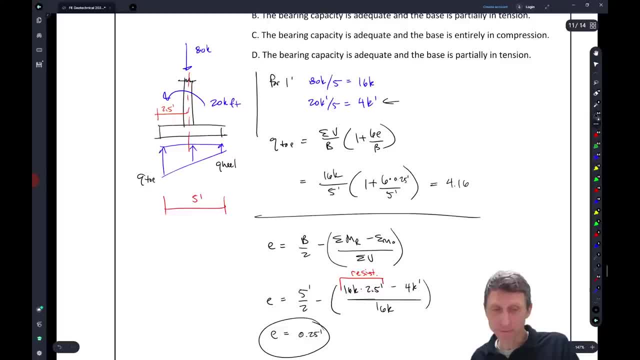 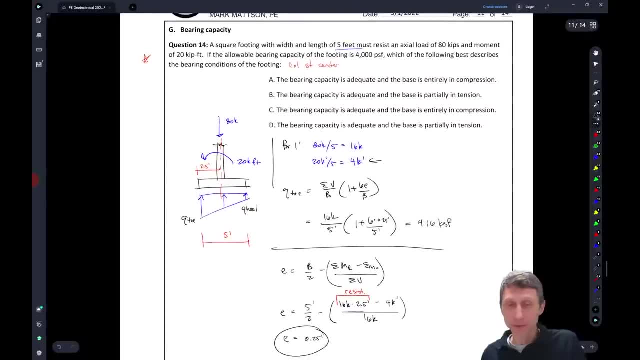 And I get like 4.16 KSF hips per square foot. What's the problem with 4.16 KSF? 4.16 KSF is greater than four KSF, which is Q allowable, Okay, QA. So what that means is the. 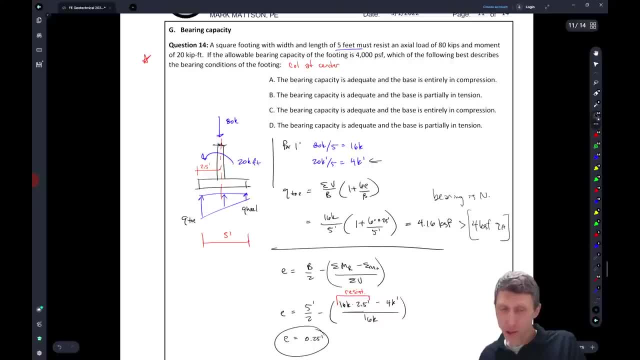 bearing is no good, It's inadequate. Okay, So the 4.16,. it's more than what the soil can hold up. So the bearing capacity is inadequate, Did I I? oh man, I made another typo, two typos, Sorry, I. 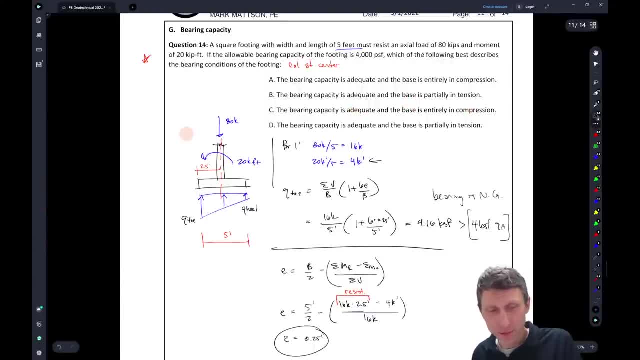 tried to double check this. Ah, okay, I need to fix this one too. The bearing capacity is adequate, or the bearing capacity is adequate, Okay, So we're going to have to have an inadequate one here and, uh man, two mistakes. I apologize, Um, inadequate, Let's. let's make these both. 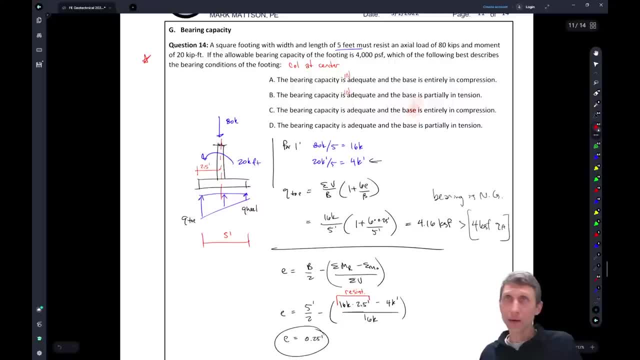 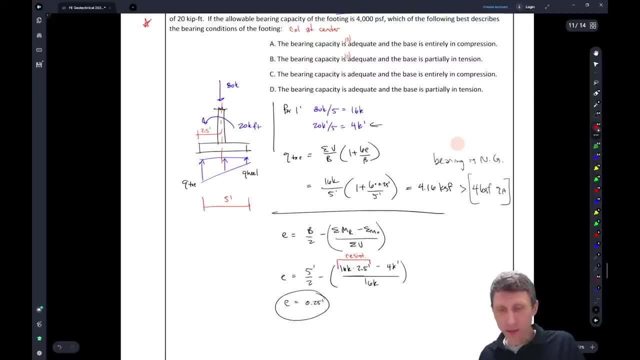 inadequate here. Okay, So it's. and then are we entirely compression Or are we partially intention? Which one is it Okay? So if we come back in here, well, how do we get the? how do we get the heel? So, if we get the heel, um, maybe you remembered that this can be. 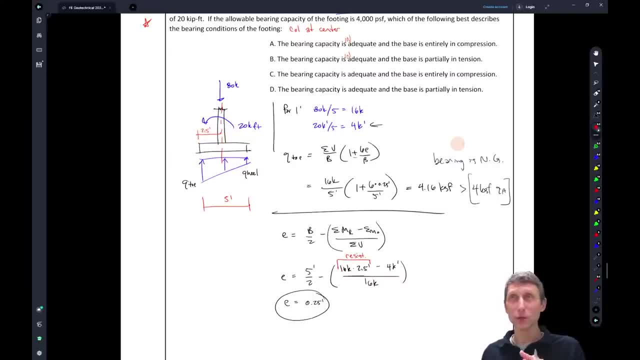 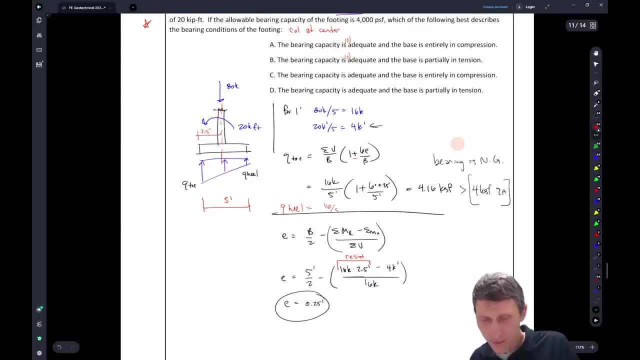 like a plus or minus. You remember that the minus is the Q heel. So the the Q heel is going to be the same equation: 16 over five. but it's going to be one minus six times 0.25.. I'm going to make 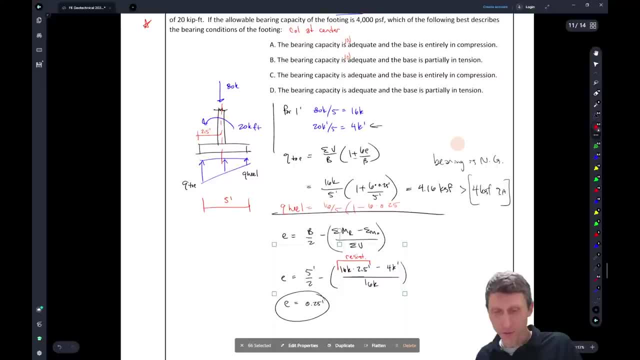 more room here. Uh, it's so easy for me to make room. I'm sorry, if you're working with a pencil maybe it's a little bit harder. Um, but you know I can make that room here. Um, six over 2.5, over five feet in this is. 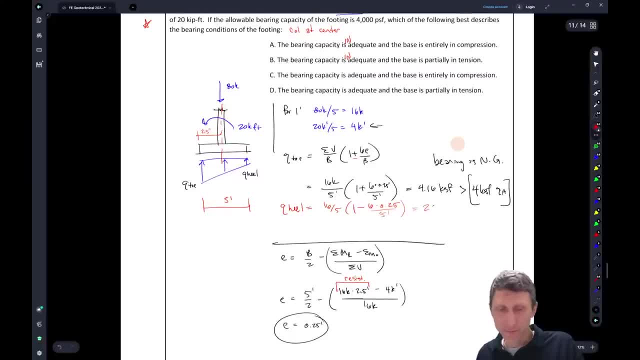 going to equal. I think I got like 2.24.. Okay, So 2.24 means it's still in compression and that's good. So the Q heel is still in compression. We didn't get a negative value, So the total: 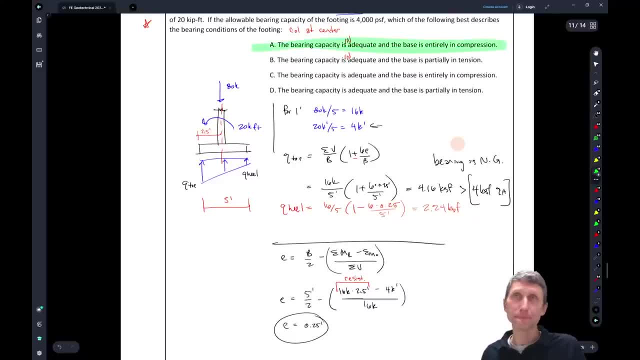 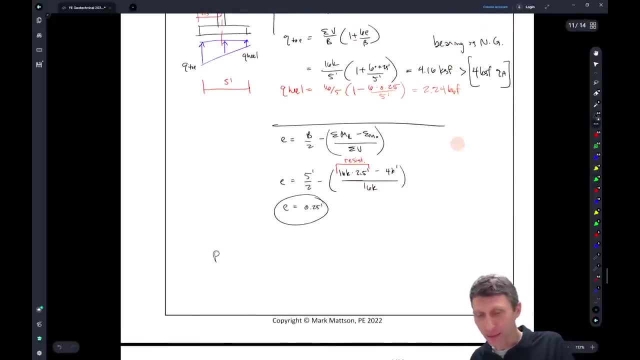 the total here is going to be in compression. All right, There's another way you can look at this. Honestly, the way that I like to look at it is like, if you remember, remember that whole um, um, mechanics and materials, maybe if you 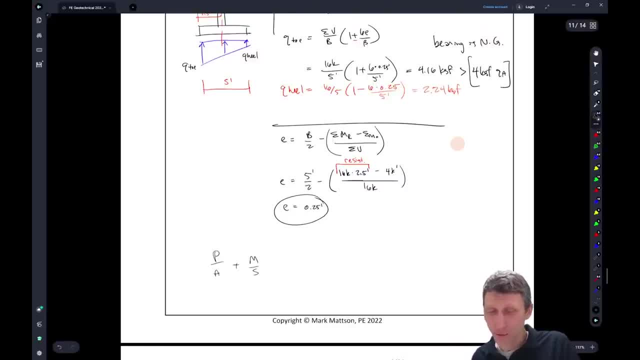 haven't looked at that review. you can but P over a, plus, M over S or um, you know, plus or minus M over S, right, The axial, uh, plus or minus the bending, Remember that combined stress thing. 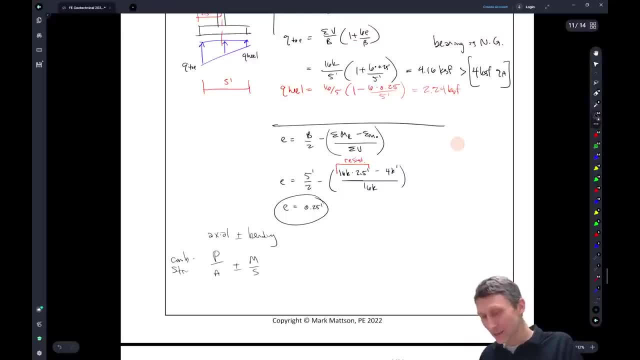 Um, right, And this is. this is another way of looking at it. This is, you're going to get the same thing, but what's this? It's like 16 kips over five. you know square feet um plus or minus. 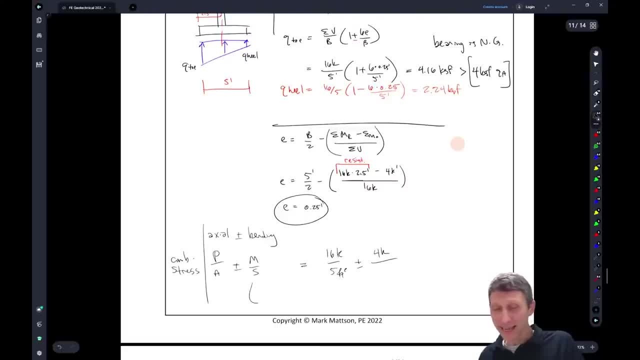 the moment, which is four kips divided by. well, what's S? S is? I looked this up. I was hoping it was in the manual. It's maybe we we shouldn't use S, we should use M Y over. I the reference. 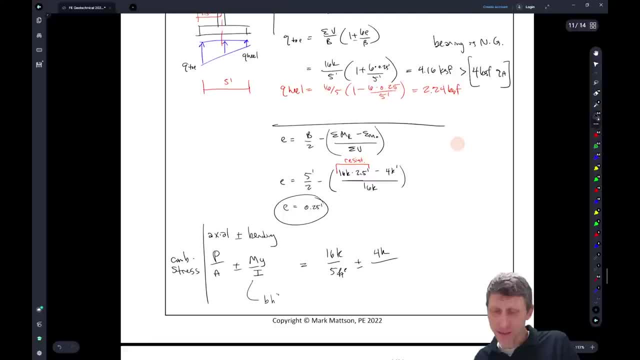 handbook has M? Y over I. I is B H, cubed over 12.. Okay, And this is going to be: the B is going to be one foot width times five, But cubed over 12, and Y is going to be 2.5.. If you do this out, um, you should actually get. 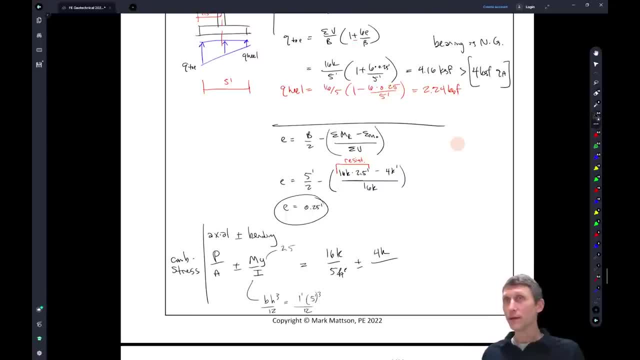 the same values. So, again, this is another approach to it, but it's it's looking at that basic mechanics of materials, um, axial and bending stresses, uh, which hopefully is something that you learned when you did mechanics and materials as well. Maybe this is, maybe this: 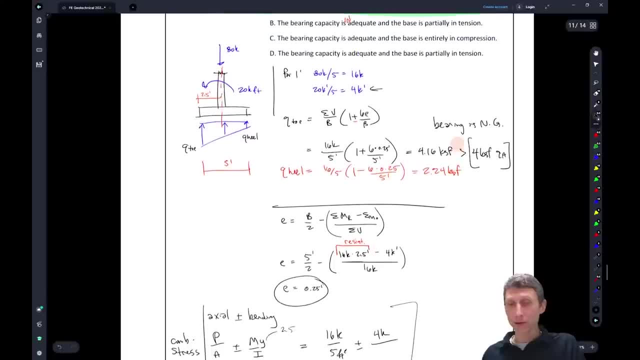 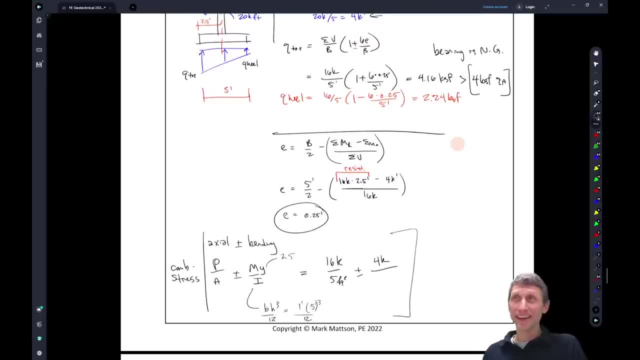 version's a little bit easier for you. I don't know, Um, if not here those equations from the, the bearing capacity, um retaining wall formula. All right, Okay, We're getting close. Okay, Um, which type of foundation? 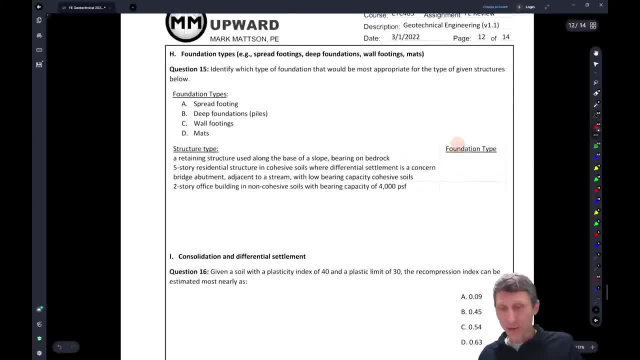 would be most appropriate for the given structure. Uh, I'm not going to spend a lot of time here, but let's, let's take a look at the retaining structure along the base of a slope. Um, we're going to use a wall footing. Okay, Wall footing um parts there, you know, see um wall footings. 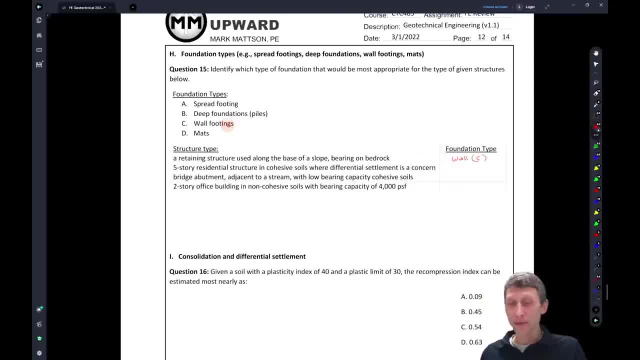 are ones that go along the length of a of a structure And that's going to be especially on bedrock. I mean, you're just going to pour the footing, pour the wall and be done with it. Uh, five-story residential. 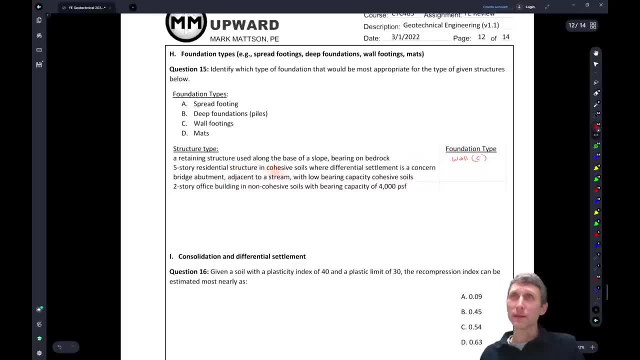 building a relative residential buildings are relatively light structures. Um cohesive soils, differential settlements- a concern. Typically, the bearing capacity is probably not the best. Um sometimes you have to worry about different pieces settling A lot of times. um, some of those. 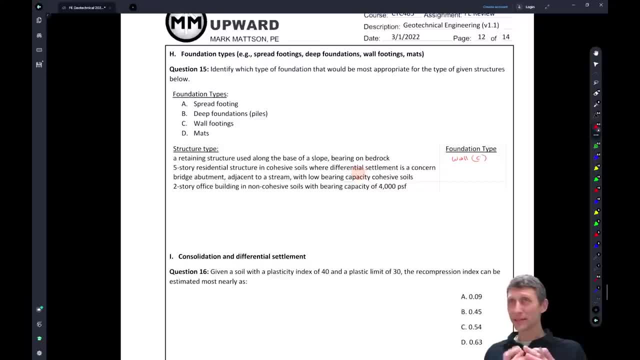 cohesive soils, you'll have- uh, you'll have- some fines in the bearing capacity. You won't be the greatest anyway. So you'll end up with bigger footings, And sometimes what that'll do is it'll turn you into a map footing, And so I would say this would probably be best suited for a map. 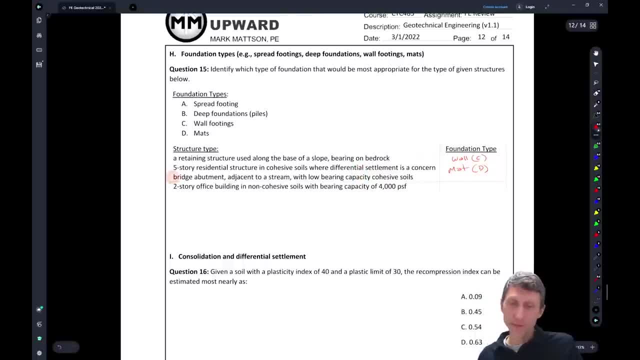 footing Uh, bridge abutment. if you've ever gone by, uh, where there's a bridge going up near where, where I live currently, and you see them pounding piles all day long. actually, they have another set of piles that they're going to put in in the spring And they're just sitting there, right. Why? Because 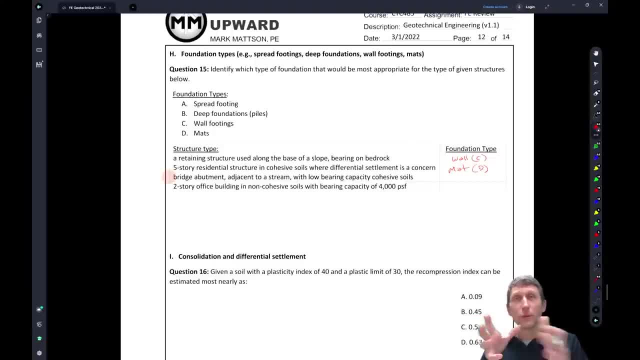 you get this big bridge span. This is on a little area and you want to distribute that load. A lot of times also, uh, near a stream, you don't have the best bearing capacity. So you want to get down deep to something good. So we'll we'll call a deep. you know piles here, Um, we'll use piles. 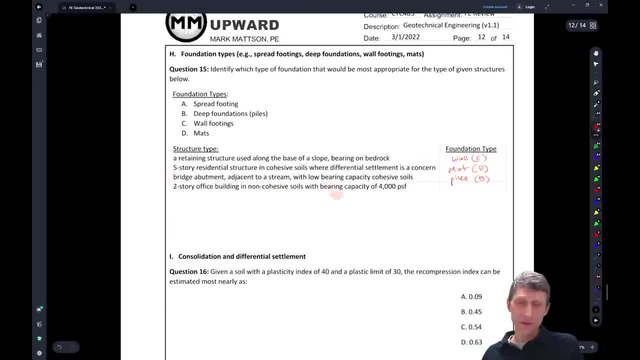 at a bridge. And what's that leave? It leaves a two-horse steward office building, non cohesive soils, bearing capacity to 4,000.. That's a pretty typical building, honestly. Uh, you know, if you get outside the city or outside a city, I mean a pretty typical building. couple stories: 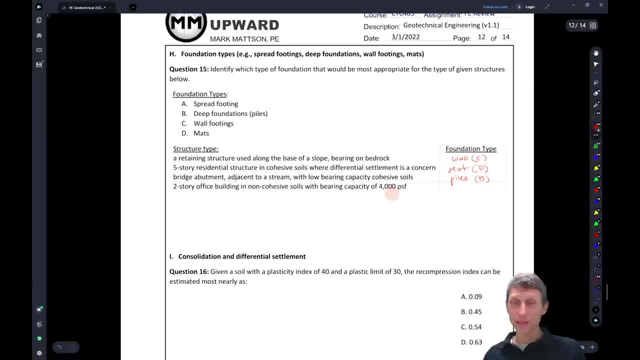 not too crazy, not huge, um, not huge footings, but this should work for you and you should get something where, um, you could use a spread footing here, Okay, So kind of a concept question. I wish I could spend more time on that, but let's just keep going. uh, today, Cause we got a few. more questions and I want to not stay up all night, but um, it's all good, You know. So let's keep going here. Soil plasticity index of 40, liquid limit of- I'm sorry- plastic limit of 30.. So PI again, we have a PI of 40, a lick a plastic limit of 30.. 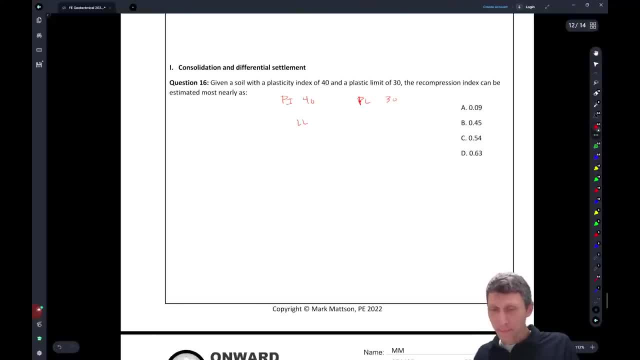 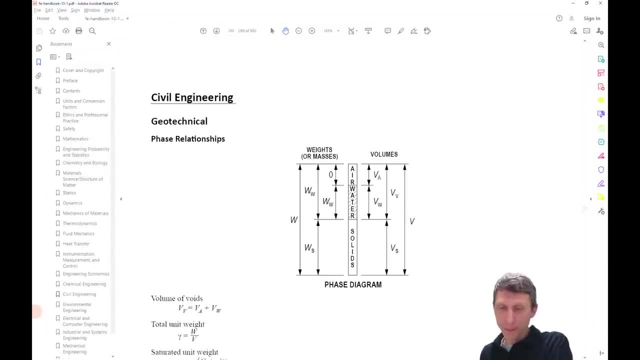 What's that mean? It means the liquid limit is going to be: uh, right, The liquid limit is the sum of those two, right? So if we come back to our liquid limit, what do we get? We get, um the the. 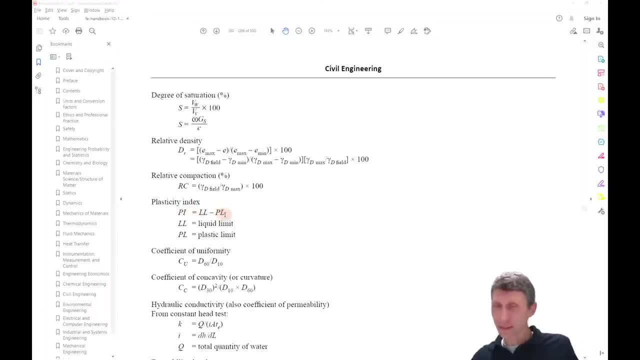 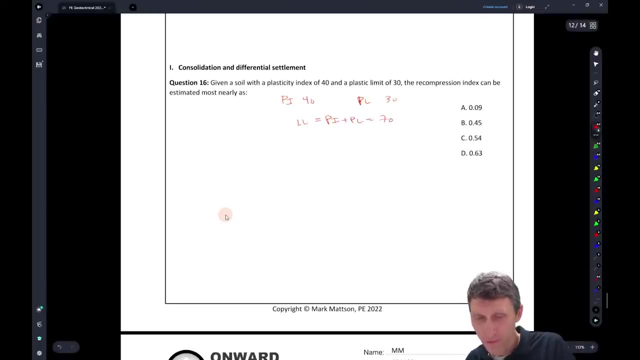 The liquid limit is the sum of the plasticity index and the plastic limit. So what does that mean? This means PI plus PL. That means our liquid limit is 70.. Okay, So this is our soil. The recompression index can be estimated most nearly as what? 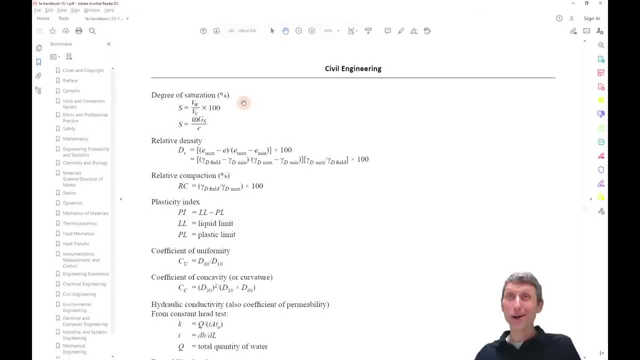 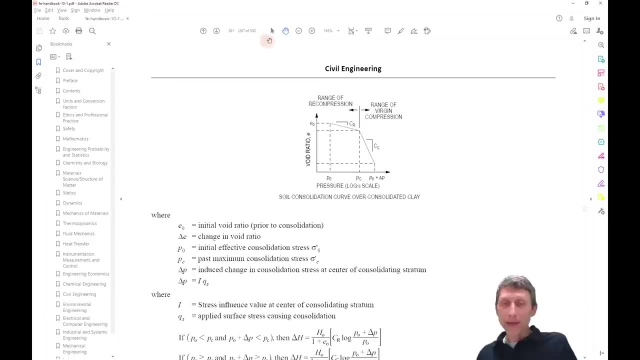 Well, what's a recompression index and what's a compression index, and what are all these pieces right? So, with clay soils or silt soils or fine soils, what we have here is a soil consolidation curve, and this gets into soil consolidation. 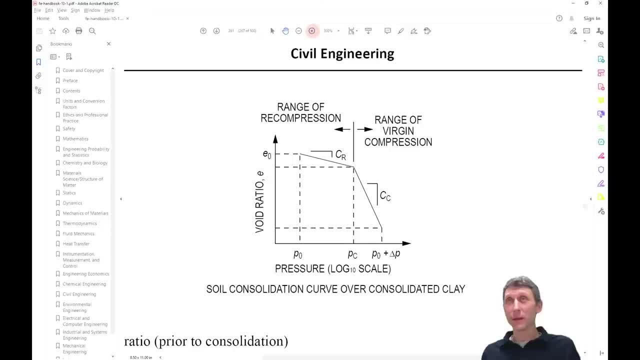 So what we have is basically, we have compression going on And if you think of it this way, there's. you know, maybe you had a soil that had like glaciers on it at one point and it compressed that soil. Well, the glaciers left and uncompressed a little bit. 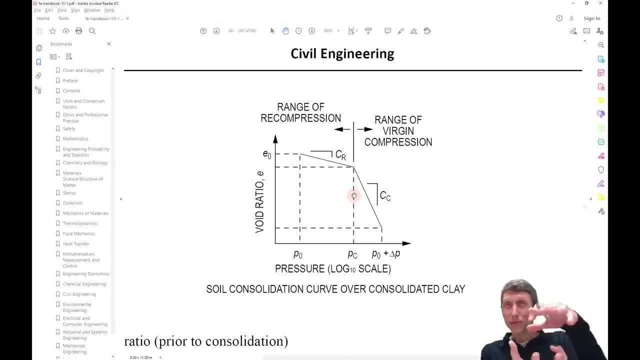 Okay, That would be like an over consolidated soil where it's already compressed Some but it didn't uncompressed all the way. Okay, Versus a virgin soil. Let's say you have a river that just deposits a whole bunch of clay and you get this virgin kind of, you know, this virgin layer that hasn't been compressed ever. 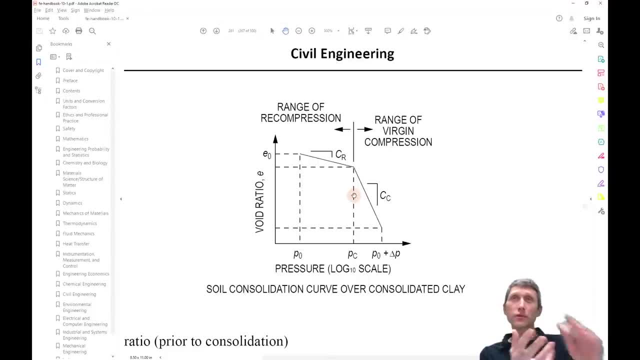 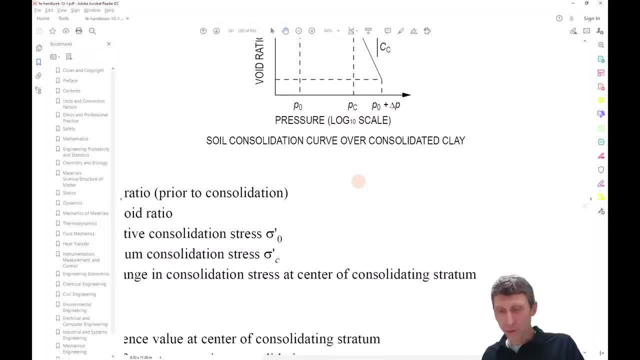 Well, when you first put load on it, it's going to go down quite a bit. Okay, So there's, there's virgin compression versus recompression. So what I'm asking you for here is: well, what's the recompression index? 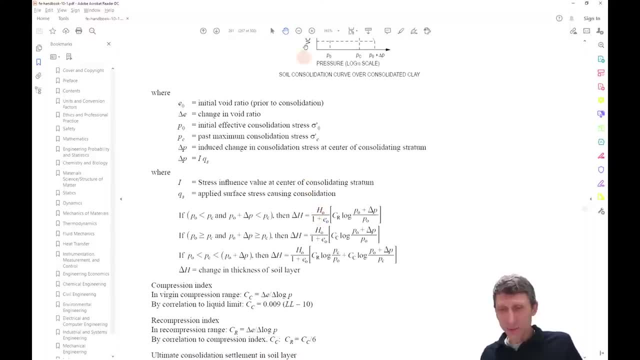 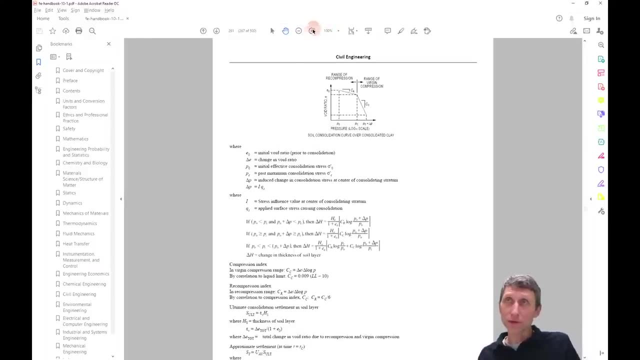 Okay, And there's a couple of different ways of looking at this And, honestly, when you look at this page at first In the reference handbook, there's a lot going on in here- and there really is. But what we have to take a look at is how can we get our answers right? 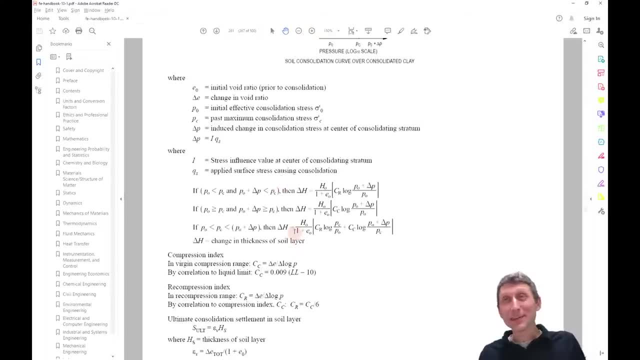 I mean on the test. that's what you want to know. Okay, And honestly, in the real world, that's what you want to know too, right, What you want to know is, well, what's this, this compression index with this, what's this recompression index? and to run these tests, to get void ratios and you know, delta, log P, and looking at those types of things. 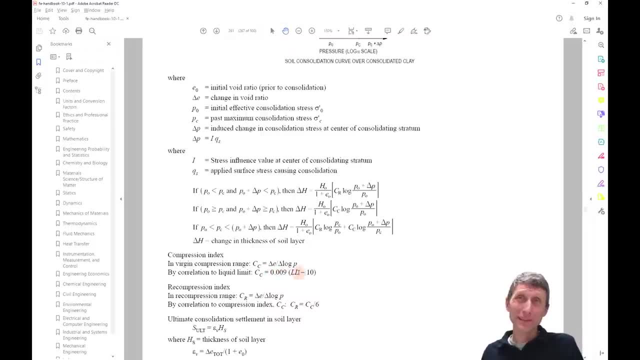 They'll take time. It's it's really pretty quick To get a liquid limit test And if you had a liquid limit test here, you could- you could- really quickly get an estimate of your compression index and recompression index, right. 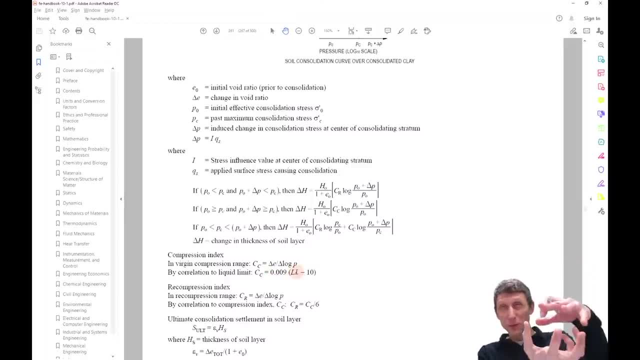 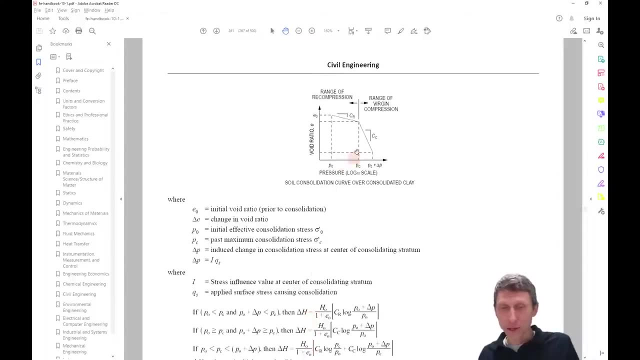 So typically your compression index is that first compression, where you're going to get a lot of compression, and your recompression index is that divided by six. So it's again: if we come back up to this curve, it's like your compression index. that's the steep part where you're getting a lot of compression right. 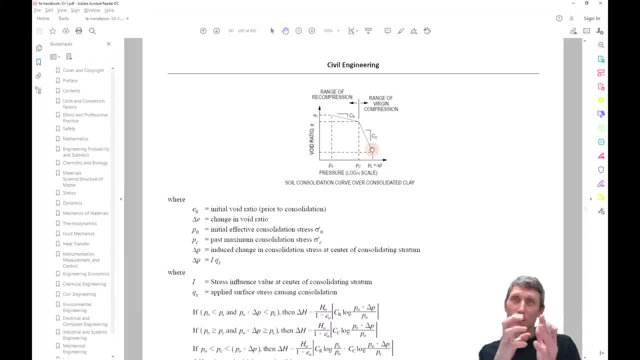 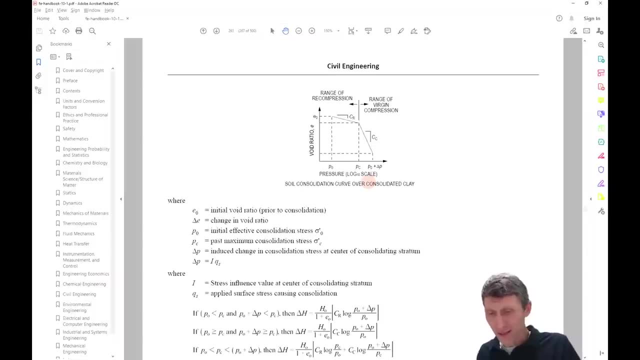 The virgin compression right away, And the recompression is where you're getting old It's, it's already compressed some, So you're not getting quite as much, Okay, So let's look at that And basically, with this one not not a crazy problem. 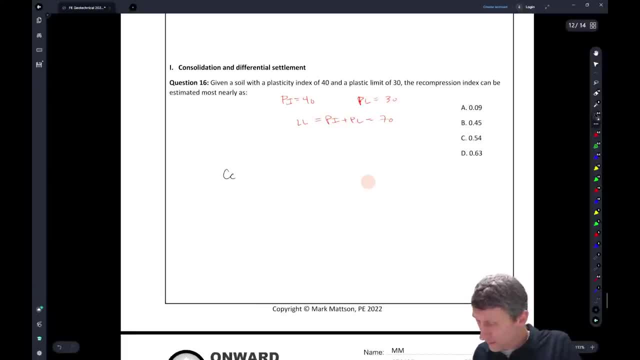 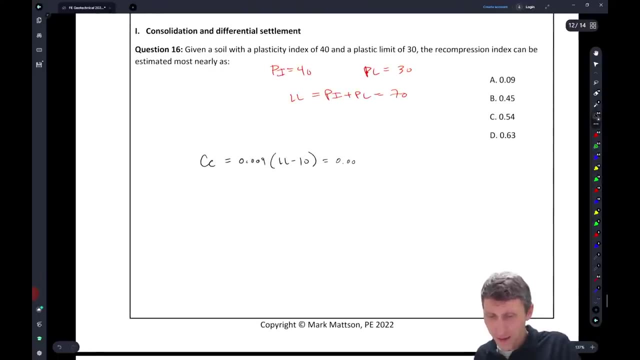 This one's actually pretty straightforward, but CC did, I did. I write that down right. CC is can be estimated as 0.009 of the liquid limit by minus 10.. So that's going to be. this comes from Terzaghi's, one of those you know icons in the soil world. 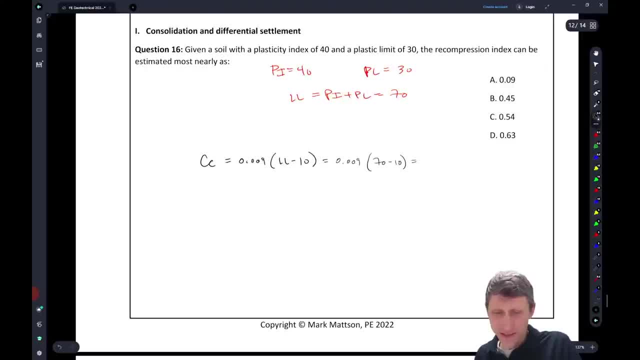 But what do we get? 70 minus 10.. So this is 0.009.. Times 60. And I think that's 0.54.. And if we take the recompression index CR, this is going to be estimated as CC over six. 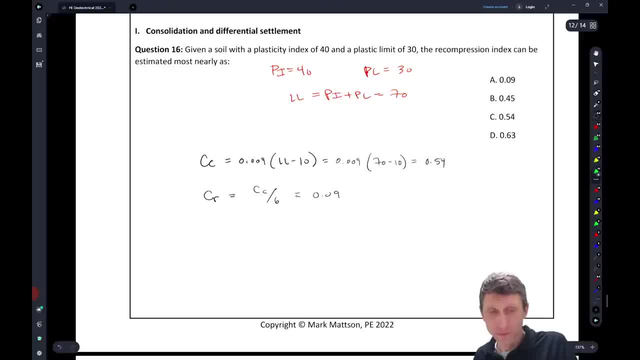 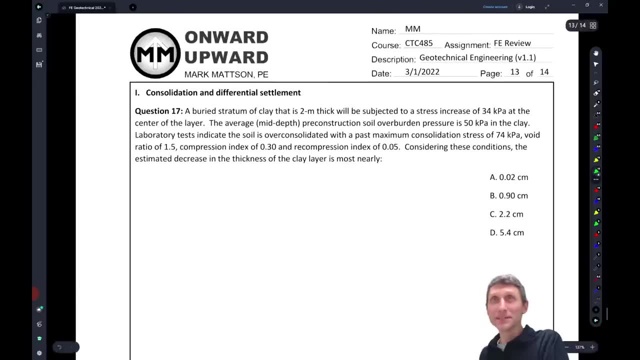 And that's going to be 0.09.. Okay, So that one's pretty good. Just a couple more. We got a couple of you still hanging on, So we'll see. I mean, you can always come back to this later too. 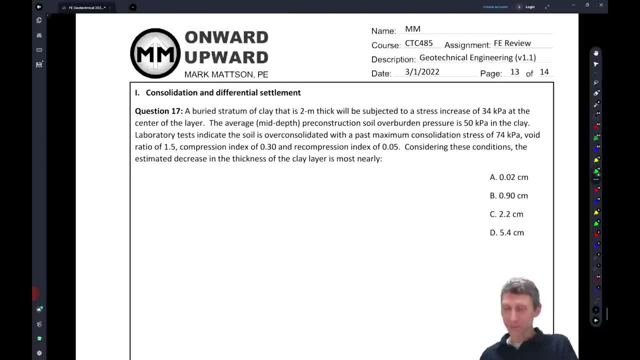 But the good news is we're making our way. We've only got a couple more problems and then we'll be done. So let's look at this one. We have a buried stray- I'm sorry, buried stratum of clay. I'm two meters thick. 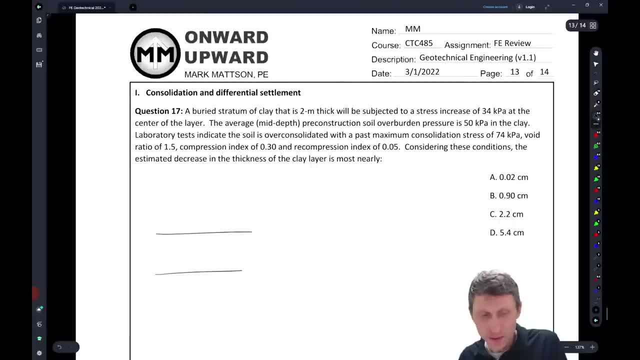 So we got this, this clay layer that's two meters thick and it's buried. Okay, Two meters And it's. you know, maybe what we have is we have some good soils above it that we that are already compressed, or maybe this was fill on top of it, or something. Okay, We have a stress increase here, So we have like a stress increase of Delta P. Okay, So we have a change in pressure of 34 KPA and at the at the center of the layer, the average mid-depth pre-construction pre-construction soil overburden pressure is 50 KPA. 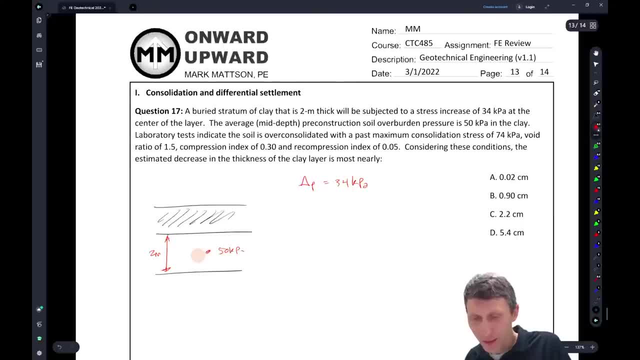 So we have got a. we got like a 50 KPA. We got an average stress there and laboratory tests indicate this is over consolidated. So it's already been consolidated but we haven't. you know, the pressure is less than what the consolidation stress is. 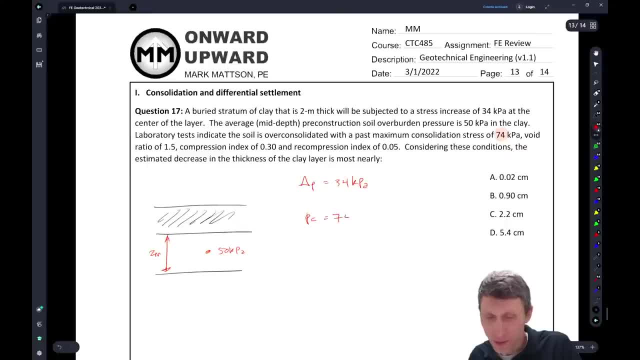 So we got 74 KPA. So that's our PC, That's our 74 KPA. avoid ratio of E is 1.5, D a compression index CC of 0.3 and a C R recompression index is 0.05.. 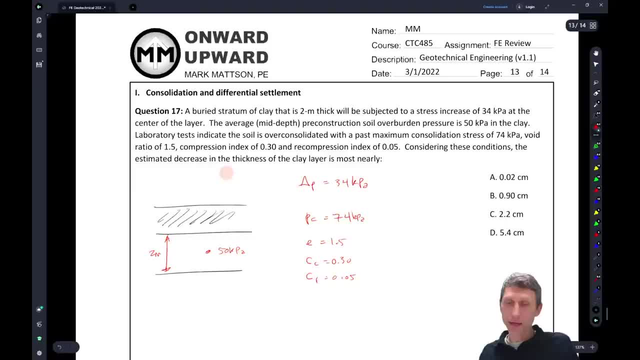 Okay. So, considering these conditions, the estimated decrease in the thickness of the clay layer is most nearly So. this is a consolidation problem, right? We're in consolidations, differential, differential set up settlement. So that's where we're at. 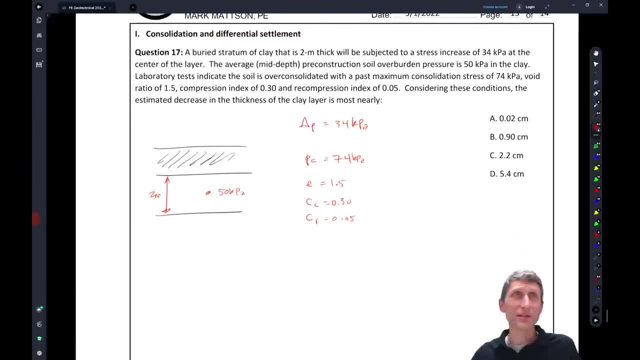 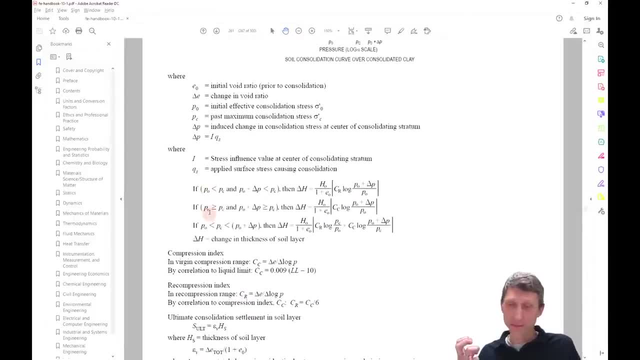 And this is kind of honestly. it turns into plug and chug. It's a little bit intimidating at first. Honestly, there's a lot going on in here, But what do all these P's, P, knots and PCs and all these things mean? 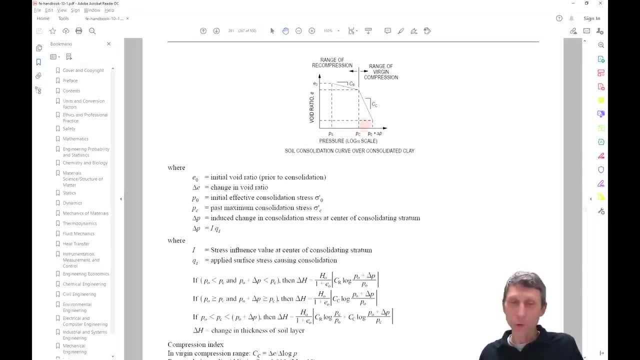 Essentially what they mean, though, is it's kind of like going back to this curve. Where are we? The 74 is kind of this layer, this, you know, this is the pre-cons, or the um, the maximum pass, consolidation, stress, the PC right. 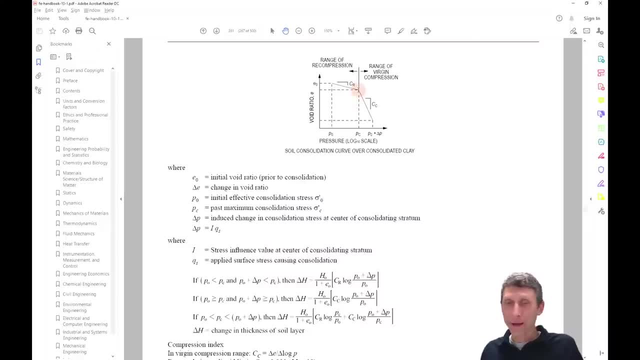 That's, that's this value. We're starting At, uh, a value of what? 50, but we're going up 34.. So we're kind of like straddling this point, if you will. So if we come back here for a second, what does that mean? 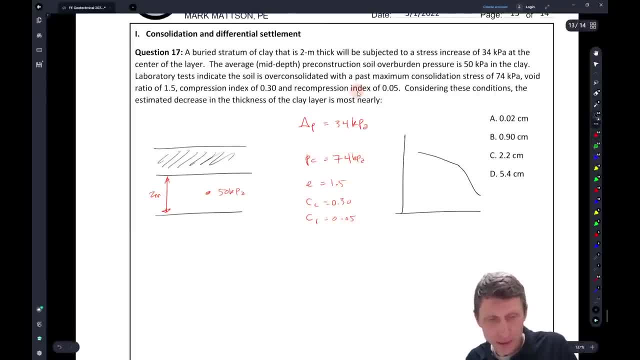 It means, if we have this curve here and we kind of have one of these things going on, right, What? what it means is we're we're at 74, that's our PC, right. We were starting at 50 and we're going to go up. 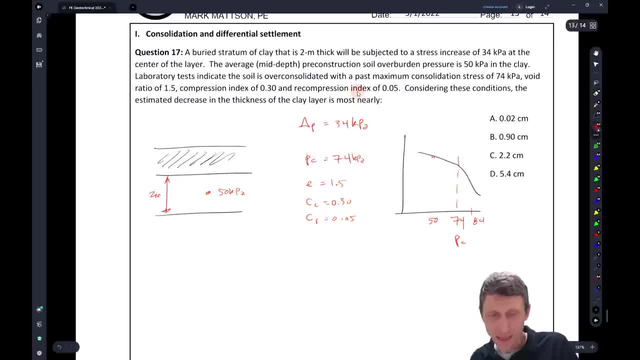 Well, what's 50 plus 34,? 50 plus 34 is going to get us to 84. So so we're Going to have some settlement that's in the, in the recompression, And then we're going to have some settlement that's in the compression. 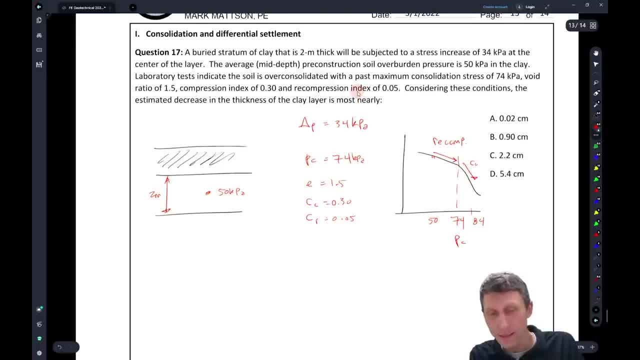 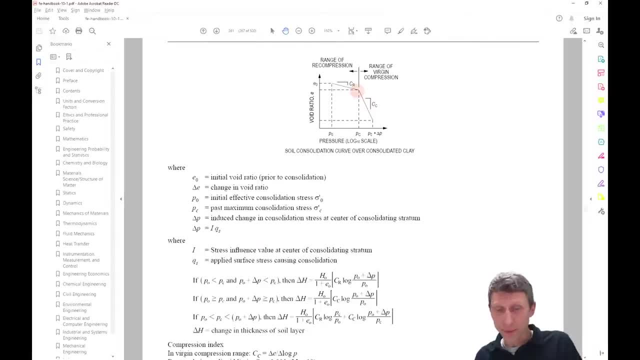 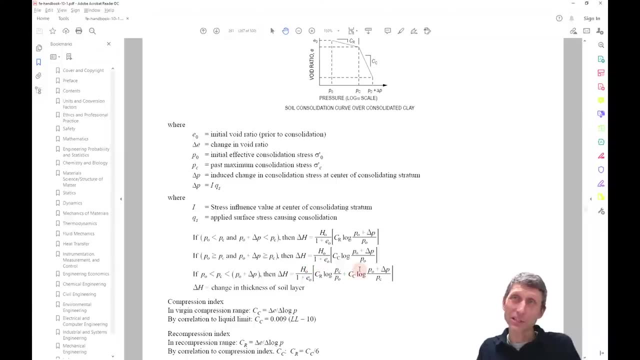 So this is recompression and this is the compression. Okay, So what that means is it tells us which formula we have to use, And that basically brings us down to here. right? So what all this means is, essentially: we have to deal with the recompression and the compression. 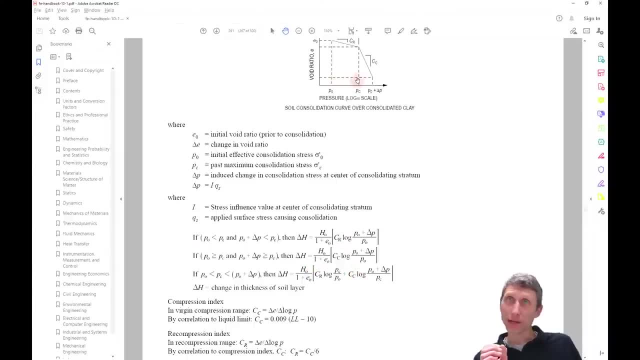 Okay, We're not just in the recompression phase, We're not just to the left of it, We're not just to the right of it with the, The, The verging impression, we're in both of them. So we have to use the big, long formula here. but the good news is, even though it's a big, 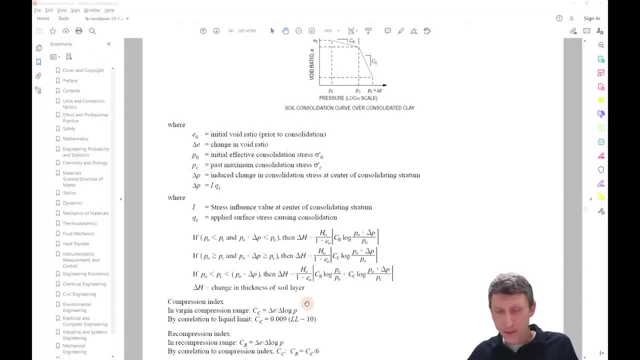 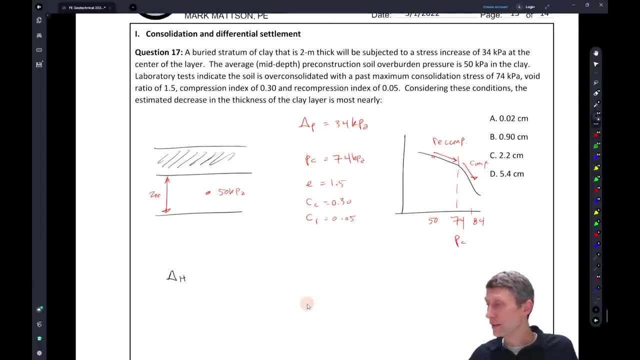 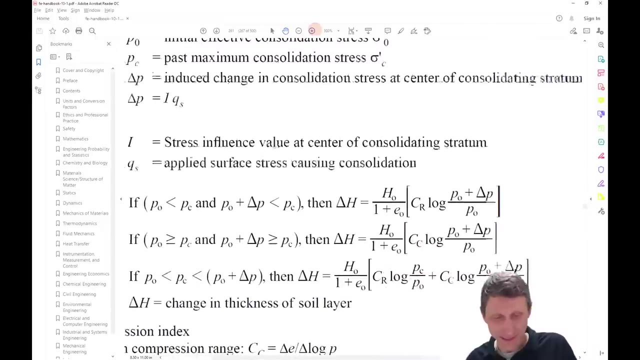 long formula. it's just a plug and chug formula, So let me try to write it down here: Delta H equals equals what? Let me? actually, this is a long formula here. I think I might be able to copy this in just because it's so long. 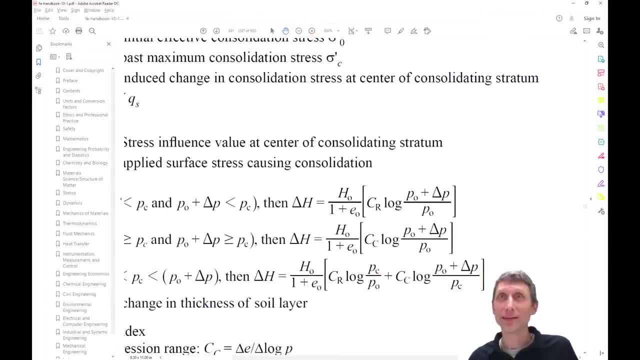 Let me try that here. Hold on a second. I tried it last time. It didn't work. I think I've got a better way of doing it here. So let me, let me look, and maybe I can just do this. I don't know. 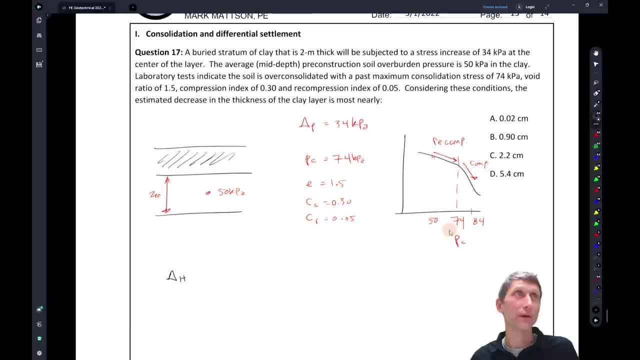 That work. Um, maybe the snipping tool come to my rescue here and I can. I mean, wouldn't it be nice? Oh, look at that, It's perfect. So it wouldn't be nice if you just do that on the test too. 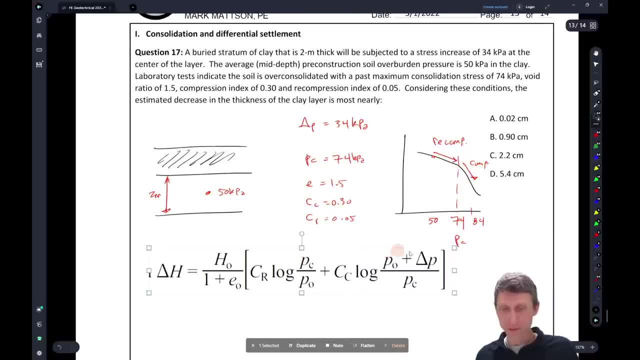 Um, that would be so awesome installer, but you know, sometimes it's not that easy. So let's, uh, let's, let's take a look here, Let's do our plug and chug and make it work, Okay. 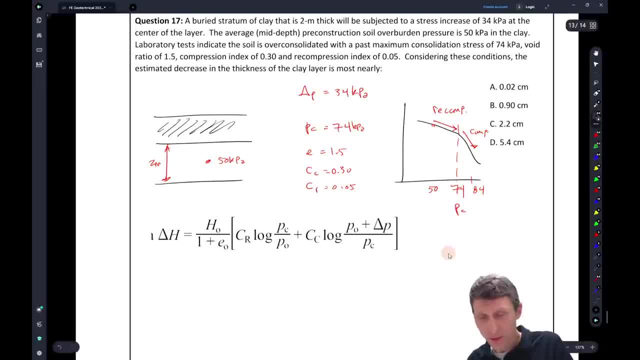 So what do we get? We got our our layer of two meters Over One plus 1.5.. That's our, our. our void ratio, CR was 0.3, the log of PC. So PC 74 over peanut, that's 50 plus CC, which was 0.05.. 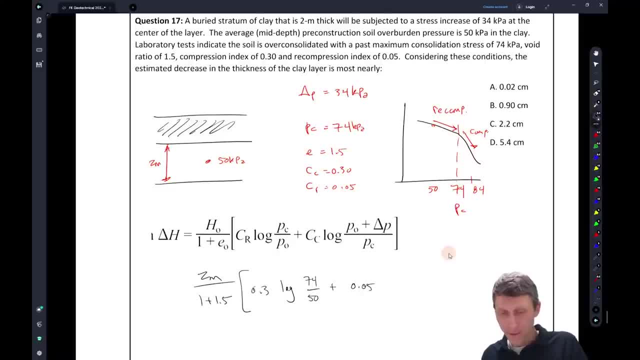 That's the virgin impression of of what of? uh, peanut plus Delta piece. That's our 84 over uh over 74.. Okay, And I I got to write my log in here to to make it right. 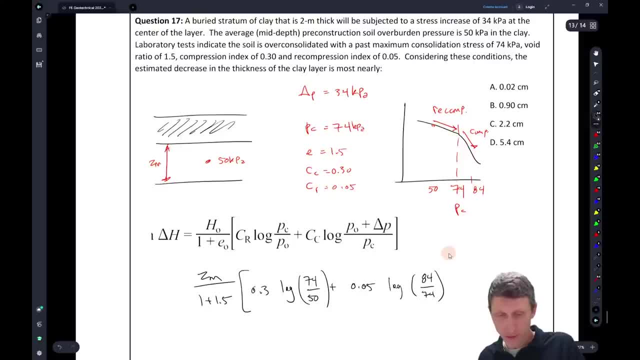 Okay, So that's my log and we plug all this in. You have to be careful, though, because what do we ask for the units up here? Meters we've got- uh- or I'm sorry, So you know it's up up top- or centimeters units over here are meters. 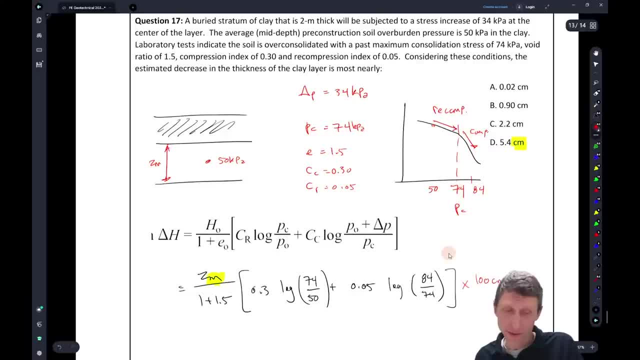 So I need to multiply by what: A hundred centimeters per meter. right, The meters cancel out and I'm left with centimeters. So if we do all that, I believe the value that we get here is going to be this: 2.2. 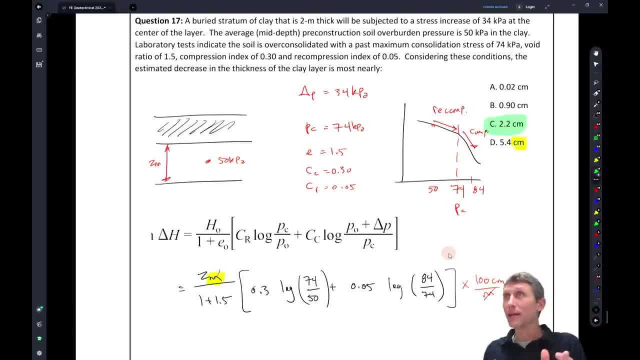 Okay, So again, consolidation. you got to understand that consolidation curve a little bit. but I thought this: I liked this problem. I kind of tailored it so that you can kind of be on both sides of that, of that um. 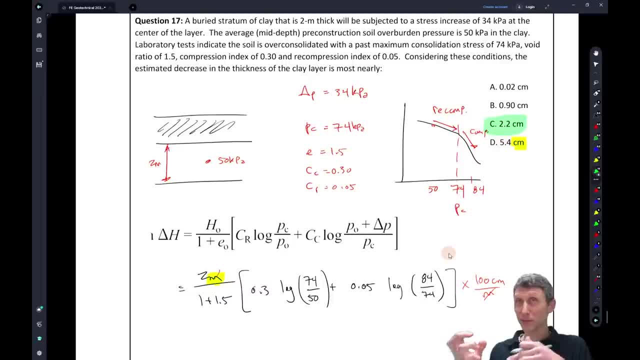 maximum consolidation stress. So you can kind of get an idea of the recompression versus compression uh side of the curve Right. So you know we've got what's this. This is the um, this is the recompression and this is the compression right. 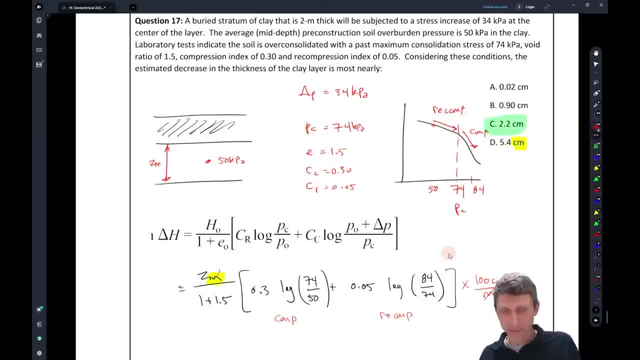 So they're both sides, Or did I flip that? I think I flipped it. but I'm sorry, I flipped it, That's okay. So the, the, the, oh no, I just typed my numbers and I put my numbers in wrong. 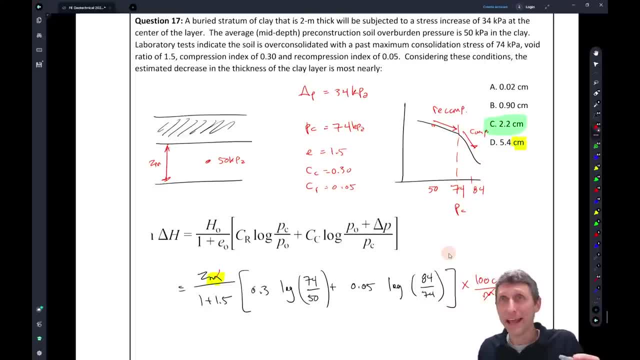 So somebody is going to yell at me here If anybody's even listening, I don't know. Maybe I'm just talking to myself, right, I plugged in wrong here. CR is is 0.05.. Right, Yeah, That's the 0.05 here. 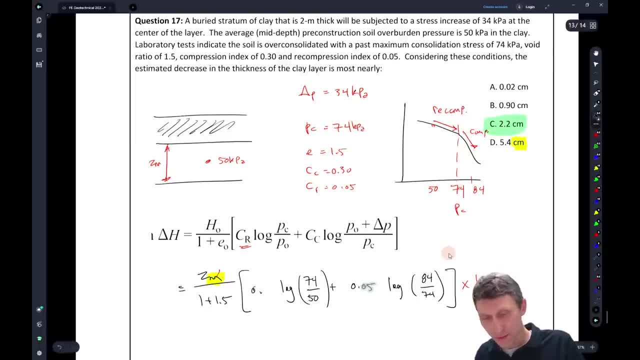 Okay, Um. so let me fix this here, Cause I cause somebody is going to yell at me 0.05.. That's the, that's the. now, I got to plug this in to make sure I did it right. 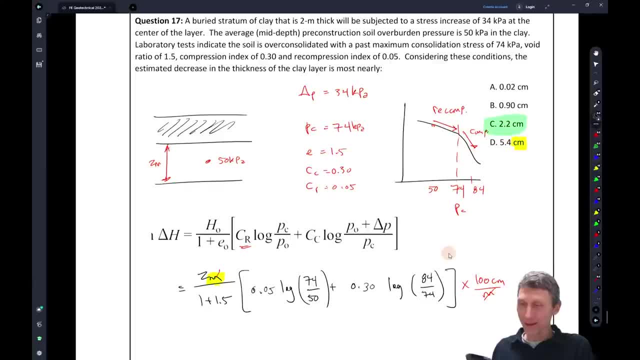 So let's just do it: Two divided by 2.5 times, a hundred times What? 0.05. Times the log, Um the log. to get the log on a T a 36 X, you have to hit it twice. 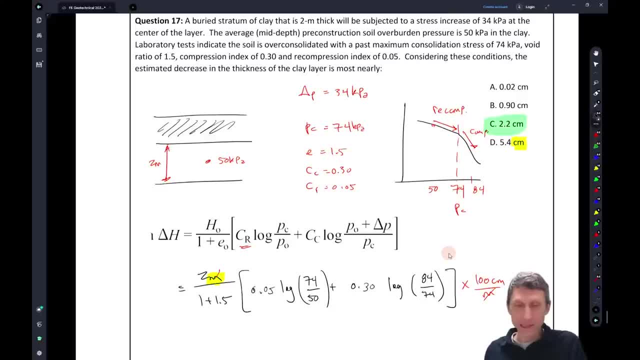 Um 74 over 50.. Yeah, That makes. that makes sense, Cause the 74 is the maximum pre consolidation and the fifties where we started. So that's the recompression range. Uh, okay, That's good. 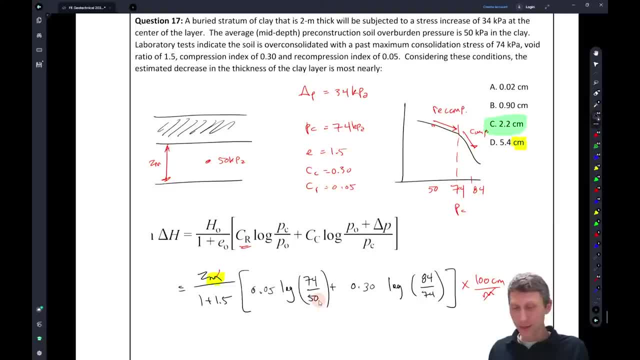 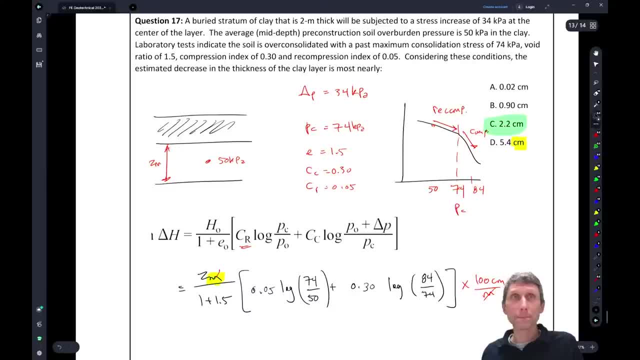 Uh, let me just make sure I did it right here, Okay, Um, so there there's man. this is almost. this isn't quite as bad as my original statics one, but, um, I did make a mistake. 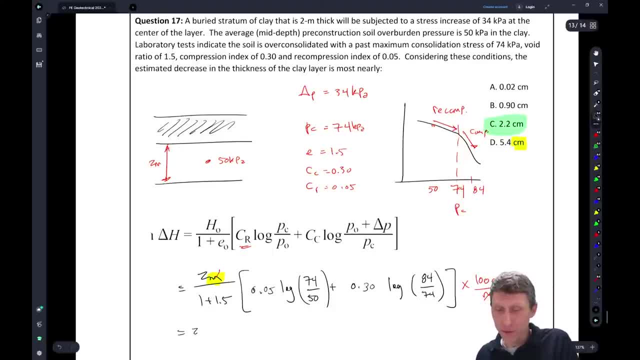 Um, this actually gets closer to about 2.2, or, I'm sorry, 2.2.. 2.0. And what I originally had in my notes was 72 kPa, So two or 2.0, it's still going. 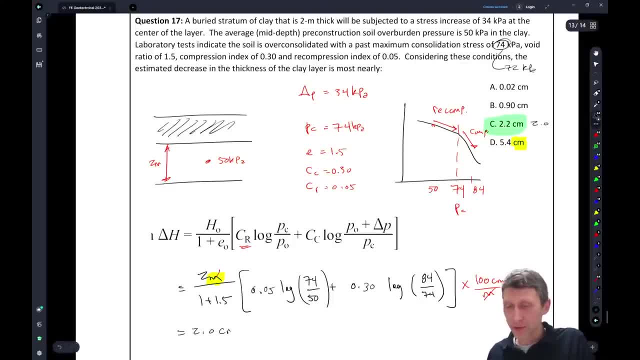 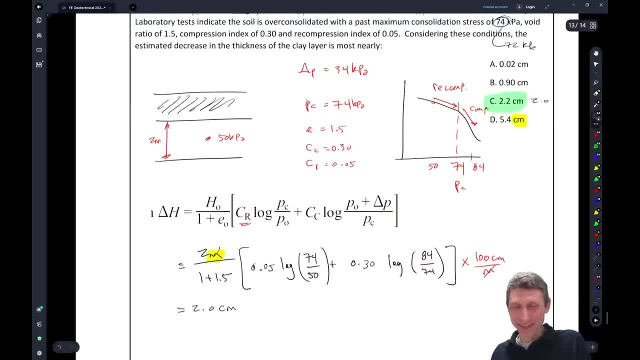 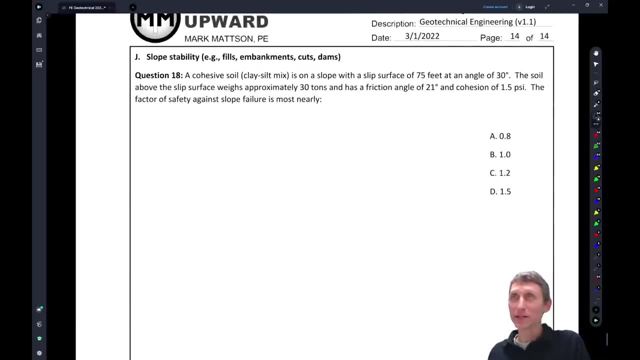 to be the closest one, But this actually gets to about 2.0 centimeters. All right, two more questions and then we're done. One of them is a conceptual question, But let's take a look at this one. This one is a is kind of a plug and chug question, But I like this. 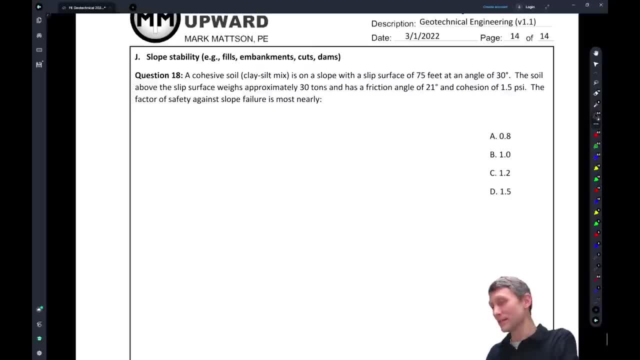 question because it brings us back to statics And so much of this. this, this test is if you can understand statics, but what we're given is a cohesive soil with what do we have with on a slope? we have a 30 degree angle here And we got you know this, this, this. 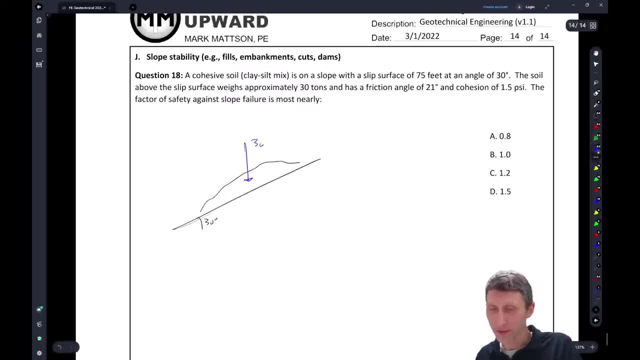 soil mass, that's. that's essentially 30 tons, right, 30 tons up here, And we have a length, this slope of 75 feet. Is this thing stable Or is it not? What's the fact? There is safety here, Okay. So what we have is is is we can go through and we can look. 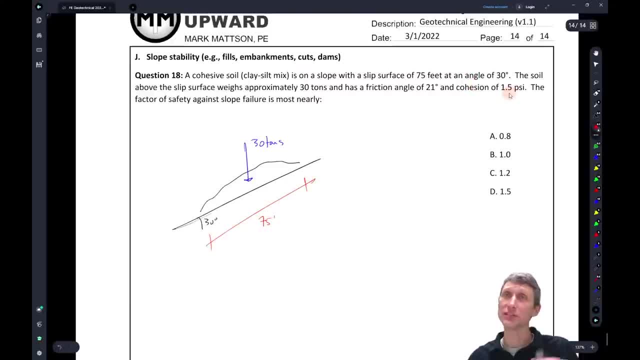 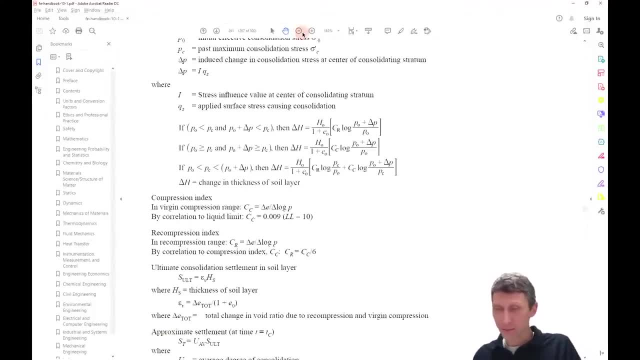 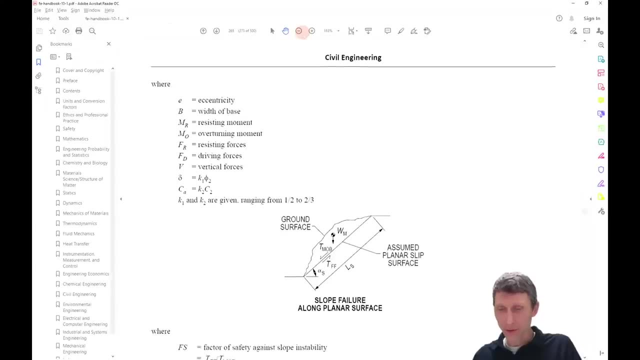 at this. But here we do have some cohesion, So that cohesion is going to add into our factor safety. But if we come back to our our reference handbook here- and I can't remember which way it is, but let's see if I can find it here- So we're looking at slope stability. 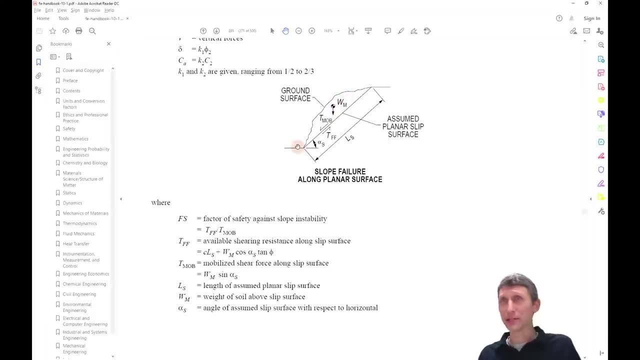 right Slope stability. here we've got this mass kind of pushing down And what we have to do is we have to take that mass And we have to look at what are the resisting forces, what are the mobilizing forces, and then come up with a factor of safety. 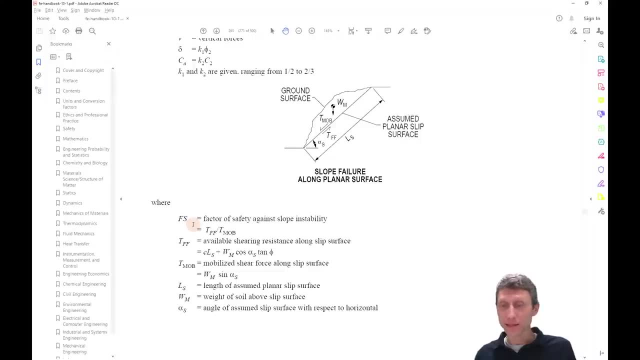 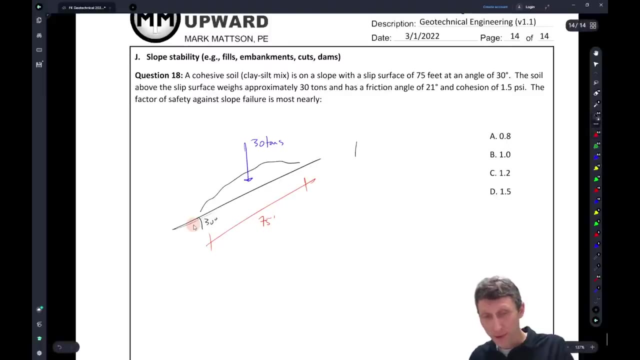 So our factor of safety is going to be: it's going to be, it's going to look like this: right, Our factor safety is what we're trying to solve for, But our factor of safety is going to be: what are our forces resisting, divided by our mobilizing forces? So we're 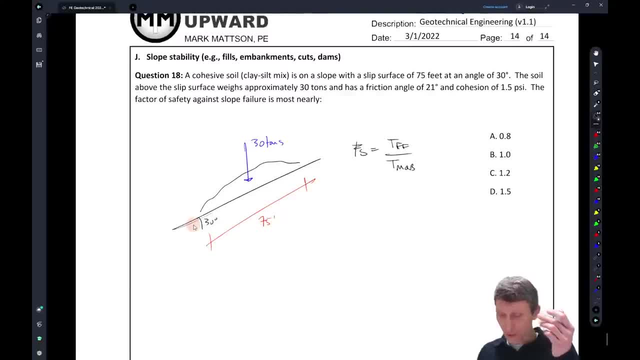 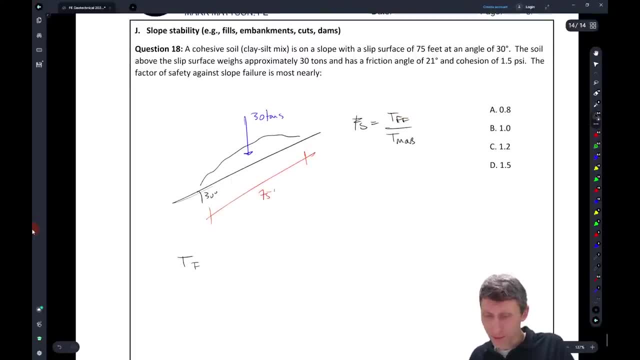 going to look at our mobilizing forces. So if we can get each of those, we should be good. So what do we have? Let's start with the, the resisting forces, the friction forces and the friction forces here. If we come back again, this is where it comes a little bit. 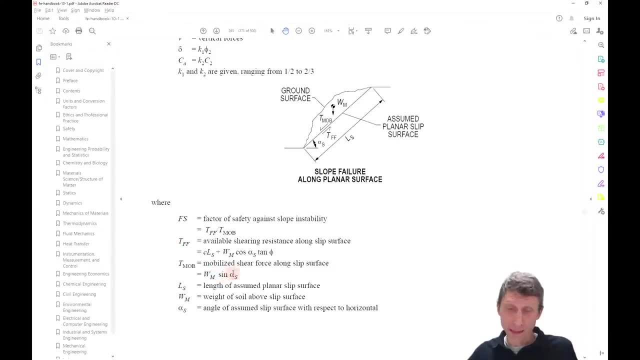 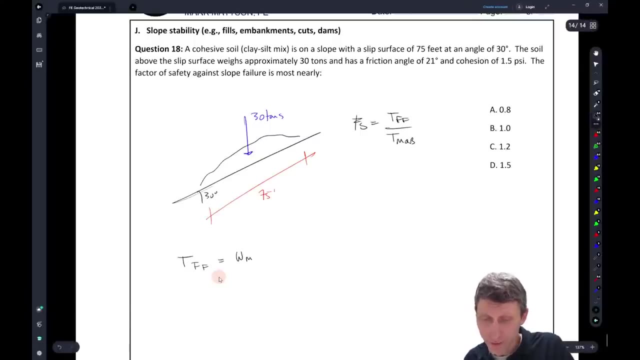 of plug and chug, But I did want to look at this because I it's on here. But what do we have with the weight times, the sine of alpha? Okay, so we have the weight of the soil, mass times divided by times, the sine of alpha. 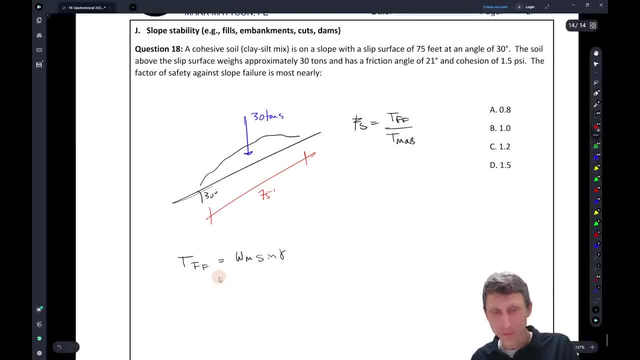 And if you think about this for a second, what do we have right? If you think about this, we have. this is going to have some component that's normal and some component that's perpendicular to the slope or parallel to the slope- normal and parallel to the slope. okay, And if this? 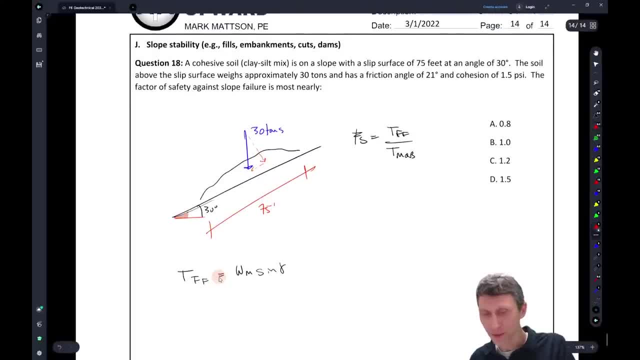 angle here is 30 degrees, right, so this angle here is 30 degrees, this angle here is 30 degrees. What angle? Or, I'm sorry, what's, What's, What's? What are we doing here? So this is what. this is what we're looking at. 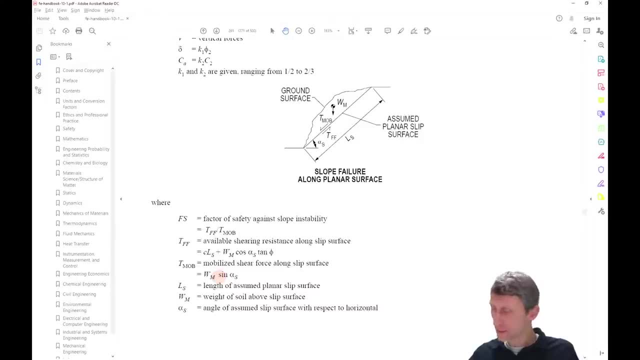 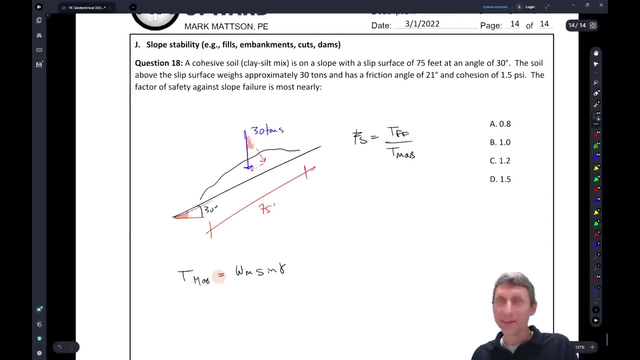 Am I getting that right? This is the mobilizing force. I'm sorry, this is our mobilizing force, Man, two hours is too much for me, I think. So we get our mobilizing force. I was just thinking like that's our mobilizing force, because why? this is the sign of 30, right? 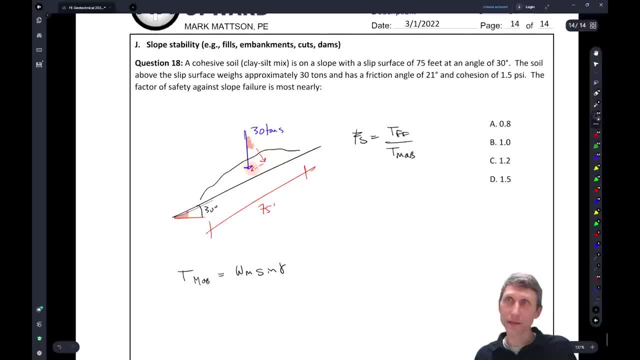 The sign of 30 is the one pushing down. it's the opposite of this angle. that's not going to be our sign of 30.. I was thinking: like what I scrub, that's our mobilizing force. right, We're going to sing down the slope. right, That's our mobilizing force And basically. 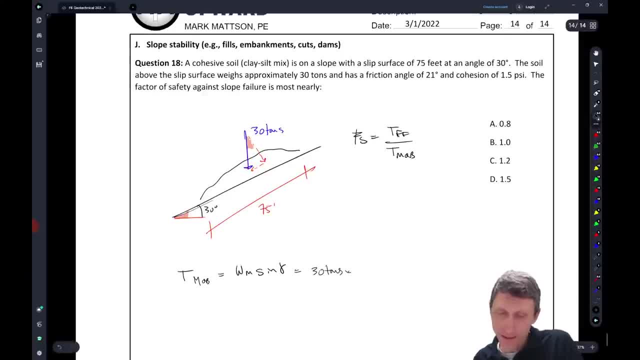 what all this is is just that 30 tons- And I like to convert this right away to kips because I don't like tons- So 30 tons times what two kips per ton equals, you know, times the sign of this alpha or sign of 30 degrees. So 30 times, two times the sign of 30, which 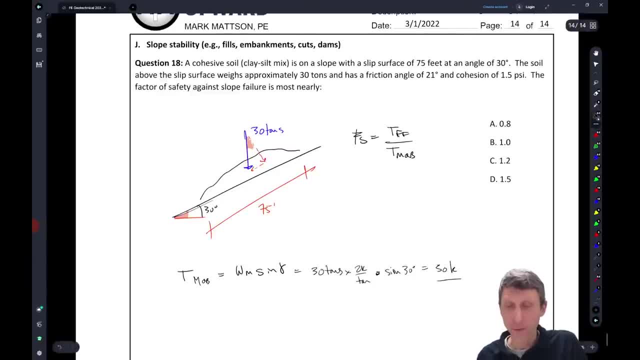 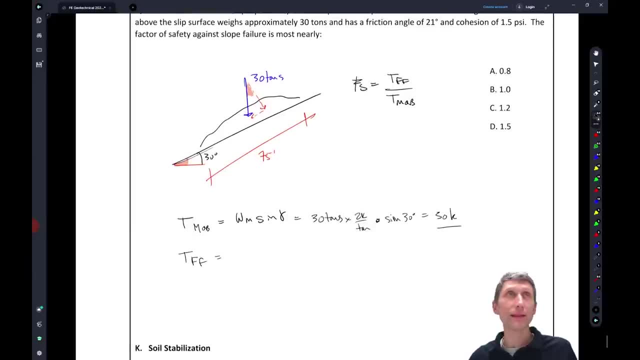 is actually one half, we get 30 kips. So 30 times two times the sign of 30 degrees, we get 30 kips of a mobilizing force. And what's resisting that? The friction force, essentially, is resisting that. In this, I like this equation. 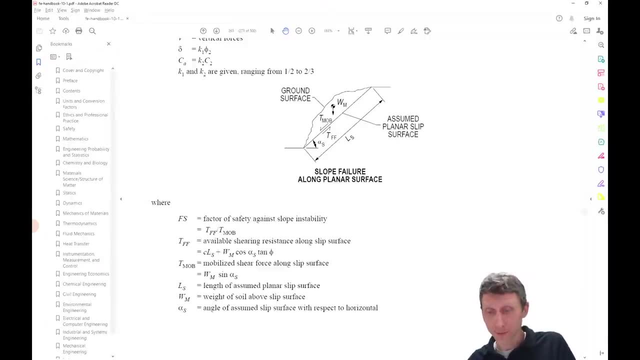 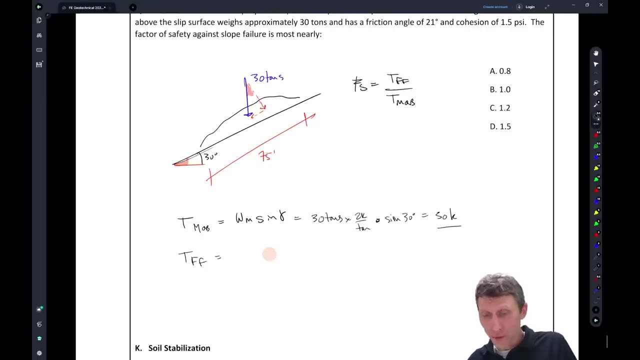 here because it again it makes us think of that friction problem. So if you know that friction about CLS, WM, cosine alpha, and then this tan phi is kind of like your friction factor, right? So what's this? This is CLS. that's the length of the slope plus the WM. 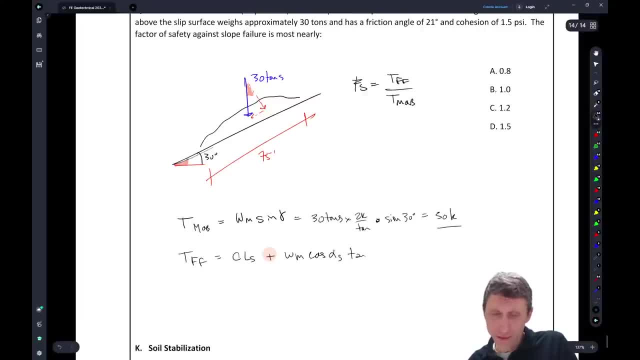 cosine alpha s times tan phi. Okay, so if we think of friction for a second right, we just said that we have this is kind of our mobilizing force: WM sine alpha. Well, we also have you know this force here, which? 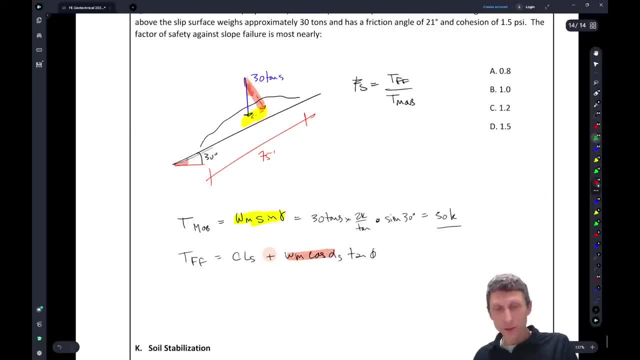 is kind of like our normal force, right. So if you remember friction, what's friction? Friction is a normal force. times mu, right. So that's kind of what we're getting in here. But then we get this, which is kind of like the glue or the cohesion that holds it together. 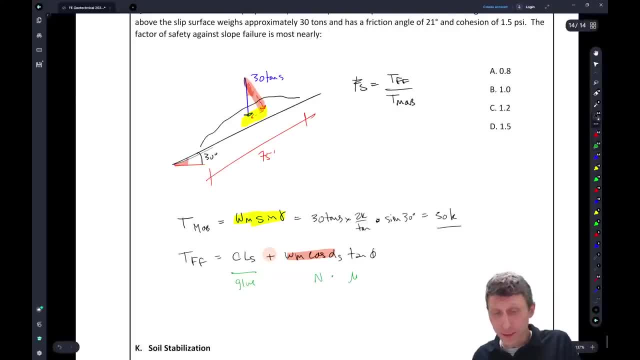 Okay, So that's one way to think of slope stability. So what's this? Our cohesion of 1.5 pounds per square inch- Yikes, we don't like pounds per square inches times 75 feet. So what's this? Well, what I'm going to do is I'm going to multiply by what 1000 pounds underneath. 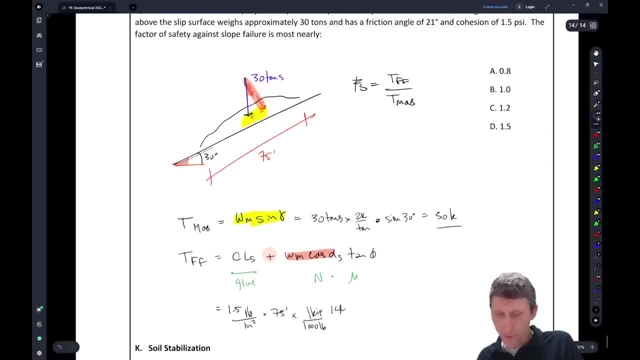 one kip And I'm going to multiply by 144 square inches per square foot. Okay, so that's my unit conversions And then, plus the, the weight of this thing, that's going to be 60 kips times the cosine of 30 times the tan of the friction angle. the friction angle is 212121 degrees And 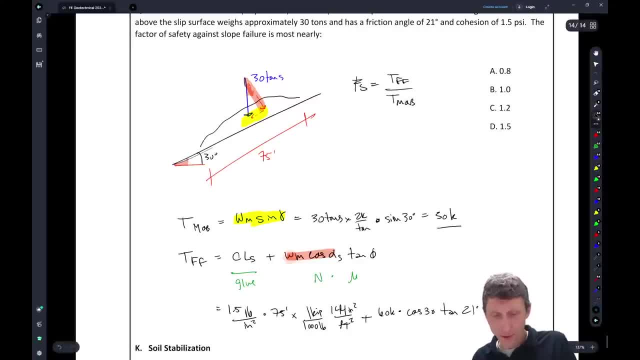 good news is I think that actually is an answer that we can calculate. The answer that I got was about 36.1 kips. So if we come back and take both of these values, we're going to be able to calculate that, And then plus the weight of this thing, that's going to be 60 kips times the cosine. 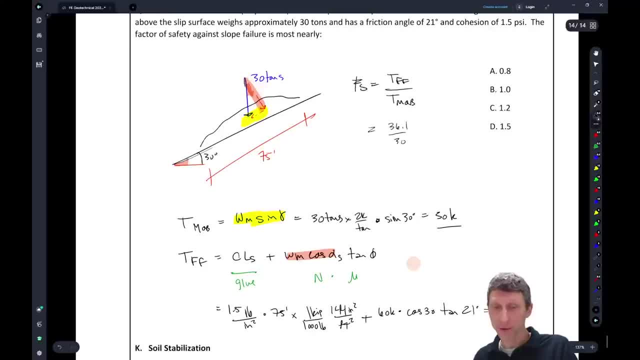 of the friction angle And we're going to multiply it by the new values, Our factor safety is going to be 36.1 over 30, which is going to equal. I think that works out to about 1.2.. Yeah, so I think we get about 1.2 there And we have a good answer, Okay so. 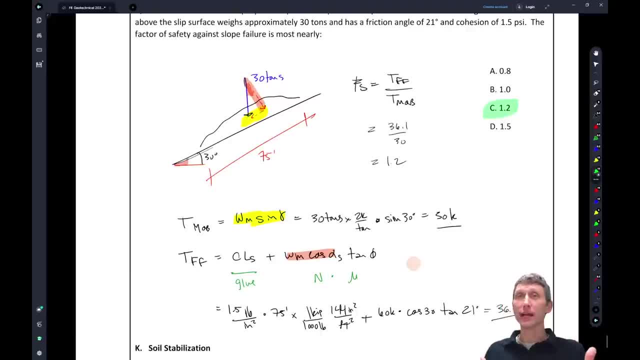 but again, I like this problem because it gets back to that whole friction idea of how do you do a block on a plane, right? I mean, we did this problem, I think, in statics or strength of materials, I can't remember which one, but it's a bad. Maybe we didn't do this. 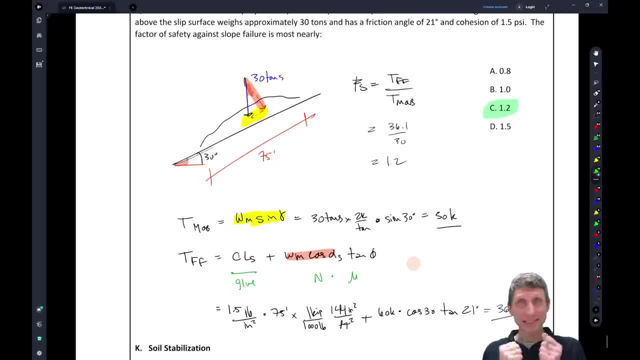 block on a plane, right, it's, it's, it's, it's so similar to slope stability, if you can kind of think of that. those angles, those force components, those vectors- uh, it's going to help you out there in solving this type of a problem as well. so last question- here it's a concept question, and then 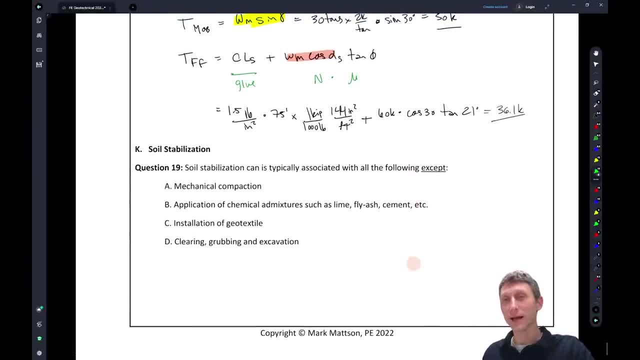 we're done for the night and that's good, because, um, i'm just losing ground here, sorry, there's another bad pun. okay, um, i'm digging myself into a hole. um, sorry, i, i'm trying, i'm trying, i'm really trying here, but um, what do we have? question 19: soil stabilization. last thing here, uh, you know. 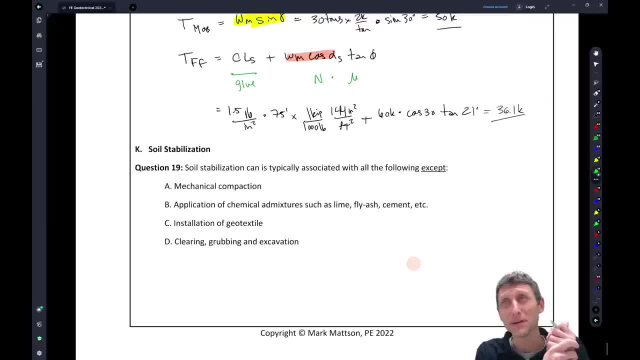 there could be some, i don't know. maybe there's going to be a numerical question, but i think this is probably more of a concept question. with, with, when you get into erosion sediment control, it becomes huge on job sites. i mean, i've seen more, uh, more silt fence put in, wrong probably, than right. 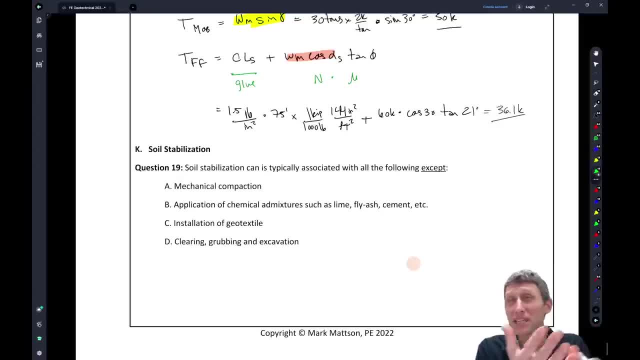 in my life- silt fence is one of those things that never gets put in right. but erosion sediment control- maybe that's going to be on there. i mean just hay on a you know or mulch, and probably not hay, but straw on a on a you know. straw mulch on an empty site cuts so much down on erosion right. so here the question. 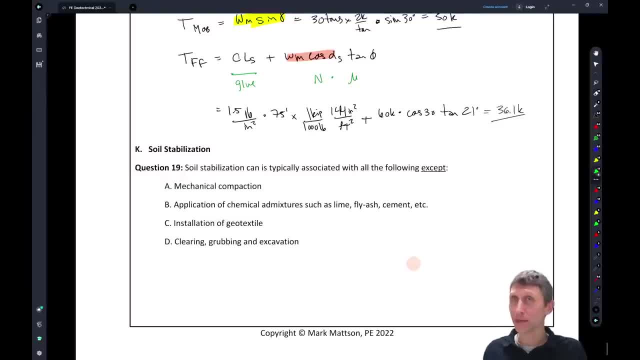 is: how do we stabilize soil? what are some ways we can stabilize soil? um, typically it's associated all of the following except, okay, mechanical compaction. if you compact it, make it denser, it's going to be less like less susceptible to wash out. that's okay, that that does stabilize. 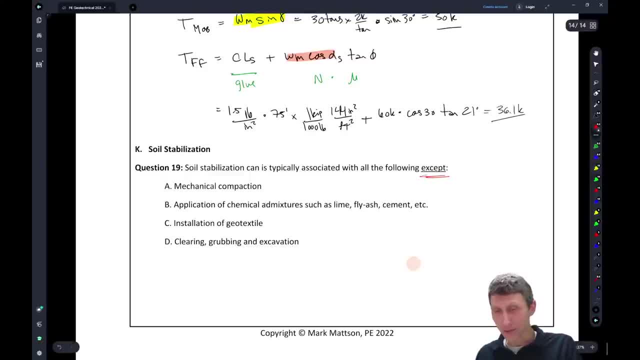 the soil. so, uh, it's, it's. we're looking for an accept here. so we're looking for a not chemical add mixtures. well, if i add some glue to the soil- not really glue, but let's say, like a cement, for example, if you put a binder in the soil, you can hold it together. okay, that's gonna provide soil stabilization. 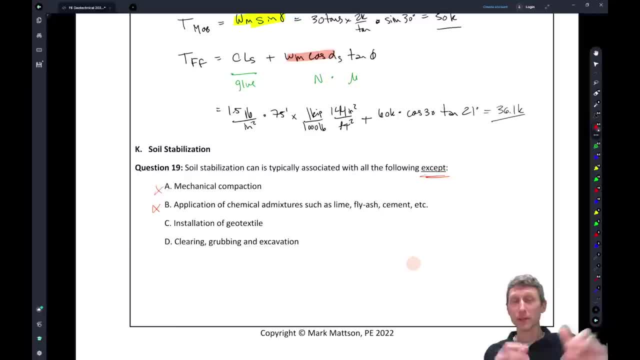 geotextiles. a lot of times geotextiles are put there just to distribute loads and stabilize soils. so again, not there. clearing, grabbing an excavation- that's typically the first thing that's done on a site after erosion, sediment control, you know, are put in appropriately to. 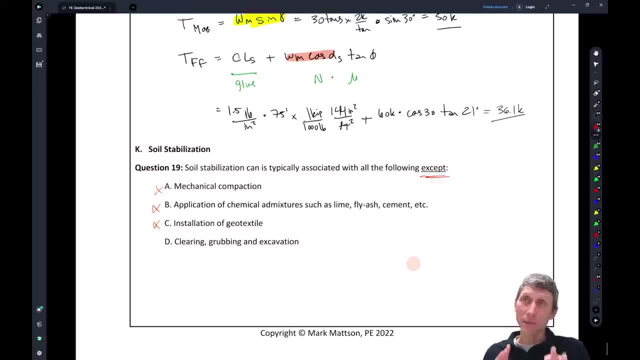 protect all those waters that you want to protect in the wetlands and all that stuff. But the clearing, grubbing and excavation is what rips up the soil, It takes away the vegetation, It takes away the trees And that opens it up and exposes it. 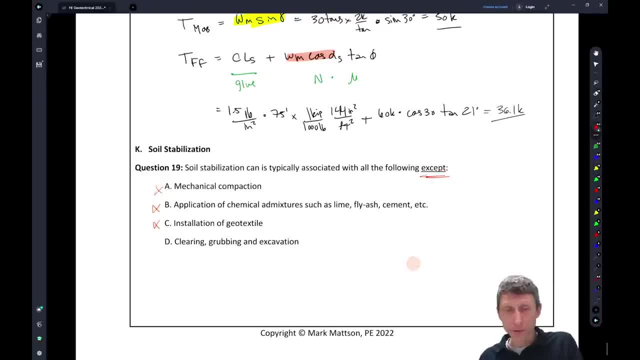 So if you get rain, it gives it the potential to wash out, So it can be associated. Soil stabilization can be associated with all of them, except for really clearing, grubbing and excavation. There are smart ways of doing excavation, But typically this is what's going to cause your soil to become unstable- is when you do clearing, grubbing and excavation. 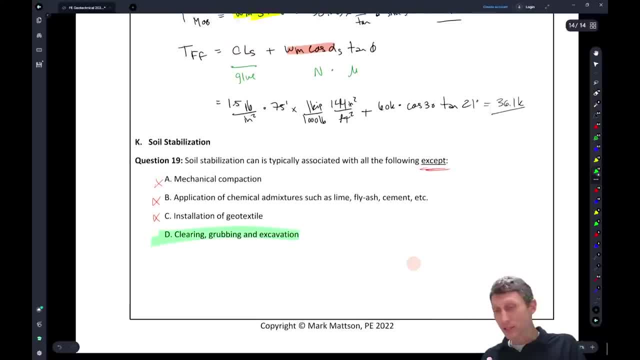 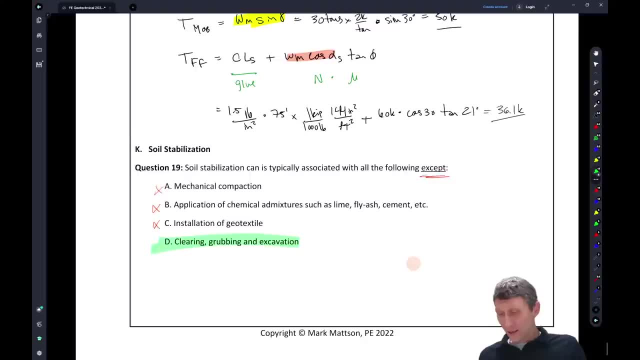 So, man, that's it, That's it, That's it. We got no more questions, We're done. And man, this was probably the longest one yet I thought it was going to be a little bit quicker with some of those questions, the concept questions. 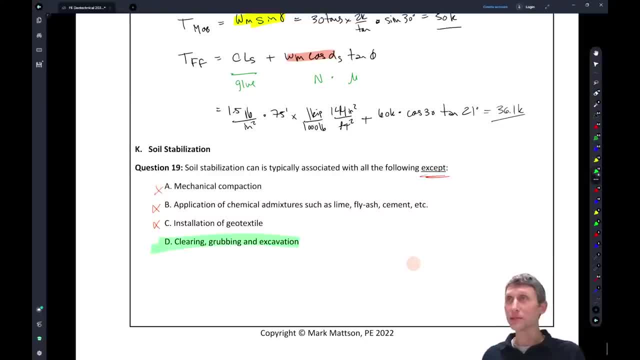 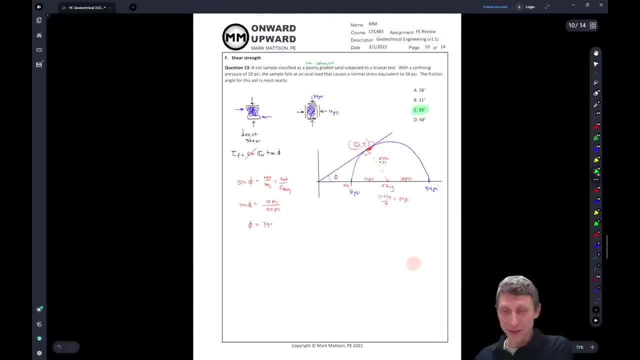 But we made it Okay and hopefully on the test you're able to make it as well. Uh-oh, Man, now you're going back to question 13.. Uh-oh, let's go back to question 13.. 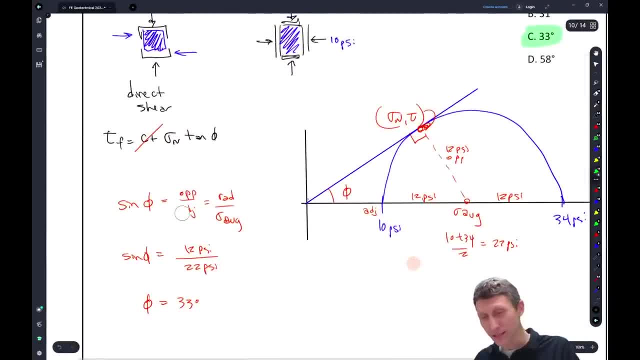 What'd I do? Zion is: oh, good grief, You are so right, That's totally what I did is I did opposite over hypotenuse and I failed trig 101.. So thank you so much. I so appreciate that. 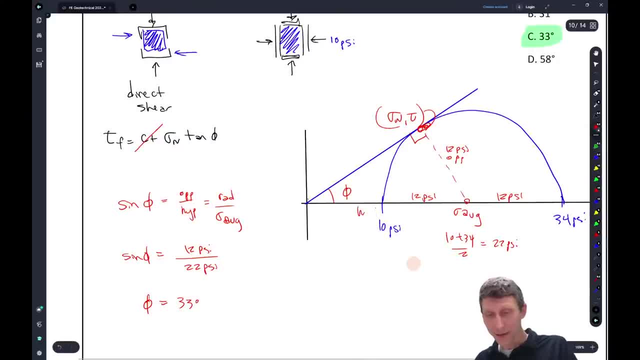 Yeah, opposite over Man. I don't. This is the hypotenuse right. So if we look at this right triangle, this right triangle, it's opposite over hypotenuse Man. I'm so thankful for that because that's going to come up in a comment below. 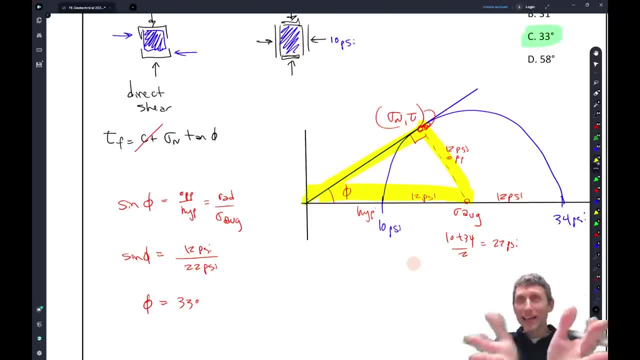 Somebody's going to be like: but you don't even know, trig, I'm going to be like, you're right, I screwed it up, But you know, You know, I'm trying here. It's, it's, uh, it's. it's rare for these to go without at least some stupid mistake like that. 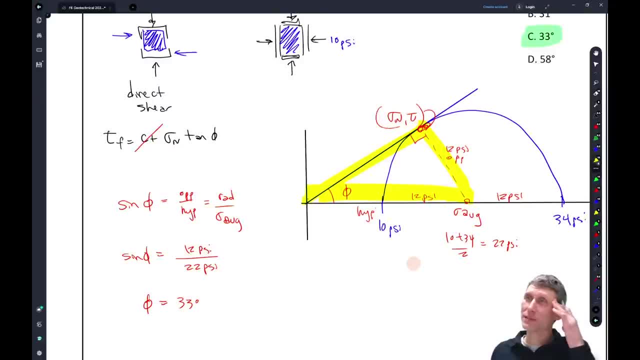 And honestly, on the test you're probably going to have some silly mistake where it's like: uh-oh, I made a mistake, you know, but hopefully they don't dominate and you guys are going to do a great job, And maybe even you write down the wrong thing, but you do it right anyway, because I still did opposite over adjacent here, or good grief. 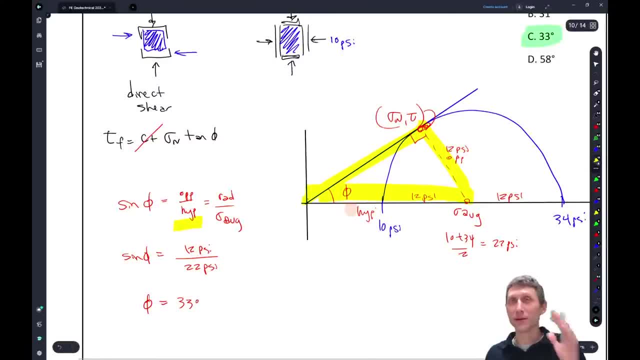 I said it wrong again: Opposite over hypotenuse. I still did opposite Over hypotenuse, even though I wrote it down wrong. So you know, maybe, maybe it comes from um. when I was younger I had a condition and it was hard for me to think sometimes. 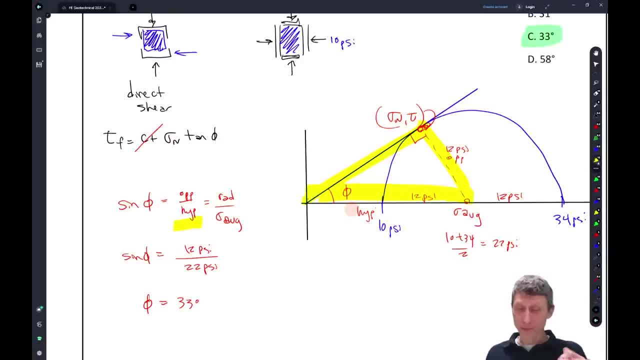 And my older brother. he just said you should just eat dirt three times a day. I'm really glad he told me about it. Sorry, That was supposed to be a joke. I think I'm really lucky that my older brother told me that. 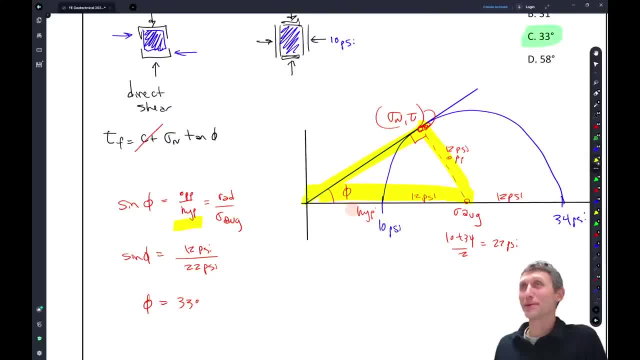 No, don't go eat dirt before your test. That's not going to make you any smarter. You know it's, it's, uh, it's. And when you ask for fresh ground coffee, um, make sure they don't put dirt in it. 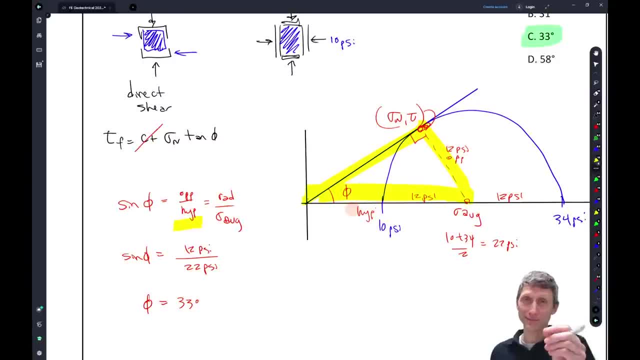 And you know there's no soil in fresh ground. You don't want the ground, you know them to grind. Sorry, The puns are just bad, but um, what gets bigger the more you take out of it. 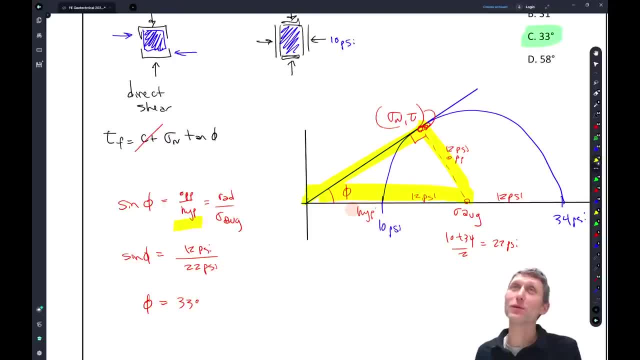 Um, the hole I'm digging myself, Okay, So there you go. So we'll end on those bad jokes. Um, sorry They're. they're probably not as funny today as as maybe some of the other ones, But, um, if you have questions, definitely shoot me. you know, reach out, shoot. a comment below.